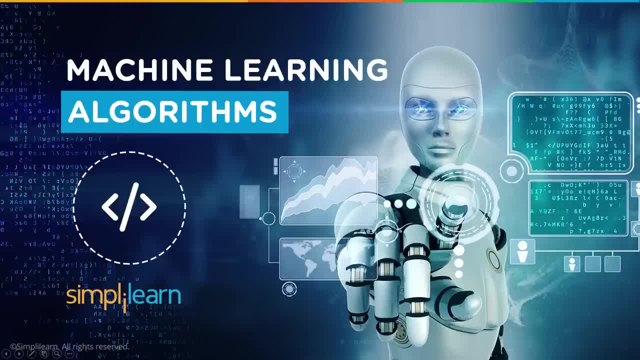 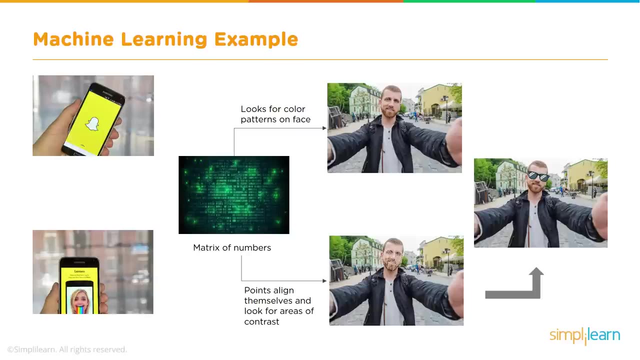 understand some of the most common algorithms, like linear regression, logistic regression and along the way. we will take some real-life examples Now. most of you must be using Snapchat to apply filters on your photos. but do you know how Snapchat recognizes your photo on the screen and puts filters on it? Even if there are multiple faces on the photo, it applies filters. 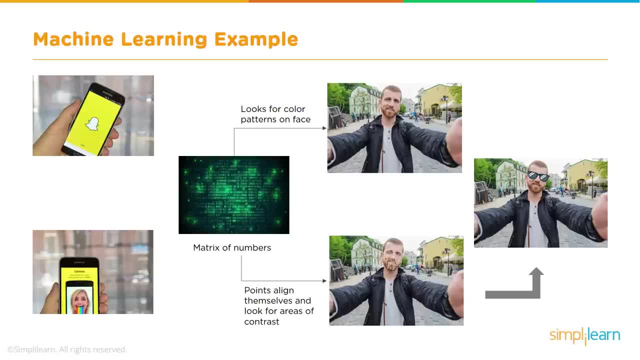 in the appropriate position. Snapchat actually does this using a technique called facial recognition, which in turn uses machine learning. The machine learning algorithm detects the features on your face, like the nose, the eyes, and it knows where exactly your eyes are, where exactly your nose is, and accordingly it applies the filters. We will take a few more examples as 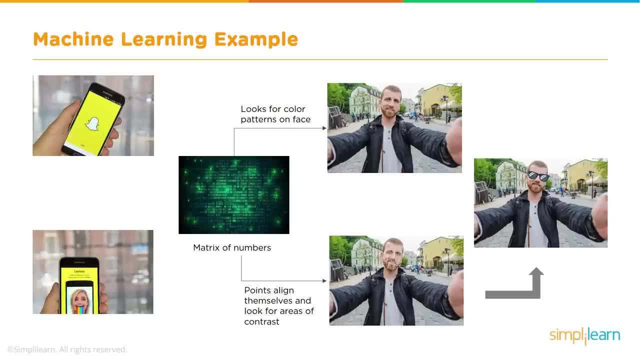 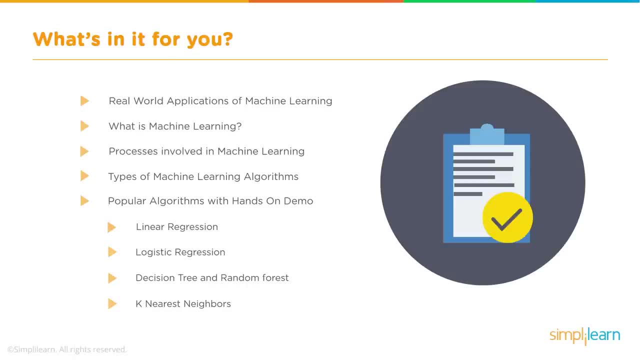 we move along and try to understand how machine learning algorithms can be applied to solve some of our real-life problems. So what will you learn from this video? We will talk about some real-world applications of machine learning. We will also see and understand what exactly is machine learning. 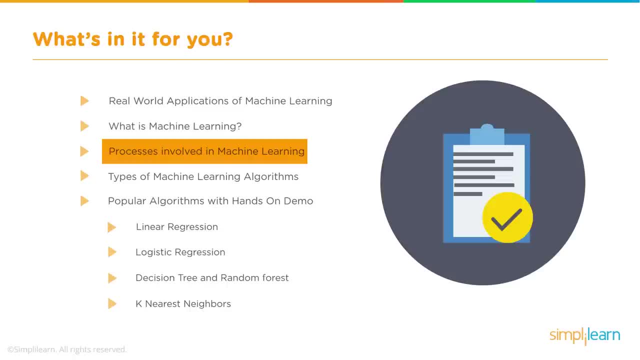 and how it works. We will also see the process involved in machine learning, the types of machine learning algorithms, and we will also see a few hands-on, including some code, Python code of the following algorithms: linear regression, logistic regression, decision tree and random forest and k- nearest neighbors. Okay, so let's get started. So let's consider some of. 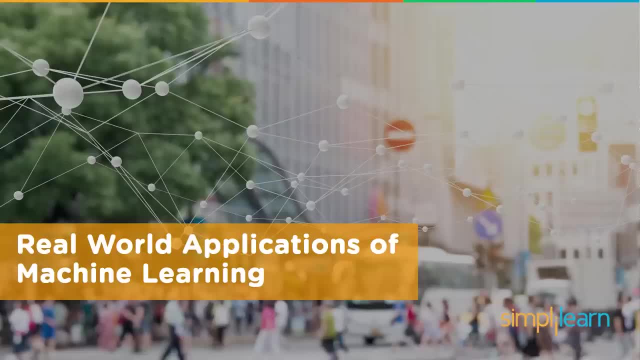 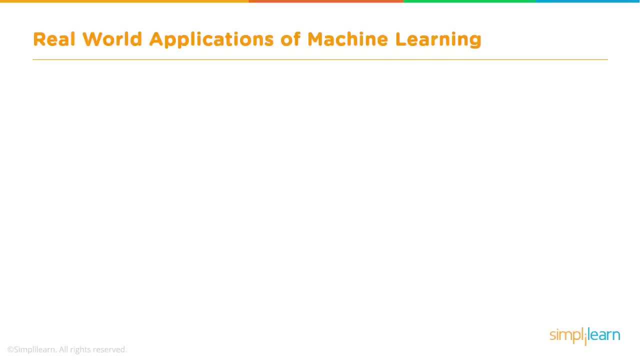 the real-world applications of machine learning. It's no longer just a buzzword. Machine learning is being used in a variety of industries to solve machine learning problems. Machine learning is used to solve a variety of problems. Facial recognition is one of them. It's becoming very 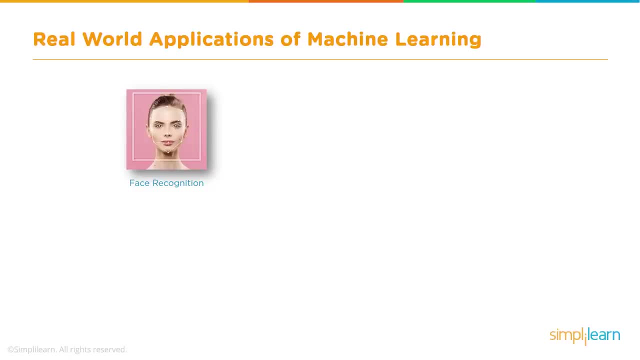 popular these days for security, for police, for solving crime. A lot of areas. facial recognition is being used. Voice recognition is another area. It's becoming very common these days. Some of you must be using Siri. That's an example of machine learning and voice recognition. Healthcare industry. 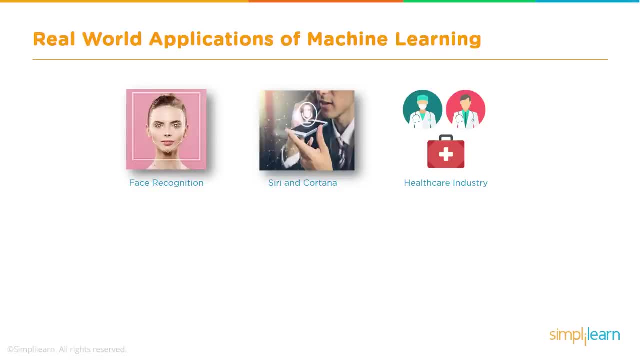 is another big area where machine learning is adopted in a very big way. As you all may be aware, diagnostics needs analysis of images, let's say like x-ray or MRI, And increasingly, because of the shortage of doctors, machine learning and artificial intelligence is being used to help. 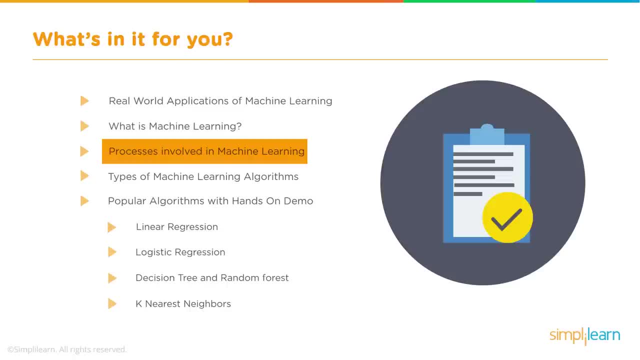 and how it works. We will also see the process involved in machine learning, the types of machine learning algorithms, and we will also see a few hands-on, including some code, Python code of the following algorithms: linear regression, logistic regression, decision tree and random forest and k- nearest neighbors. Okay, so let's get started. So let's consider some of. 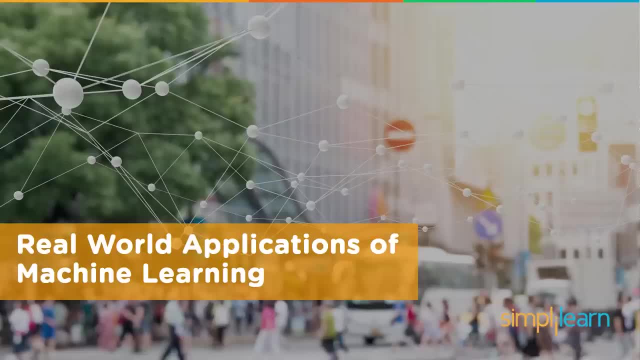 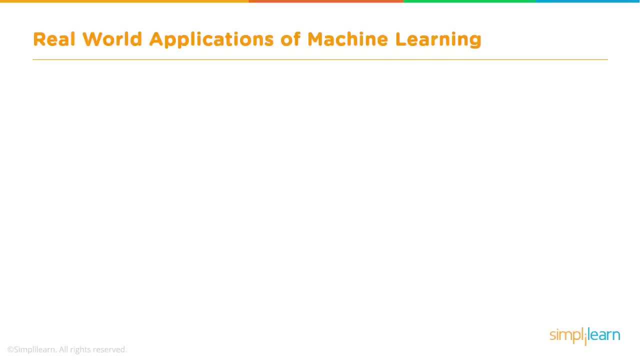 the real-world applications of machine learning. It's no longer just a buzzword. Machine learning is being used in a variety of industries to solve machine learning problems. Machine learning is used to solve a variety of problems. Facial recognition is one of them. It's becoming very 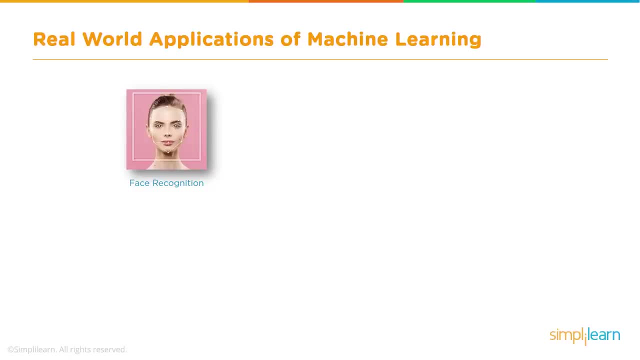 popular these days for security, for police, for solving crime. a lot of areas. facial recognition is being used. Voice recognition is another area. It's becoming very common these days. Some of you must be using Siri. That's an example of machine learning and voice recognition. Healthcare industry. 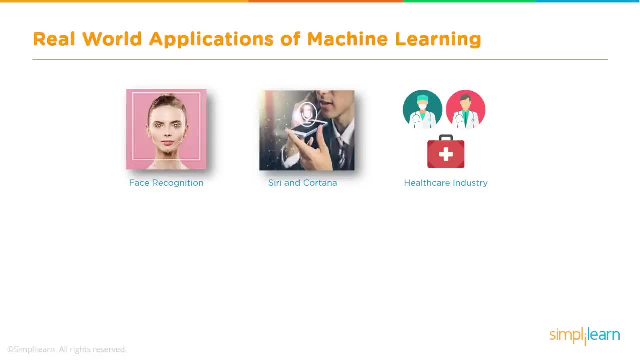 is another big area where machine learning is adopted in a very big way. As you all may be aware, diagnostics needs analysis of images, let's say like X-ray or MRI, And increasingly, because of the shortage of doctors, machine learning and artificial intelligence is being used to help. 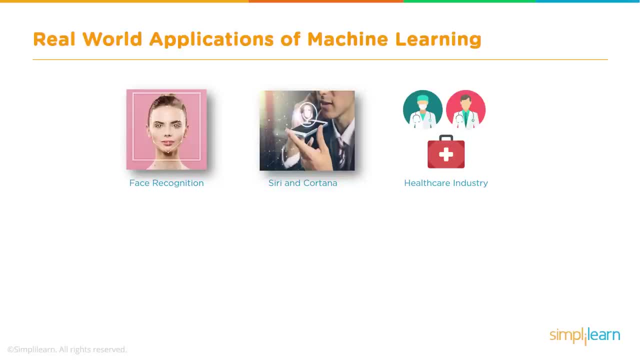 and support doctors in analyzing these images and identifying the advent of any diseases. Weather forecast is another area. Netflix has actually come up with a very interesting use case. You all must be aware of the House of Cards show on Netflix. so they did an analysis on their customer behavior. they got data. 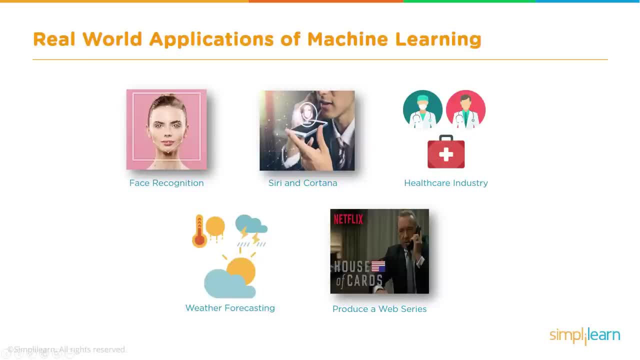 of their 30 million customers information about where they pause, where they fast-forward a video, and they used this information. they provided this information to their play rates and told them that this is what we want. this is, this is what our audience is looking for. these are the areas that interest them. 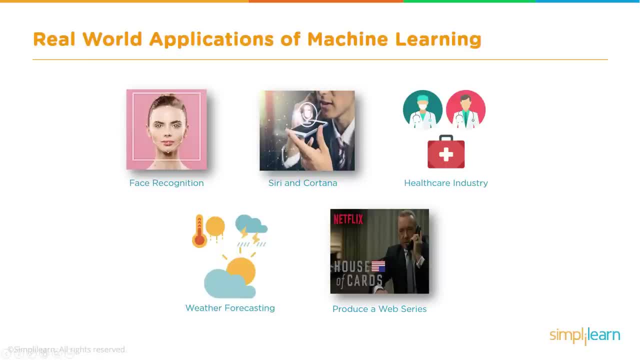 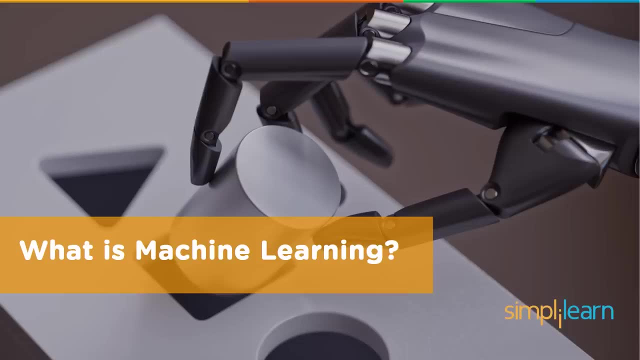 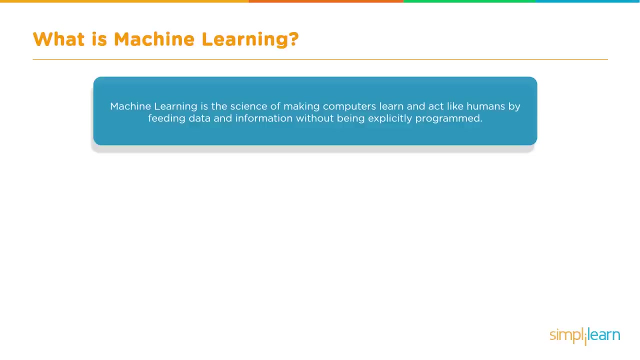 and these are the areas where they get bored, and the play rates wrote the scripts accordingly. this is really, really interesting and it actually brings a new era. so what is machine learning? machine learning is a science of making computers learn and act like humans. so here, when we say computers, 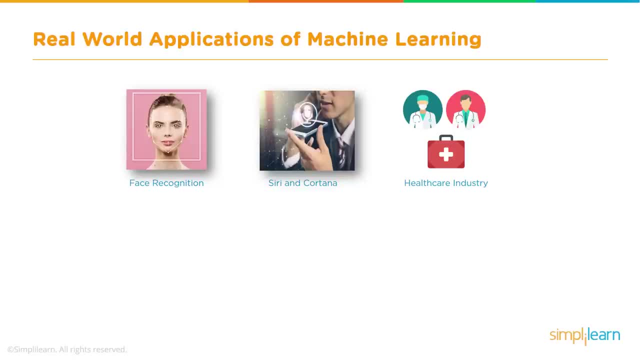 and support doctors in analyzing these images and identifying the advent of any diseases. Weather forecast is another area and in fact Netflix has actually come up with a very interesting use case. You all must be aware of the House of Cards show on Netflix. so they did an analysis on their customer behavior. they got data. 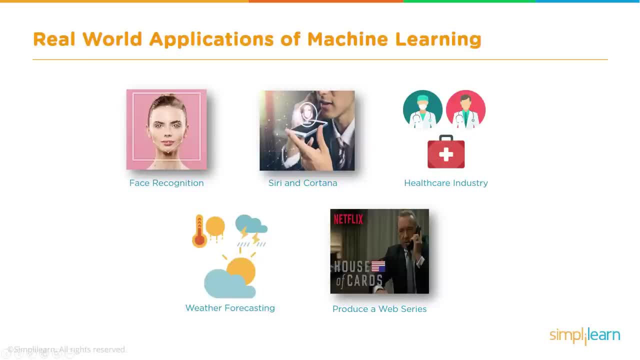 of their 30 million customers information about where they pause, where they fast-forward a video, and they used this information. they provided this information to their play rates and told them that this is what we want. this is, this is what our audience is looking for. these are the areas that interest them. 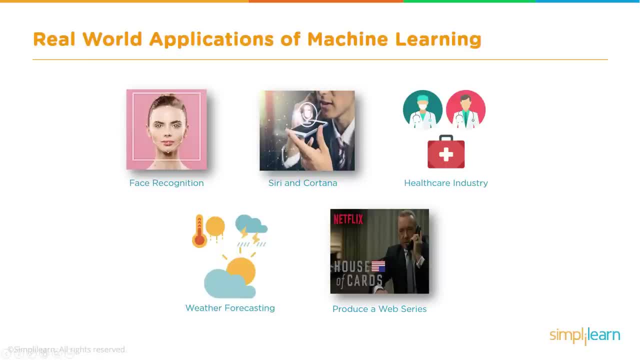 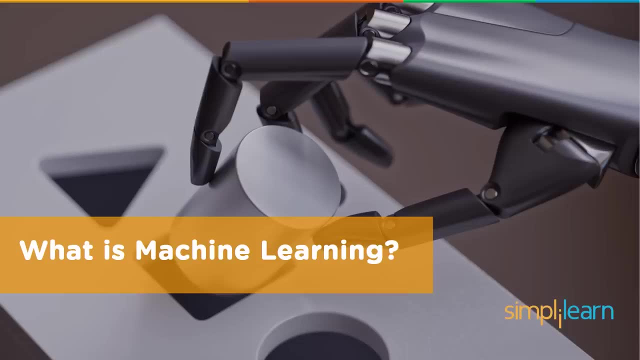 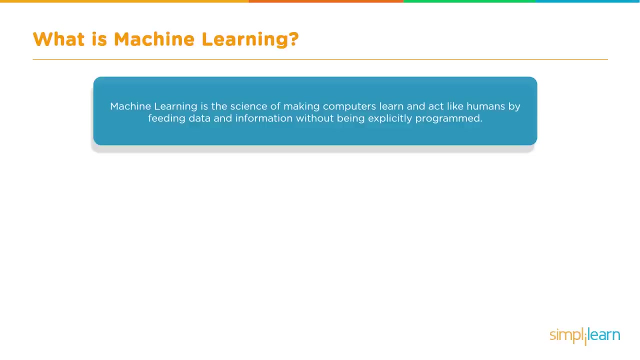 and these are the areas where they get bored, and the play rates wrote the scripts accordingly. this is really, really interesting and it actually brings a new era. so what is machine learning? machine learning is a science of making computers learn and act like humans. so here, when we say computers, 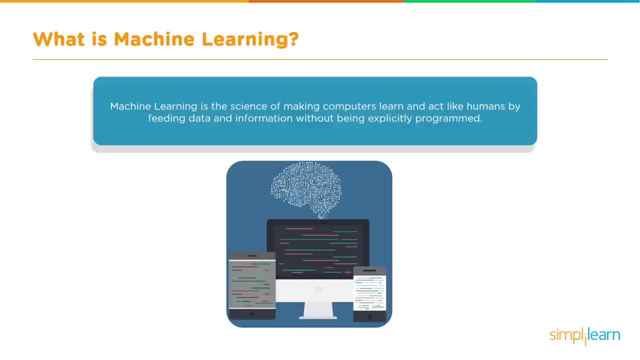 very often what comes to our mind is writing a piece of code or program and telling the computer, step by step, what to do. but in machine learning we don't do that. the system learns on its own. we just provide past data, historical data, what we call as labeled data, and 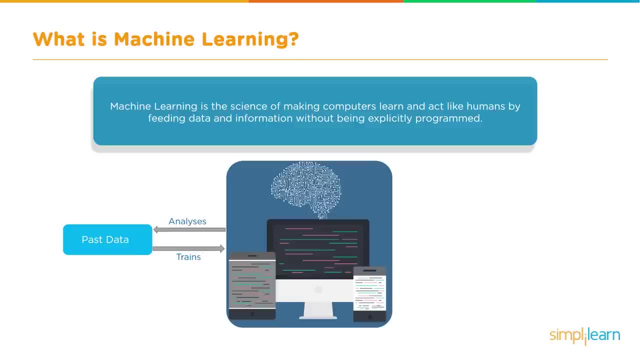 the system learns during the process, what is known as training process. we tell the system whether the outcomes are right or wrong, and that feedback is taken by the system and it corrects itself. and that's how it learns till it's correct gives the correct output. for most of the cases, obviously, it won't be. 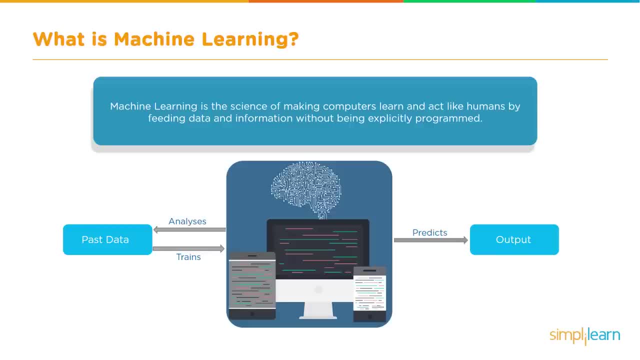 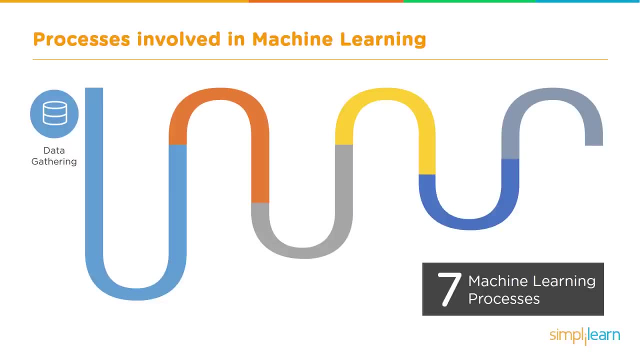 100 correct, but the aim is to get as accurate as possible. so let's take you through step by step, process of machine learning. the first step in machine learning is data gathering. machine learning needs a lot of past data, especially we will see a little later supervised learning. we will see what. 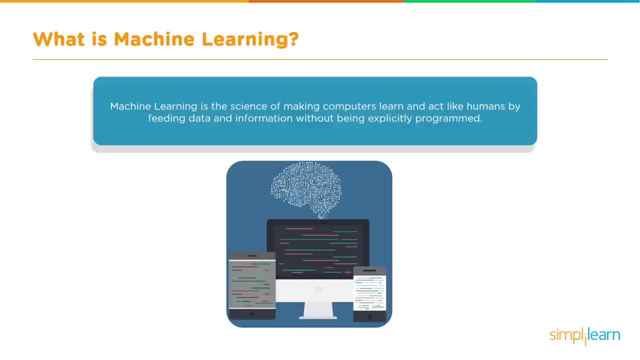 very often what comes to our mind is writing a piece of code or program and telling the computer, step by step, what to do. but in machine learning we don't do that. the system learns on its own. we just provide past data, historical data, what we call as labeled data, and 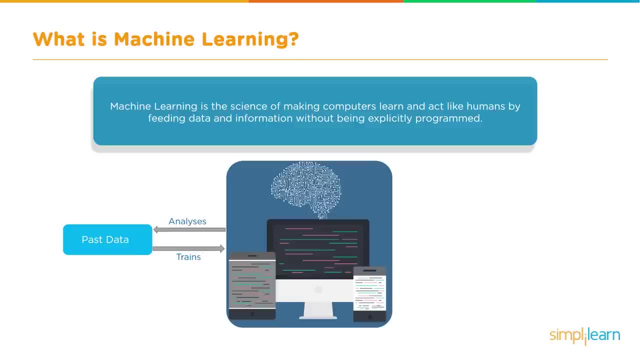 the system learns during the process, what is known as training process. we tell the system whether the outcomes are right or wrong, and that feedback is taken by the system and it corrects itself. and that's how it learns till it's correct gives the correct output. for most of the cases, obviously, it won't be. 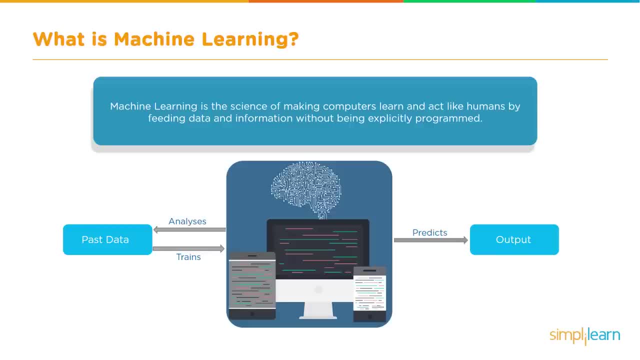 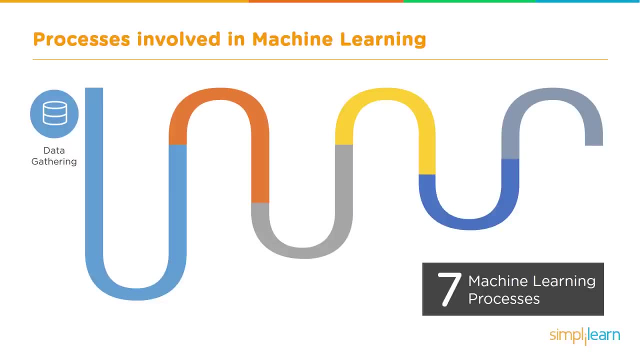 100 correct, but the aim is to get as accurate as possible. so let's take you through step by step, process of machine learning. the first step in machine learning is data gathering. machine learning needs a lot of past data, especially we will see a little later supervised learning. we will see what. 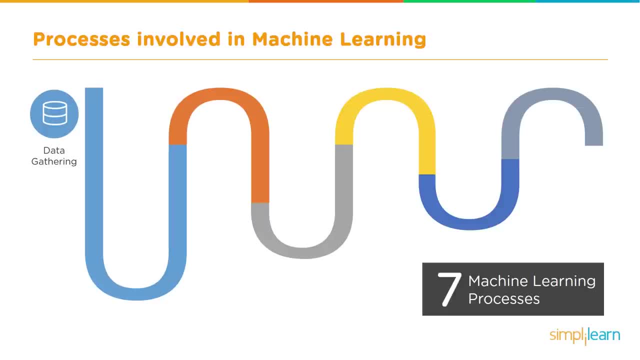 that is in a little while, but that's the most common form of learning. so the first step there is data gathering. you need to have sufficient historical data. then the second step is pre-processing of this data so that this can be used for the machine learning process. the raw data cannot be used. 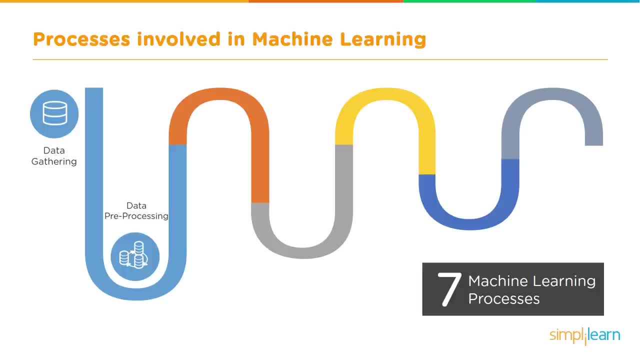 directly, so it needs to be pre-processed before it is fed into the machine learning system. the next step is to choose a model. so what kind of algorithm and what kind of model within that algorithm are we going to use? and then we need to train this model. so before training the model, it's just like a 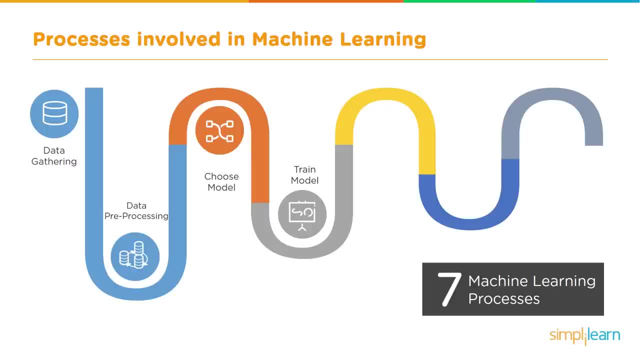 blank model and after training it becomes a trained model. and once we train the model, we need to also test it to make sure it is predicting correctly. it's working fine, with minimum errors, and subsequently it will be deployed and once again it may have to be tuned from. 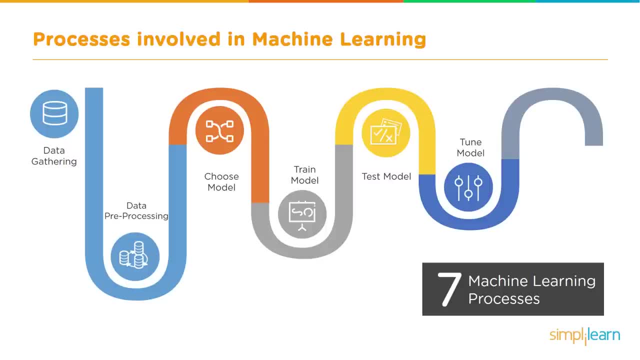 time to time, or fine-tuned from time to time to improve the accuracy, and so on and so forth. after training the model, we have to test the model, and during testing we may have to, we may find out that the accuracy is not good enough, so we may have to tune the model, we may change some parameters and 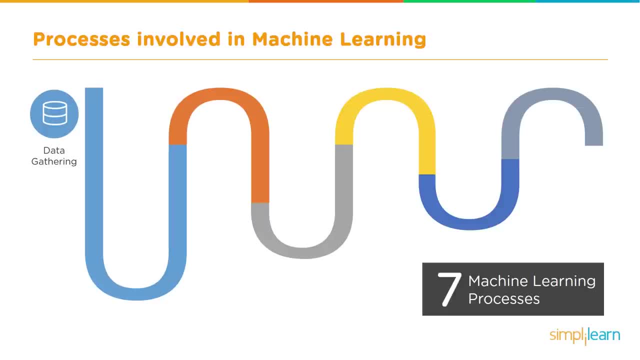 that is in a little while, but that's the most common form of learning. so the first step there is data gathering. you need to have sufficient historical data. then the second step is pre-processing of this data so that this can be used for the machine learning process. the raw data cannot be used. 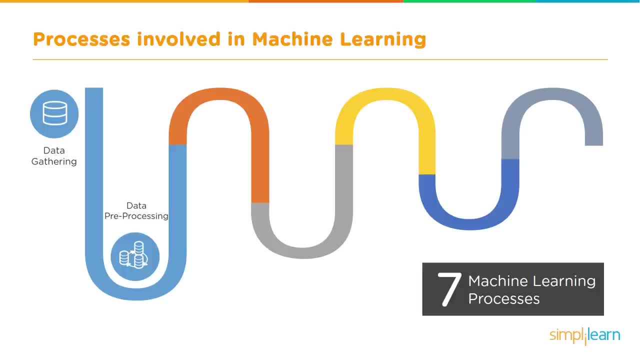 directly, so it needs to be pre-processed before it is fed into the machine learning system. the next step is to choose a model. so what kind of algorithm and what kind of model within that algorithm are we going to use? and then we need to train this model. so before training the model, it's just like a 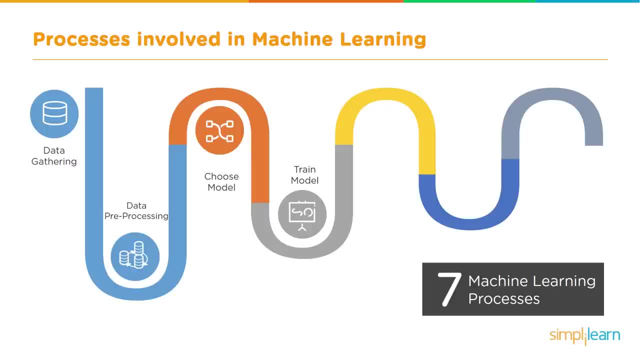 blank model and after training it becomes a trained model. and once we train the model, we need to also test it to make sure it is predicting correctly. it's working fine, with minimum errors, and subsequently it will be deployed and once again it may have to be tuned from. 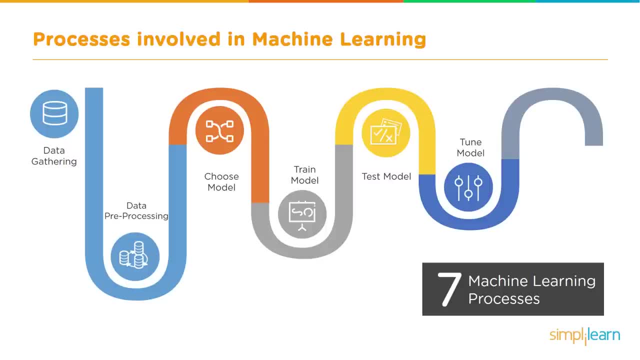 time to time, or fine-tuned from time to time to improve the accuracy, and so on and so forth. after training the model, we have to test the model, and during testing we may have to, we may find out that the accuracy is not good enough, so we may have to tune the model, we may change some parameters and 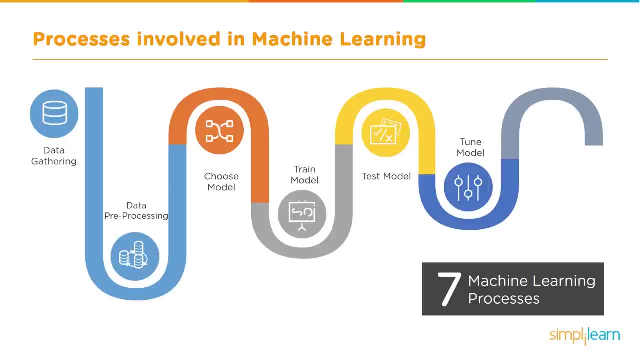 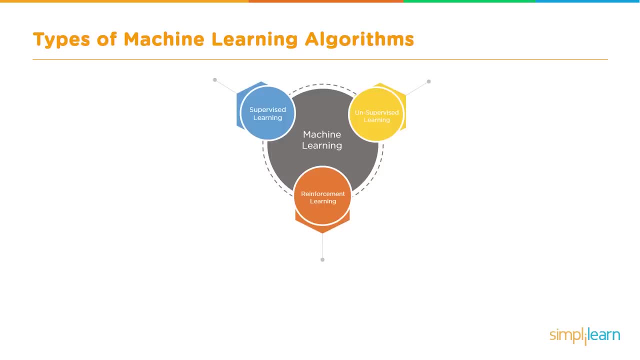 run through this process once again, perform the training once again, so it can be an iterative process, and once the model is ready, then we deploy it to do the predictions. what are the different types of machine learning algorithms? machine learning algorithms are broadly classified into three types: the 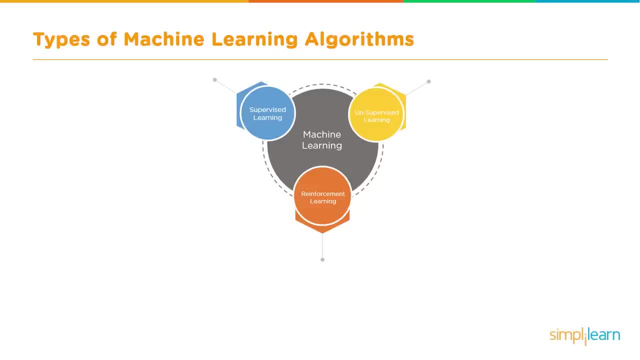 supervised learning, unsupervised learning and reinforcement learning. supervised learning in turn consists of techniques like regression and classification, and unsupervised learning we use techniques like association and clustering, and reinforcement learning is a recently developed technique and it is very popular in gaming. some of you must have heard about AlphaGo, so 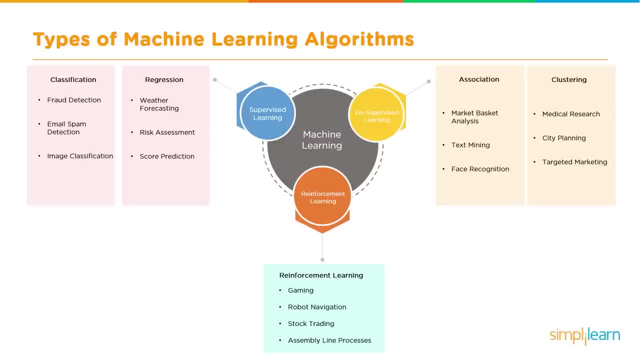 this was developed using reinforcement learning, primary difference between supervised learning and unsupervised learning: supervised learning is used when we have historical data and we have labeled data, which means that we know how the data is classified. so we know the classes if we are doing classification, or we know the values when we are doing regression, so if we have historical data, 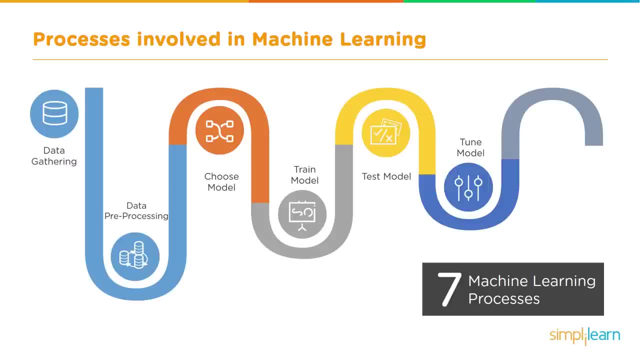 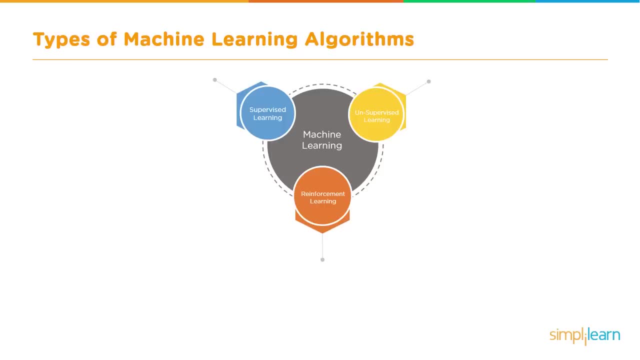 run through this process once again, perform the training once again, so it can be an iterative process, and once the model is ready, then we deploy it to do the predictions. what are the different types of machine learning algorithms? machine learning algorithms are broadly classified into three types: the 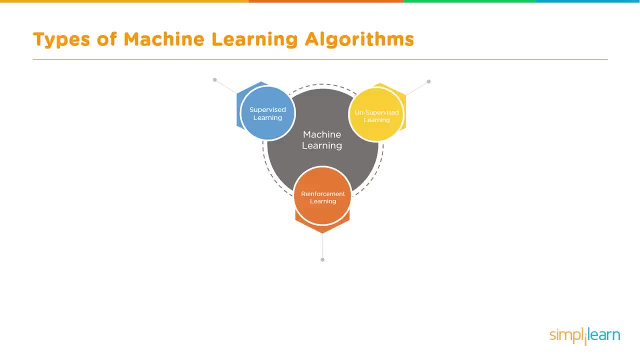 supervised learning, unsupervised learning and reinforcement learning. supervised learning in turn consists of techniques like regression and classification, and unsupervised learning we use techniques like association and clustering, and reinforcement learning is a recently developed technique and it is very popular in gaming. some of you must have heard about AlphaGo, so 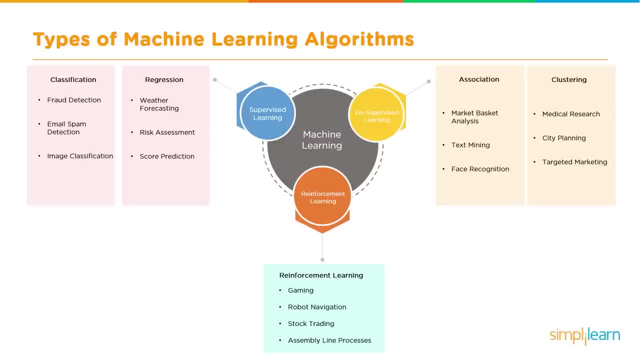 this was developed using reinforcement learning, primary difference between supervised learning and unsupervised learning: supervised learning is used when we have historical data and we have labeled data, which means that we know how the data is classified. so we know the classes if we are doing classification, or we know the values when we are doing regression, so if we have historical data, 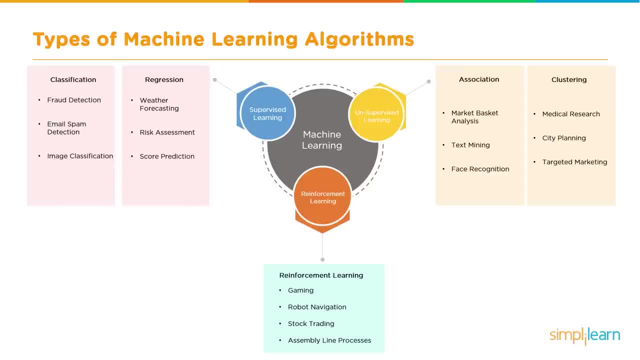 with these values, which are known as labels, then we use supervised learning. in case of unsupervised learning, we do not have past labeled data, historical labeled data, so we use techniques like association and clustering to maybe form clusters or new classes maybe, and then we move from there. in case of reinforcement learning, the 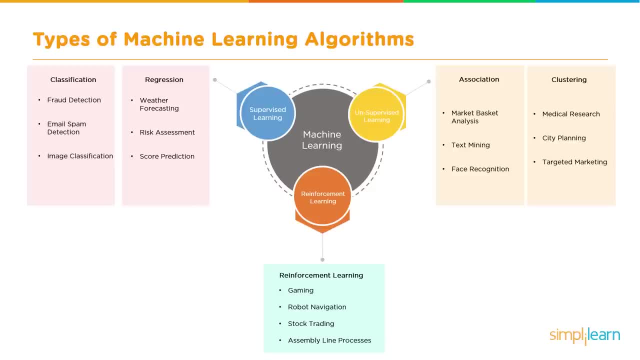 system learns pretty much from scratch. there is an agent and there is an environment. the agent is given a certain target and it is rewarded when it is moving towards that target and it is penalized if it is moving in a direction which is not achieving that target. so it's. 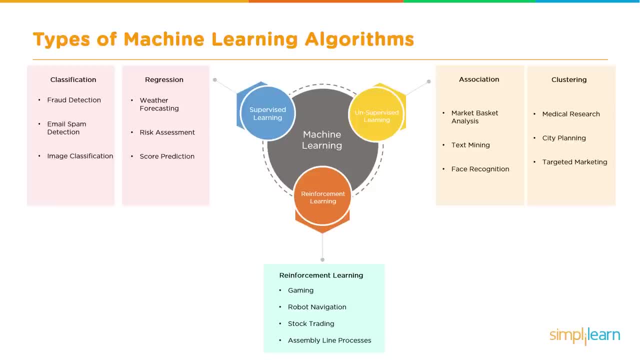 more like a carrot and stick model. so what is the difference between these three types of algorithms? supervised algorithms or supervised learning algorithms are used when you have a specific target value that you would like to predict. the target could be categorical, having two or more possible outcomes, or classes, if you will. that is what is classification, or the target. 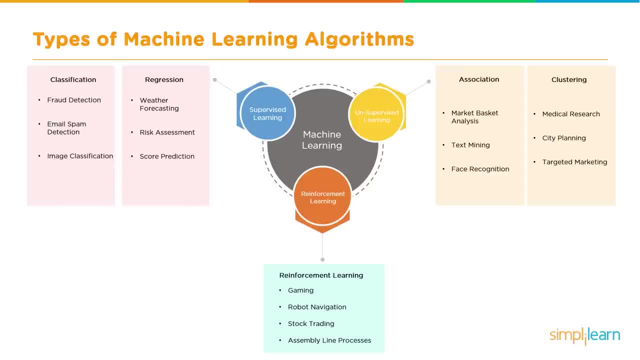 with these values, which are known as labels, then we use supervised learning. in case of unsupervised learning, we do not have past labeled data, historical labeled data, so we use techniques like association and clustering to maybe form clusters or new classes maybe, and then we move from there. in case of reinforcement learning, the 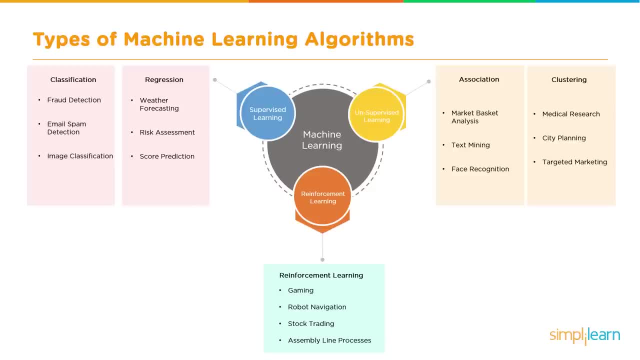 system learns pretty much from scratch. there is an agent and there is an environment. the agent is given a certain target and it is rewarded when it is moving towards that target and it is penalized if it is moving in a direction which is not achieving that target. so it's. 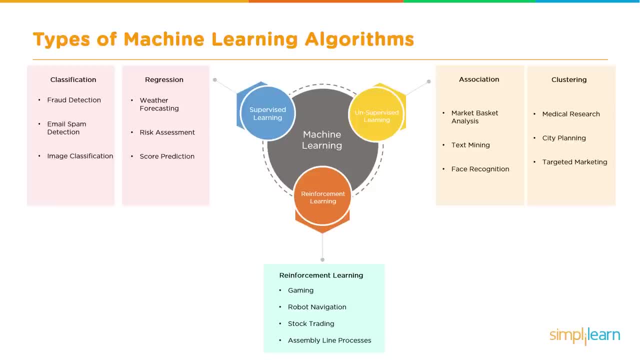 more like a carrot and stick model. so what is the difference between these three types of algorithms? supervised algorithms or supervised learning algorithms are used when you have a specific target value that you would like to predict. the target could be categorical, having two or more possible outcomes, or classes, if you will. that is what is classification, or the target. 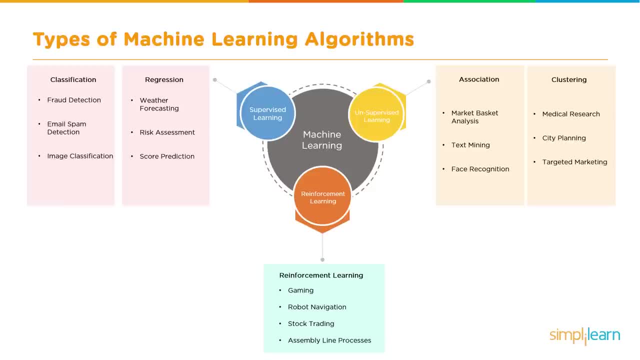 could be a value which can be measured, and that's where we use regression, like, for example, weather forecasting. you want to find the temperature, whereas in classification you want to find out whether or not a fraud or if it is email spam, whether it is spam or not spam. so that is a 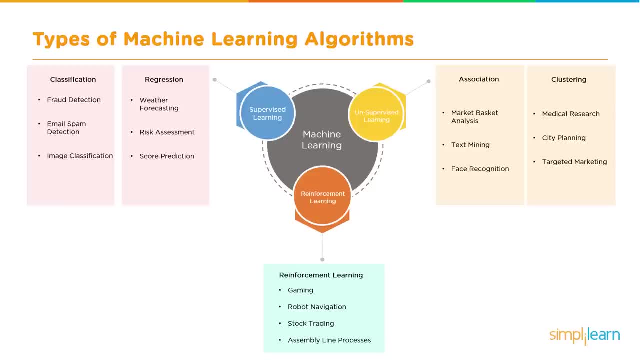 classification example. so if you know- or this is known as labeled information- if you have the labeled information, then you use supervised learning. in case of unsupervised learning, we have input data but we don't have the labels or what the output is supposed to be. so that is when 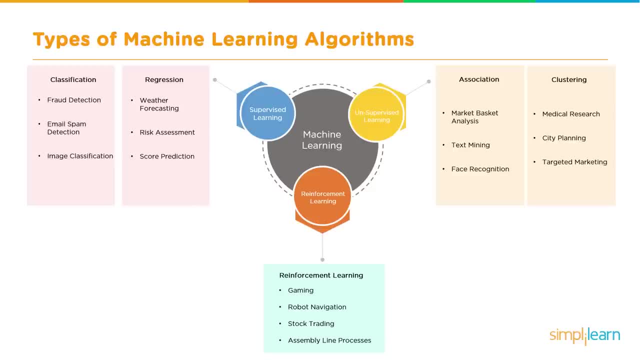 we use unsupervised learning techniques like clustering and association, and we try to analyze the data. in case of reinforcement learning, it allows the agent to automatically determine the ideal behavior within a specific context, and it has to do this to maximize the performance, like, for example, playing a game. so the agent is told that you. 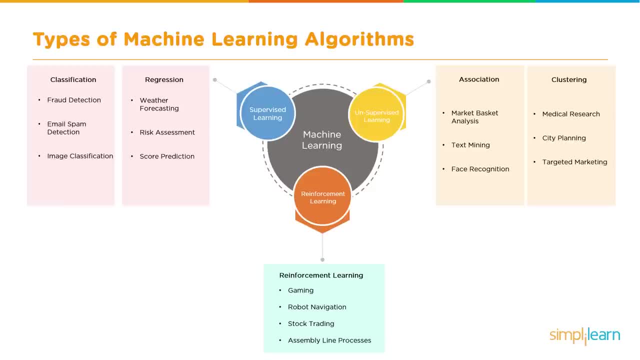 could be a value which can be measured, and that's where we use regression, like, for example, weather forecasting. you want to find the temperature, whereas in classification you want to find out whether or not a fraud or if it is email spam, whether it is spam or not spam. so that is a 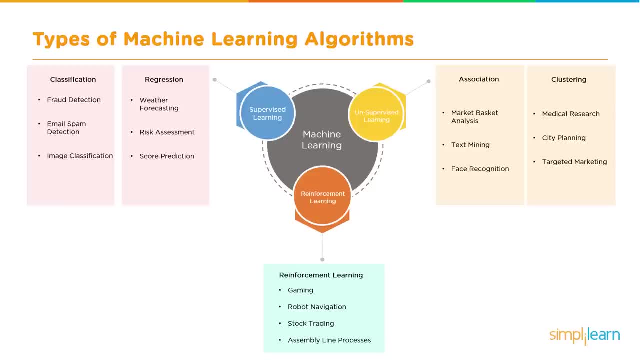 classification example. so if you know- or this is known as labeled information- if you have the labeled information, then you use supervised learning. in case of unsupervised learning, we have input data but we don't have the labels or what the output is supposed to be. so that is when 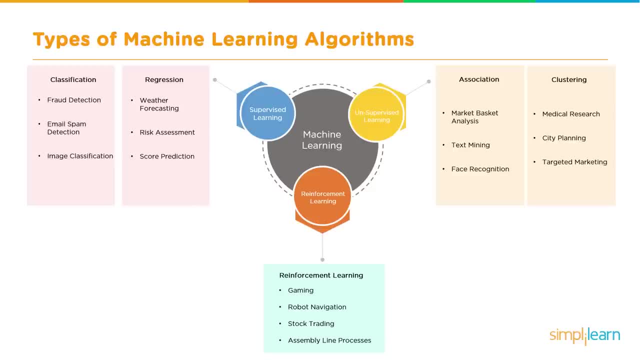 we use unsupervised learning techniques like clustering and association, and we try to analyze the data. in case of reinforcement learning, it allows the agent to automatically determine the ideal behavior within a specific context, and it has to do this to maximize the performance, like, for example, playing a game. so the agent is told that you. 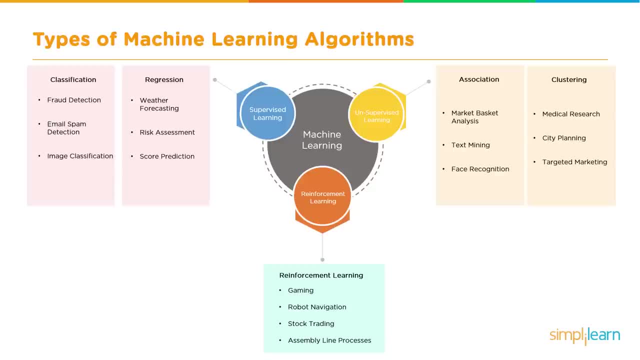 need to score the maximum score possible without losing lives. so that is a target that is given to the agent and it is allowed to learn from scratch. play the game itself multiple times and slowly it will learn the behavior which will increase the score and keep the lives to the maximum. that's an example of reinforcement learning, so we will discuss. 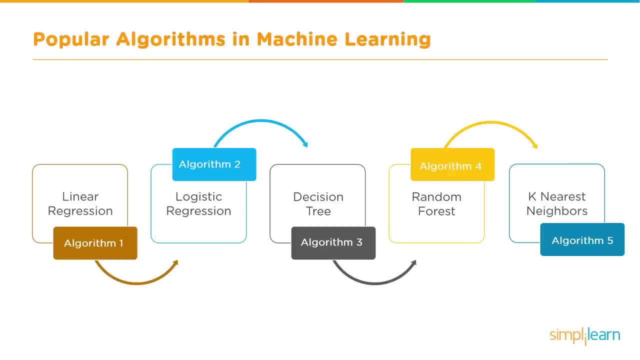 about some of the most popular algorithms in machine learning. a few of them are listed here. this is by no means an exhaustive list. there are really a lot of algorithms available out there, but these are some of the most common ones. what are these algorithms? linear regression, logistic. 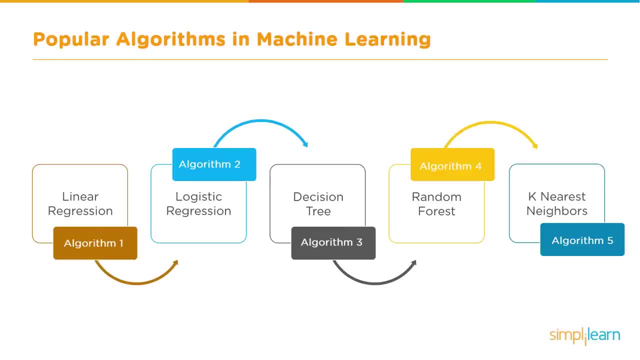 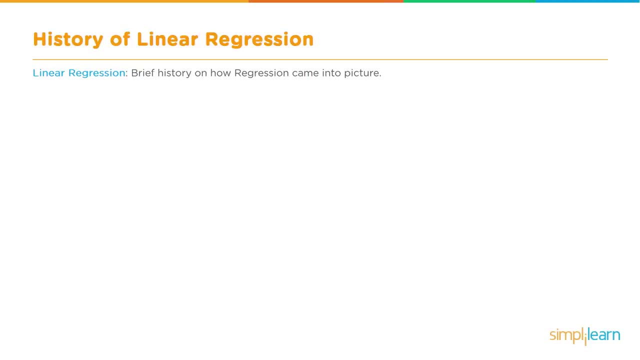 regression decision tree, random forest and k nearest neighbors. so let's look at each of these in detail. linear regression: a little history about linear regression. Sir Francis Galton is credited with the discovery of the linear regression model. so what he did was he started studying the heights of father and son to predict. 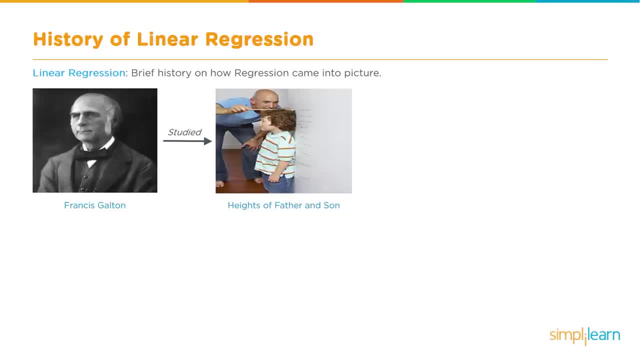 the son's height or the child's height even before he or she is born. so he collected enough data of the heights of father and the respective sons. he plotted this data on the x and y axis and he drew a line in such a way that the distance of 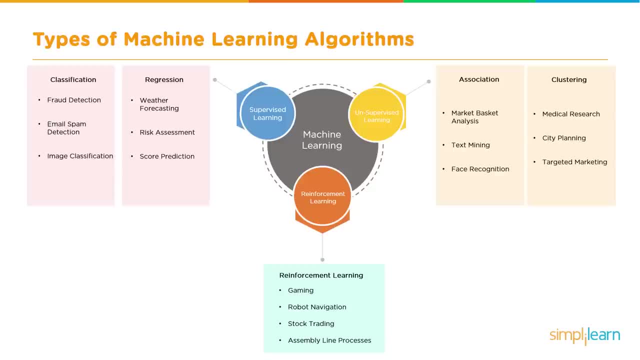 need to score the maximum score possible without losing lives. so that is a target that is given to the agent and it is allowed to learn from scratch. play the game itself multiple times and slowly it will learn the behavior which will increase the score and keep the lives to the maximum. that's an example of reinforcement learning, so we will discuss. 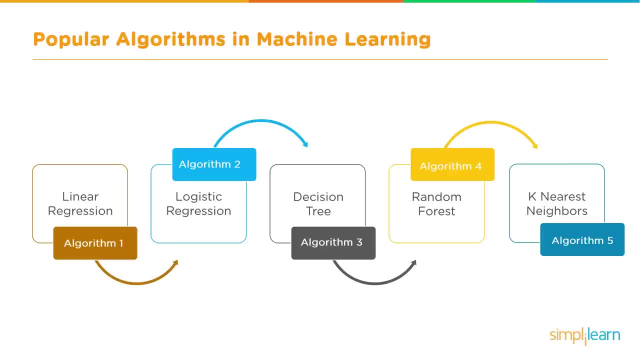 about some of the most popular algorithms in machine learning. a few of them are listed here. this is by no means an exhaustive list. there are really a lot of algorithms available out there, but these are some of the most common ones. what are these algorithms? linear regression, logistic. 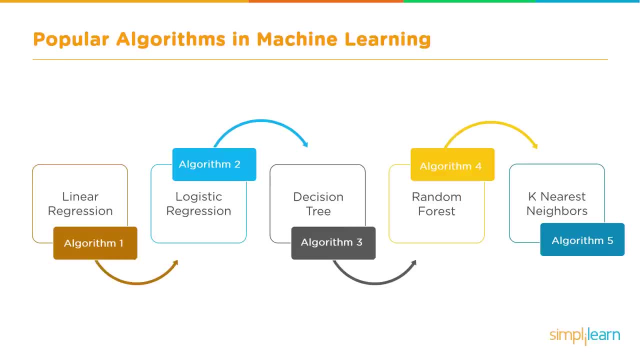 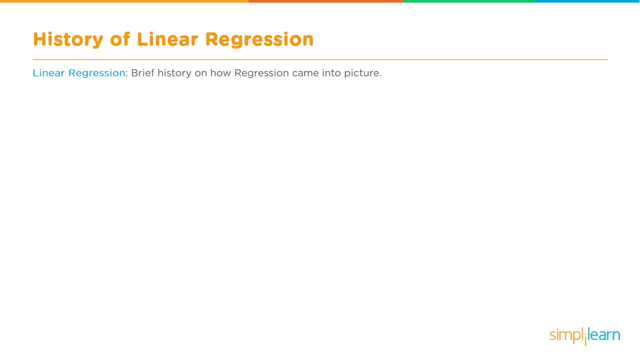 regression decision tree, random forest and k nearest neighbors. so let's look at each of these in detail. linear regression: a little history about linear regression. Sir Francis Galton is credited with the discovery of the linear regression model. so what he did was he started studying the heights of father and son to predict. 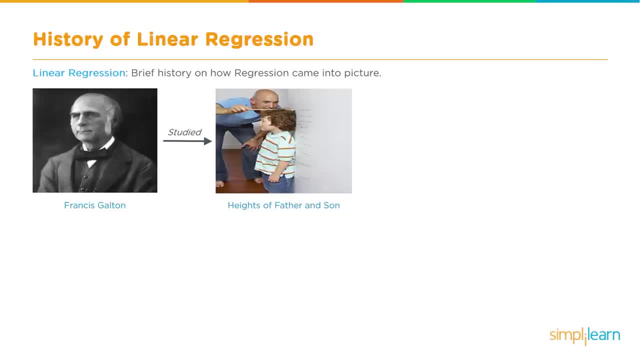 the son's height or the child's height even before he or she is born. so he collected enough data of the heights of father and the respective sons. he plotted this data on the x and y axis and he drew a line in such a way that the distance of 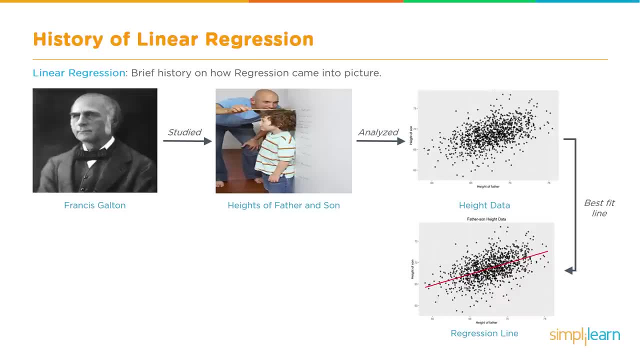 these points from the line was the least, which is now what we call it as mean square error. so at that time this term was probably not there, but that's what he did. and then he was able to use this line to predict the height of the child which was yet to be born, based on the height of the father. so 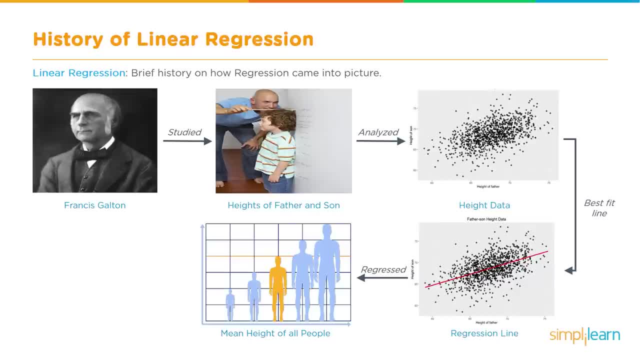 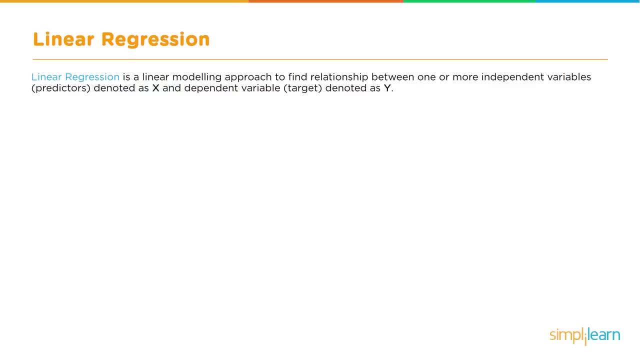 that was the very beginning or very initial phase of linear regression algorithm. so that was a little bit of history. but what is linear regression? so linear regression is a way of modeling a linear model, creating a linear model to find the relationship between one or more independent variables denoted. 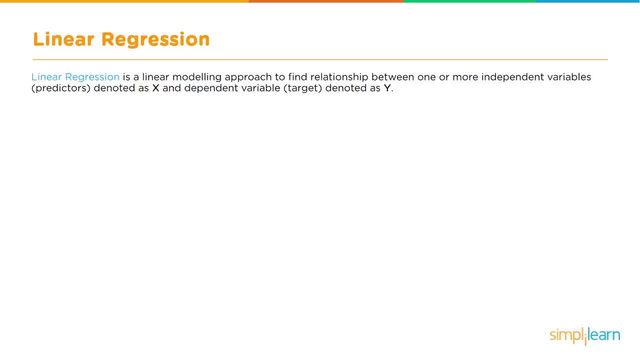 by X and a dependent variable, which is also known as the target and denoted as Y. a few examples are shown here. let's say we are going to plot the sales of ice cream and the temperature, so temperature on the x-axis and the sales on the y-axis, and this is how the data would look. and 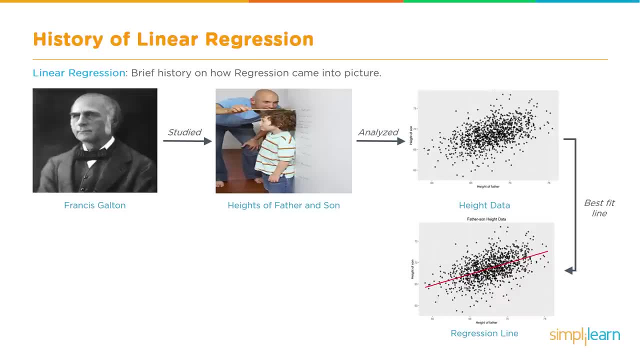 these points from the line was the least, which is now what we call it as mean square error. so at that time this term was probably not there, but that's what he did. and then he was able to use this line to predict the height of the child which was yet to be born, based on the height of the father. so 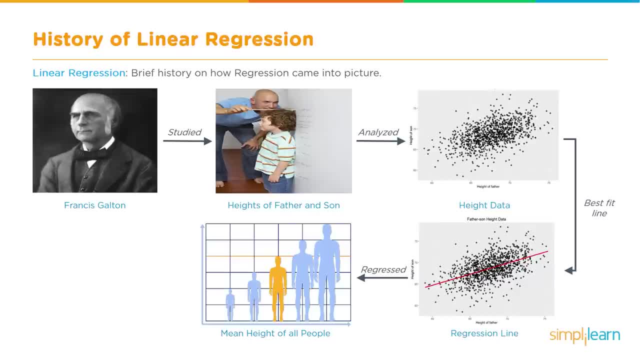 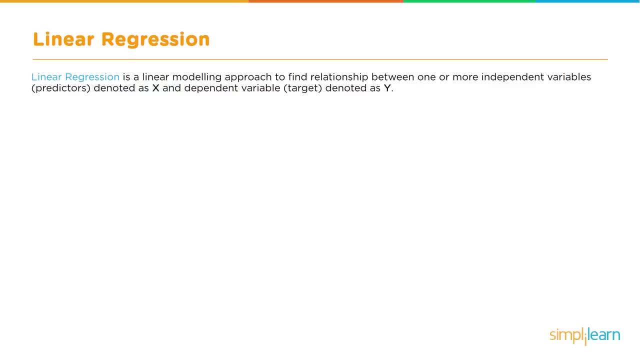 that was the very beginning or very initial phase of linear regression algorithm. so that was a little bit of history. but what is linear regression? so linear regression is a way of modeling a linear model, creating a linear model to find the relationship between one or more independent variables denoted. 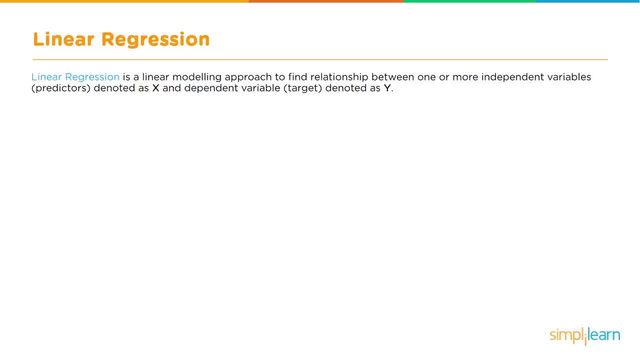 by X and a dependent variable, which is also known as the target and denoted as Y. a few examples are shown here. let's say we are going to plot the sales of ice cream and the temperature, so temperature on the x-axis and the sales on the y-axis, and this is how the data would look. and 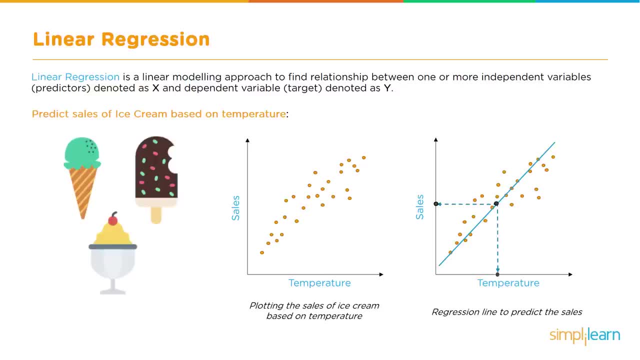 if we draw a line in such a way that the distance of each of these points from this line is minimum, that is known as a regression line or the best fit line. so regression is all about finding this line, because it is a straight line, linear, and the equation doesn't have any non-linear component. 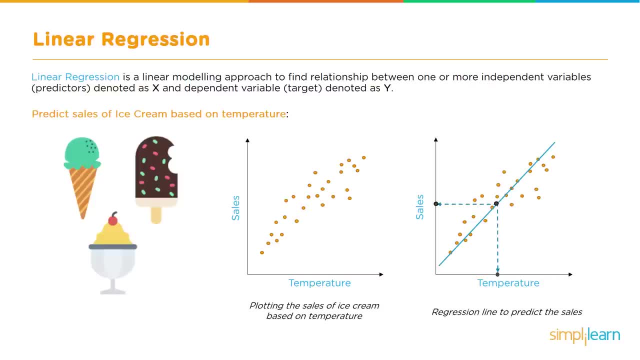 which means we do not have x to the power of 2 or 3 or any of this. so this is simple linear regression. and simple linear regression is when there is only one independent variable, so there is only one X. so that is simple linear regression. so let's see how this is actually done. so linear. 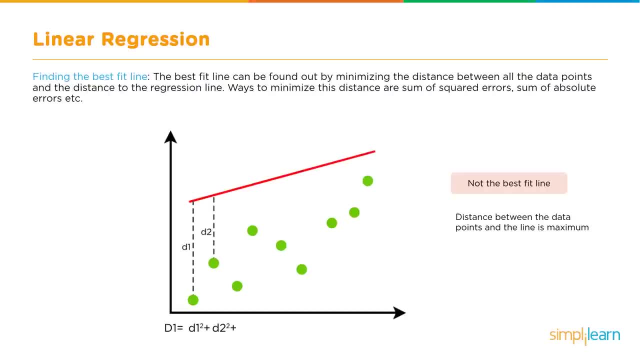 regression is all about finding the best fit line, and the way it is done is in a recursive manner. so first a random line is drawn and the distance is calculated from this line of all the points, as you can see in this example, and that distance is known as the error and to ensure that there are no negative values, this is squared. 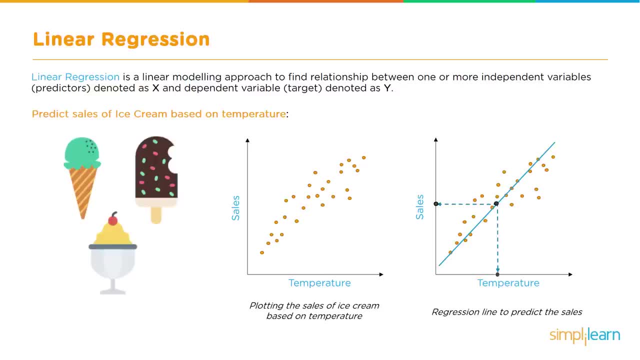 if we draw a line in such a way that the distance of each of these points from this line is minimum, that is known as the regression line or the best fit line. so regression is all about finding this line, and it is called linear regression because it is a straight line, linear, and the equation doesn't have any non-linear component. 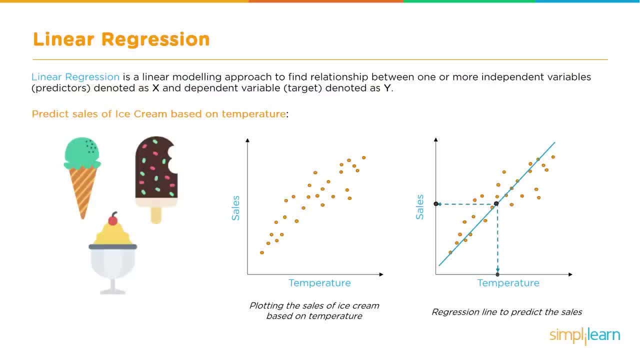 which means we do not have x to the power of 2 or 3 or any of this. so this is simple linear regression. and simple linear regression is when there is only one independent variable, so there is only one X. so that is simple linear regression. so let's see how this is actually done. so linear. 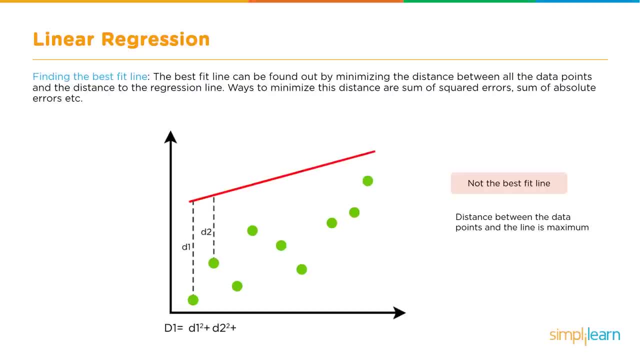 regression is all about finding the best fit line, and the way it is done is in a recursive manner. so first a random line is drawn and the distance is calculated from this line of all the points, as you can see in this example, and that distance is known as the error and to ensure that there are no negative values, this is squared. 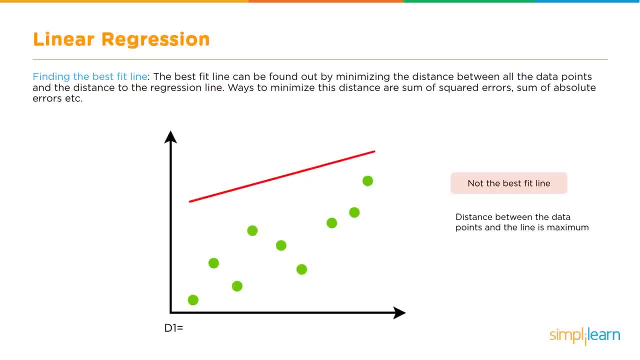 so we actually take the square of the distance of the point from the line and add it up, and we ensure that at the end, this sum, which is known as the sum of squared errors, is the minimum. so, as you can see, this is where we start, and then we keep changing the line in such a way and calculate. 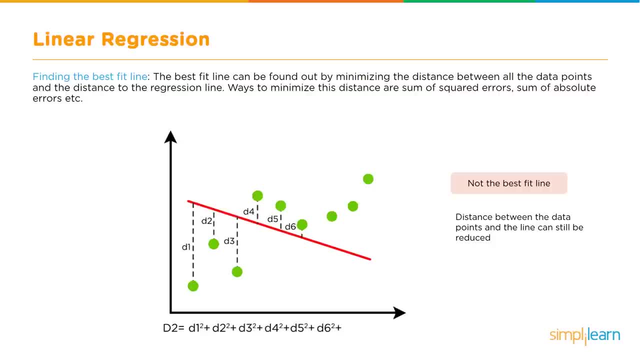 the distance once again, the sum of the squares once again. and here again you will see that this is probably not minimum, and we keep changing this, unless until we get a line where this value is minimum. so here we find that the sum of the squares of the distance, which is also the sum of squared errors, capital D denoted. 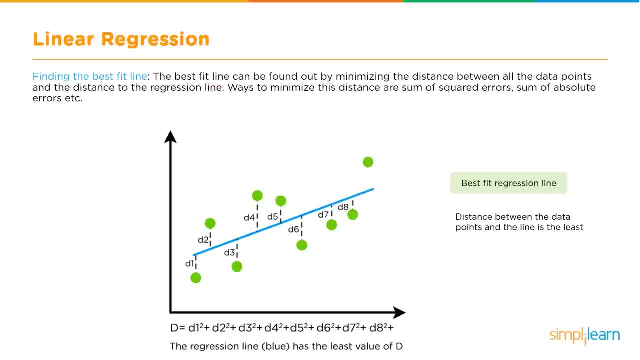 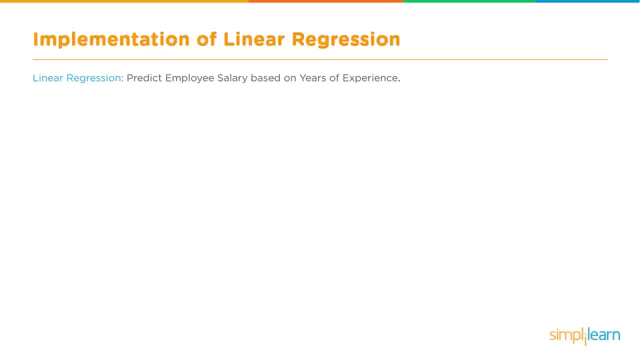 by capital D is minimum. so now we found the best fit regression line. so this is a recursive process, it's an iterative process and this is what behind the scenes. this is what happens when we try to do linear regression. now we'll take an example of a linear regression and we will actually 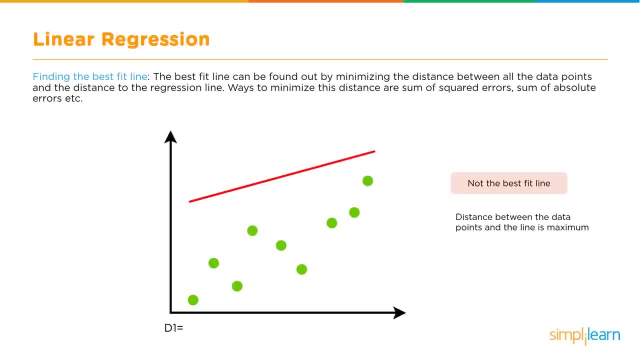 so we actually take the square of the distance of the point from the line and add it up, and we make sure that at the end, this sum, which is known as the sum of squared errors, is the minimum. so, as you can see, this is where we start, and then we keep changing the line in such a way and calculate the. 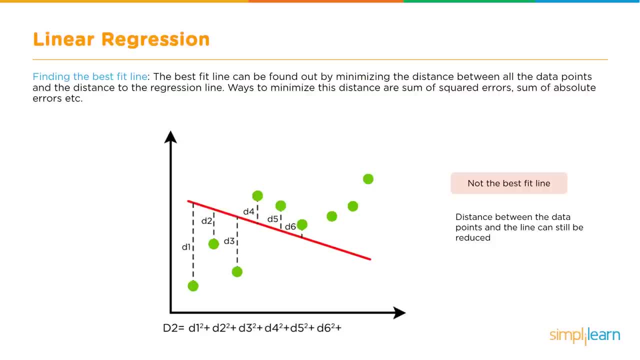 distance once again, the sum of the squares once again. and here again you will see that this is probably not minimum, and we keep changing this, unless until we get a line where this value is minimum. so here we find that the sum of the squares of the distance, which is also the sum of squared errors, capital D denoted. 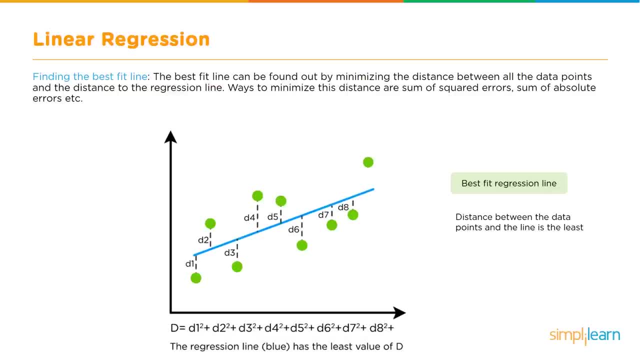 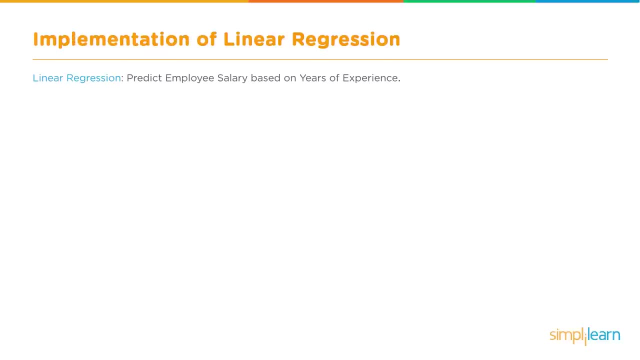 by capital D is minimum. so now we found the best fit regression line. so this is a recursive process, it's an iterative process and this is what behind the scenes. this is what happens when we try to do linear regression. now we'll take an example of a linear regression and we will actually demonstrate. 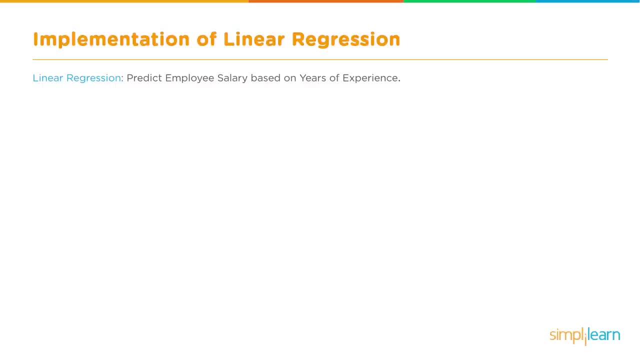 this using Python and we will be using book for this case. you are familiar with jupyter notebook. i think that would be very helpful and if you need the data set, please put a comment under this video so that we can provide you with the data set before we go there. just let's try to understand what this example is all about. 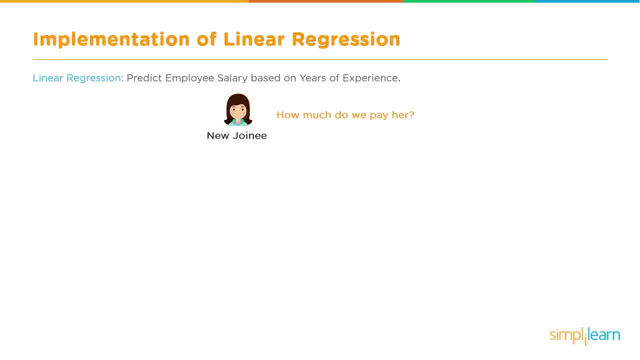 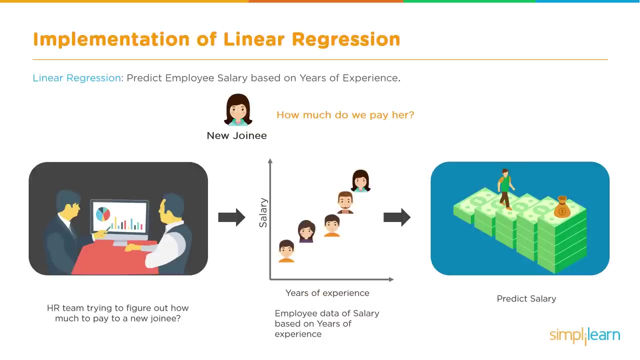 let's say there is a new joining joining the company and we want to determine what should be the pay or the salary for this new joining, and for that we already have the labeled data, which is the details of our employees, based on their years of experience and their salaries. and for the new 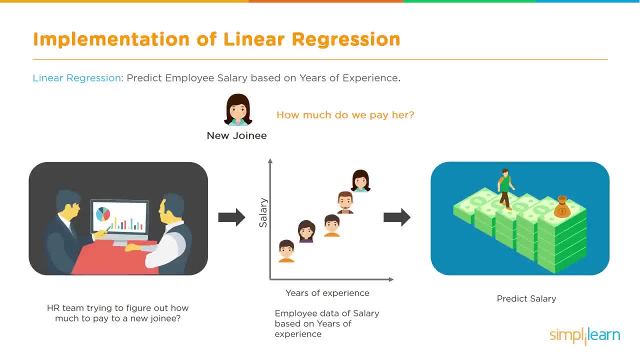 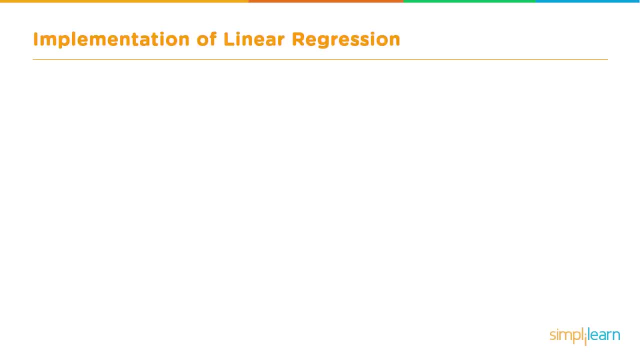 journey. we have the experience and we need to determine what should be the salary. so let's take a look at the demo. so, before we go into the jupyter notebook, let's quickly review the code, what the code is doing. the first section is about importing the libraries. some of you who are 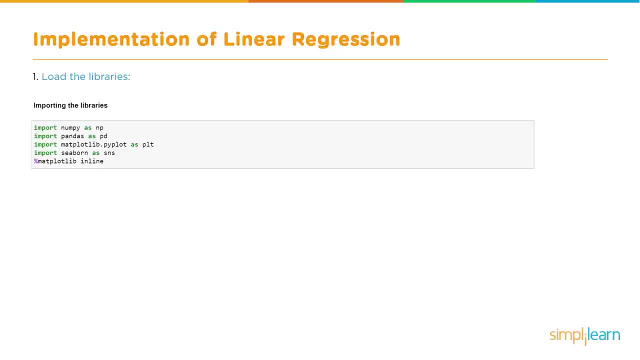 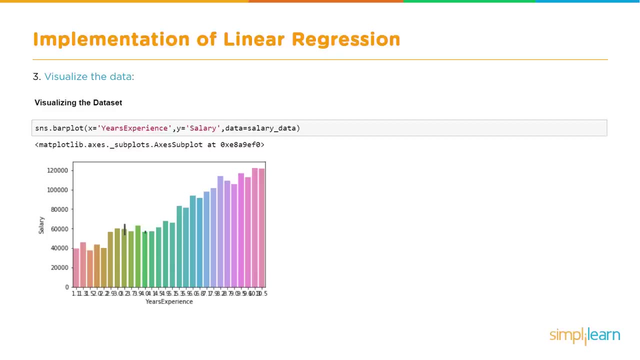 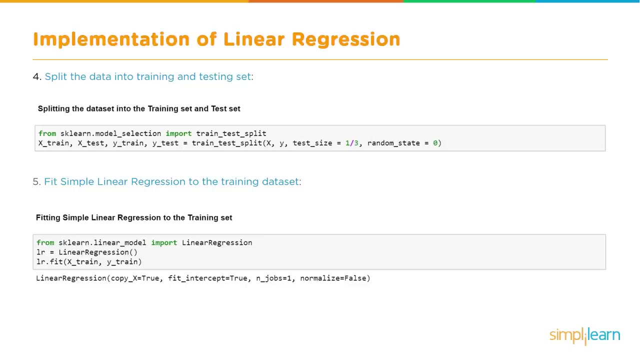 familiar with python will already be knowing this. you don't have to go into details. and then we import the data set and then we visualize the data just to get a quick idea about how the data is looking. and then we split the data into training and test data sets. this is a common procedure in machine learning. 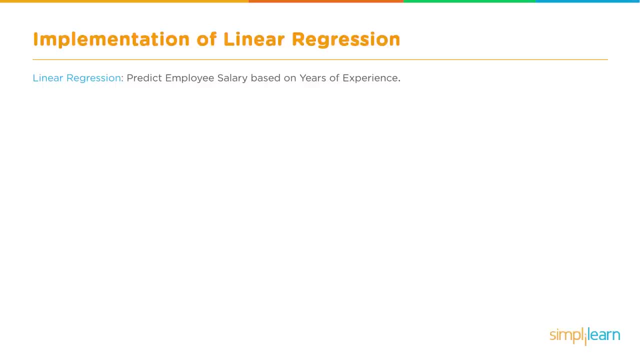 demonstrate this using python, and we will be using a notebook for this. in case you are familiar with Jupiter notebook, I think that would be very helpful and if you need the data set, please put a comment under this video so that we can provide you with the data set before we go there. just let's try to understand what this example is all about. let's 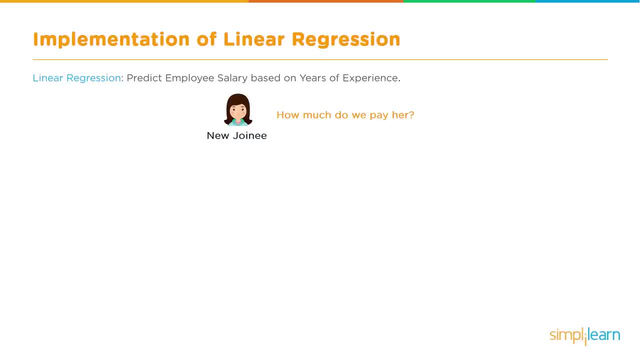 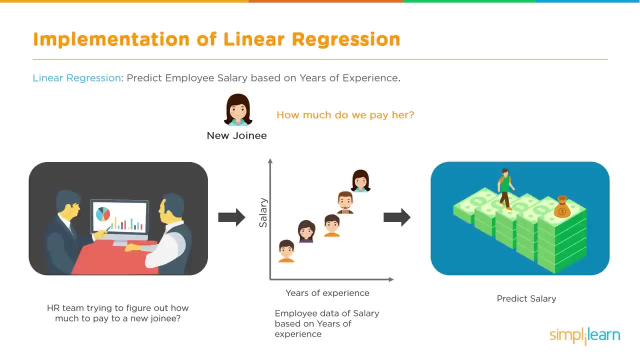 say, there is a new joining joining the company and we want to determine what should be the pay or the salary for this new joining, and for that we already have the labeled data, which is the details of our employees, based on their years of experience and their salaries. and for the new 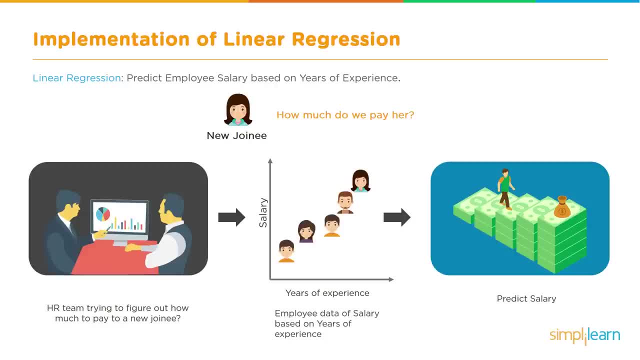 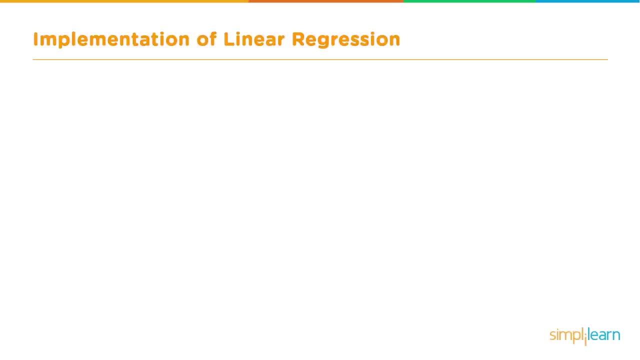 journey. we have the experience and we need to determine what should be the salary. so let's take a look at the demo. so, before we go into the Jupiter notebook, let's quickly review the code, what the code is doing. the first section is about importing the libraries some of you who are familiar with. 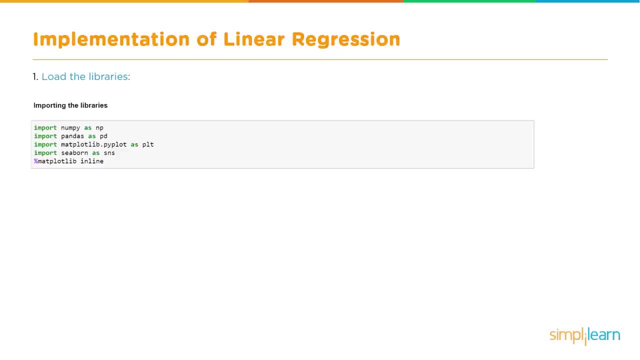 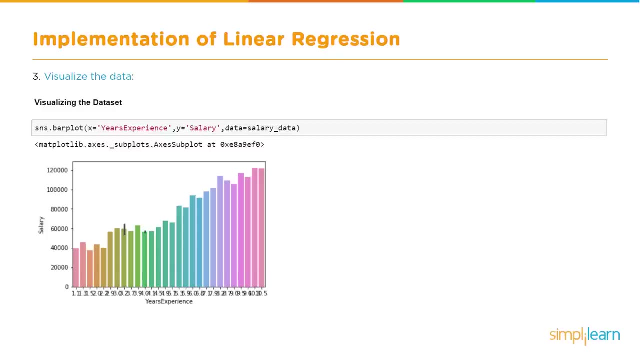 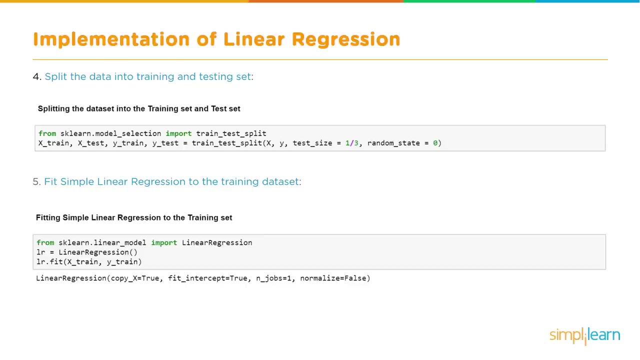 the python will already be knowing this. you don't have to go into details. and then we import the data and we visualize the data just to get a quick idea about how the data is looking. and then we split the data into training and test data sets. this is a common procedure in machine learning process any 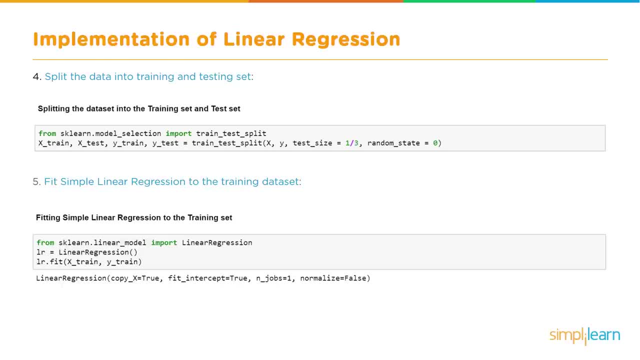 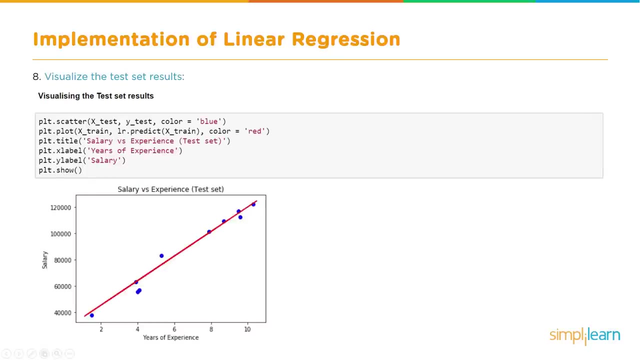 machine learning process and the overall training and test process. we do with two different data sets, so that's what we're doing here, and then we build or train our model- the linear regression model- and then we do the testing and we find out what is the errors and visualize our results and 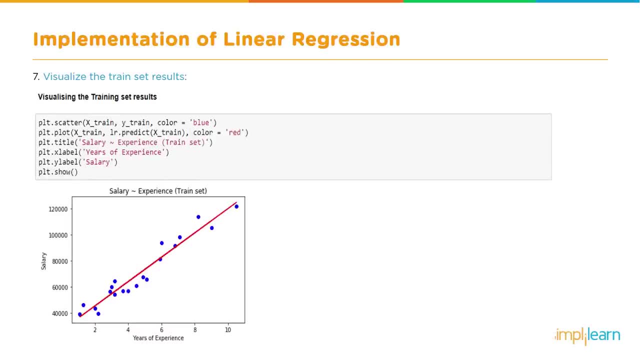 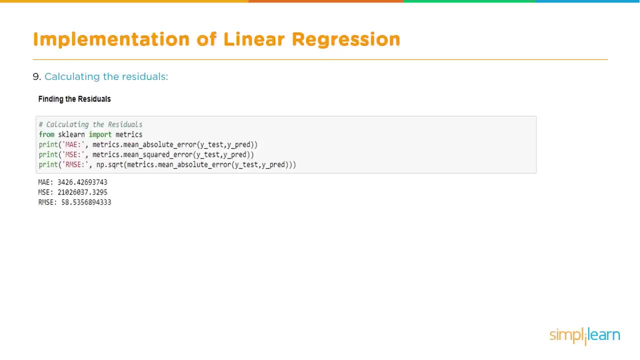 this is the test results. look, and this is how the training result looks. all right, and then we calculate the residuals. residuals are nothing but the errors. there are a couple of ways of measuring the accuracy. the root mean- square error- is the most common one, rmsc, and in this case we got root mean. 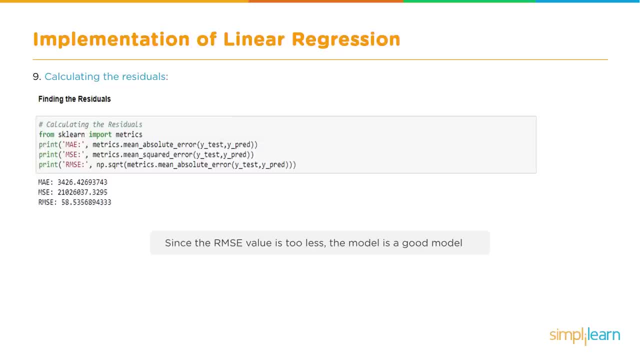 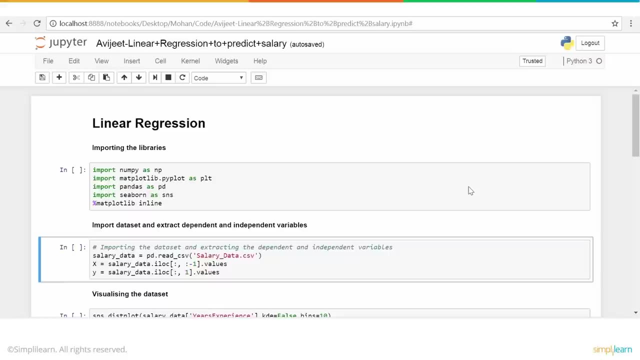 square error of 58, which is pretty good and that's our best fit, all right, so now let's go into the Jupiter notebook and take a look at by running it live. okay, so this is our code for the linear regression demo and this is how the Jupiter notebook looks. and this code in the Jupiter 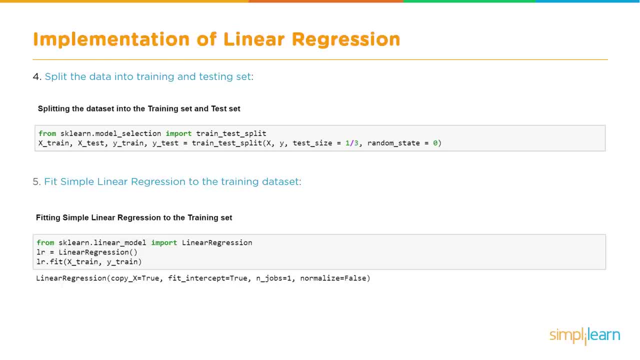 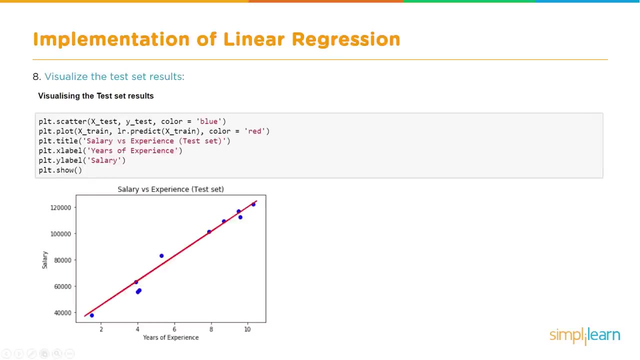 process- any machine learning process- and the overall training and test process. we do with two different data sets, so that's what we're doing here, and then we build or train our model- the linear regression model- and then we do the testing and we find out what is the errors and visualize. 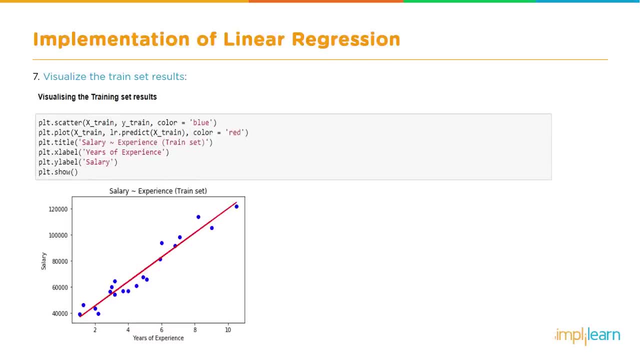 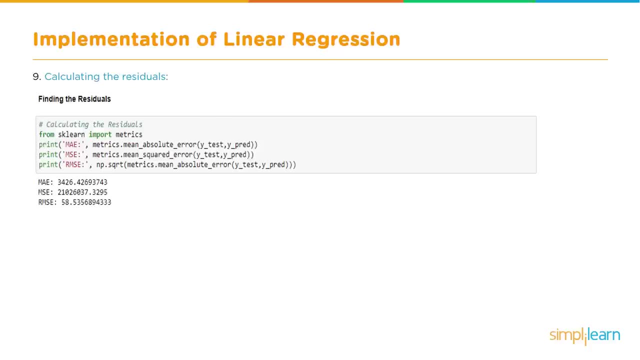 this is how the test results look and this is how the training result looks. all right, and then we calculate the residuals. residuals are nothing but the errors. there are a couple of ways of measuring the accuracy. the root mean square error is the most common one, rmsc, and in this case we got root. 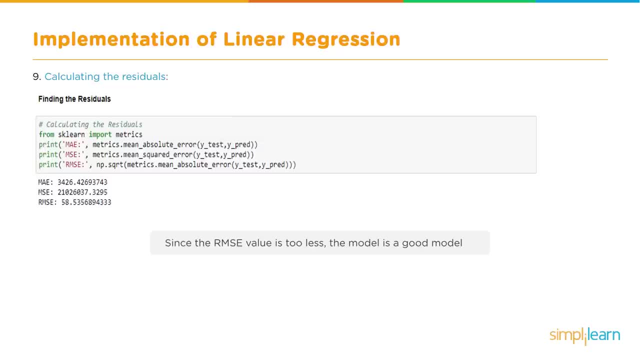 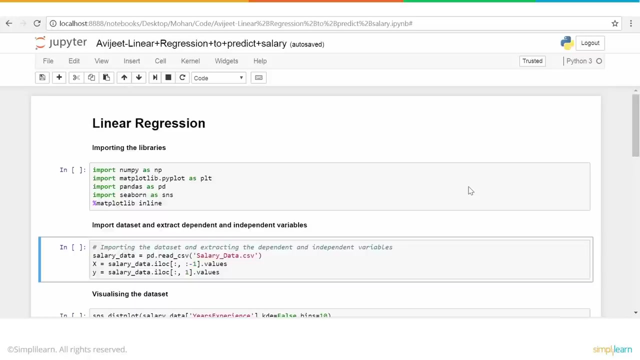 mean square error of 58, which is pretty good and that's our best fit. all right, so now let's go into jupyter notebook and take a look at by running it live. okay, so this is our code for the linear regression demo and this is how the jupyter notebook looks, and 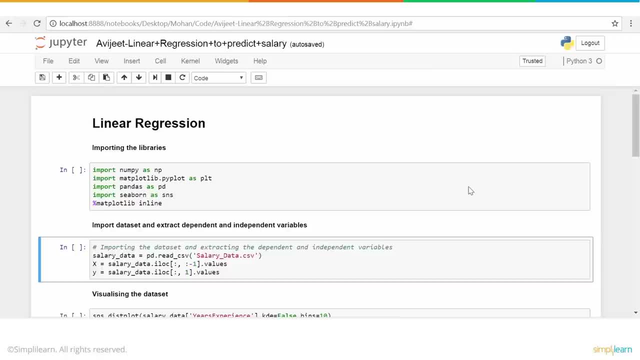 this code in the jupyter notebook looks. i will walk you through the code pretty much line by line and let's see how this works. the linear regression, so the first part, is pretty much a standard template in pretty much all our code. we will see this is importing the required library. so 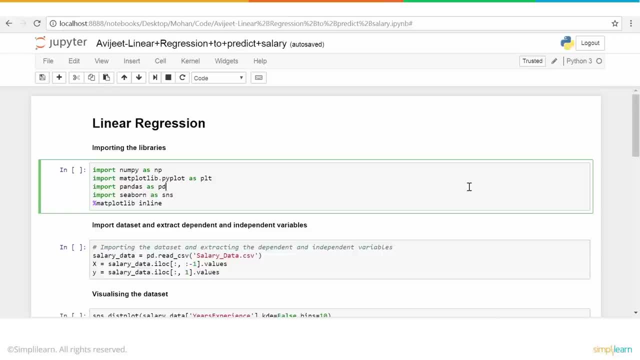 numpy is a library, matplotlib is a library, pandas and so on. so these libraries are required. each of these libraries have a different purpose, so some of them are required for manipulating your data, some for plotting, as the name suggests- matplotlib, and so on and so forth. okay, so let's go ahead and import all these libraries, and then we will. 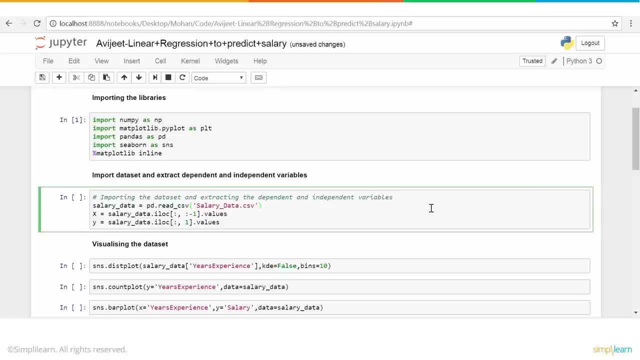 import our data. so in this example, what we are trying to do, the use case in this particular example, is we have some historical value of salary data and now we want to a model so that we can predict the salary for new employee, a person who is joining new, and we will 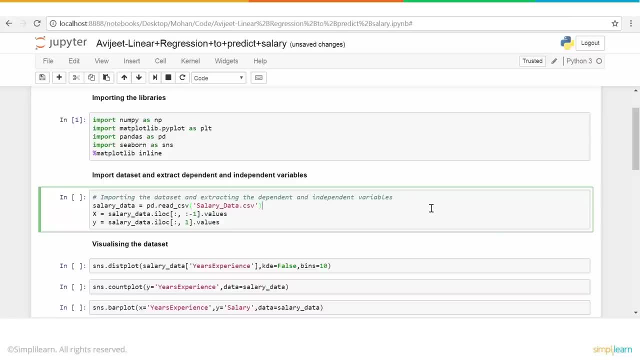 use the same, the characteristics that were available to us or the features that were available to us, and we will try to predict what will be this salary of this new person. okay, so that's the kind of the use case. so let's go ahead and load the data and let me introduce a cell and see how the data looks. so 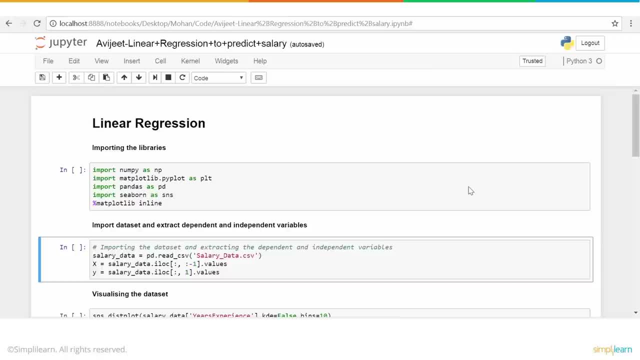 notebook looks. I will walk you through the code pretty much line by line and let's see how this works. the linear regression. so the first part is pretty much a standard template in pretty much all our code we will see. this is importing the required library. so numpy is a library, matplotlib is a library, pandas and so on. so these libraries are required. 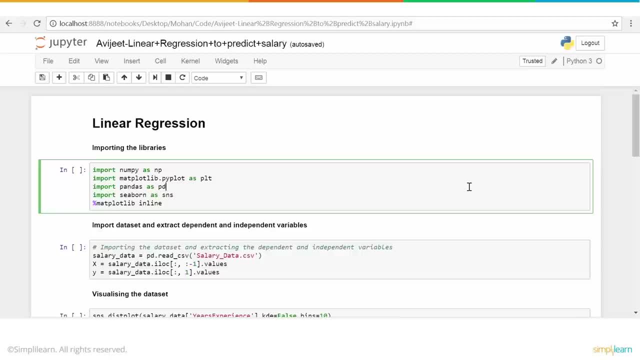 each of these libraries have a different purpose, so some of them are required for manipulating your data, some for plotting, as the name suggests- matplotlib, and so on and so forth. okay, so let's go ahead and import all these libraries, and then we will import our data. so, in this example, what? 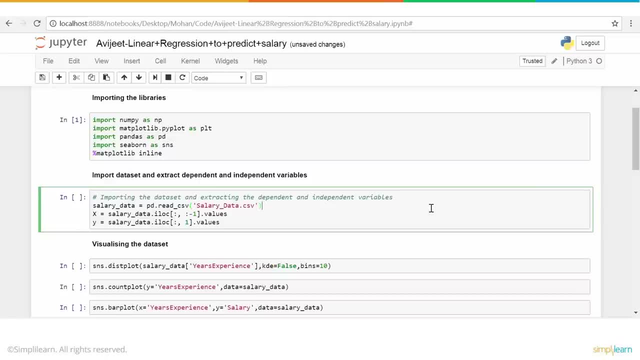 we are trying to do. the use case in this particular example is we have some historical value of salary data and now we want to build a model so that we can predict the salary for new employee, a person who is joining new, and we will use the same, the characteristics that were. 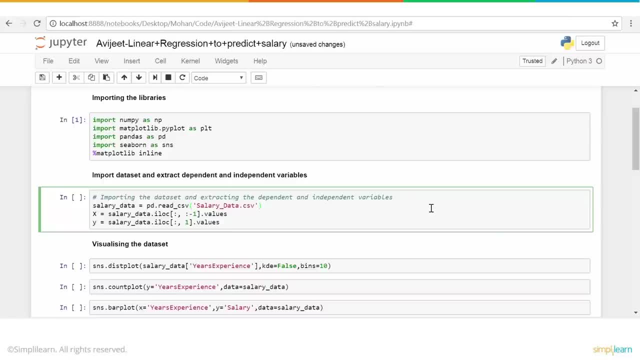 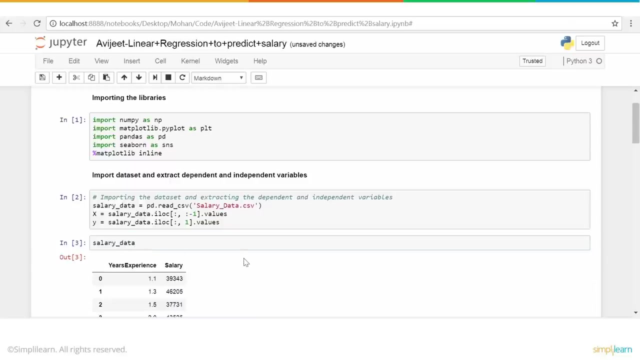 available to us, or the features that were available to us, and we will try to predict what will be this salary of this new person. okay, so that's the kind of the use case. so let's go ahead and load the data and see how the data looks. so, salary underscore data. so we have basically two features, right? so 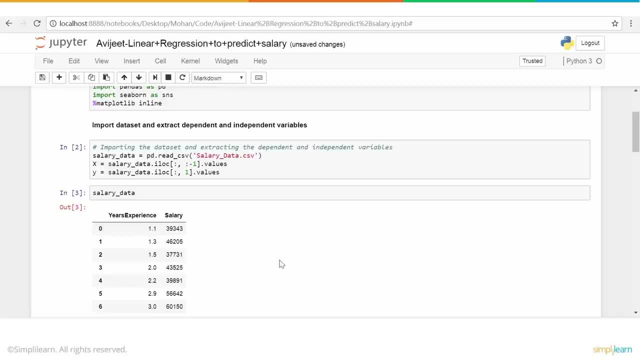 it's pretty much like a simple linear regression we are trying to do so. we have years of experience and salary and in this case, what we are trying to do is this is our predictor. so years of experience is our predictor and we are trying to predict what the salary would be. so, once again, so X is. 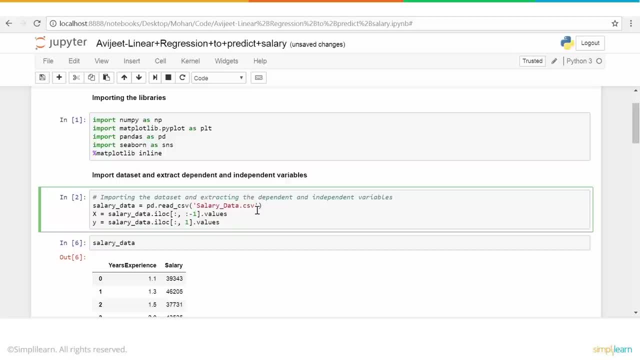 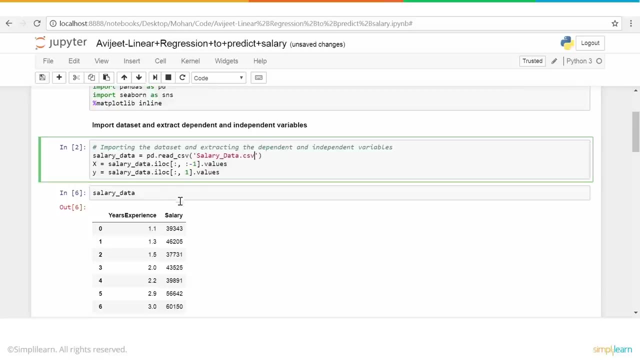 what is known as the predictor, and Y is the target, so number of years of experience we are taking as input and we will try to find what will be the salary of this person based on that. okay, so that's what we are going to do. so I have shown what is how, the overall how, the data, data that has been. 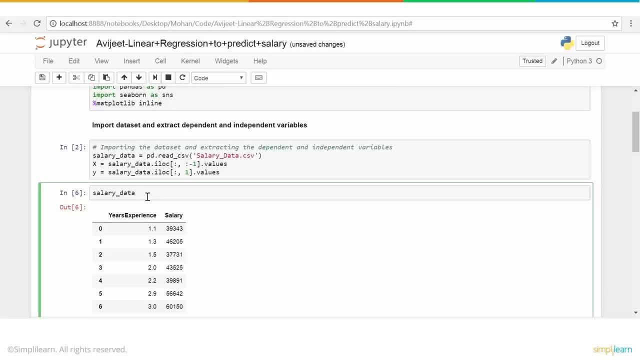 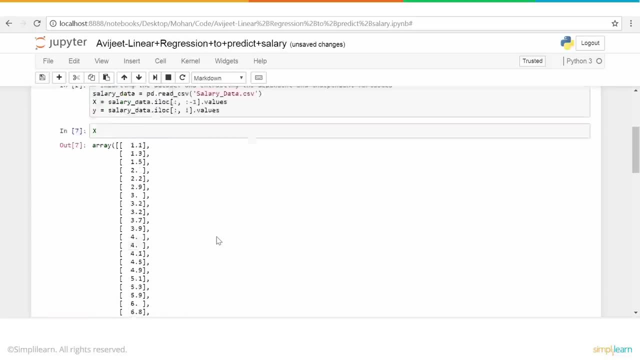 imported looks. now let's take a quick look at these extracted values or extracted columns as well. so let me put in X here and see how it looks. so there's basically one column, and same way if we put Y here, we will see what exactly. I'm sorry this has to be in small, lower. 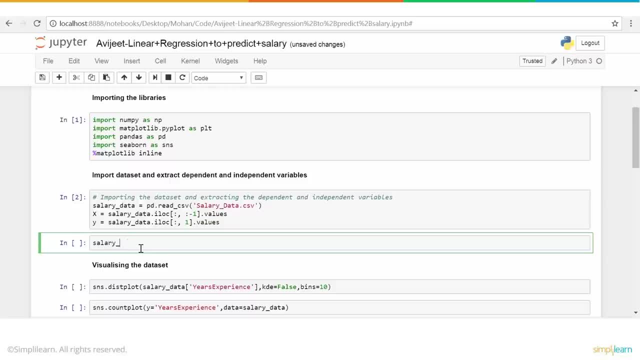 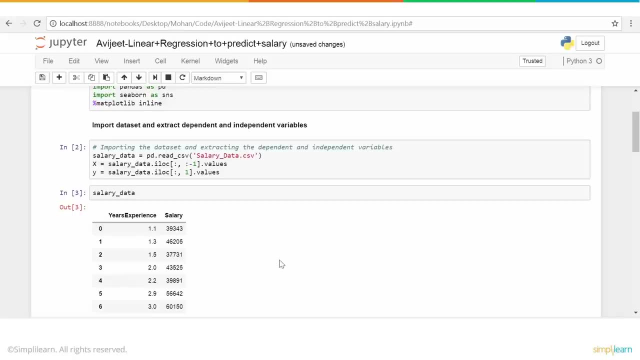 salary, underscore date, and so we have basically two features, right? so it's pretty much like a simple linear regression. we are trying to do so. we have years of experience and salary, and in this case, what we are trying to do is this is our predictor. so years of experience is our predictor and, um, we are trying. 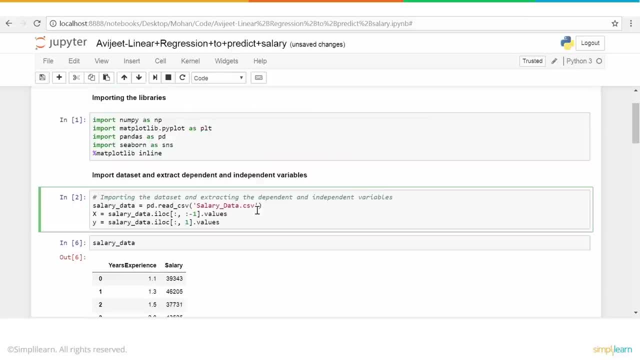 to predict what the salary would. so once again, so x is what is known as the predictor and y is the target. so number of years of experience we are trying to target and so that is пожалуйста. so this is of years of experience we are taking as input And we will try to find what will be the salary. 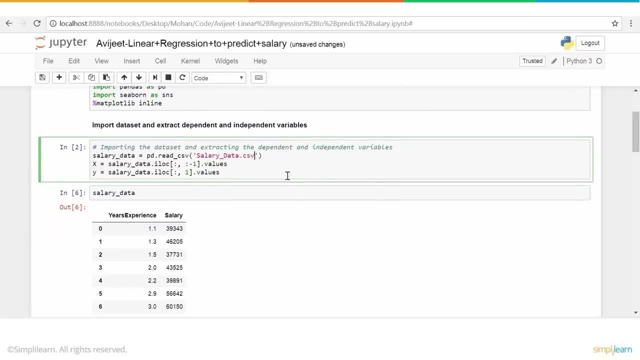 of this person based on that. Okay, so that's what we're going to do. So I have shown what is how the overall, how the data data that has been imported- looks. Now let's take a quick look at these extracted values or extracted columns as well. So let me put in x here and see how it. 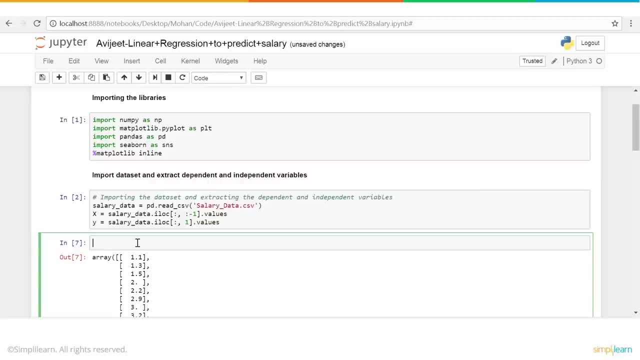 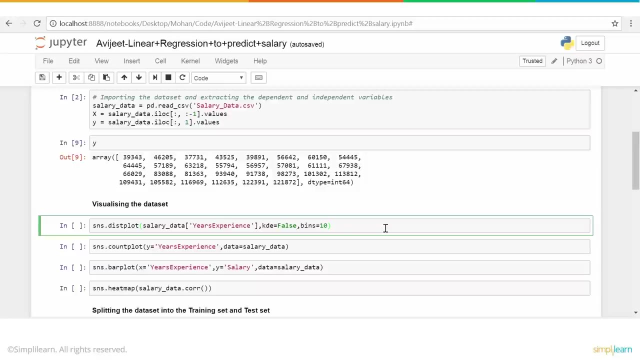 looks. So there's basically one column And same way. if we put y here, we will see what exactly. I'm sorry this has to be in small lowercase. So this is the salary information. Okay, so this is our data is, and then we can do a little bit of plotting of the data to play around a little bit. 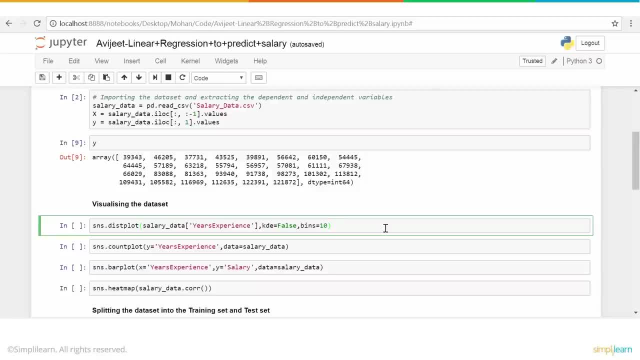 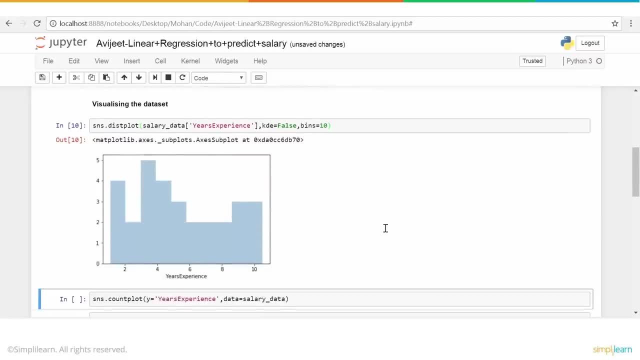 because we imported the data. Typically we want to do some exploratory analysis: how they compare with each other and so on and so forth, how they are correlated. So let's draw a quick plot, a bar plot, and see how the years of experience are being. 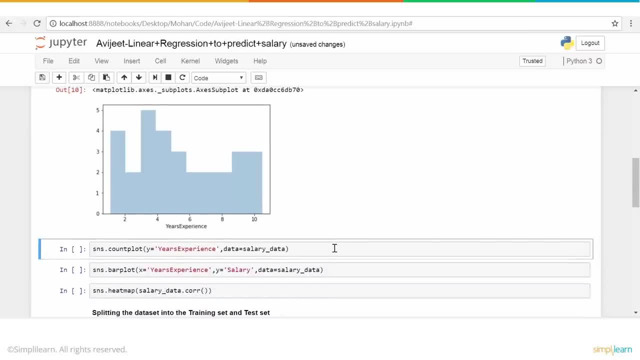 set. So let's draw a quick plot, a bar plot, and see how the years of experience are being set. So let's draw a quick plot, a bar plot, and see how the years of experience are being set. seen here, right? So this is how the bar plot looks. Similarly, let's do one more, which is 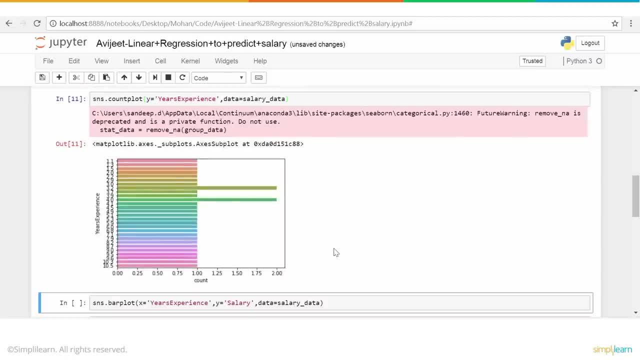 basically, more like this is horizontal bar plot. Okay, so how many people and with what experience, and so on and so forth. So what this shows is the count: how many records are there with a given experience, and things like that. Okay, so this is another way of visualizing the data And 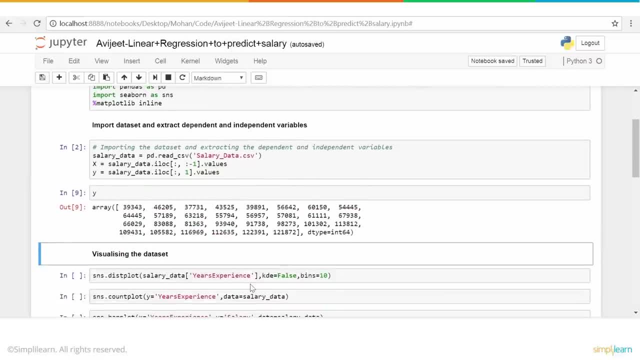 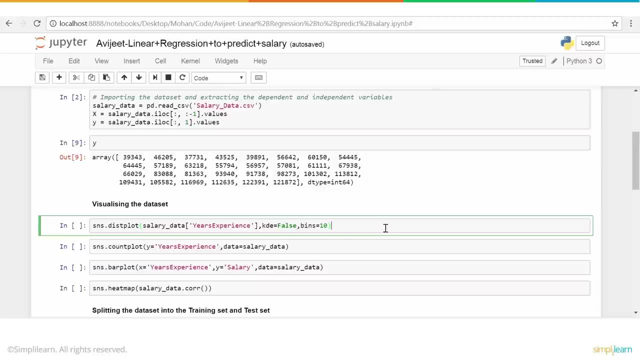 case. so this is the salary information. okay, so this is how our data is, and then we can do a little bit of plotting of the data, to play around a little bit, because we imported the data. typically we want to do some exploratory analysis: how they compare with each other, and so on and so forth. 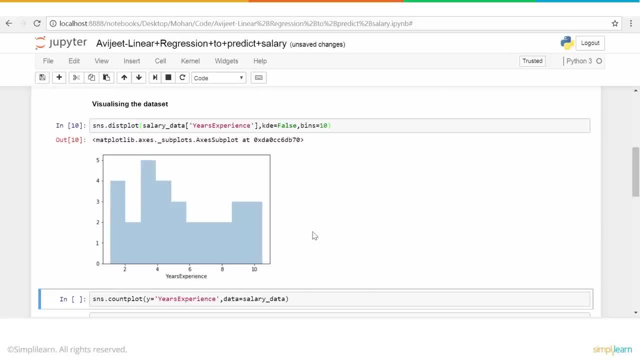 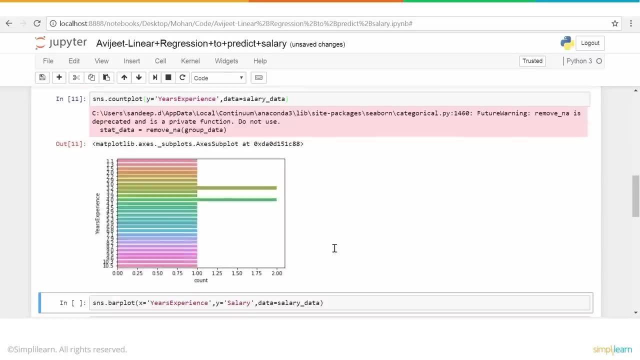 and see how the years of experience are being seen here. right? so this is how the bar plot looks. similarly, let's do one more, which is basically more like a. this is horizontal bar plot, okay, so how many people and with what experience, and so on and so forth. so what this shows is the 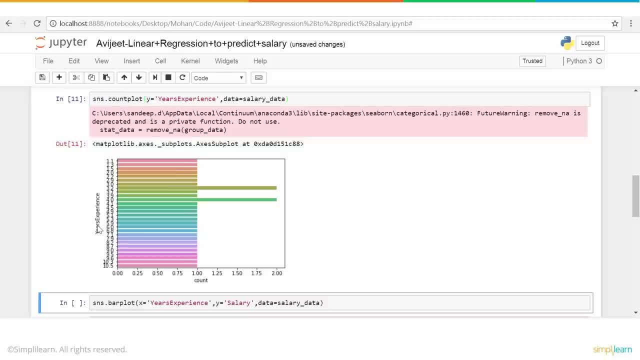 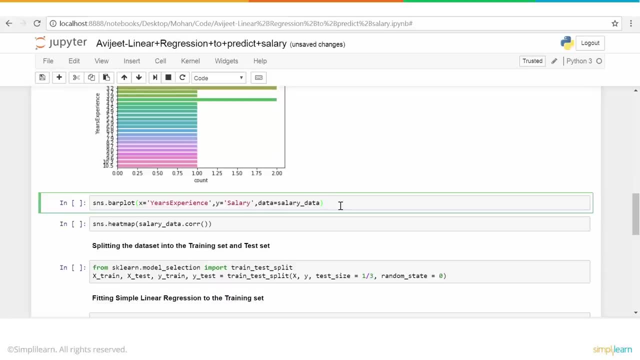 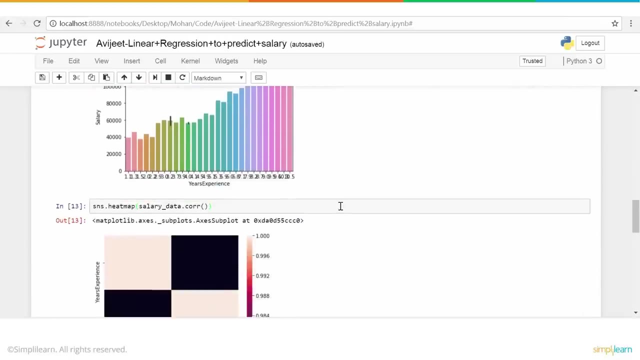 count how many records are there with a given experience and things like that. okay, so this is kind of visualizing the data and this is a third view, and this is one more view, and then we can do a quick heat map. so there are, there's only one, or actually there are only two variables. so there is. 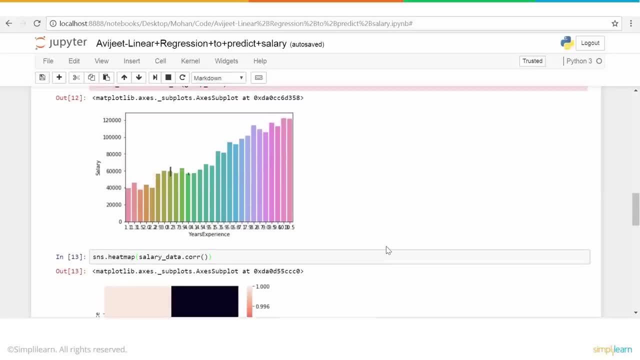 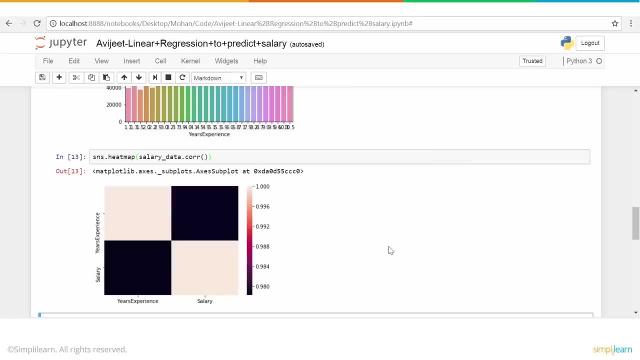 an. there's not a lot of plotting that we can do or not a lot of visualization that we can do, since there are only two variables, but nevertheless, whatever is possible, we can do a quick to get a quick idea about how the data is looking and how the variables are related to each other. is there a correlation and things like that all. 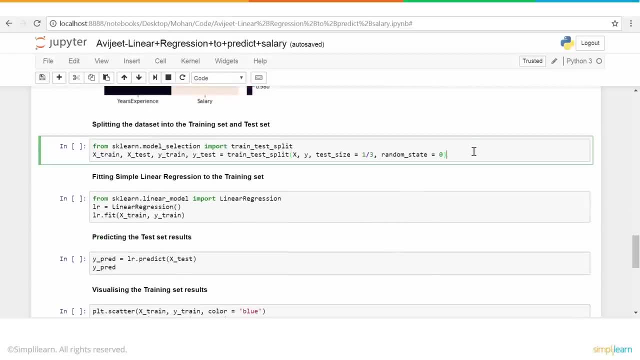 right. so once we are done with that, this is the most important part of our demo here, which is basically this is the beginning of our training process. so the first thing before we start the model building and model training process is to split the data into training and test data sets. 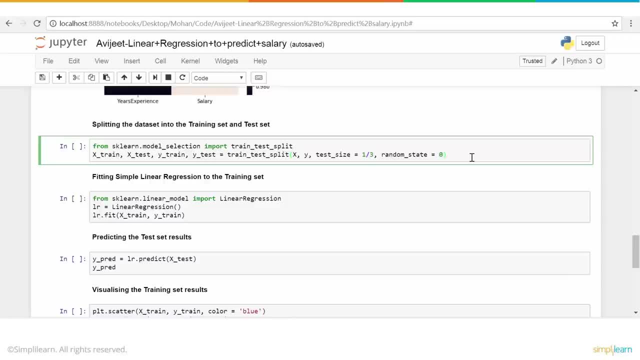 okay now, whenever we do any machine learning exercise, especially supervised learning, we never use the entire label data for training purpose, the reason being then we will not be able to correctly evaluate how well the training has happened. okay, so what we do is we split the data, we take a portion of the data, we call that as the training data set and we set aside some portion of. 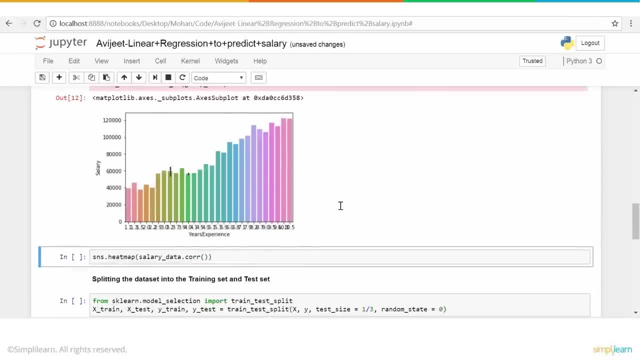 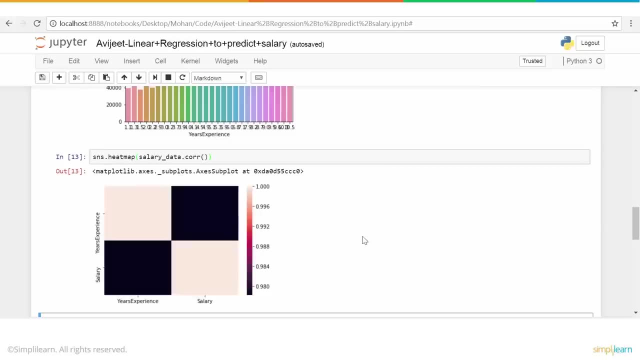 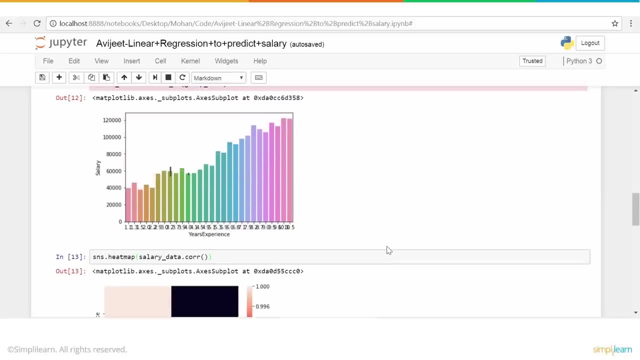 this is a third view, And this is one more view, And then we can do a quick heat map. So there are there's only one, or actually there are only two variables. So there isn't there's not a lot of plotting that we can do or not a lot of visualization that we can do, since there are only 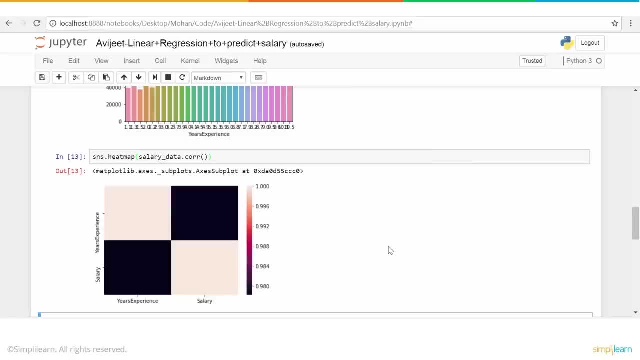 two variables But nevertheless, whatever is possible, we can do a quick to get a quick idea about how the data is looking and how the variables are related to each other. Is there a course correlation and things like that? All right, So once we are done with that, this is the most. 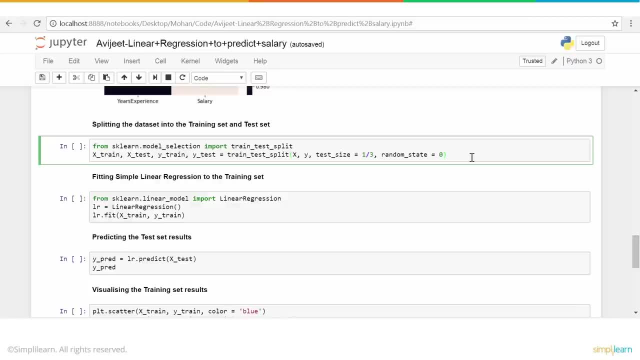 important part of our demo here, which is basically: this is the beginning of our training process. So the first thing before we start the model building and model training process is to split the data into training and test data sets. Okay, Now, whenever we do any machine learning, 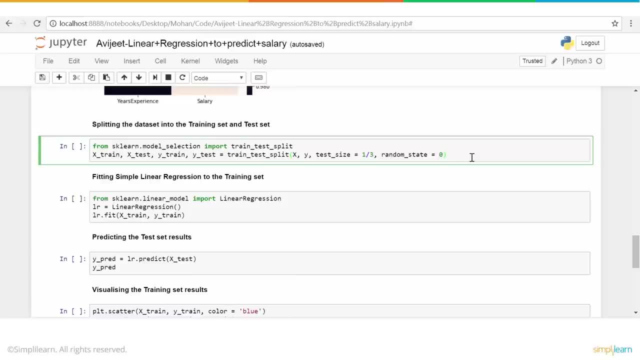 exercise, especially supervised learning. we never use the entire label data for training purpose, The reason being then we will not be able to correctly evaluate how well the training has happened. Okay, So what we do is we split the data, we take a portion of the data, we call that. 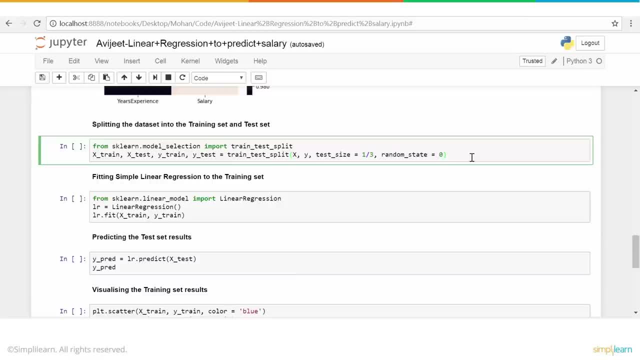 as the training data set and we set aside some portion of the data. we call that as a test data set. We use the training data set to actually perform the training, to train our model, And once that is done, we use the test data set to check how well the model has been trained. 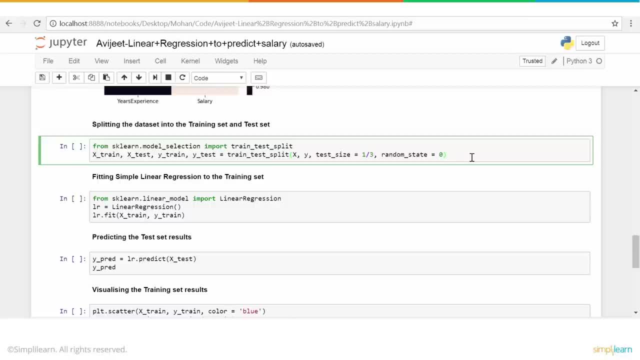 how accurately it is able to predict. Okay, Now the reason is in for our with our test data set also, since that is also labeled, we allow the model to predict the values and we compare it with the labeled information to see whether it has predicted correctly or not. Okay, So that is. 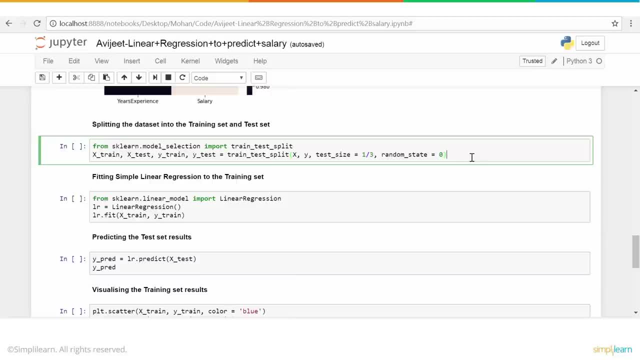 the reason in all machine learning activities, Whenever we perform machine learning, we especially training of a model. we split this data into training and test data set, And that's what we are going to do here Now we there is no need to. 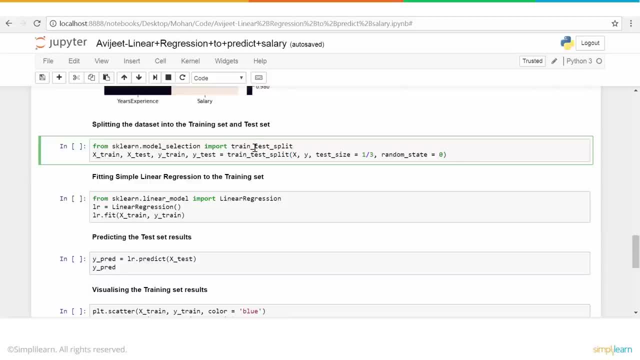 write any separate code for that. There is a readily available function for that train: underscore test, underscore split. So that's what we are going to use here. It takes the data set- x and y is the data set- And in addition, it takes a parameter which tells how the data has to be split. So for 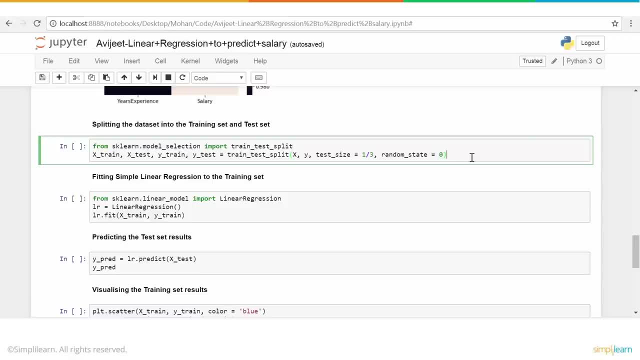 the data. we call that as a test data set. we use the training data set to actually perform the training, to train our model, and once that is done, we use the test data set to check how well the model has been trained, how accurately it is able to predict. okay, now the reason is in for our with our test data set also, since that is also labeled. 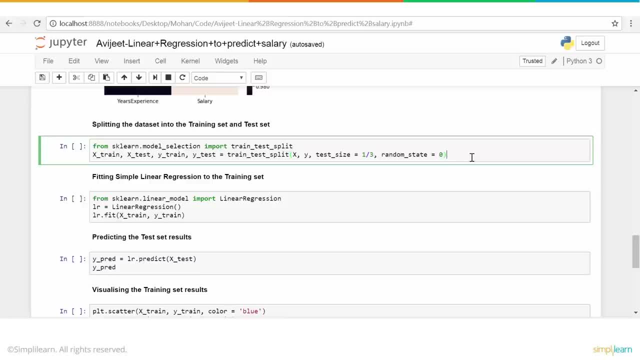 we allow the model to predict the values and we compare it with the labeled information to see whether it has predicted correctly or not. okay, so that is the reason in all machine learning activities, whenever we perform machine learning, we especially think of a model. we split this data into training and test data set, and that's what we are going to. 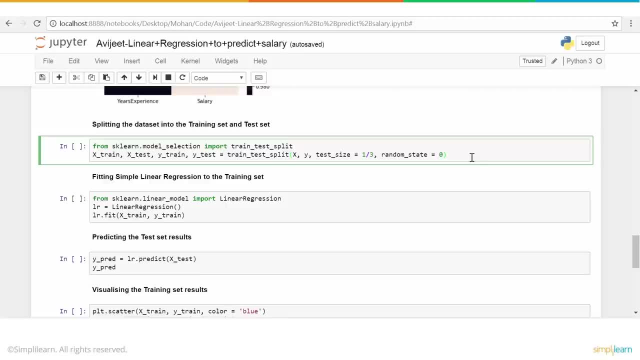 do here now we. there is no need to write any separate code for that. there is a readily available function for that- train underscore test, underscore split. so that's what we are going to use here. it takes the data set, the x and y is the data set and in addition, it takes a parameter. 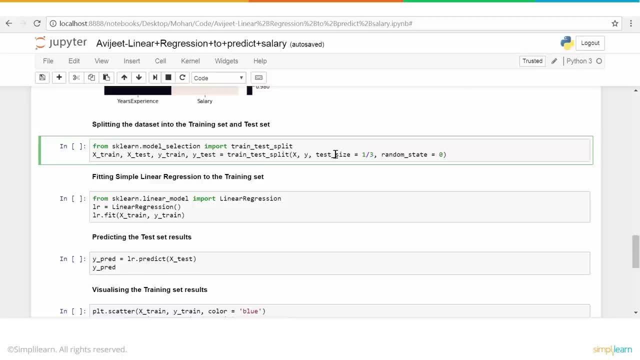 which tells how the data has to be split. so, for example, here it says: test size is equal to 1 by 3. that means it is 33 percent, right? 33.33. so one third of their data you want to set aside for test. now there are no hard and fast rules as to what should be this split of test and training data. 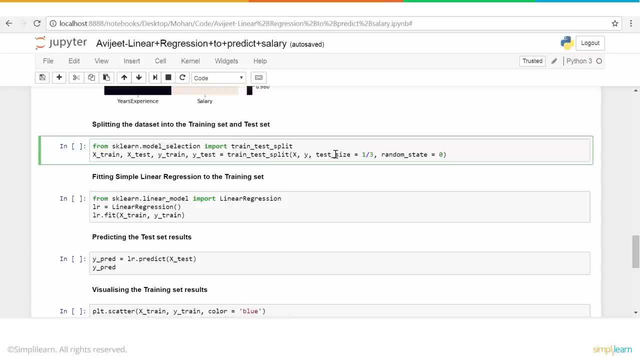 set. it is a matter of individual preferences. some people would like to have 50- 50, some people would prefer 80, 20, and so on and so forth. so it is completely up to the individuals to to decide on that. so, in this particular case, what we are doing is we are setting aside. 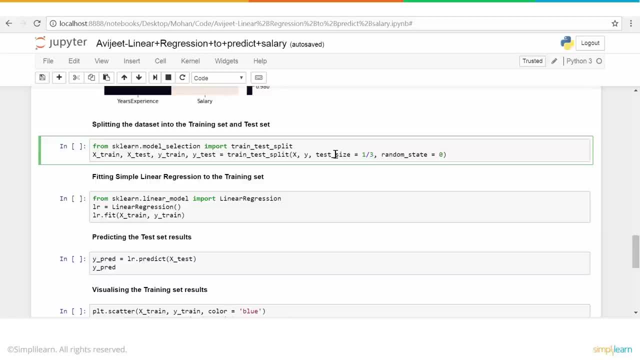 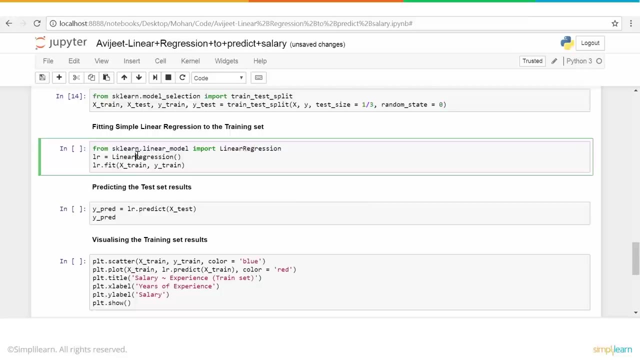 one third of the data set for testing purpose and two-thirds of the data set for training purpose. okay, so that's exactly what we are doing here. now the next step is to create an instance of linear regression. so linear regression model is readily available. so we create an instance of the linear 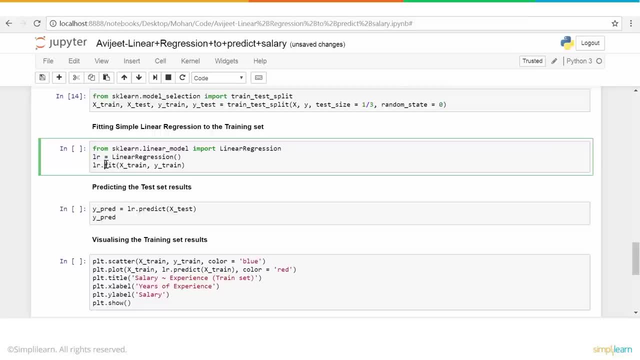 regression model and give it a name like LR, and then we call the fit method of the linear regression model. now this fit method is common across all the algorithms, so any algorithm you use if you want to start the training process, you call the fit method. okay, and 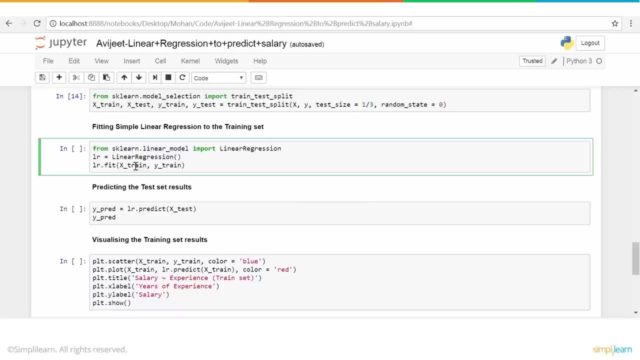 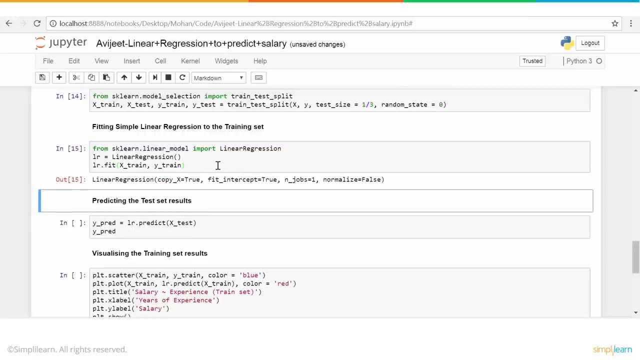 then we pass the training data set. now training data set, we send the predictor, as I was saying, or the independent variable and also the dependent variable. we pass both of them, okay, and the system will basically learn based on this. so now the training has happened, training is completed and 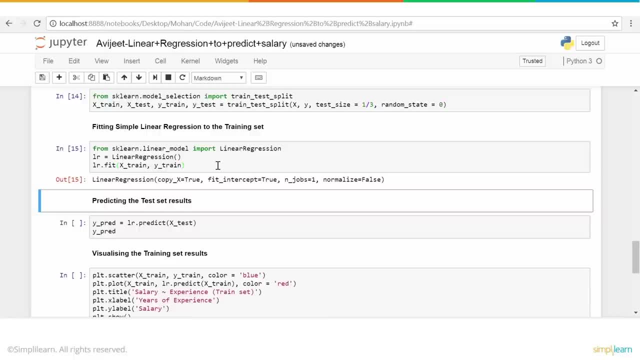 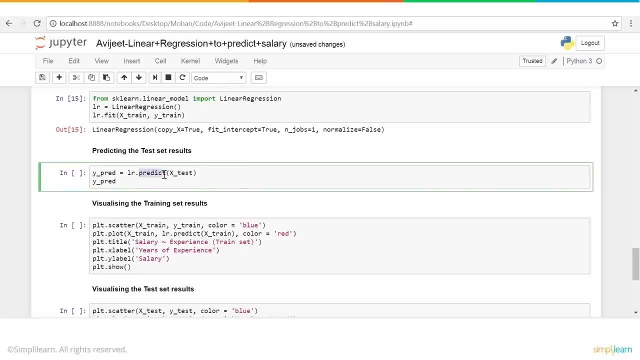 now we need to see whether it is predicting correctly or not. we need to test it right. so for testing, we have another method called predict. again, this is common across all algorithms. any algorithm you use, you will have this predict method for testing your, your model, okay- or for actually predicting the values, whether 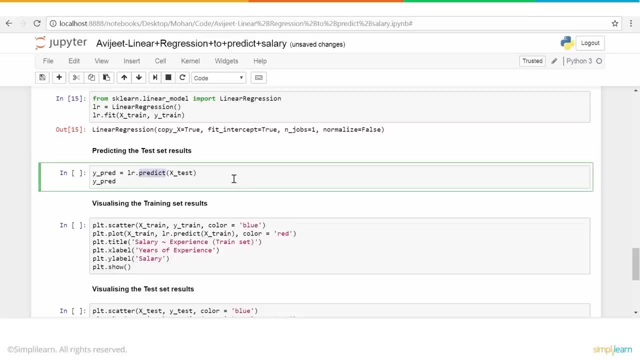 during testing or when you actually deploy the model. okay, now here, predict will take only one parameter, which is the dependent variables, right? the reason being the dependent variable is what it will predict, right? so y underscore test, we don't have to pass, whereas here, y underscore train, we passed for training. 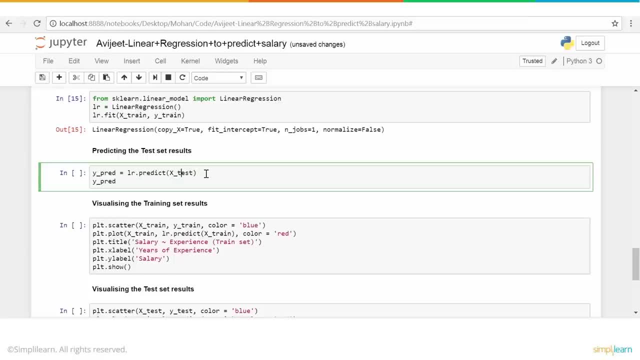 purpose. but y underscore test we do not pass because that is what the model will predict, so we don't have to pass that. and then the model will predict, and that is what we call it as y underscore pred. but we will use y underscore test to compare with what the model has predicted, and thereby we 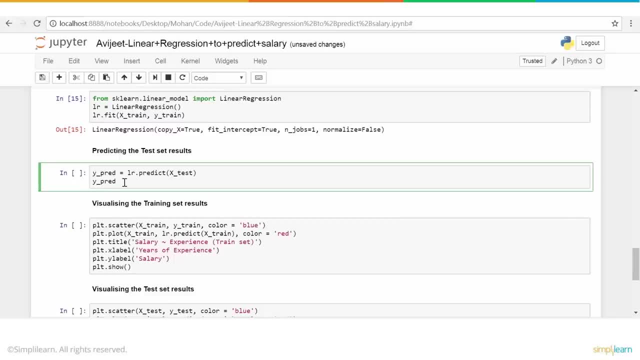 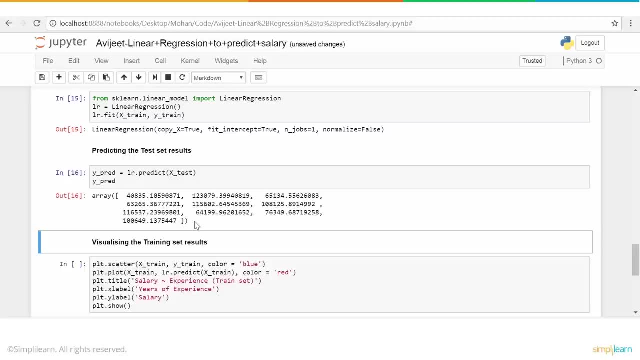 determine how accurate the model is. okay, so let me go ahead and run this code. so it has done with the testing or with the prediction of the values. so these are the predicted values and now we can visualize. we can generate some plots to visualize this information. so let's plot this training set. 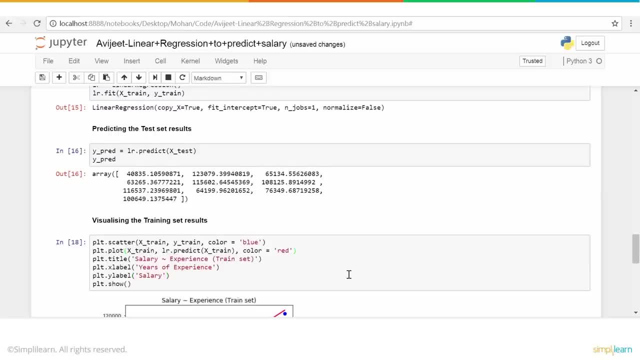 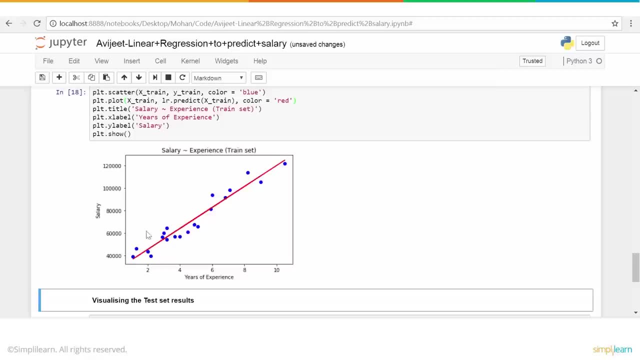 results, information and see how it looks. so what? what we are doing here is basically, we have the training data set plotted, the salary versus the years of experience, right, this is the training data, the the dots, basically, and then this line is what our model has, so this is the best fit. so linear regression: what is a linear regression process? 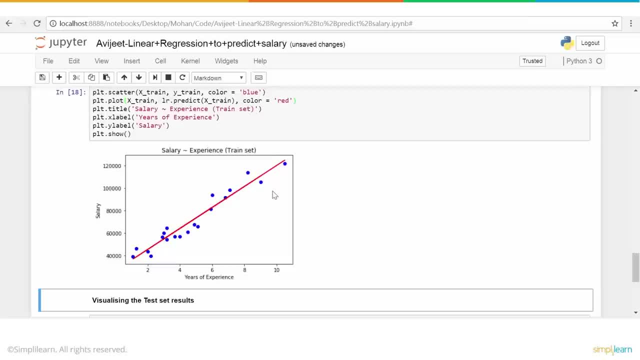 we find a equation of a line which is the best fit. so our model- this is the equation or this is the line that our model has kind of come up with saying that this is the best fit model. okay, so as you can see, intuitively it feels okay because it is passing through. 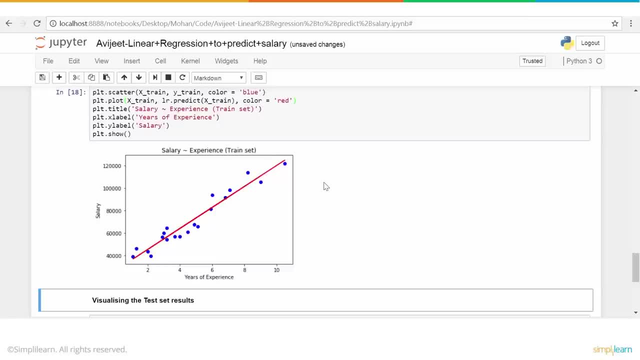 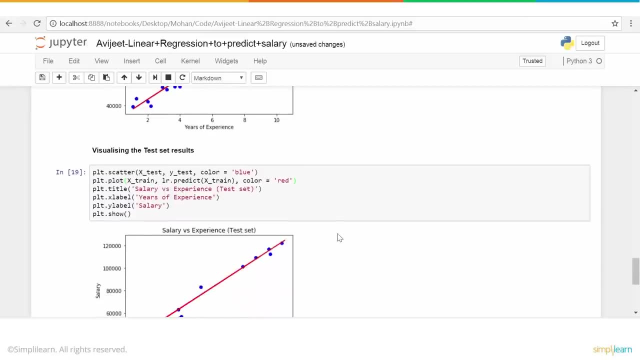 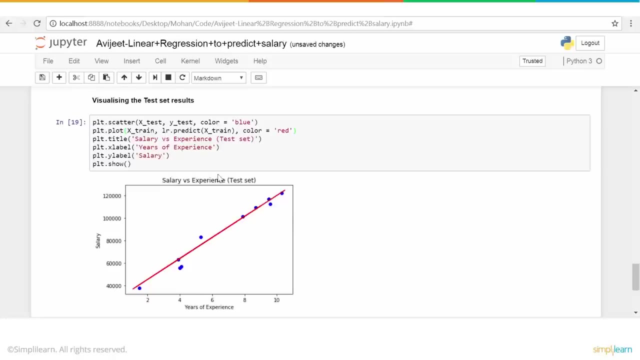 pretty much the middle of our data set. okay, so this is for the training part. now we do the same for our test as well and see how it is doing, or how it looks here also, it looks pretty good because the line passes pretty much in the middle of the overall data set. that's what we are trying to do. 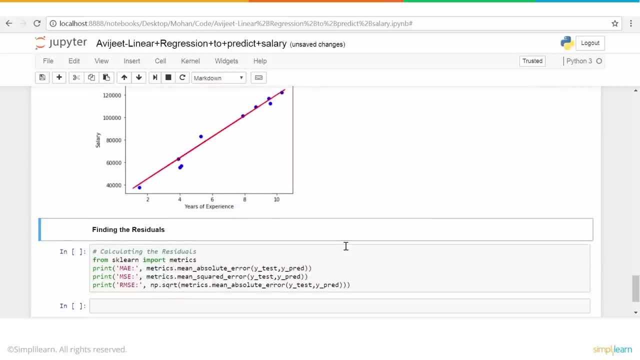 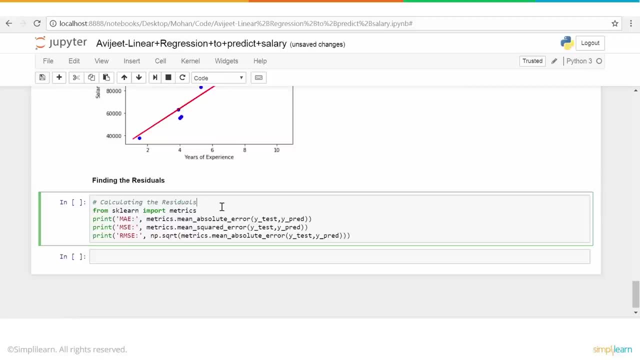 here. all right, and then how do we measure the accuracy? so these residuals are nothing but the errors. the term residuals is nothing but the errors we have seen in the past. we have seen in the past in the slides as well. so we calculate the accuracy of our model by calculating the various residuals. 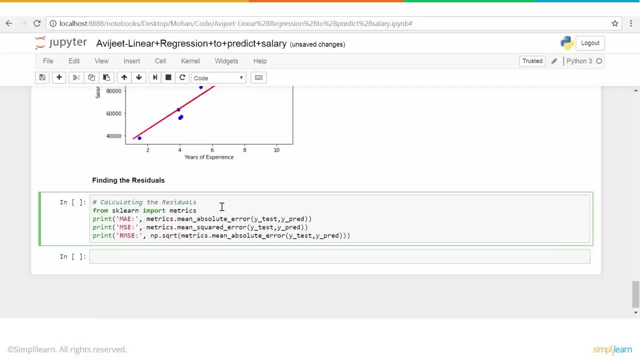 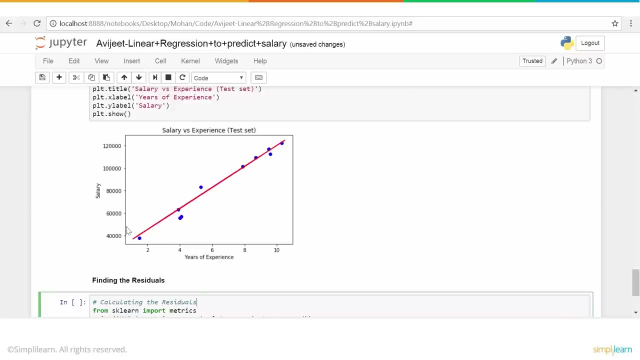 we have like mean square error, then we have the mean absolute error and then we have the root mean square error. they are pretty much they're very closely related. this is nothing but the error and the actual value, right? so, for example, let me explain with this this particular line. 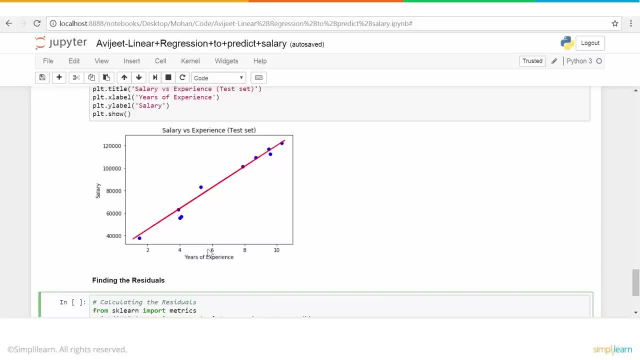 so what our model says is: if the value of the years of experience right. so let me take at this point: maybe if the value of the years of experience is four, then the salary will be, according to our data, that salary probably should be. what is this? maybe around uh 58 000, right, and there are, of course, uh three points. 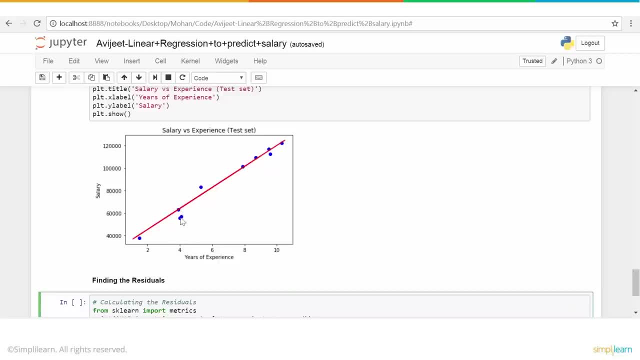 three data points pretty much around this. four years experience, uh, one may be around 58, or in fact two of them are around 58 and there is one more which is probably 60.. okay, now, these are the three data points, whereas our model predicts that if the years of experience is four, then the salary should be sixty thousand. let's say okay. 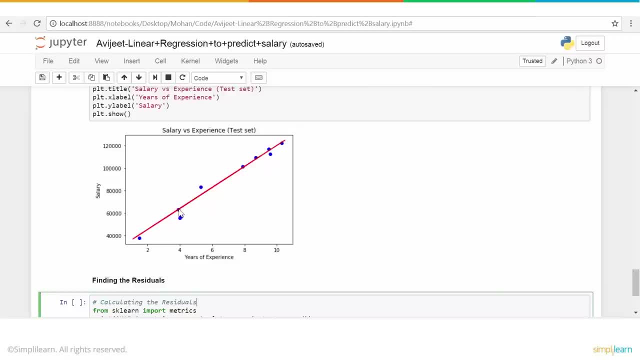 let's assume this goes to sixty thousand, which means that one of the data points is very accurately predicted by our model, but there are two of them which are off. so there is an error for these two values. and what is that error? the error is nothing but the distance of this point from. 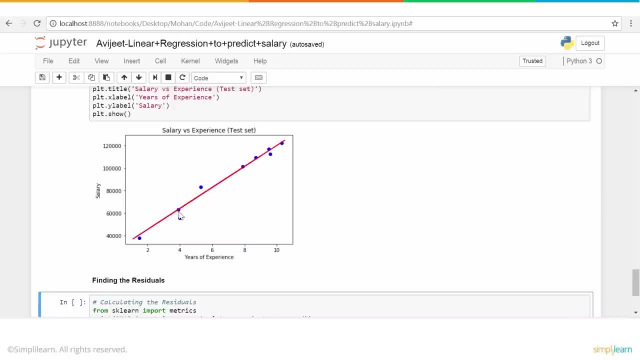 this line right. the distance of this point, of each of these data points, from the from the line is the error. okay, so that's basically for each of the values. it will correct. so it will calculate rather, and, and, instead of taking the absolute value, we kind of take a square of that. so, because the value 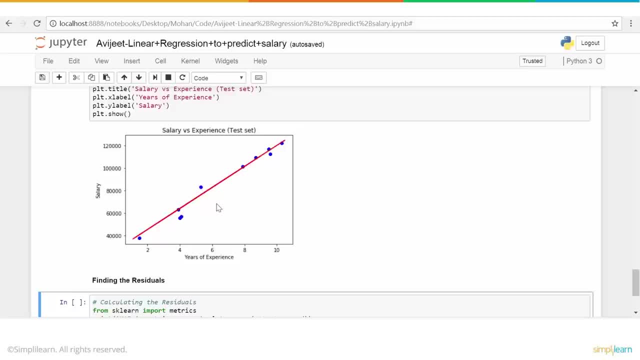 can be positive or negative. so in order to avoid a cancellation, so there are some positive values, there are some negative values and they get cancelled out. so what we do is we take a square of that. so that is basically what is the root mean square or the 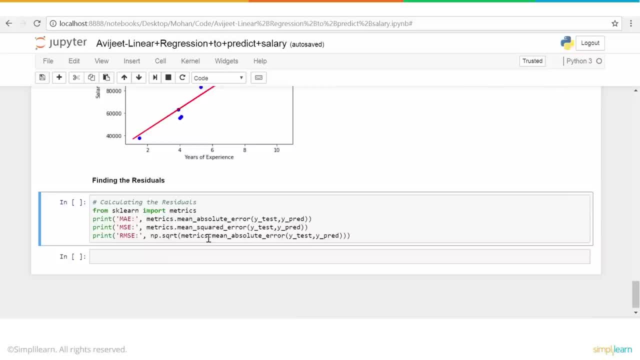 mean square error and then if we take a square root of that, it becomes root mean square error, right? so this was explained, probably in the slides as well. so that is what we will calculate here, and uh, we, we print it, okay. and uh, these values- the root mean square error, the me mean squared error. 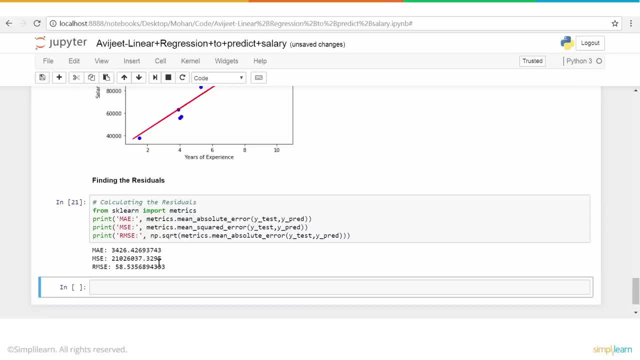 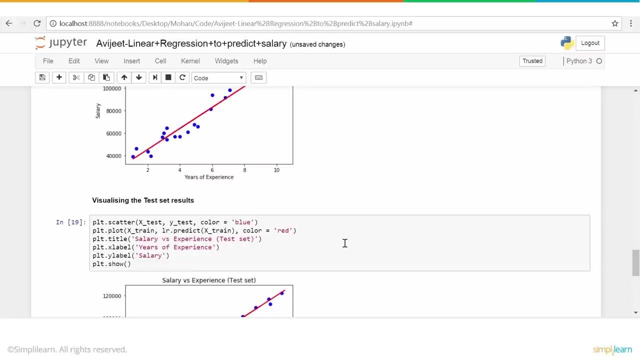 and the mean absolute error. the lower these values are, the better, so the accuracy is higher if these values are lower, so in a way it is inversely proportional. okay, so that's the way we measure the accuracy of our linear regression model. all right, so that brings us to the end of this demo and we will continue with the other demos. all. 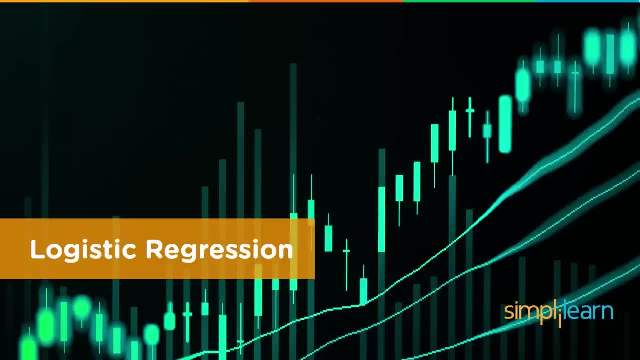 right now that we have seen linear regression, let's take a look at our next machine learning, which is logistic regression. now, what's interesting about this algorithm is that, while it says regression, the name has regression in it. but keep in mind, this is not used for regression, but this: 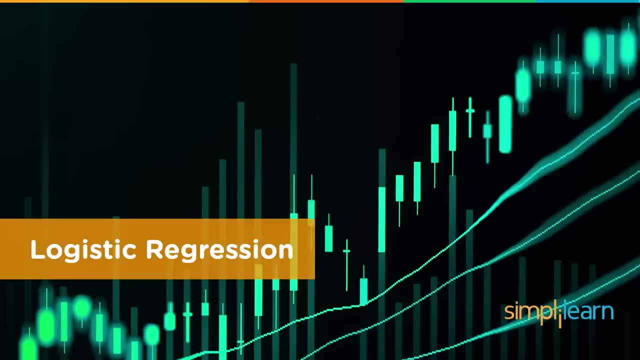 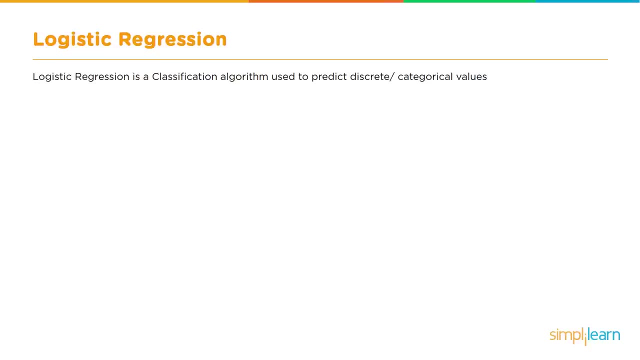 algorithm is used for classification. now, many people get confused by this name, so you need to be aware of it. linear regression is used to solve regression problems, where we are trying to predict a value, whereas logistic regression is used to solve a classification problem, so we are trying to find, for example, whether a person 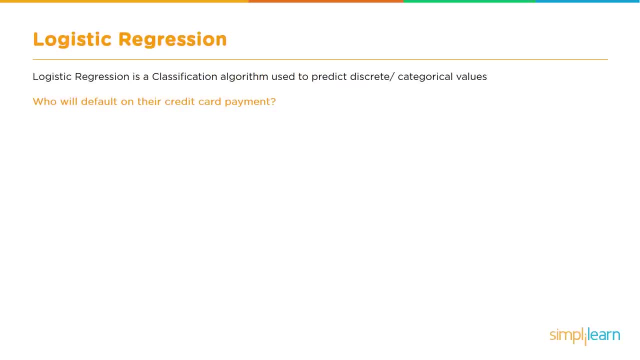 will repay the loan or not, or whether we want to find whether this image is of a cat or a dog. so this is a classification problem, okay, so just that you should be aware of the name. so in this slide we are talking about whether a person, credit card user or credit card holder- will default on the 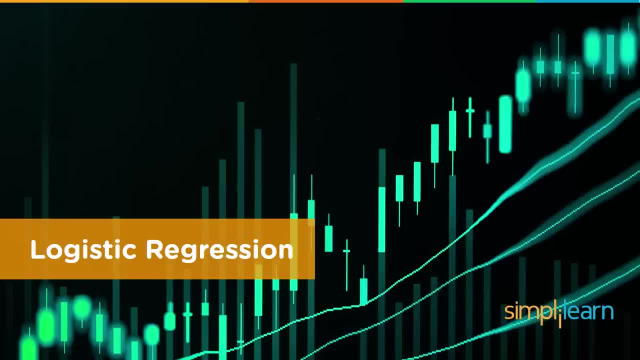 But keep in mind this is not used for regression, but this algorithm is used for classification. Now, many people get confused by this name, so you need to be aware of it. Linear regression is used to solve regression problems where we are trying to predict a. 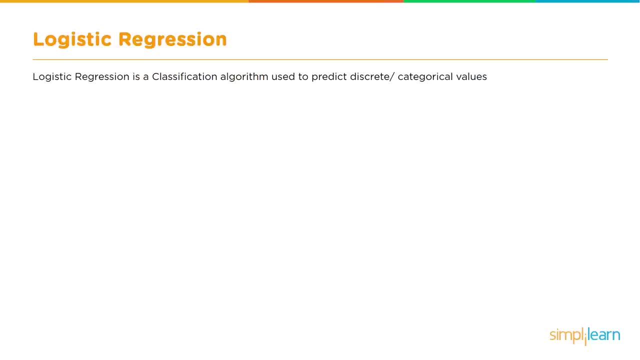 value, whereas logistic regression is used to solve a classification problem. So we are trying to find, for example, whether a person will repay the loan or not, or whether we want to find whether this image is of a cat or a dog. So this is a classification problem. 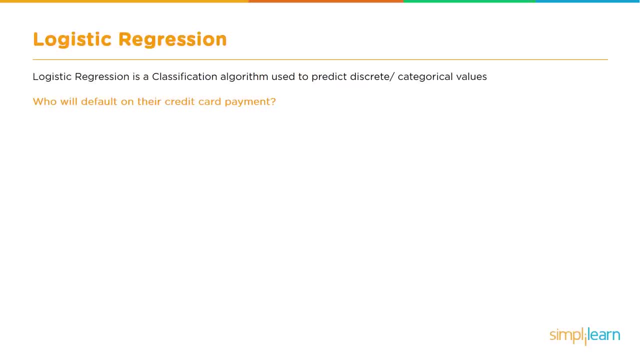 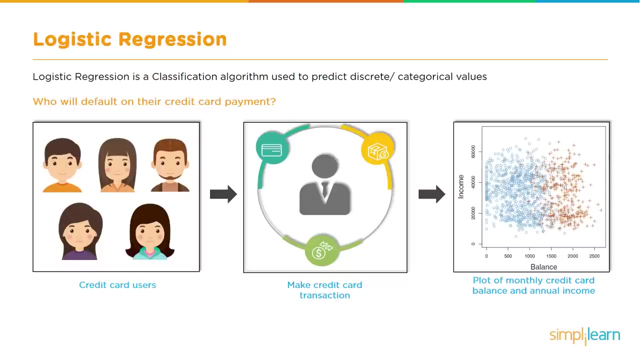 So just that you should be aware of the name. So in this slide we are talking about whether a person, credit card user or credit card holder, will default on the payment So we can create a profile- we have historical data and of people, their income and their 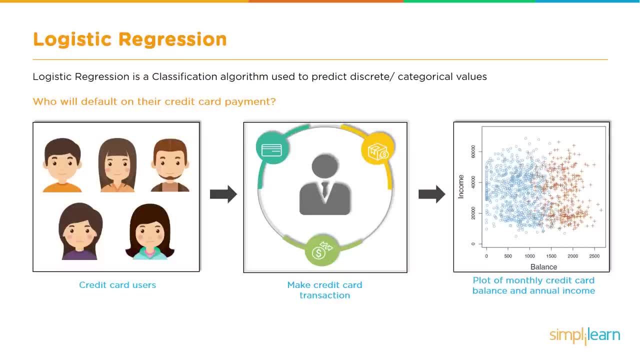 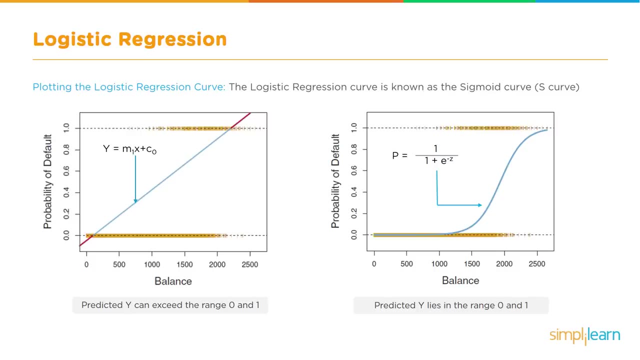 credit card balance, And we have examples of people who have defaulted and people who have not defaulted, And based on that, we let the system learn to predict this particular value, whether the person will default on the payment or not. Now, how does the logistic regression work? 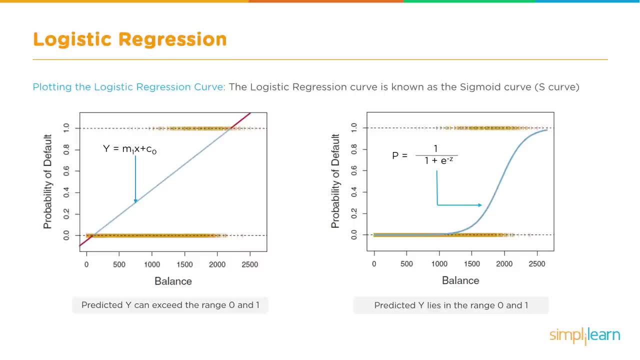 If we try to draw a straight line to determine the probability, so we are trying to predict whether this person will default or not. okay, So if we draw a straight line, then the predicted value can exceed 0 and 1, which is not a good. 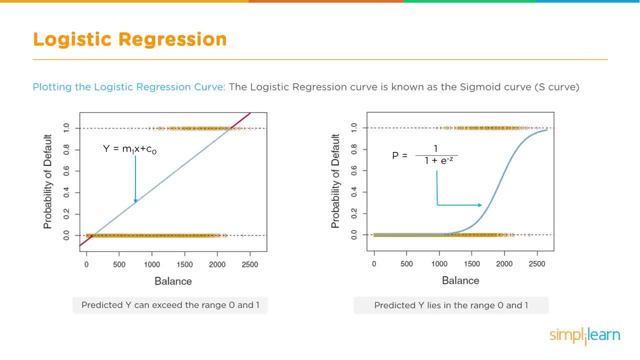 one. So the probability is calculated between 0 and 1 using what is known as a sigmoid curve. So it is not a straight line, but we use a different formula, a different mechanism to find the probability and find the value between 0 and 1.. 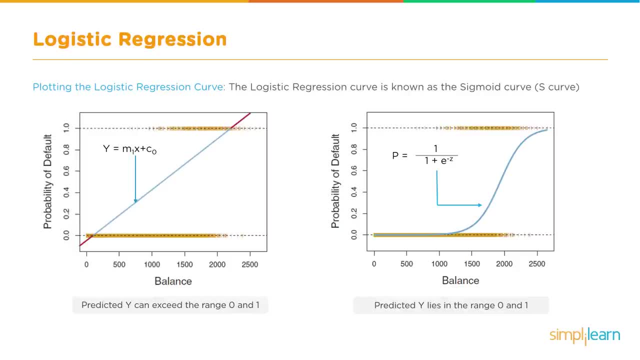 And the formula for that is: P is equal to 1 by 1 plus e, to the power of minus z. Here z is actually the linear equation that we used in figure 1.. So z is equal to m1 x plus c0. 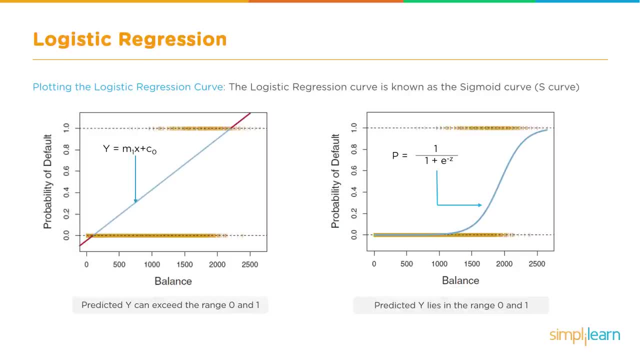 So this is fed to P and the value is calculated between 0 and 1.. And we will see, actually, mathematically, we will see here that if z is negative and much, much higher, a very high value it will. the equation will be 1 by 1 plus 0, which is equal. 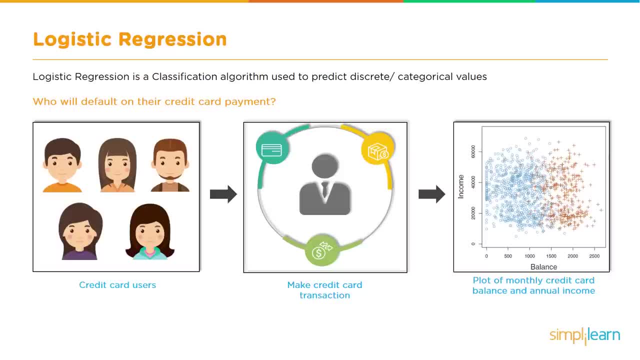 payment so we can create a profile. we have historical data and of people, their income and their credit card balance, and we have examples of people who have defaulted and people who have not defaulted and, based on that, we let the system learn to predict this particular value: whether the person will default on the payment or not. now how? 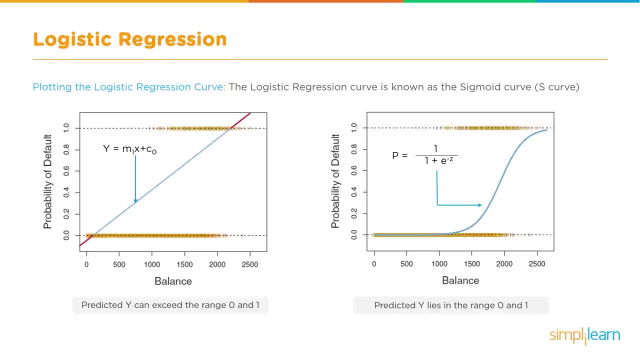 does the logistic regression work if we try to draw a straight line to determine the probability, so we are trying to predict whether this person will default or not. okay, so if we draw a straight line, then the predicted value can exceed 0 and 1, which is not a good idea. so the probability is calculated between 0 and 1 using what is known. 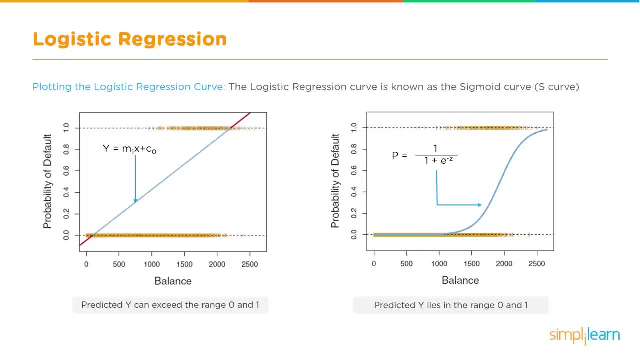 as a sigmoid curve, so it is not a straight line. but we use a different formula, a different mechanism to find the probability and find the value between 0 and 1, and the formula for that is: p is equal to 1 by 1 plus e to the power of minus z. here z is actually the linear equation that we used in. 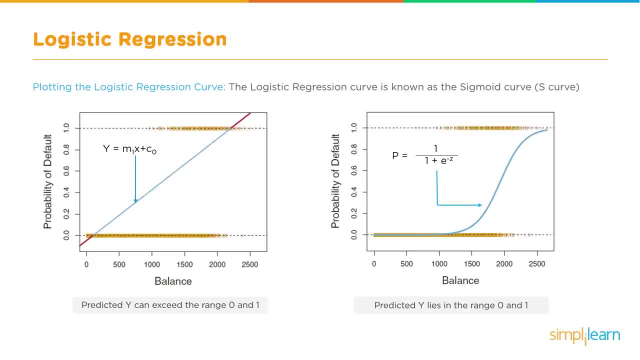 figure 1, which is m1x plus c0. so this is fed to p and the value is calculated between 0 and 1 and we will see, actually, mathematically, you will see here that if z is negative and much, much higher, a very high value it will. the equation will be one by one plus zero, which is equal to one. 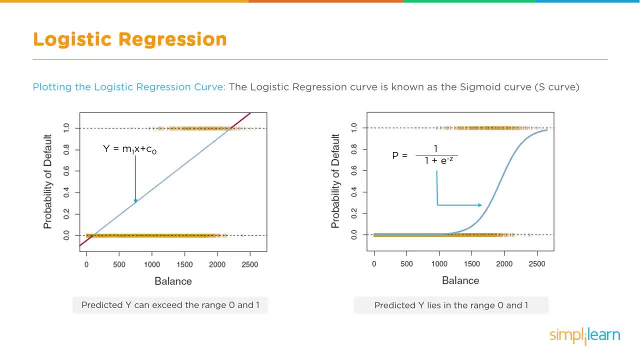 so we will see here that if the value of z is positive, and it is some high number, then the value of p can at the most be equal to one, because this portion here is one by a very high number, let's say Infinity. so one by Infinity is zero. so this whole thing becomes one by one. so that is. 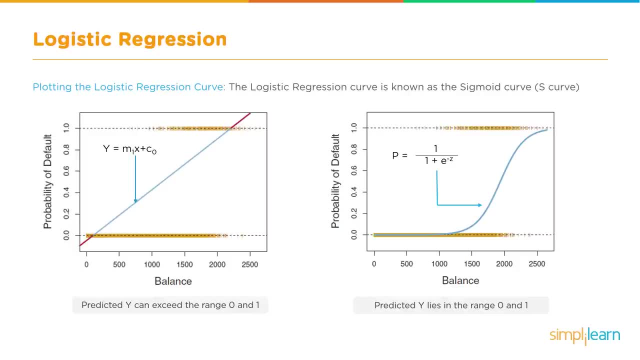 equal to one, p is equal to one, so that is where it the maximum value it can achieve as well. similarly, if the value is negative, if the z value is negative or negative and very high value, then this will become very high and therefore the denominator will become Infinity. so 1 by Infinity is 0 and therefore p is equal to 0.. so that's the. 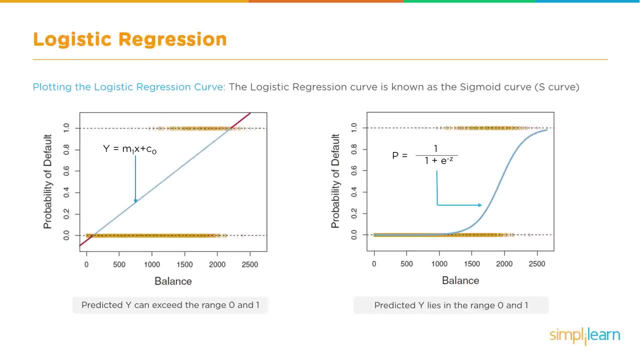 to 1.. So we will see here that if the value of z is positive, and it is some high number, then the value of P can at the most be equal to 1.. Okay, P is equal to 1 because this portion here is 1 by a very high number, let's say infinity. 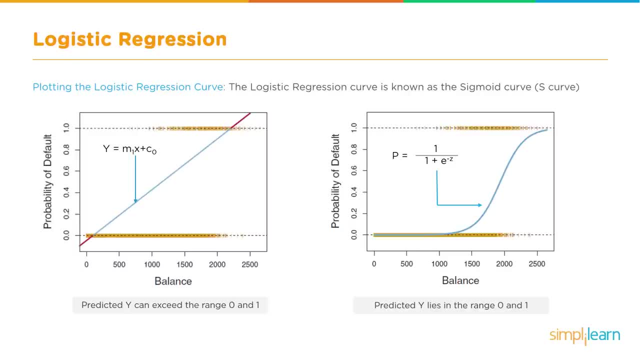 So 1 by infinity is 0. So this whole thing becomes 1 by 1.. So that is equal to 1, P is equal to 1.. So that is where the maximum value it can achieve is 1.. Similarly, if the value is negative, if the z value is negative or negative and very high, 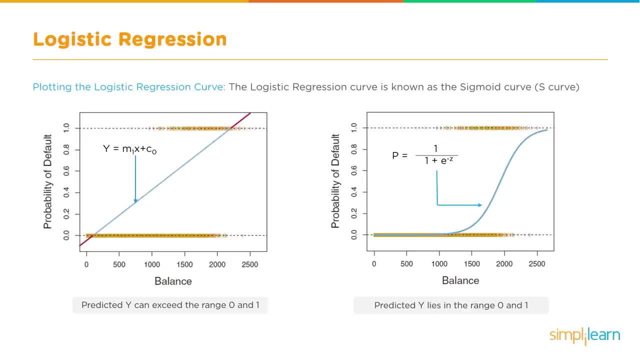 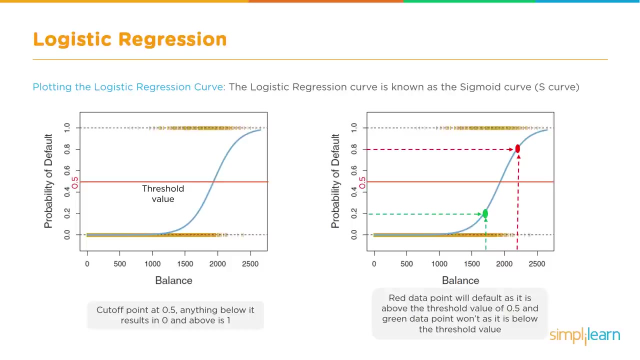 value, then this will become very high and therefore the denominator will become infinity. So 1 by infinity is 0 and therefore P is equal to 0.. So that's the way the sigmoid function works. This is how the graph looks, And there has to be a threshold value which is, like in this case, 0.5.. 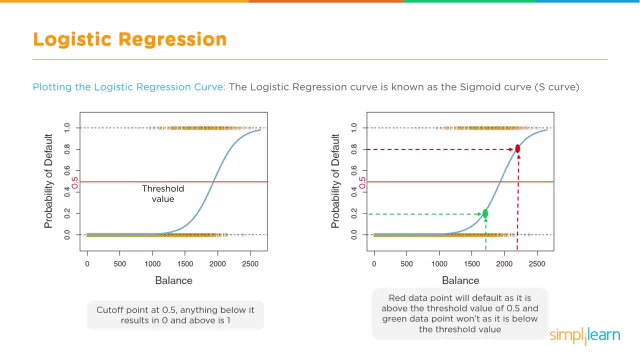 So, if the value is greater than 0.5, we consider the output as 1, whereas if the value is less than 0.5, we consider the value as 0. Because- remember, let me go back- in this case it doesn't exactly give us a 1 or a 0. 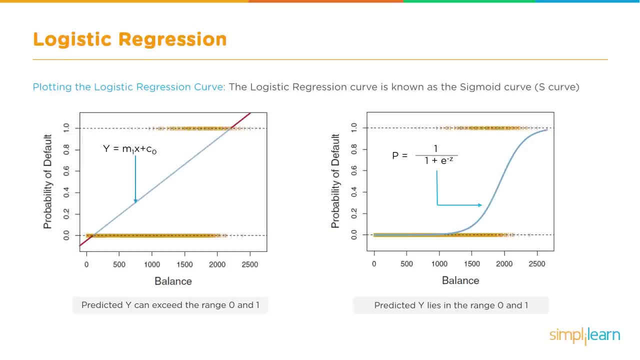 Okay, So we need to keep that in mind. It doesn't give us exactly a 1 or a 0. It will give a value between 0 and 1, irrespective of what the value of z is. It will give us a value between 0 and 1.. 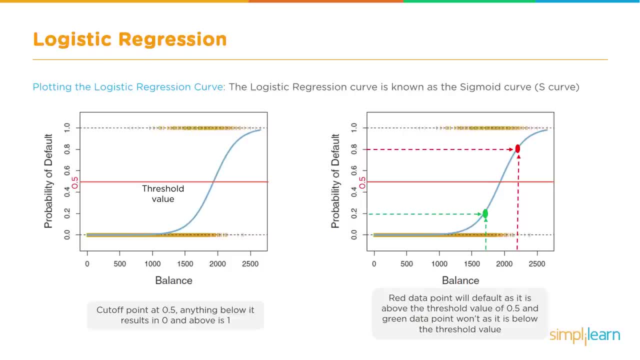 It's like the probability between 0 and 1.. Now we have to have a threshold and then, based on what the value is, if the value is greater than 0.5, then we say, okay, this probability is 1, and if the value is less than 0.5, the 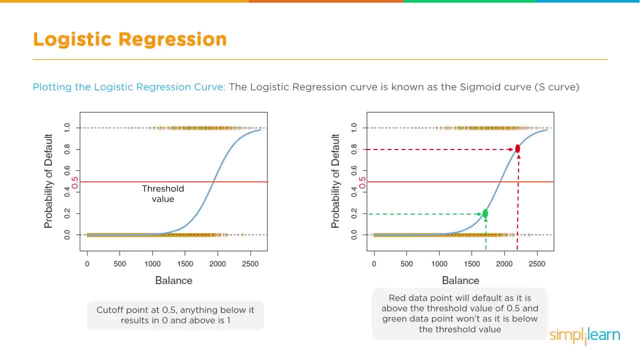 probability is 0.. So we decide that based on the cutoff or a threshold value. So, for example, we continue on that. If a person having a balance of- maybe this is 1,750,, then the probability that he will repay the loan is 0.2, which means which is less than 0.5, the threshold value which 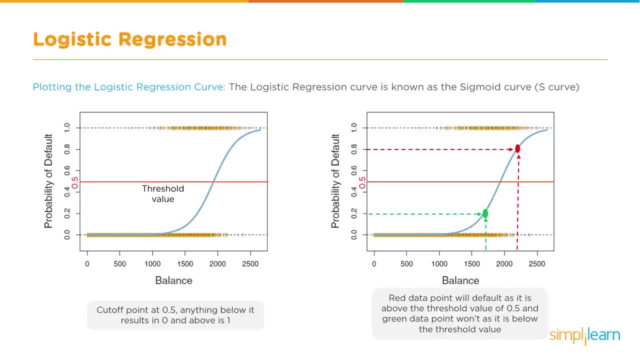 we have set, That means the probability is 0,, which means the person will not repay, Whereas if the balance is somewhere in the range of 2,250 maybe, which is this red dot- then the sigmoid function calculates the probability of default. 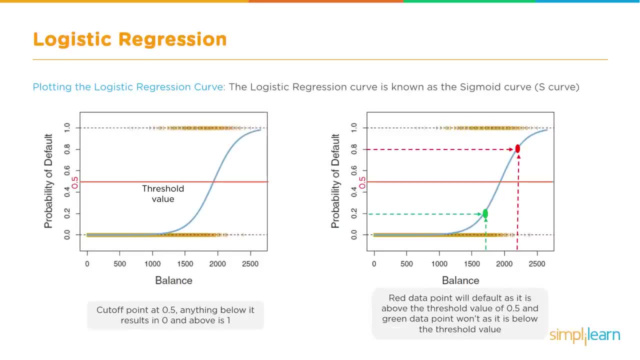 way the sigmoid function works. this is how the graph looks- and there has to be a threshold value which is, like in this case, 0.5. so if the value is greater than 0.5, we consider the output as one, whereas if the value is less than 0.5. 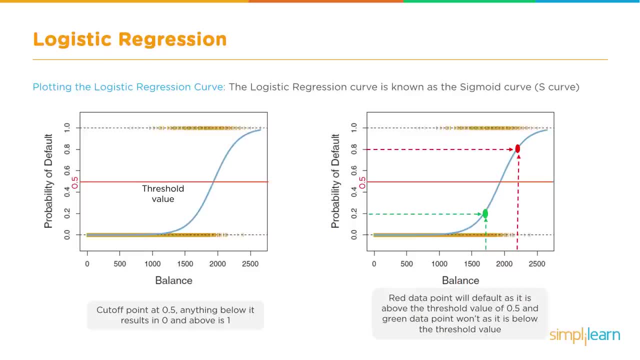 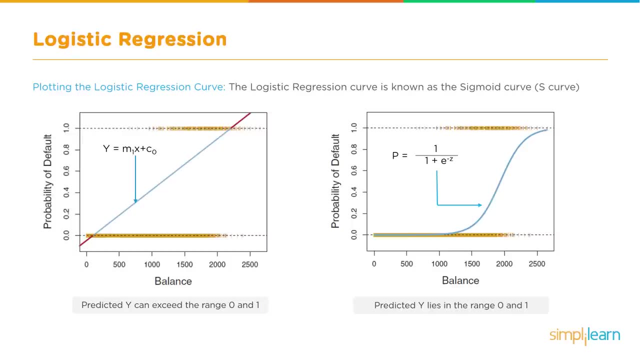 we consider the value as zero because- remember, let me go back in this case- it doesn't exactly give us a one or a zero. okay, so we need to keep that in mind. it doesn't give us exactly a one or a zero. it will give a value between zero and one, irrespective of what the value of z is it. 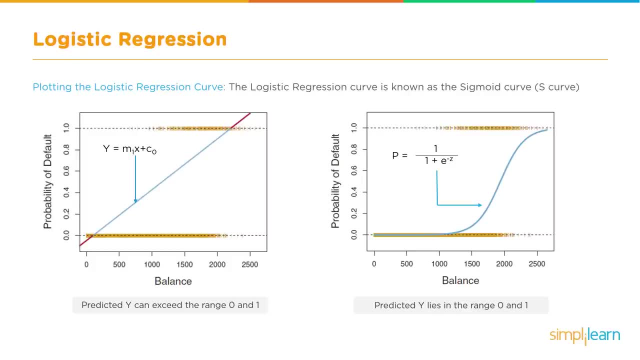 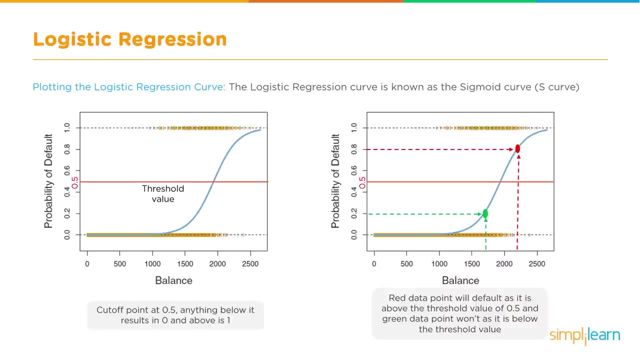 will give us a value between zero and one. it's like the probability between zero and one. now we have to have a threshold and then, based on what the value is, if the value is greater than zero, then we say, okay, this probability is one, and if the value is less than 0.5, the probability is. 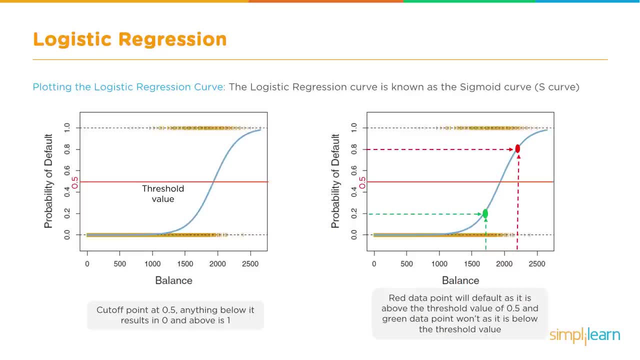 zero. so we decide that based on the cutoff or a threshold value. so, for example, if we continue on that, if a person having a balance of- maybe this is 1750, then the probability that he will repay the loan is 0.2, which means which is less than 0.5 the threshold value which we have said, that 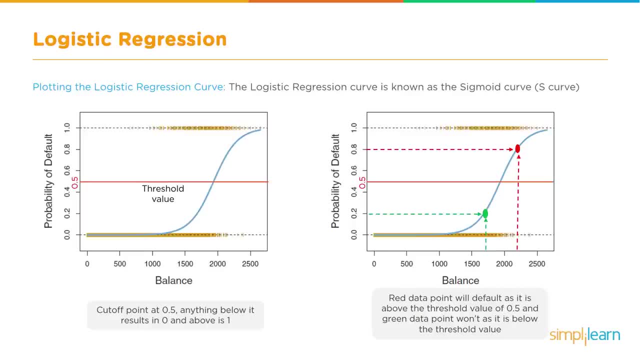 means the probability is zero, which means the person will not repay, whereas if the balance is somewhere in the range of 2250 maybe, which is this red dot, then the sigmoid function calculates the probability of default as point eight, which means the output is one, which means: 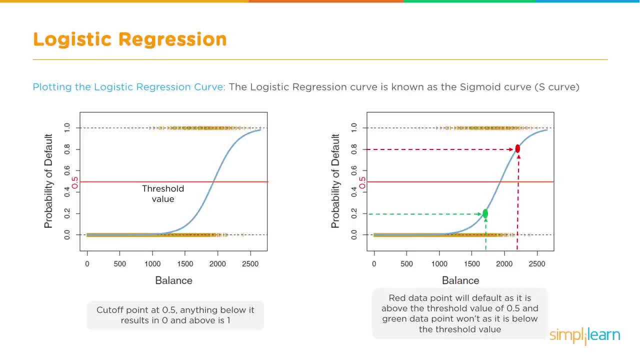 the person will default on payment. okay, so that is how the logistic regression works. so in this case it says that, okay, this person will default. so it is classified as a defaulter. in this case, the the second one, and in the first case it is a non-default. so these are the two. 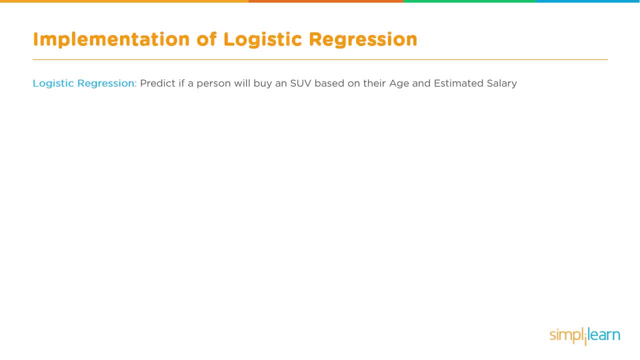 different classes of these two different cases. so let's move on and see how logistic regression is implemented. so this is another example of logistic regression. can we predict whether a person is going to buy an SUV based on their age and their estimated salary? so these are our two. 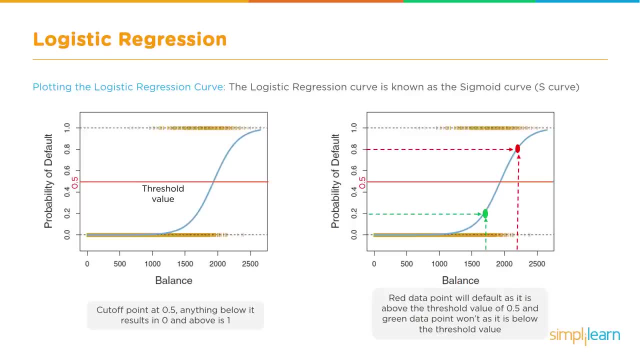 Okay, So that is how the logistic regression works. So in this case it says that, okay, this person will default. it is classified as a defaulter, In this case the second one, and in the first case it is a non-default. 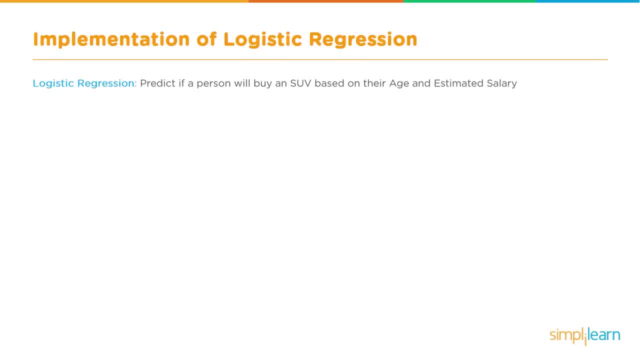 So these are the two different classes of these two different cases. So let's move on and see how logistic regression is implemented. So this is another example of logistic regression: Can we predict whether a person is going to buy an SUV based on their age and their estimated? 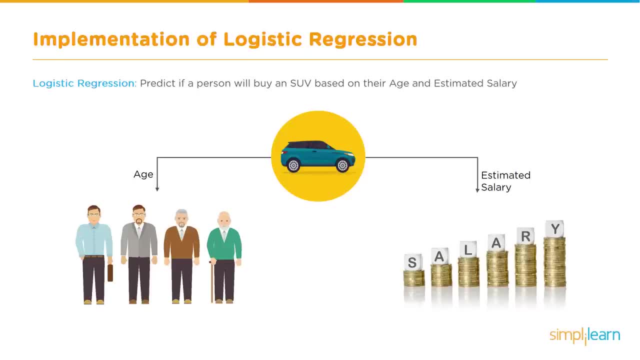 salary. So these are our two inputs And based on that can we predict whether this person will buy an SUV or not. So this is a logistic regression problem And we are going to demonstrate this using PythonCard and in Jupyter Notebook. 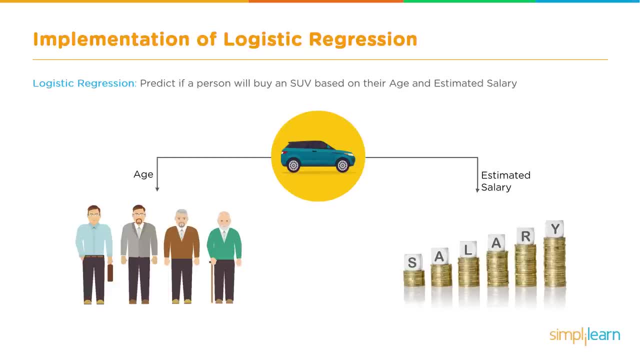 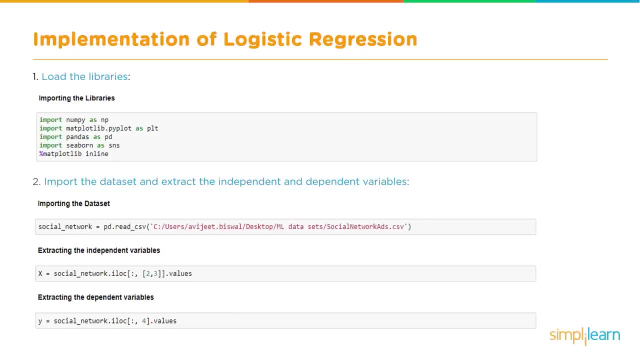 And before going into Jupyter Notebook, let's take a look at how we go about solving this problem and how the code looks. So this is the implementation of logistic regression. This is the code, the Python code. I just take you very briefly, at a high level, what each parts are. 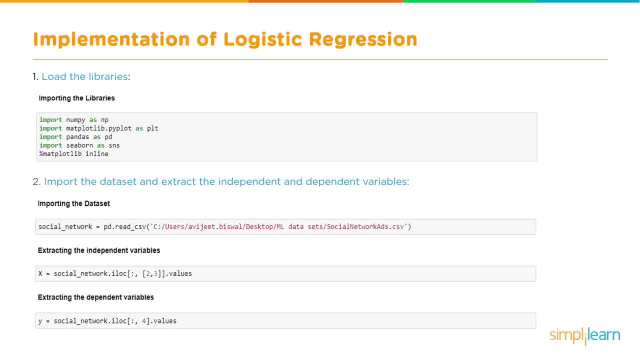 So first section, of course, is importing the libraries, and then we import the data set And within this data set we just take, for performing or for training, our model. we only take the independent variables into one, create one vector, and then we extract the labels. 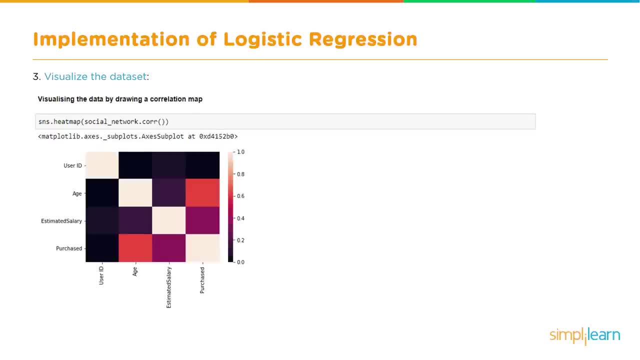 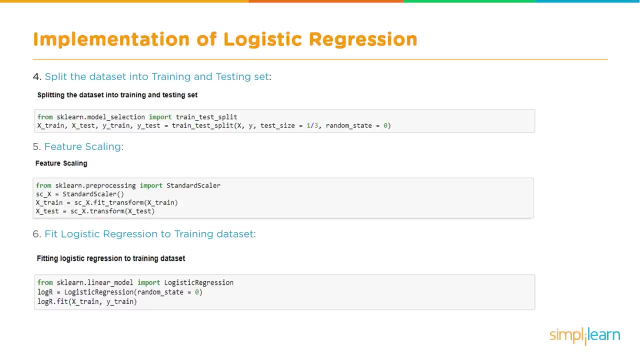 separately, And then we visualize our data. This is how the data looks- And then we split the data into training and test set, like we did in linear regression, And we do some feature scaling as well, which improves the performance of our model. 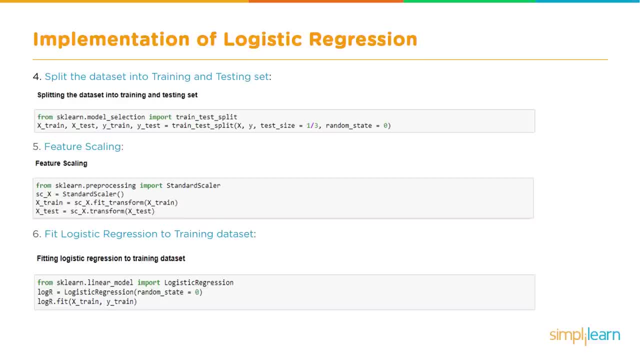 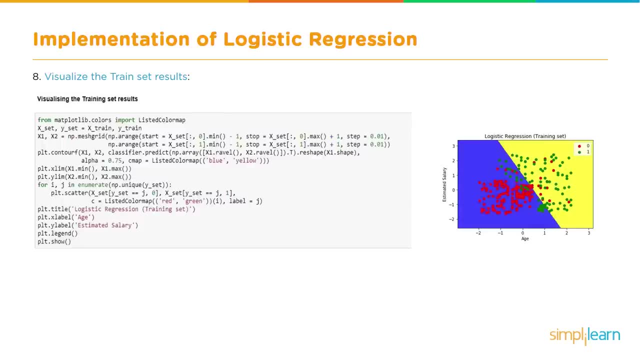 And then we train and test the model. So these are the test results and we visualize the test results. So this is the visualization of the trained results. They look pretty good. The classification: they are reasonably accurately classified. The red dots and the green dots. 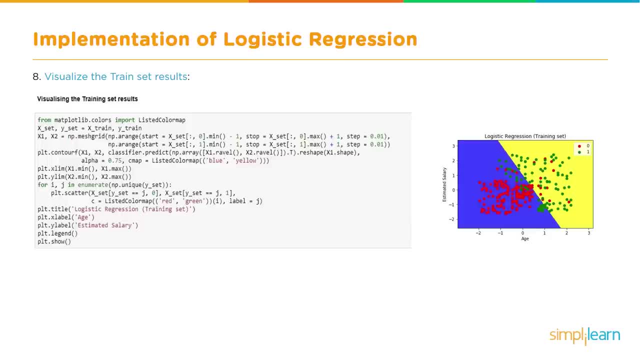 And there are a few, of course, miscalculations or misclassifications, But by and large it looks pretty good. And this is the visualization of the test results. again looks pretty good. And then we evaluate our model and this is what we'll be doing in the code as well. 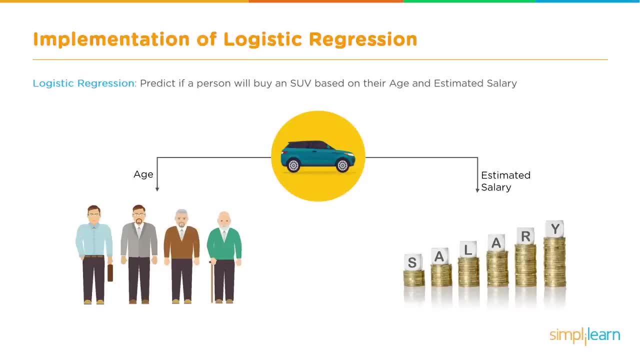 inputs and based on that can we predict whether this person will buy an SUV or not. so this is a logistic regression problem and we are going to demonstrate this using python curd and in Jupiter notebook. and before going into Jupiter notebook, let's take a look at how we go about. 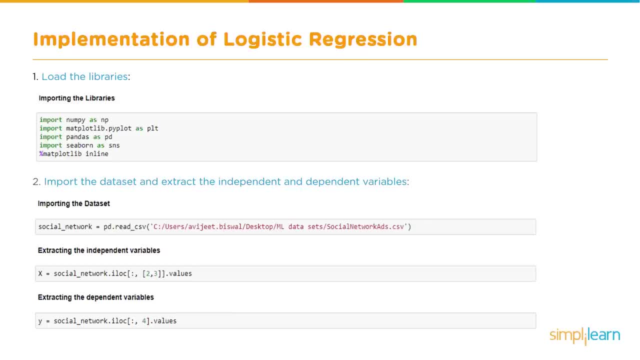 solving this problem and how the code looks. so this is the implementation of logistic regression. this is the code, the python code. I just take you very briefly, at a high level, what each parts are. so first section, of course, is importing the libraries, and then we import the data set and 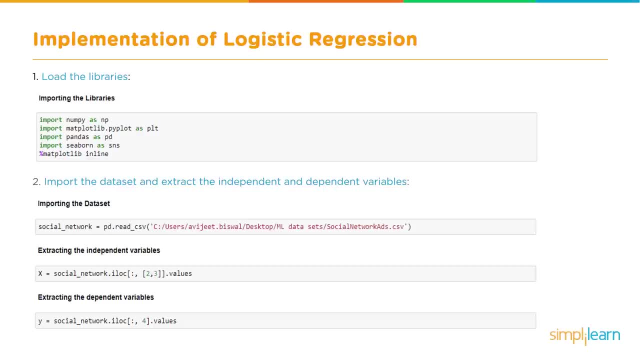 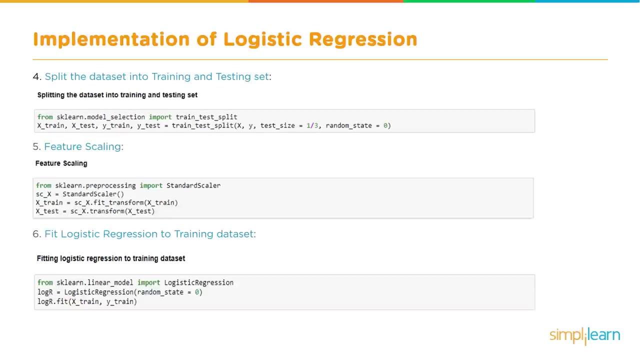 within this data set we just take for performing or for training our model. we only take the independent variables into one create one vector, and then we extract the labels separately and then we visualize our data. this is how the data looks and then we split the data into training and test set, like we did in. 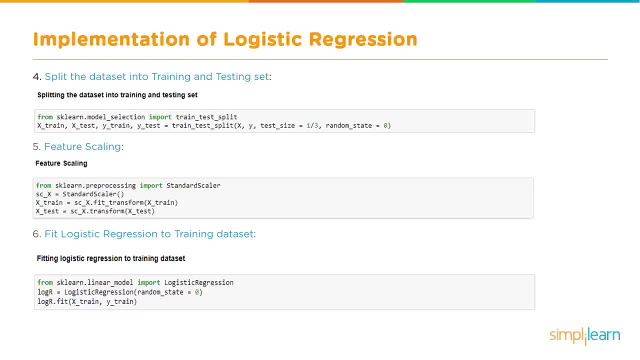 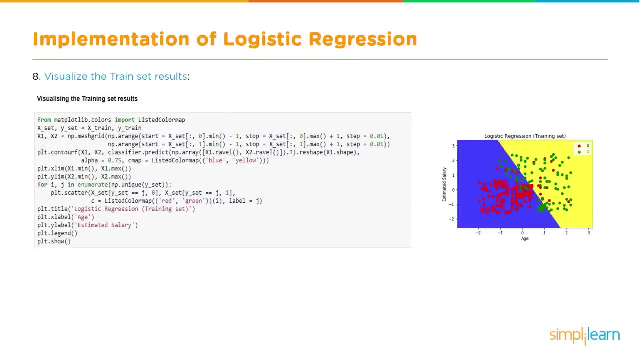 linear regression and we do some feature scaling as well, which improves the performance of our model. and then we train and test the model. so these are the test results and we visualize the test results. so this is the visualization of the trained results. they look pretty good. the classification: then they are reasonably accurately classified. the 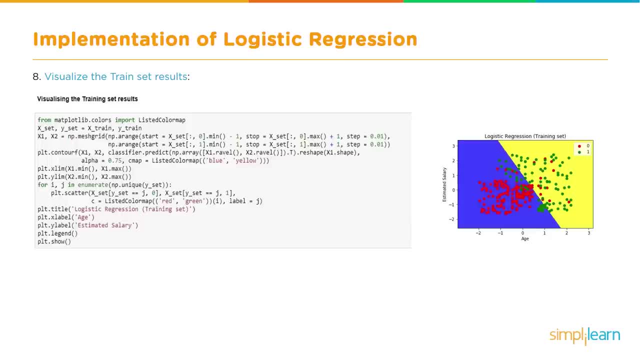 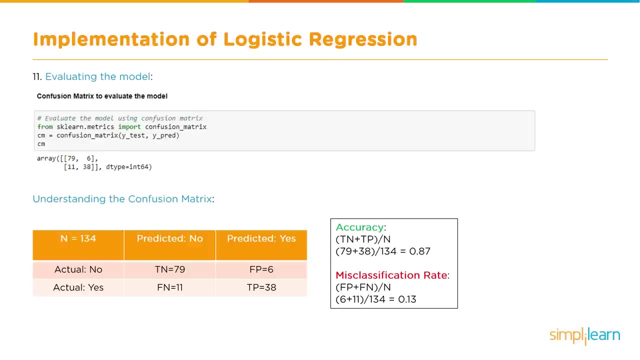 red dots and the green dots, and there are a few, of course, miscalculations or misclassifications, but by and large it looks pretty good. and this is the visualization of the test results. again, uh, looks pretty good. and then we evaluate our model and this is what we'll be doing in the 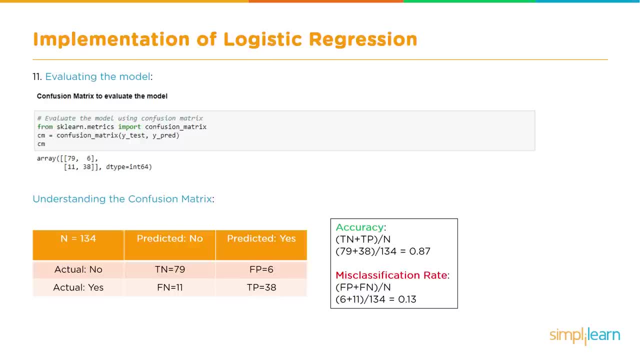 code as well, and for this we use what is known as confusion matrix. now let's try to understand what this confusion Matrix is. I know the name itself is confusing, but actually it is very simple. now, once we predict these values and compare with the actual values, we can create or represent the 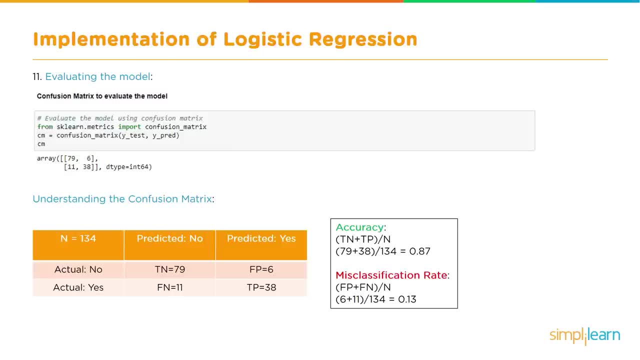 results in the form of a matrix. so we have all together 134 observations and, if we put it in a tabular form, the predicted values and the actual values. first of all, in order to identify whether the model is more accurate or less accurate, the criteria is that the values along the diagonal 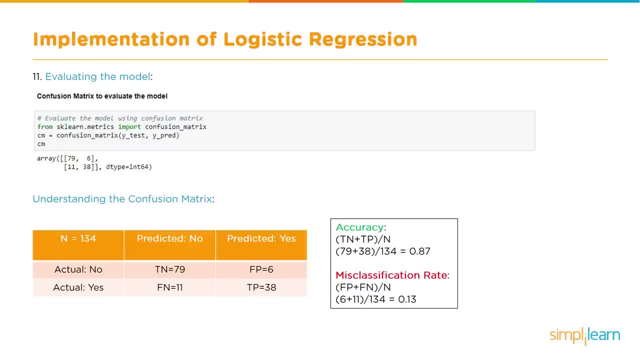 And for this we use what is known as confusion matrix. Now let's try to understand what this confusion matrix is. I know the name itself is confusing, but actually it is very simple. Now, once we predict these values and compare with the actual values we can create or represent. 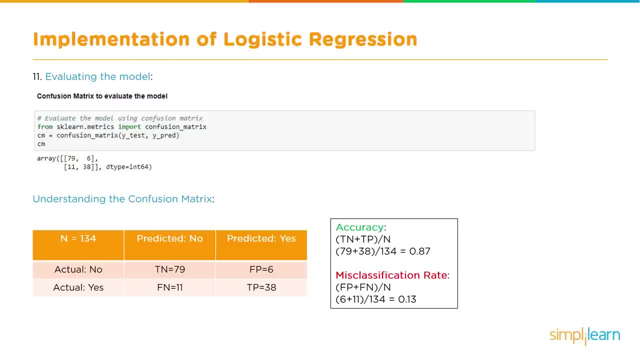 the results in the form of a matrix. So we have altogether 134 observations And, if we put it in a tabular form, the predicted values and the actual values. first of all, in order to identify whether our model is more accurate or less accurate. the criteria: 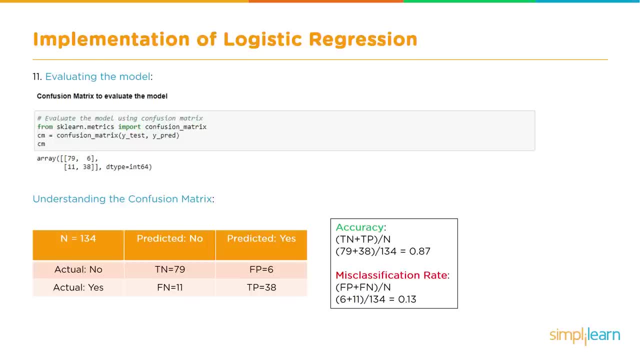 is that the values along the diagonal should be maximum. So, for example, this is 79 and this is 38. The sum of these should be maximum. So what do we mean by that? That means that if we have a perfect model, then this sum will be equal to 134 and the 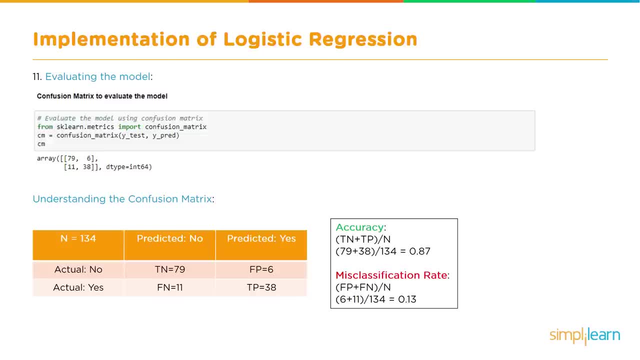 values here will be zero. So that is an ideal, perfect, logistic regression model. That is, of course, very rare, But that is the aim. The sum of these numbers, Okay, Or the maximum numbers, should be in the diagonal, and in the other cells there should be as: 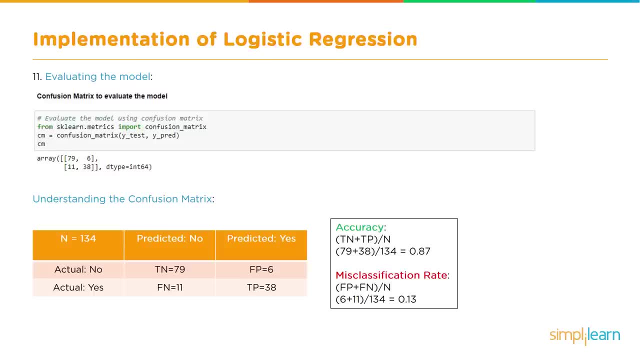 less as possible. Okay, So here we see, in this case, that it is 79 plus 38, and so that is equal to 117.. So 117 of them have been correctly predicted, which gives us an accuracy of 87%. So out of 134,, 117 have been correctly predicted. 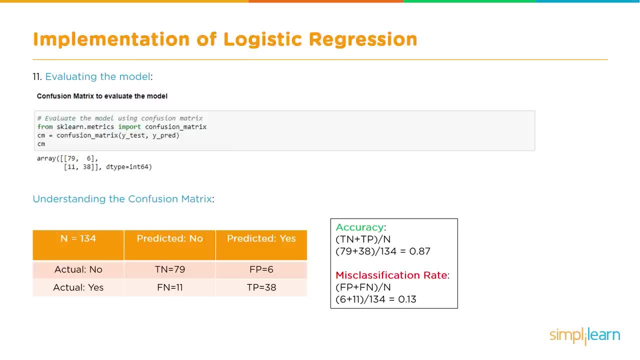 And the 6 plus 11.. 17 of them have been incorrectly, So this is 6 plus 11, 17 of them have been misclassified, So which is about 0.13%. So we have an accuracy of 87%. 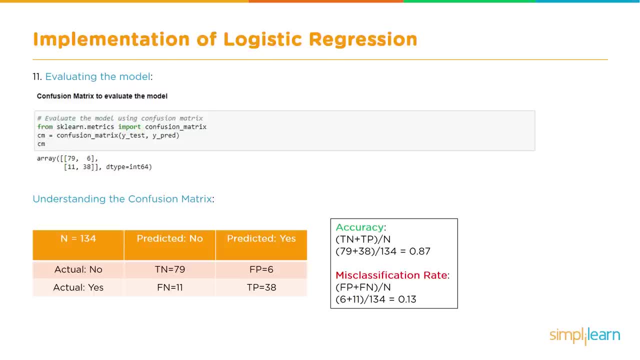 should be maximum. so, for example, this is 79 and this is 38. the sum of these should be maximum. so what do we mean by that? that means that if we have a perfect model, then this sum will be equal to 134 and the values here will be zero. so that is an ideal, perfect, logistic regression model. that is 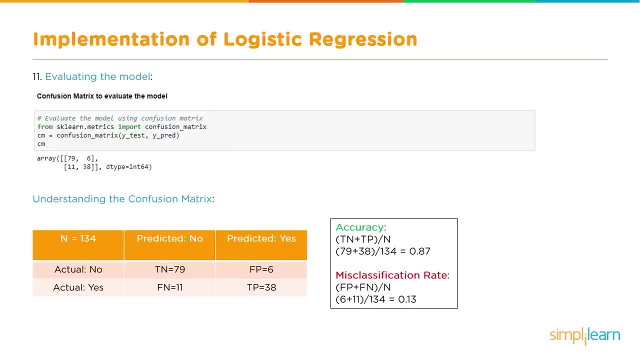 of course very rare, but that is the aim. the sum of these numbers are the maximum numbers should be in the diagonal, and in the other cells there should be as less as possible. okay, so here we see in this case that it is 79 plus 38, and so that is equal to 117.. so 117 of them have been. 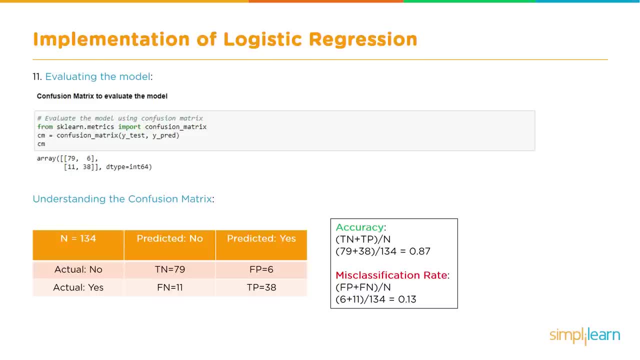 correctly predicted, which gives us an accuracy of 87 percent. so, out of 134, 117 have been correctly predicted, and the 6 plus 11, 17 of them have been incorrectly, so this is 6 plus 11, 17 of them have been misclassified, so which is about 0.13 percent, so we have an accuracy of 87 percent. 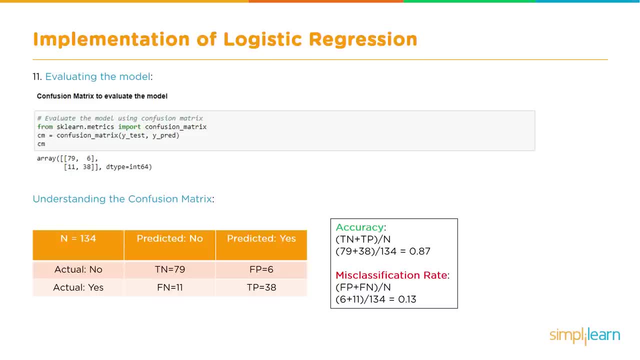 okay, so I hope the way we calculate, or with the way we find accuracy from confusion Matrix. I hope it is clear. by the way, once again a quick reminder: if you need this data set to perform this on your own, please put a comment and under the this video, and we will send you the data set. all right, so let's go and check in Python notebook how. 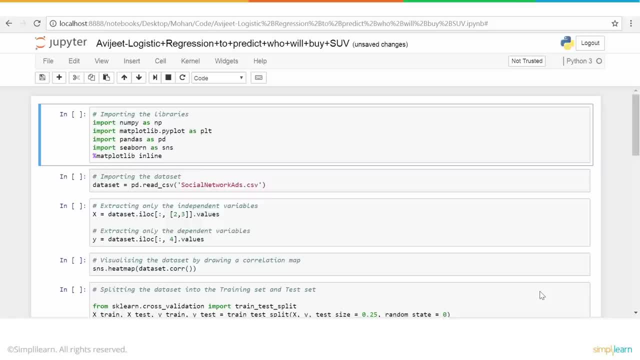 exactly this is done, all right. so this is the demo of logistic regression, and here what we are doing is we have taken an example of a data set and a scenario where we will predict whether a person is going to buy an SUV or not, and we will use logistic regression for this and the parameters. 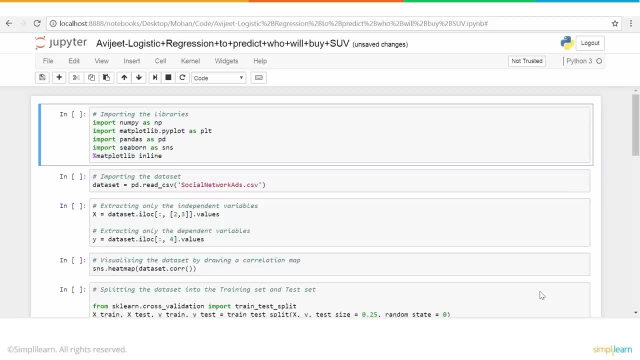 we will take are, for example, the person's age, is the salary and a few other parameters. we will see very quickly what those are. okay, so the first step, we import the required libraries- so that's what we are doing in this particular cell- like, for example, numpy, matplotlib, pandas, so for performing any preparation of the data before we actually 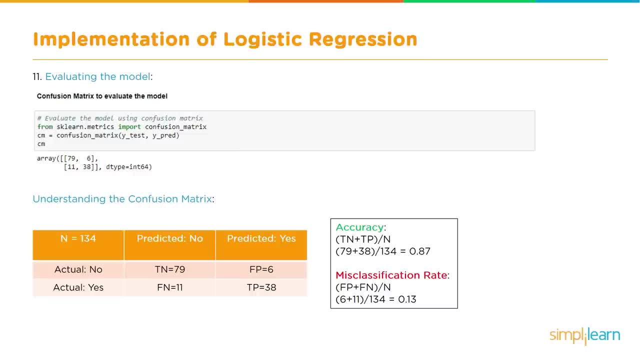 Okay, So I hope the way we calculate, or with the way we find accuracy from confusion matrix. I hope it is clear. By the way, once again a quick reminder: if you need this data set to perform this on your own, please put a comment and under this video, and we will send you the data set. 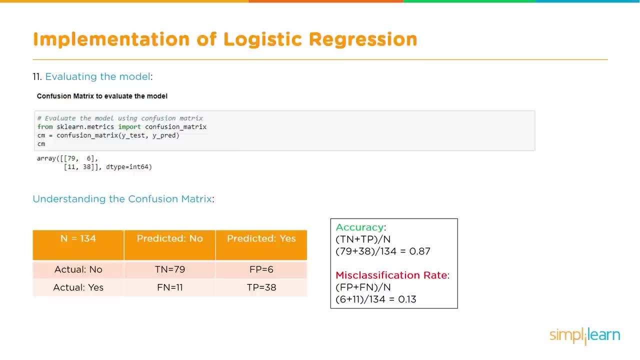 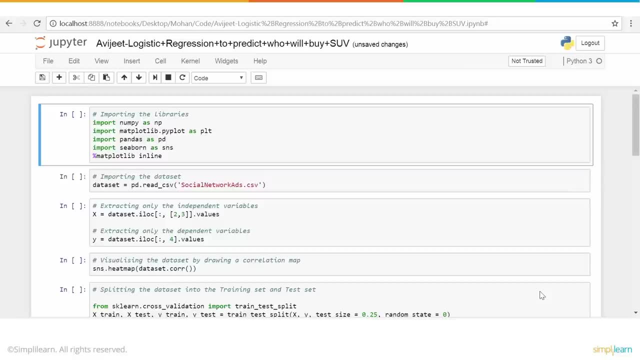 All right, So let's go and check in Python notebook how exactly this is done. All right, So this is the demo of logistic regression, And here what we're doing is we've taken an example of a data set and a scenario where 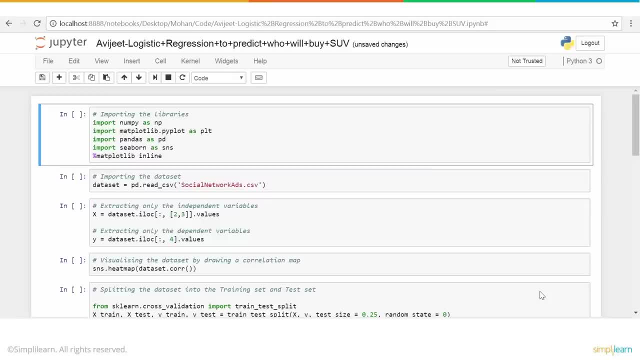 we will predict whether a person is going to buy an SUV or not, And we will use logistic regression for this, And the parameters we will take are, for example, the person's age, his salary and a few other parameters, And we will see very quickly what those are. 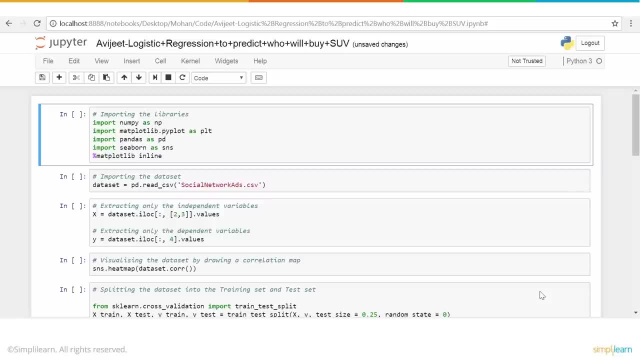 Okay, So the first step, we import the required libraries- So that's what we are doing in this particular cell- like, for example, NumPy, Matplotlib, Pandas, So for performing any preparation of the data before we actually launch into the learning. 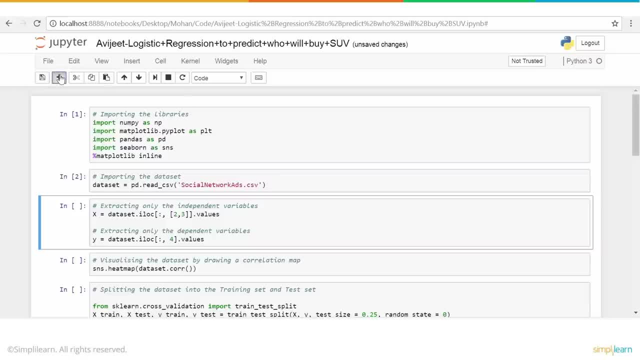 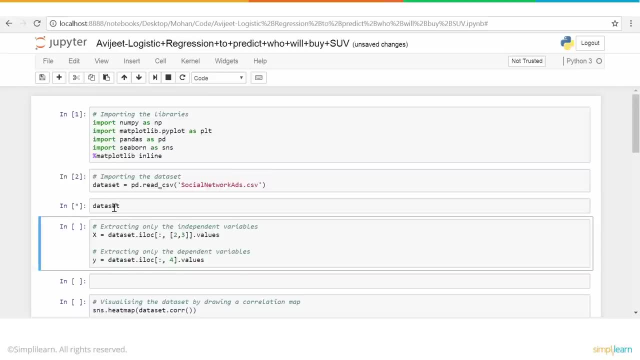 process And then we load the data. So let me just introduce one more cell and see how the data looks. So why don't we do that here? And if I say data set and then if I run this, this is our data set. 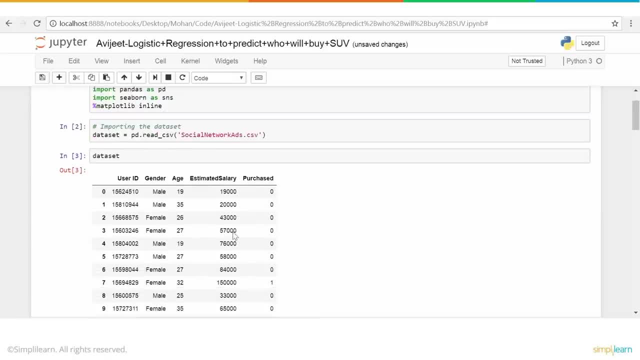 Okay, Okay, So this is how our data looks. So these are the parameters, or the features, as we call it in machine learning language. We have gender, age and estimated salary. User ID is also there, but it's not really a feature. it will probably not contribute. 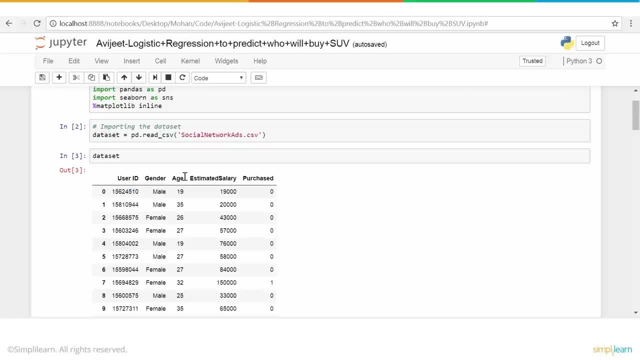 So we will not be using this. We will primarily be using these three columns And in technical terms, these columns are known as predictors. And then we have the labeled value. This is known as our target And this is the labeled value. 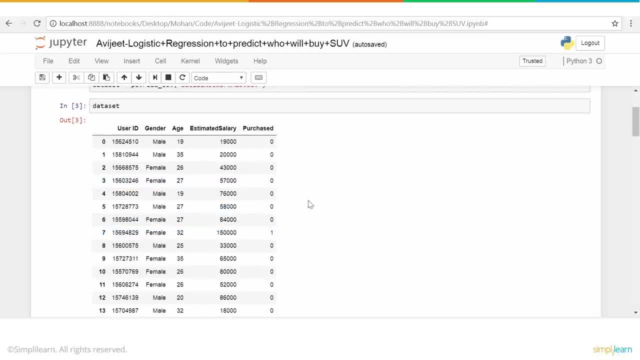 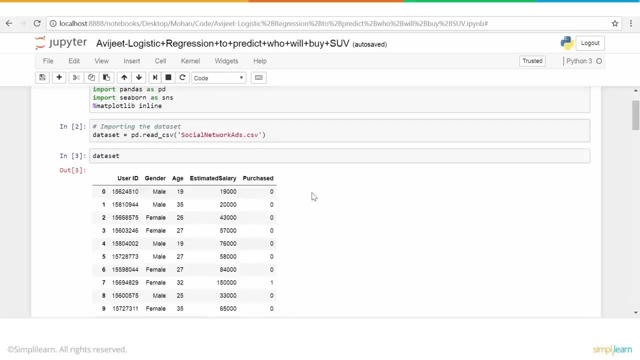 So it has zero or one. So we are basically performing a binary classification- zero or one- whether the person will purchase or not purchase. Zero means he will not purchase, One means he will purchase. Okay, And the other way of also looking at it is from a more from a mathematical perspective. 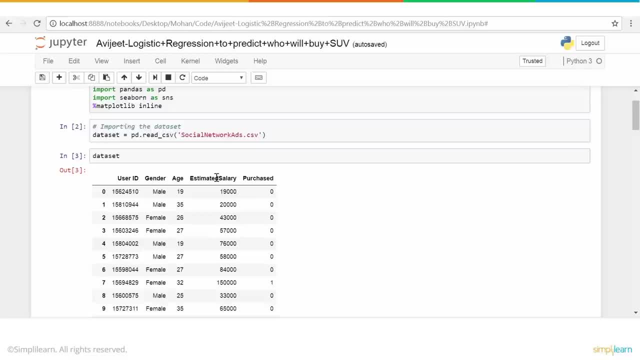 These are our independent variables. gender, age and estimated salary are our independent variables and purchased is our dependent variables. So in our equation, like, y is equal to something, something 1x plus mx And so on. This is our y. 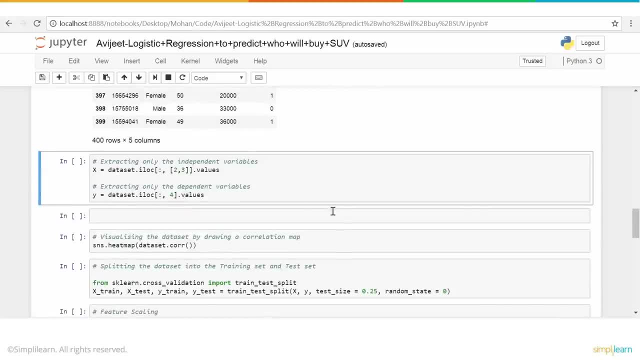 Okay, All right. So now let's move forward. What we will do next is to extract this, the, or separate out the independent variables and the dependent variables. How do we do that? So we load them into x, capital, X and y. 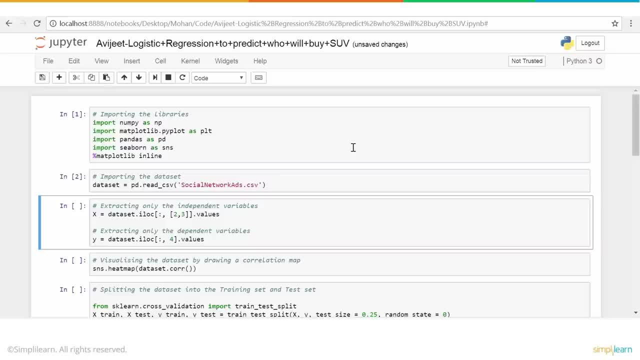 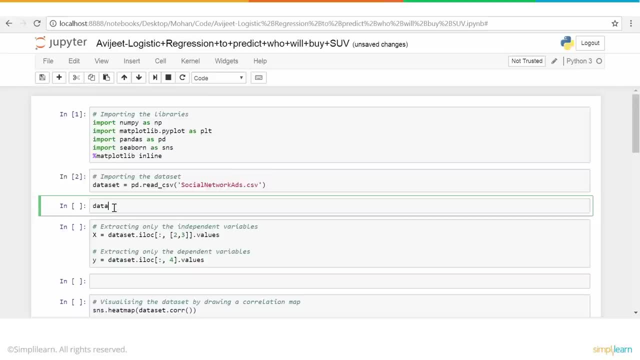 launch into the learning process and then we load the data. so let me just introduce one more cell and see how the data looks. so why don't we do that here? and if I say data set and then if I run this, this is how our data looks. so these are the parameters or the features. 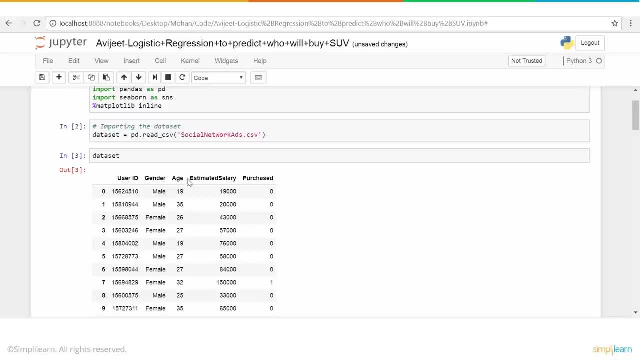 as we call it in machine learning language. we have gender, age and estimated salary. user ID is also there, but it's not really a feature. it will probably not contribute, so we will not be using this. we will primarily be using these three columns and, in technical terms, these columns: 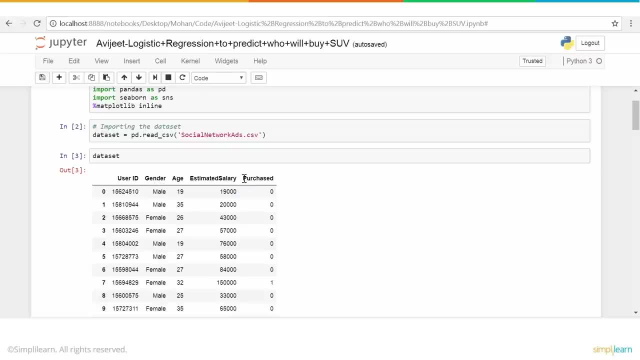 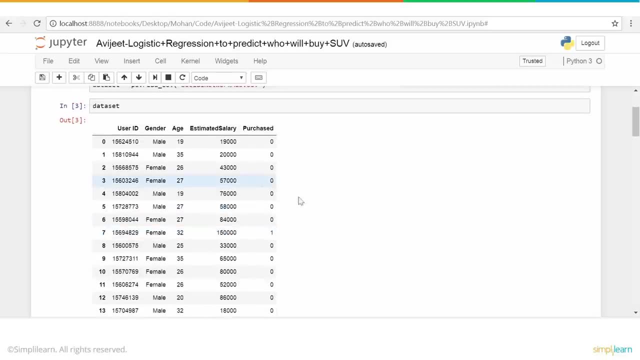 are known as predictors, and then we have the labeled value. this is known as our target and in this is the labeled value. so it has zero or one. so we are basically performing a binary classification- zero or one- whether the person will purchase or not purchase. zero means he will not. 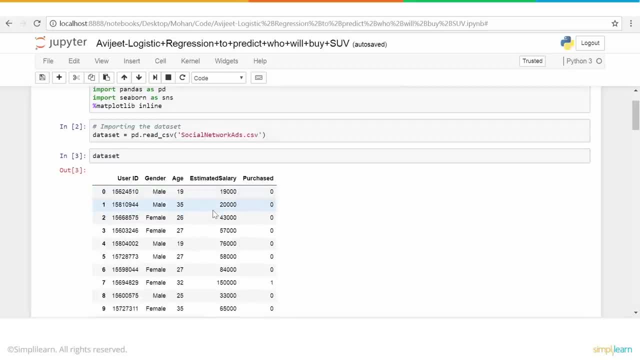 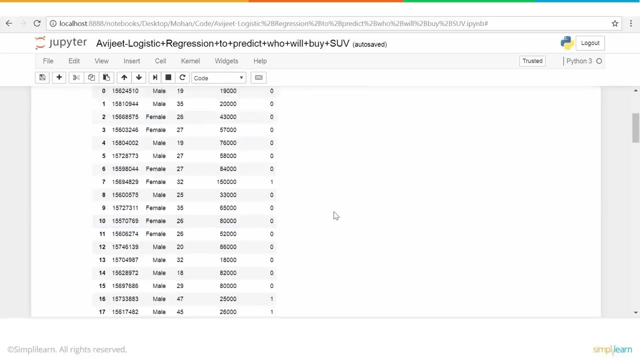 purchase. one means he will purchase, okay, and the. the other way of also looking at it is from a more, from a mathematical perspective. these are our independent variables. gender, age and estimated salary are our independent variables and purchased is our dependent variables. so in our equation, like we do something, something, 1x plus m2x and so on, this is our Y. okay, all right, so now let's move. 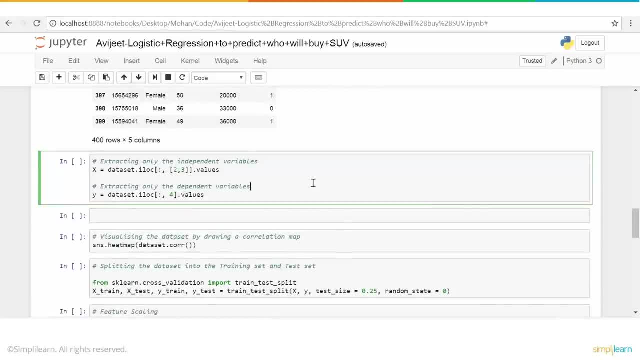 forward. what we will do next is to extract this, the, or separate out the independent variables and the dependent variables. how do we do that? so we load them into X capital, X and Y, and what we are doing here is we are taking the second and the third column, we are taking these three right. so 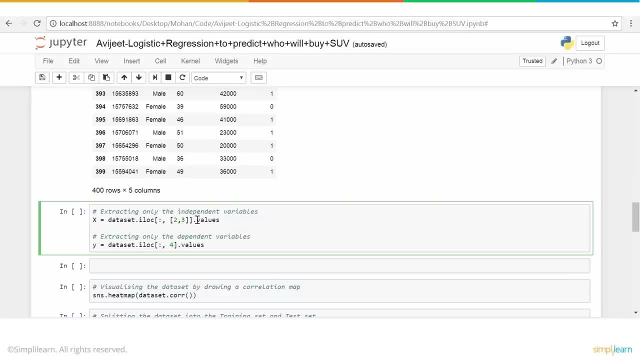 gender, age and estimated salary. so that is what we are taking here: two up to three, and then Y is basically the last column, which is the fourth column. so let's go ahead and extract that. and, once again, why don't we take a look at how the data is looking? so let me just print X. so we only- yeah, we are basically taking 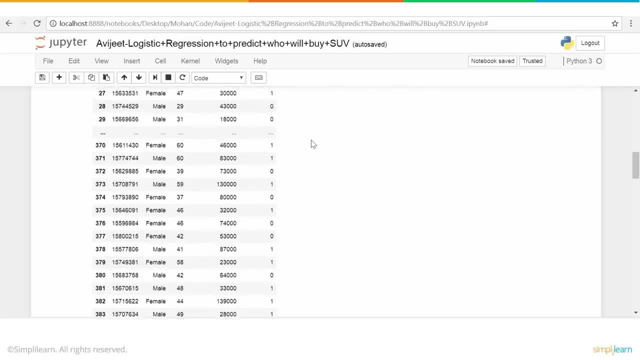 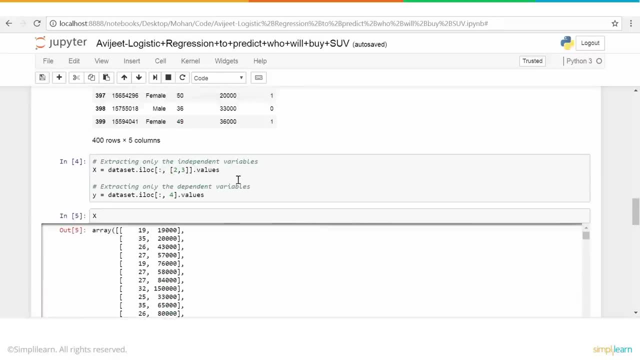 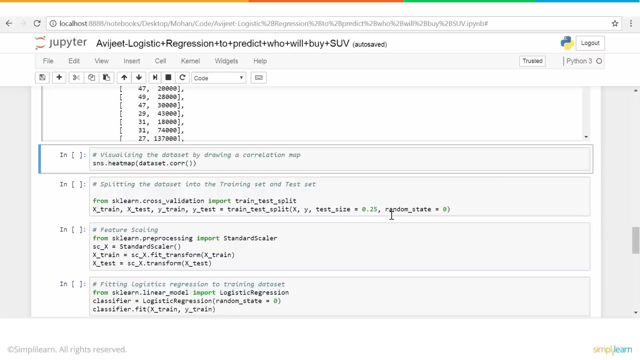 two and three. so what is two and three? two and three is our age and our estimated salary. yeah, that's right. so these are the only two independent variables, and our dependent variable is obviously the last one- whether the person will buy or not. okay, so we have the data loaded now let's, now that we have the data in uh python, let's take a quick look at. 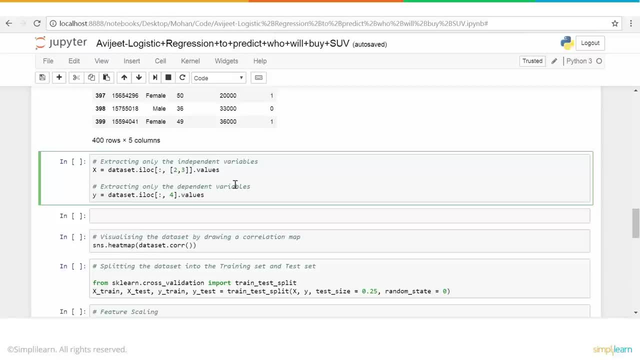 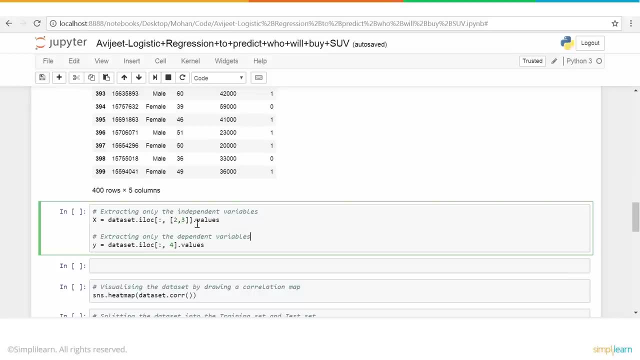 And what we are doing here is we are taking the second and the third column. we are taking these three right, So gender, age and estimated salary. So that is what we are taking here, Two up to three, And then y is basically the last column, which is the fourth column. 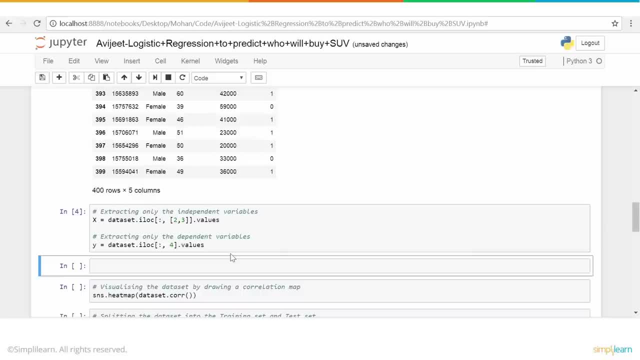 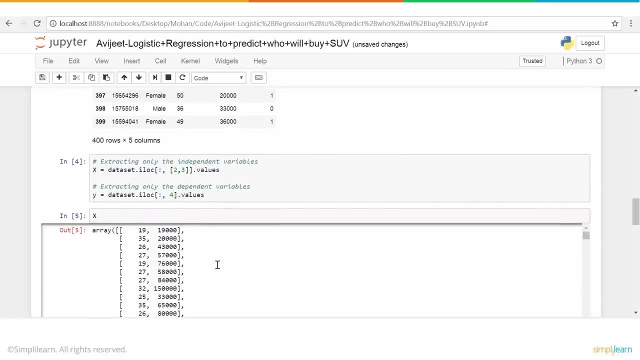 So let's go ahead and extract that. And, once again, why don't we take a look at how the data is looking? So let me just print x. So we only- yeah, we are basically taking two and three. So what is two and three? two and three is our age and our estimated salary. 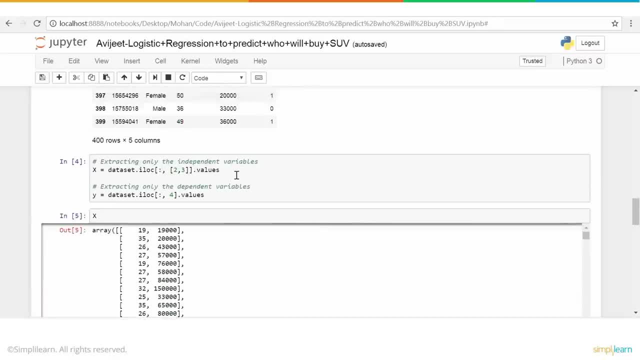 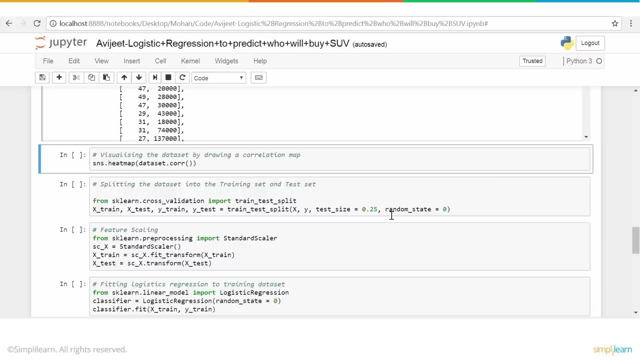 Yeah, that's right. So these are the only two independent variables, And our dependent variable is obviously our age. Okay, Okay, Okay, So we have the data loaded Now. let's, now that we have the data in Python, let's take a quick look at how the data looks. 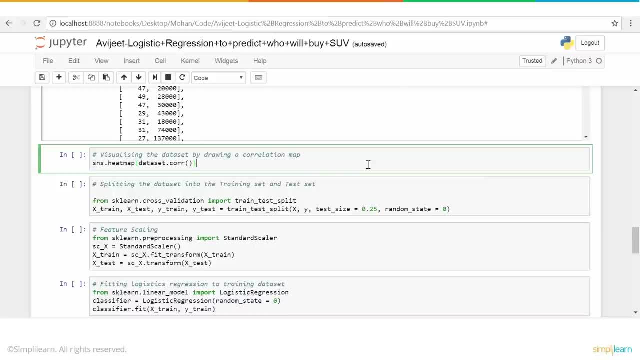 So, in terms of visualization, let's visualize the data and perform a little bit of what is known as exploratory analysis, right? So, as a data scientist, whenever you get new data, you just play around and see how the data is looking before you actually launch into the actual training or the model. 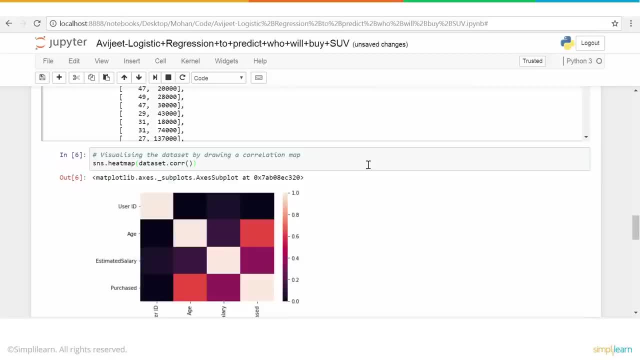 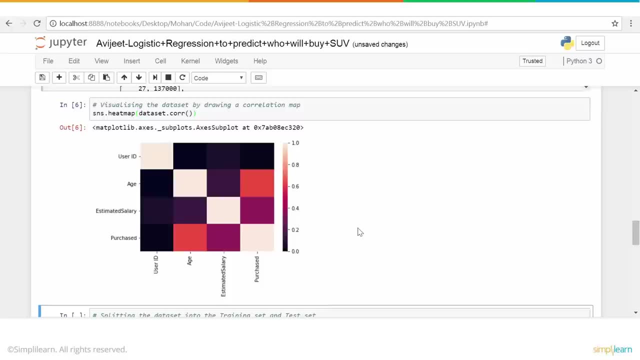 So that's the modeling part of it. So let's run a small heat map and see how the data looks. So we have just passed the entire data set here and this is how the heat map looks: how, how they are related, how the various- what do you call- features are related to each other. 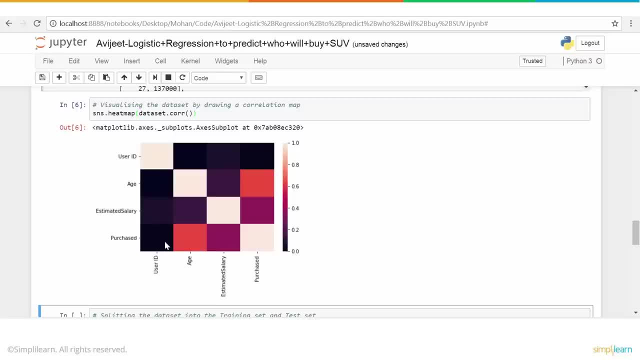 And this is a scale here. Very dark means basically there is a pretty much no, no correlation- This is in a way to measure the correlation as well- And light means there is a very high correlation. So, as you can see, A value or a feature will have very high correlation of one to itself. 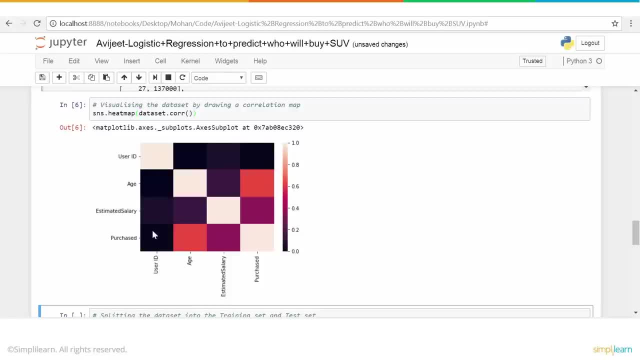 So the user ID- and this is user ID- It has a very high correlation to itself, Similarly purchased and purchased data, So the diagonal will be very high. So that is really not relevant. but then the other values is what we have to see. 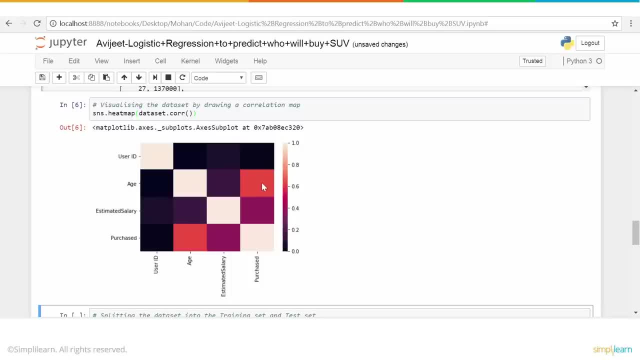 For example, there is a correlation of 0.6 in this area, which is basically, if you take age and purchased right, whether the person has purchased and the age. So that's, that's a quick look at it, Exploring the data. 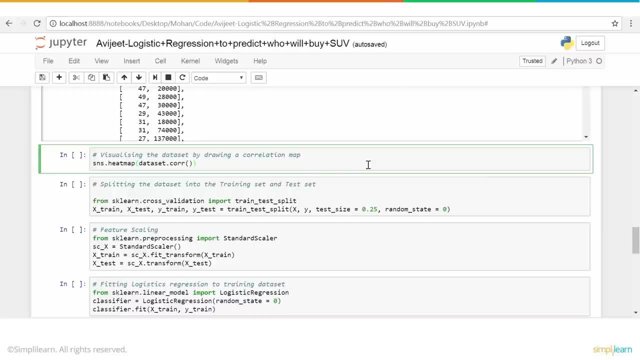 how the data looks. so, in terms of visualization, let's visualize the data and perform a little bit of what is known as exploratory analysis, right? so, as a data scientist, whenever you get new data, you just play around and see how the data is looking before you actually launch into the. 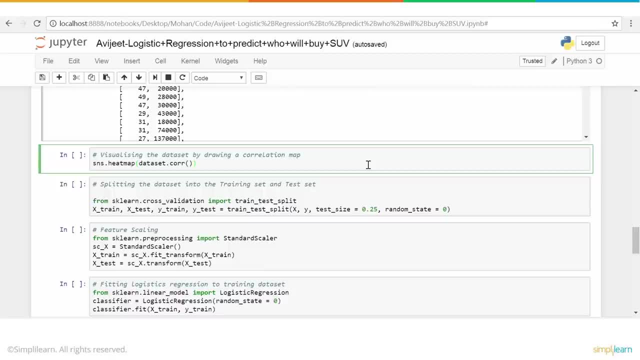 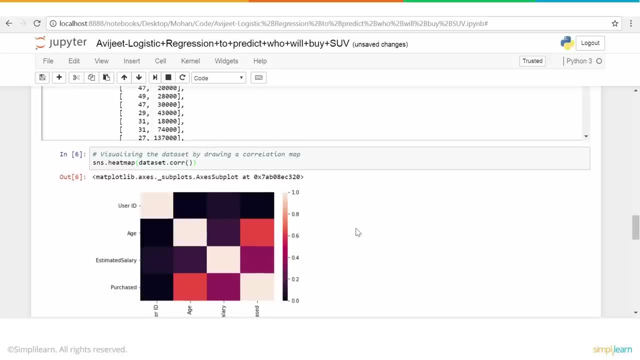 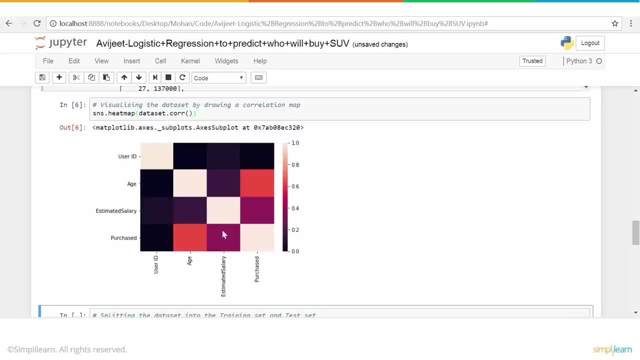 actual training or the modeling part of it. so let's run a small heat map and see how the data looks. so we have just passed the entire data set here and this is how the heat map looks: how, how they are related, how the various what you call features are related to each other, and this is a scale here very dark. 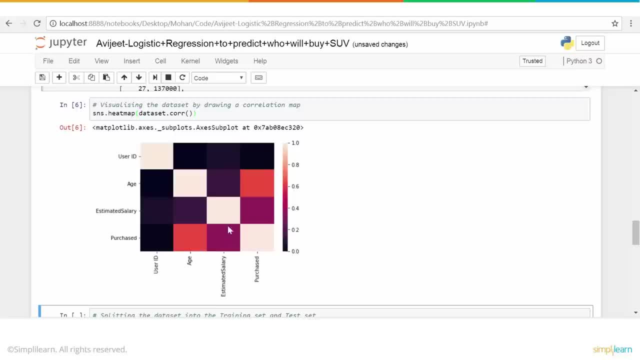 means basically there is a pretty much no, no correlation. this is in a way to measure the correlation as well, and light means there is a very high correlation. so, as you can see, a value or a feature will have very high correlation of one to itself. so the user ID- and this is user ID- it has a very high correlation to itself, similarly purchased. 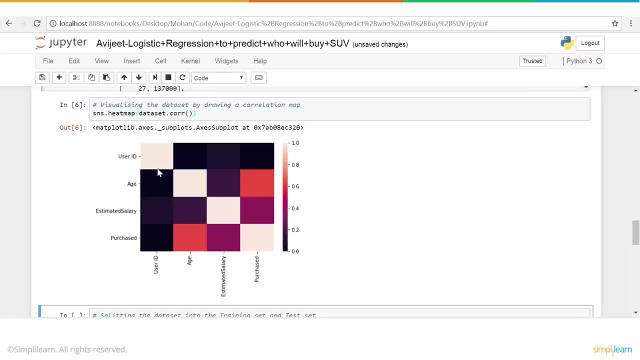 and purchased it has, so the diagonal will be very high. so that is really not relevant. but then the other values is what we have to see. for example, there is a correlation of 0.6 in this area, which is basically, if you take age and purchased right, whether the person has purchased and the age. 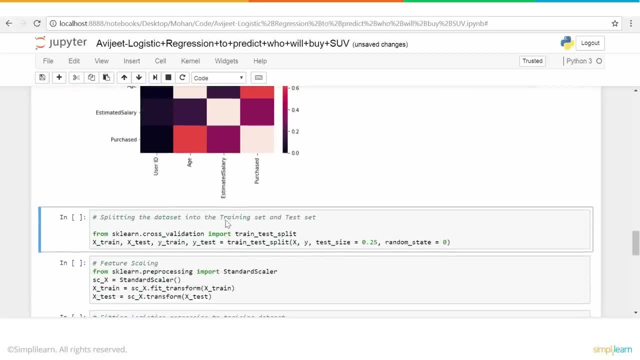 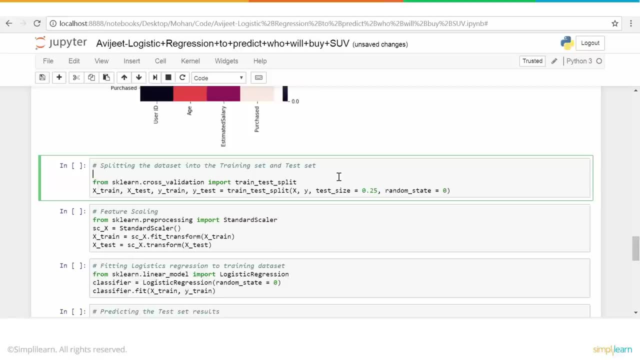 so that's a quick look at exploring the data. so that's all we are doing here. here's where the actual- uh, the crux of this code is. so, from here on, what's what we do is the first step before we start the training process is split our data into train and test: training data set and test data set. 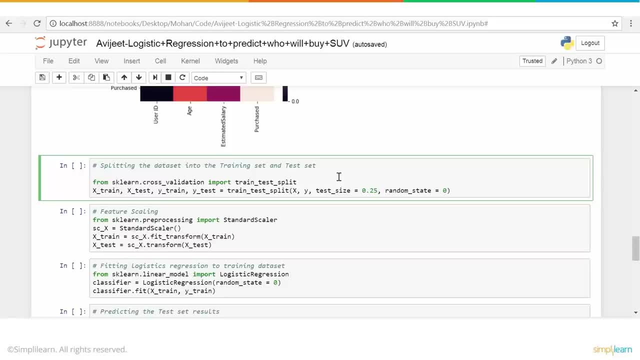 so whenever we perform any machine learning activity, we have, let's say, our label data. we never pass the entire data to the model, because then we are, then when we are measuring the accuracy, whether the model is performing well or not. we will not be able to do that if we use up the entire data for training purpose, so we split. 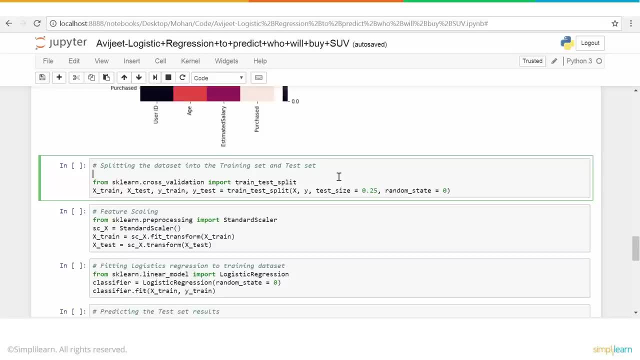 the data into what is known as a training data set. we train the model with the training data set and then this test data set, which is kept separately, which the model has not yet seen. we use that to check whether it is able to identify, perform the predictions correctly or not. okay, that will give. 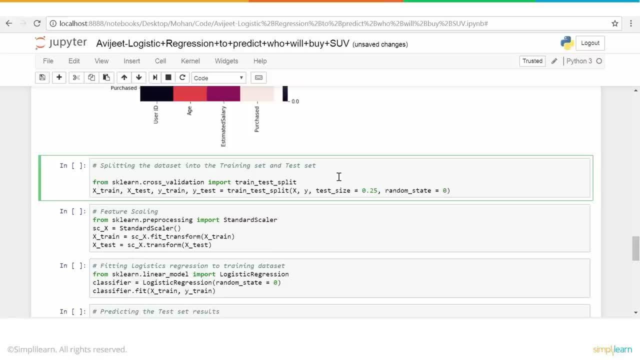 So that's all we are doing here. Here's where the actual, the, the crux of this code is. So, from here on, what's what we do is the first step, before we start the training process is split our data into train and test, training data set and test data set. 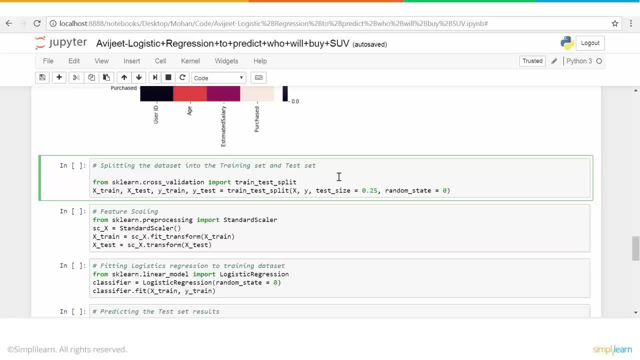 So, whenever we perform any machine learning activity, we have, let's say, our label data. We never pass the entire data to the model, Because when we are, then When we are Measuring the accuracy, whether the model is performing well or not, we will not be. 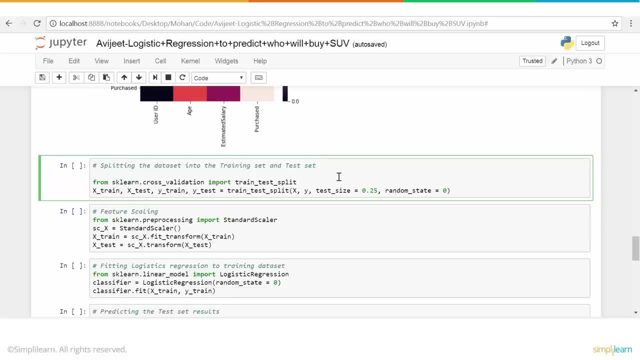 able to do that If we use up the entire data for training purpose. So we split the data into what is known as a training data set, We train the model with the training data set and then this test data set, which is kept separately, which the model has not yet seen. 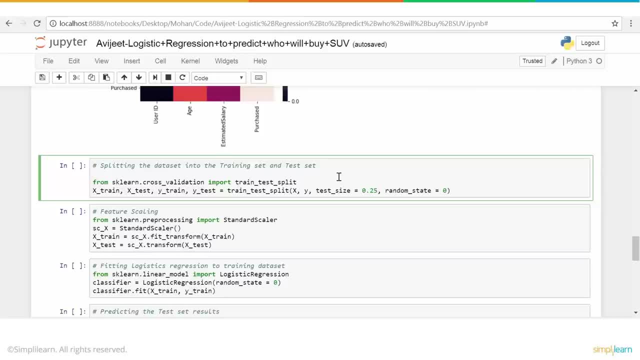 We use that to check whether it is able to identify, perform the predictions correctly or not. Okay, That will give us a higher accuracy Or or a better estimate of how the model is doing. All right, So this is a very common practice in machine learning. 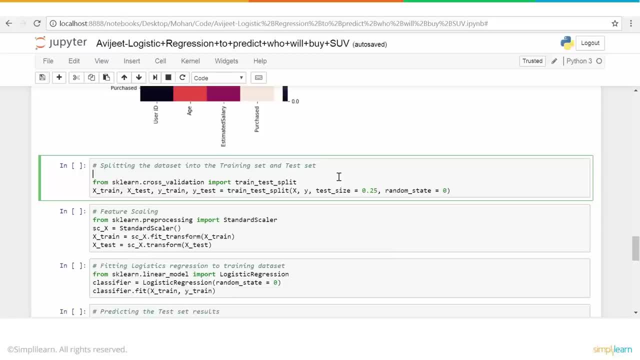 So, whenever we have, whenever we perform training of the model, we split the data into training and test it. Now, how do we do this? We don't have to write any special code. There is already a method available which is train underscore, test, underscore split. 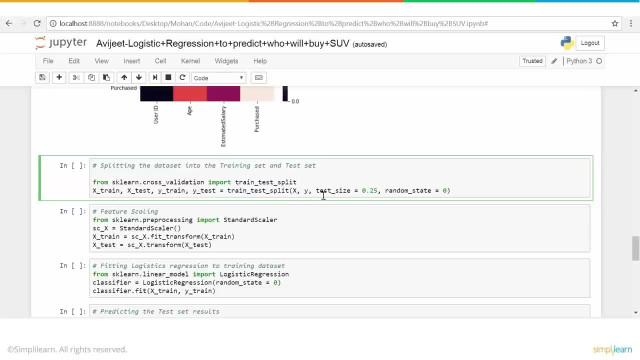 And we just call this method. Only thing is it takes these parameters and we have to specify especially this parameter which tells the, The Method How the data should be split. Now, when we are splitting the data into training and test, there are no hard and fast rules. 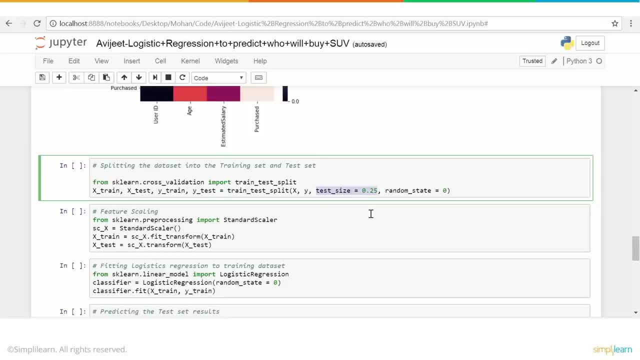 how we split this data. Some people prefer 50, 50,, some people prefer 80, 20, and so on and so forth. So that is flexible and it could be, to some extent, individual preferences. So in our case, we are splitting this data into 75, 25, which means 75% of the data we 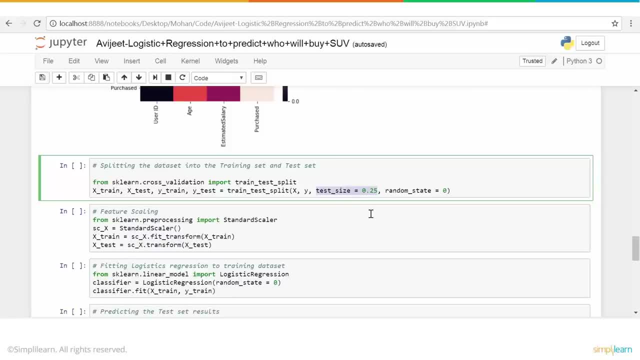 will use for training, 25% we'll use for test. So that is what we are specifying here. as a parameter, We say test underscore size is equal to 0.25.. That means put or keep 25% of the data, set aside, 25% of the data as test data and therefore 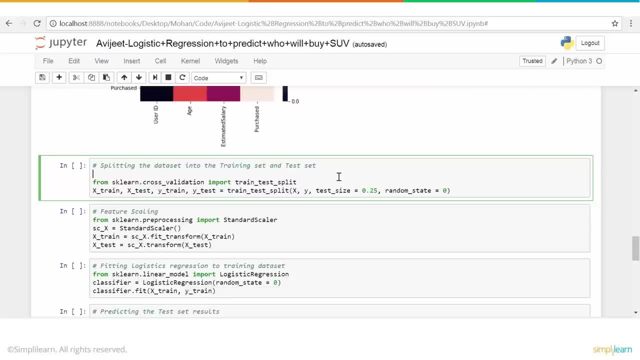 us a higher accuracy or or a better estimate of how the model is doing. all right, so this is a very common practice in machine learning. so whenever we have, whenever we perform training of the model, we split the data into training and test it. now, how do we do this? we don't have to write any special code. there is. 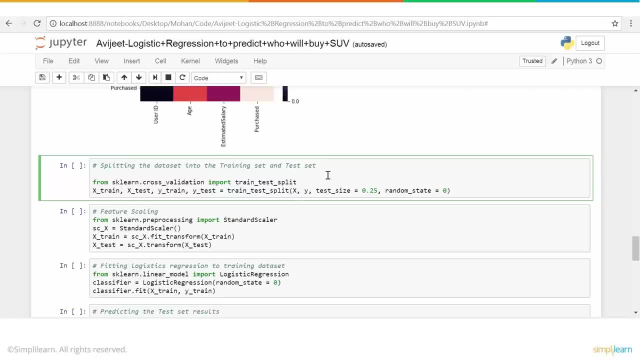 already a method available which is strain underscore, test, underscore, split, and we just call this method. only thing is it takes these parameters and we have to specify especially this parameter which tells the the method how the data should be split. now, when we are splitting the data into training and test there, 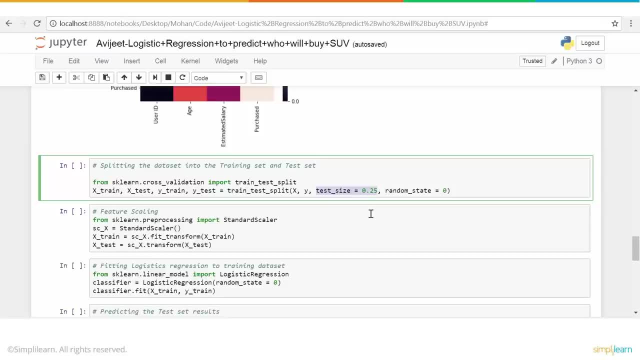 are no hard and fast rules how we split this data. some people prefer 50- 50, some people prefer 80, 20 and so on and so forth. so that is flexible and it could be to some extent, individual preferences. so in our case, we are splitting this data into 75- 25, which means 75 percent of the data will we will. 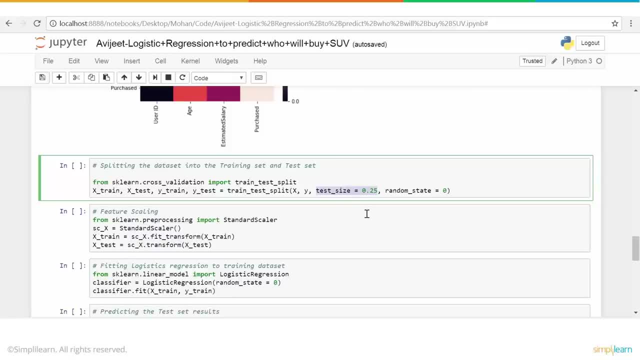 use for training. 25 percent we'll use for test. so that is what we are specifying here. as a parameter, we say test underscore size is equal to 0.25. that means put or keep uh 25 percent of the data set aside, 25 of the data as test data and therefore the remaining 75 percent will be used for training. 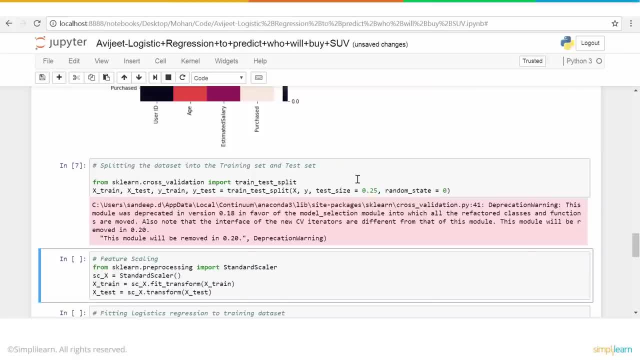 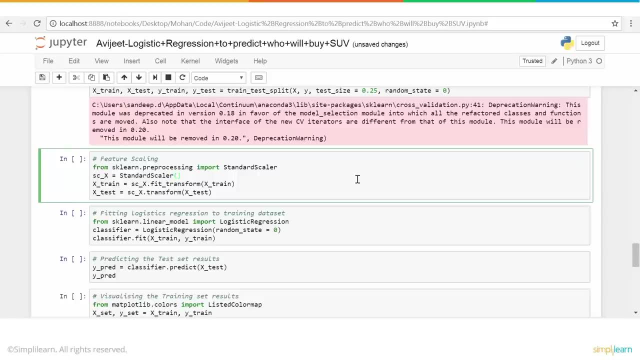 all right, so let's move on. I execute this, then we perform what is known as feature scaling. so what is feature scaling? usually what happens is, uh, the, the values that we have in the data. sometimes they numbers will be very large, some will be very small, so there is a huge variation. so, in order to, if we 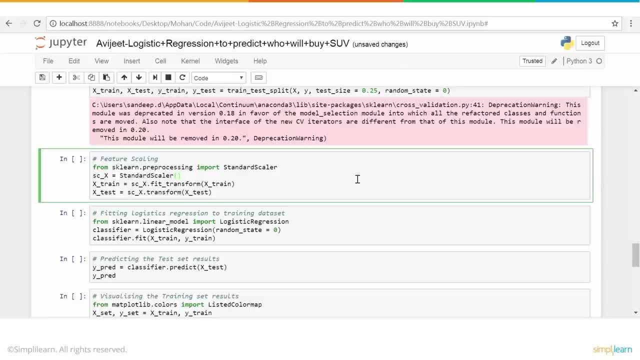 have that, and if we use that as it is, the accuracy of our model may come down. so we have to somehow normalize these values. so that is what scaling does- feature scaling does- and again, we don't have to write any special code for this. there is a standard method available or standard class. 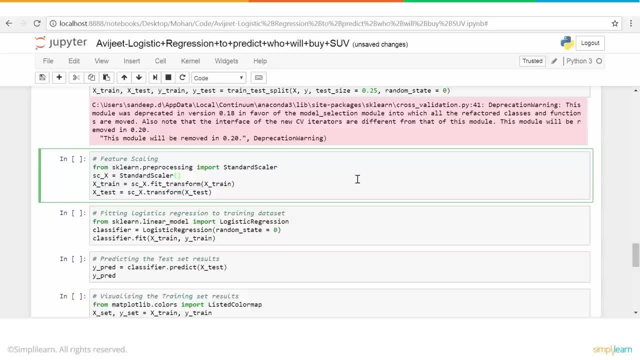 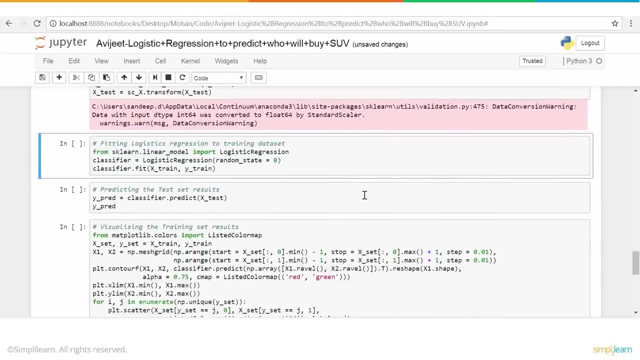 available, called standard scalar. let's create an instance of that and pass our data for scaling purpose. okay, so let's go ahead and do that now. so this is all. what we have done is more like a data preparation. so we: we chose what are the parameters, what features we want, we did the feature scaling and we split the data. now 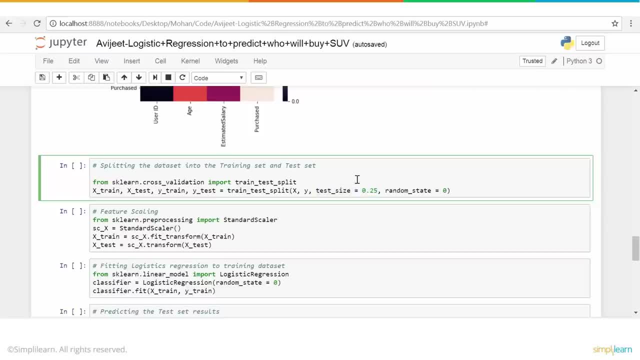 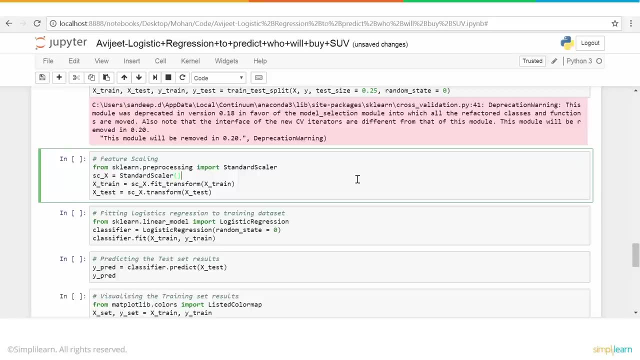 the remaining 70% will be used for training. All right, so let's move on. I execute this. Then we perform what is known as feature scaling. So what is feature scaling? Usually, what happens is the values that we have in the data. 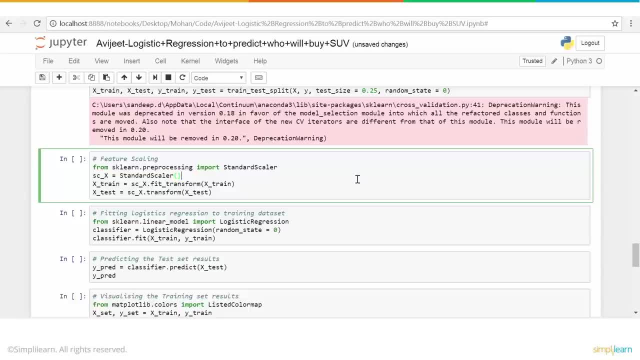 Sometimes they can be. Uh, Some numbers will be very large, some will be very small, So there is a huge variation. So, in order to if we have that and if we use that as it is, the accuracy of our model may come down. 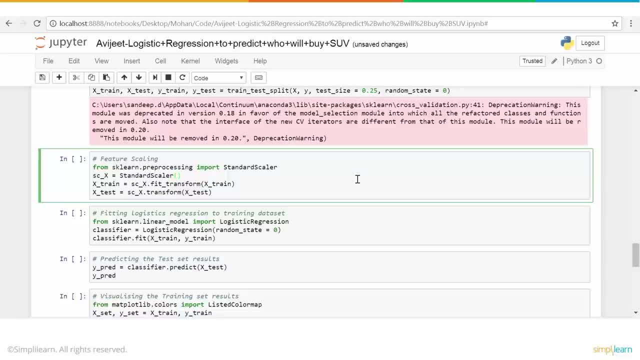 So we have to somehow normalize these values. So that is what scaling does, feature scaling does, And again, we don't have to write any special code for this. There is a standard method available or standard class available, called standard scale up. So we just create an instance of that and pass our data for scaling purpose. 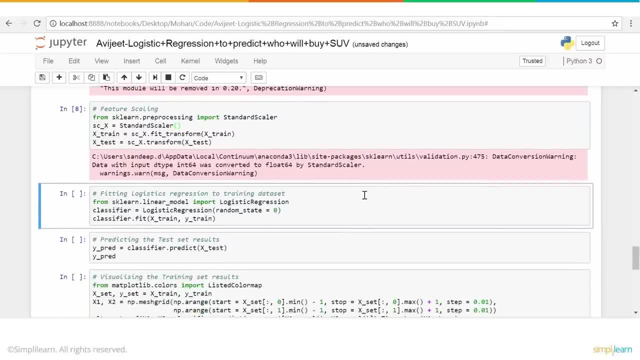 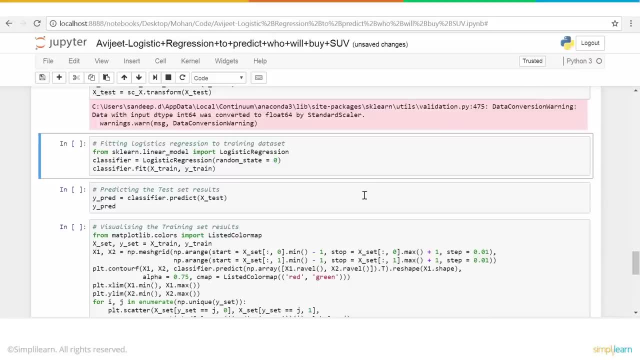 Okay, so let's go ahead and do that now. So this is all. what we have done is more like a data preparation. So we chose what are the parameters, what features we want, We did the feature scaling and we split the data. 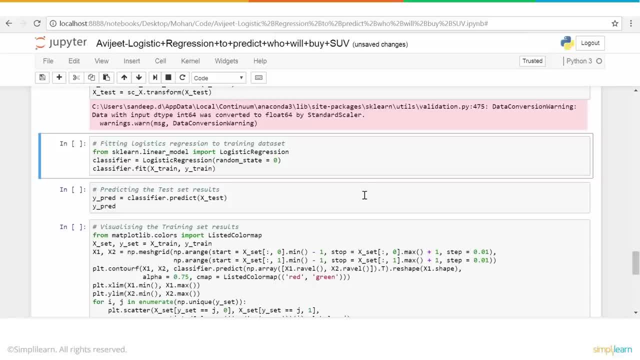 Now everything is ready. Next is to start the actual training process. So this is the most crucial part of the core. So here, as we said, we will use the Logistic Regression model. So we have to create a code, create, we create an instance of regression model. So I call that as classifier. you can give any. 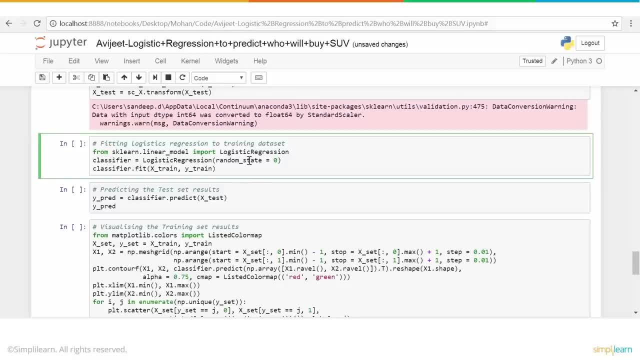 name And we just do some kind of initialization, random value initialization. So we call this as random state or we assign it as random state is equal to zero And we have an instance of the logistic regression model And we use that model, the fit method. So any, any algorithm that 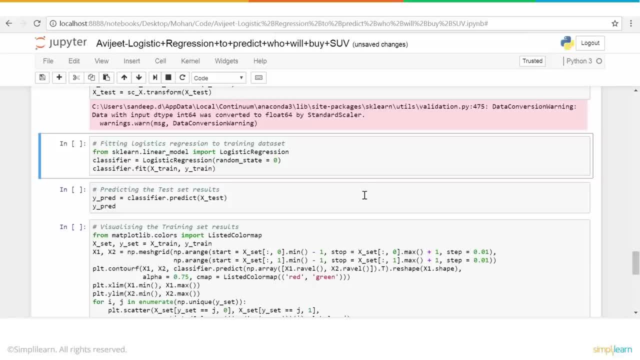 everything is ready. next is to to start the actual training process. so this is the most crucial part of the code. so here, as we said, we will use the logistic regression model. so we have to create, create an instance of regression model. so I call that as classifier. you can give any name and we 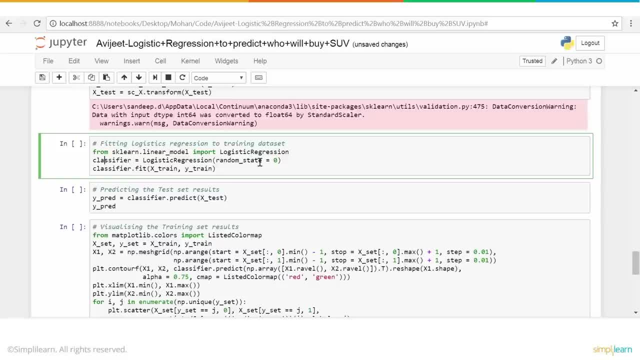 just do some kind of initialization, random value initialization. so we we call this as a random state or we assign it as random state- is equal to zero and we we have an instance of the logistic regression model and we use that model, the fit method. so any, any algorithm that we have when we 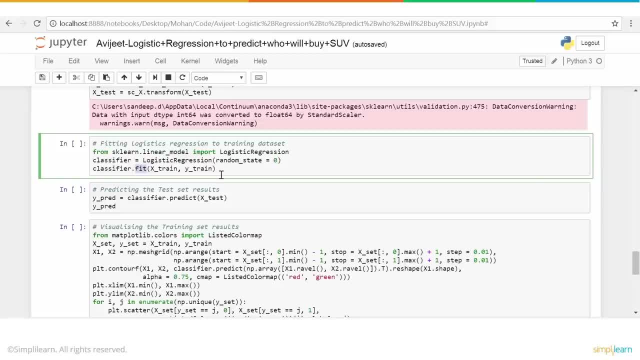 want to perform the training, we have to use the fit method. okay, we call the fit method. now, let's say, instead of logistic regression, we are using K. uh, okay, nearest neighbor's algorithm. you will have k nearest Neighborfit, or Linear Regression, linear regressionfit, right. so that is where. that is the way. 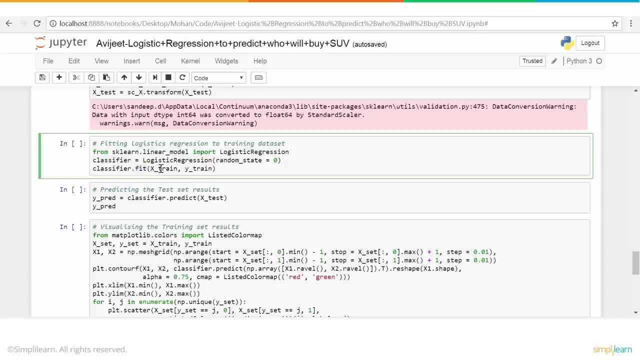 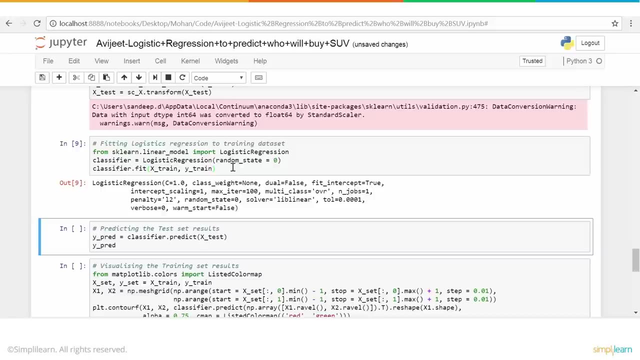 it works and we pass the training data set- the X is the independent variable- and via the labels, so pass both of them for the training purpose. So once the training is done, we get the results of: or the model is trained. Okay, the model is trained. Now the next step is to test the model. 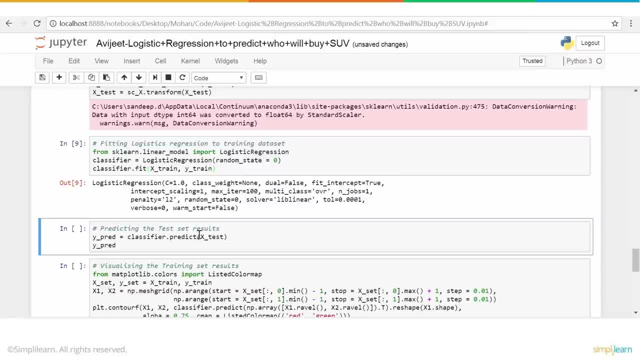 how well the model is performing. This is where we use the test data set. we pass the test test data set, And here there is a another method that we have to use that is known as a predict method. So, again, this is a predict method. is common across all algorithms that we have, So any 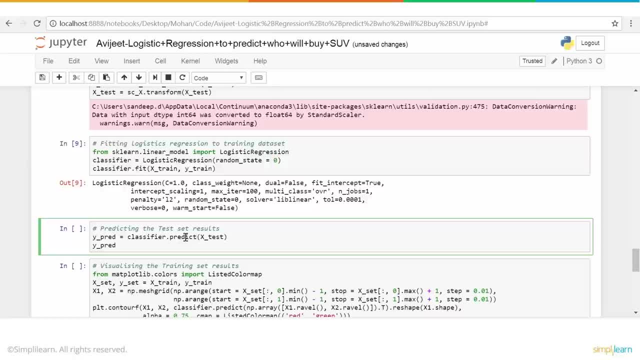 algorithm we have. we have to call the predict method for performing the test or even when we deploy it when new data comes in. we are trying to predict for new data set. we always use predict. Okay, so fit is only for the for training. Okay, then predict is used for testing and for the. 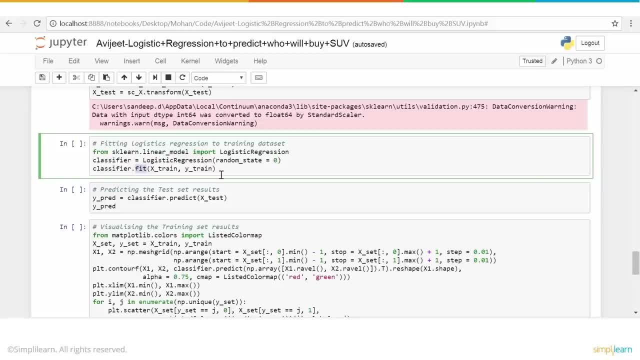 we have. when we want to perform the training, we have to use the fit method. Okay, we call the fit method. Now let's say, instead of logistic regression, we are using k, k nearest neighbors algorithm. you will have k nearest neighbor dot. fit or linear regression. linear regression dot. 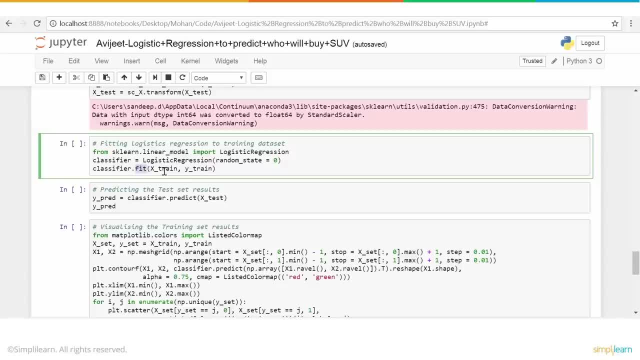 fit right. So that is where that is the way it works And we pass the training data set. the x is the independent variables and y are the labels, So we pass by both of them for the training purpose. So once the training is done we get the results of the. 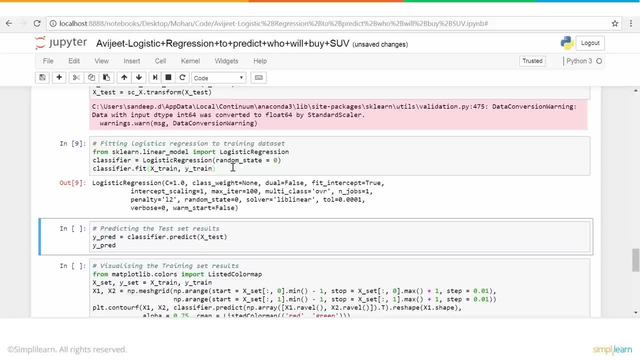 model is trained. Okay, the model is trained. Now the next step is to test the model, how well the model is performing. This is where we use the test data set. we pass the test test data set, And here there is a another method that we have to use, that is known as a predict method. So again, 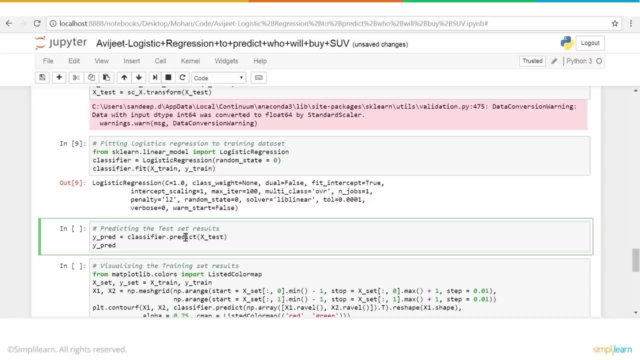 this is a predict method is common across all algorithms we have. So any algorithm we have, we have to call the predict method for performing the test or even when we deploy it when new data comes in. we are trying to predict for new data set. 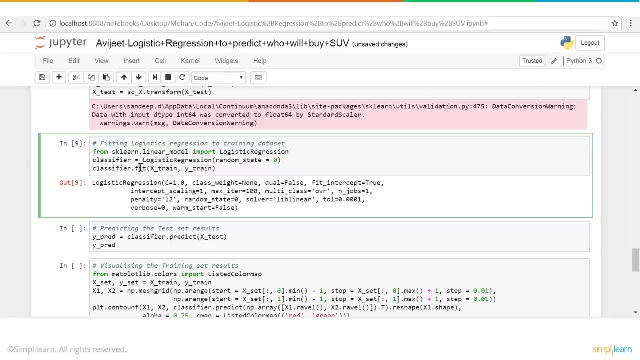 we always use predict- Okay, so fit is only for the for training. okay, then predict is used for testing and for the actual performance of the prediction. Now, one thing we need to observe here again is we only pass the x part of it and not the y part of it, So this can always some kind of a. 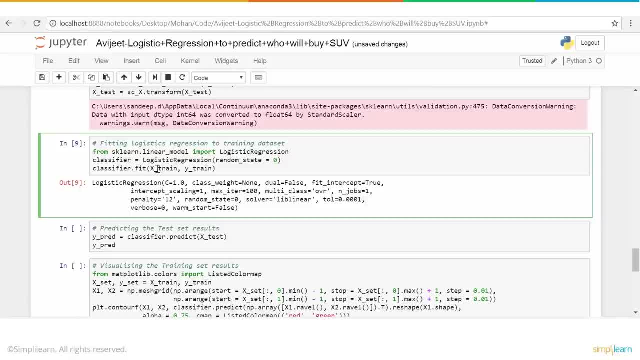 sometimes this can lead to confusion. in when we are calling fit, we are passing x and y. when we are calling predict, we are only calling x. The reason is the y part is what the model will predict. So you don't have to pass the y part, right? So y is what the model will predict for. 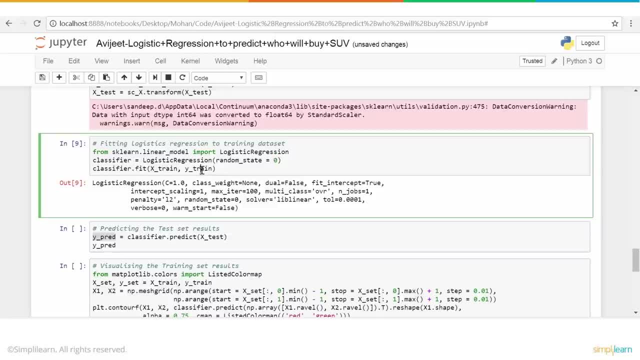 us, So you don't pass here. we had to pass it because the model has to learn from the existing values, So that's why we had to pass label as well. But when we are testing it, the model will calculate this And that's the reason why we have to pass the label as well. So that's why we have. 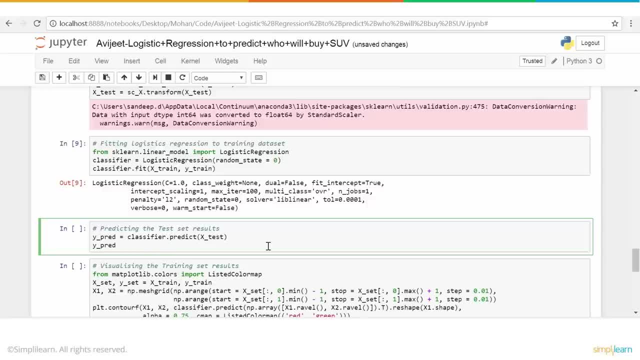 actual performance of the prediction. Now, one thing we need to observe here again is we only pass the x part of it and not the y part of it. So this can always. sometimes this can lead to confusion. in when we are calling fit, we are passing x and y. when we are calling predict. 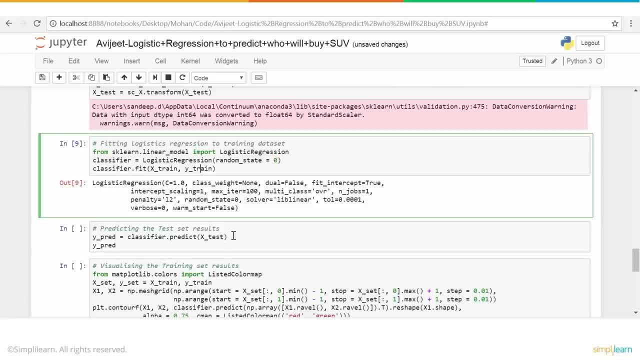 we are only calling x. The reason is the y part is what the model will predict, So you don't have to pass the y part, right? So y is what the model will predict for us, So you don't pass here we. 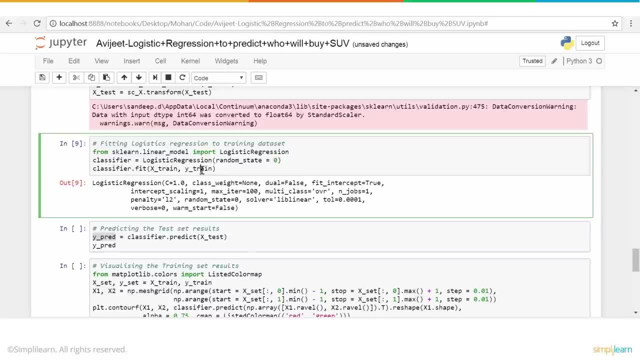 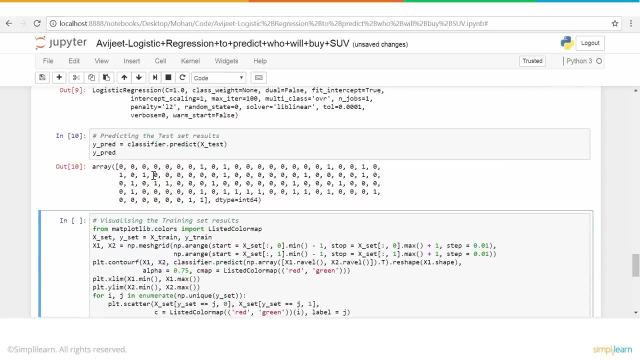 had to pass it because the model has to learn from the existing values. So that's why we had to pass label as well. But when we are testing it, the model will calculate this And that's the reason we do not pass the y value. Okay, so now when we run predict, it will calculate those values or find. 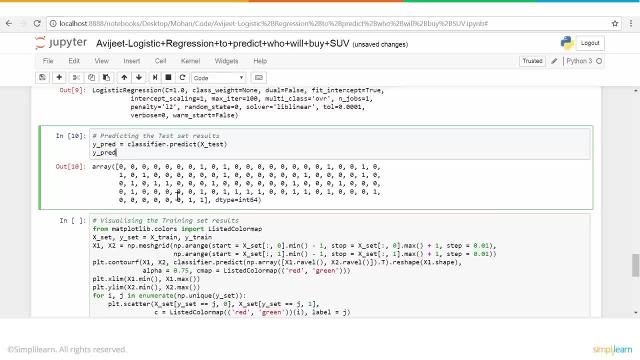 those values and it will put it in y underscore: predict. And that is what is being displayed here And, as you can see, the values can be either a zero or one, which means the person will buy the SUV, which means which is one widget which is a value of one, or zero means the person will. 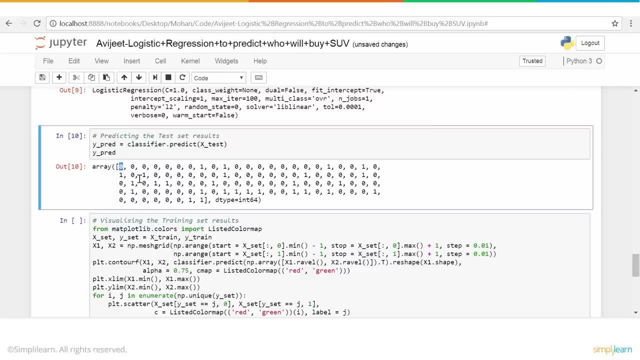 not buy the SUV. Okay now, one more thing we need to remember is, while we have not passed the y values or the labels to the system, but we have these labels available with us. right, y underscore test is available with us. That is what we have to use to find out how accurate the system is. So 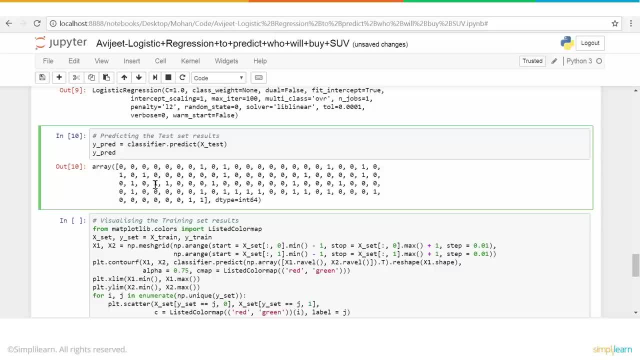 it has given us the results. Now we will compare these results, which the system has predicted, with the actual values that we have, which is available in y underscore test. So we will see how well, how that is done, how that accuracy is calculated in a little bit. Okay, now that the 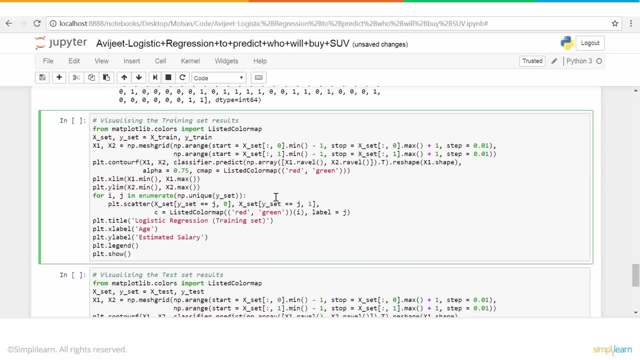 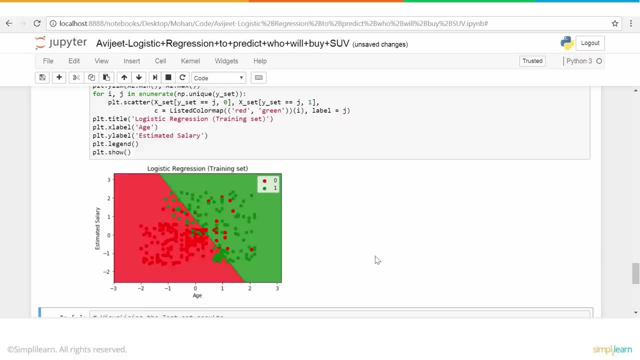 training is completed, we can go ahead and do some visualization of the training results. So let me execute this code and take a look in a form of a plot. So this is how the classification is done. So these are like the class. this is like the class boundary. the green color belongs to the 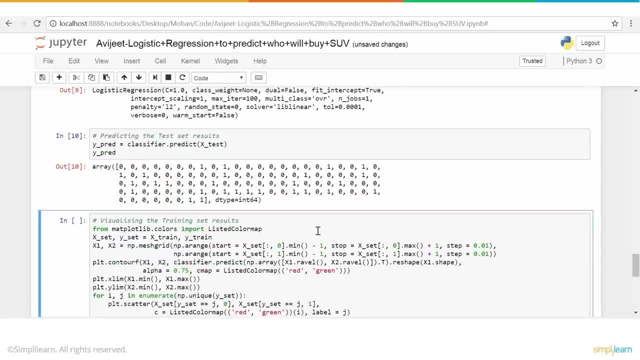 to pass label as well. So that's the reason why we have to pass label as well. So that's the reason we do not pass the y value. Okay, so now when we run predict, it will calculate those values or find those values, and it will put it in y underscore predict. And that is what is being. 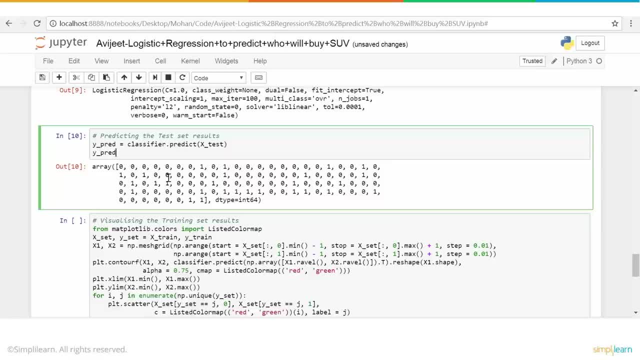 displayed here And, as you can see, the values can be either a zero or one, which means the person will buy the SUV, which means which is one, which is which is a value of one, or zero means the person will not buy the SUV. Okay now, one more thing we need to remember is, while we 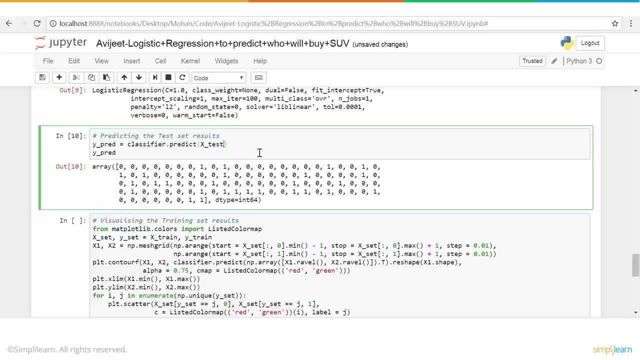 have not passed. the y values are the labels to the system, But we have these labels available with us. right y underscore test is available with us. That is what we have to use to find out how accurate the system is. So it has given us the results. Now we will compare these results. 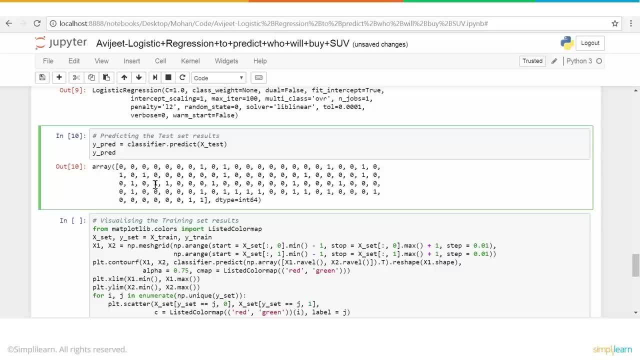 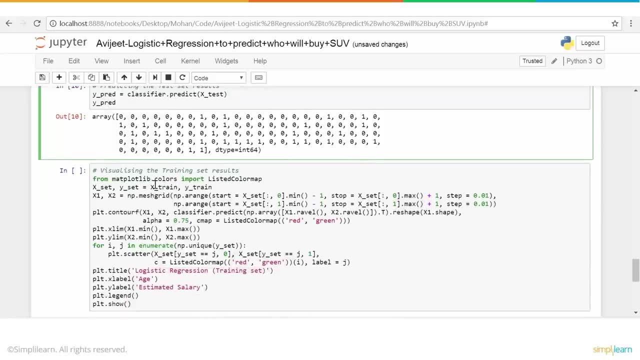 which the system has predicted with the actual values that we have, which is available in y underscore test. So we will see how well, how that is done, how that accuracy is calculated in a little bit. Okay, Now that the training is completed, we can go ahead and do some visualization of the 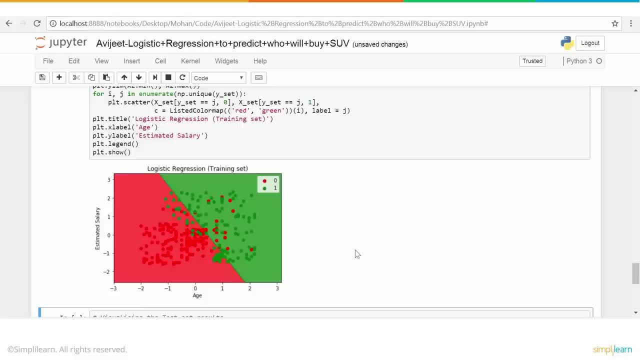 training results. So let me execute this code and take a look in a form of a plot. So this is how the classification is done. So these are like the class. This is like the class boundary: The green color belongs to the class one and the red color belongs to class zero. 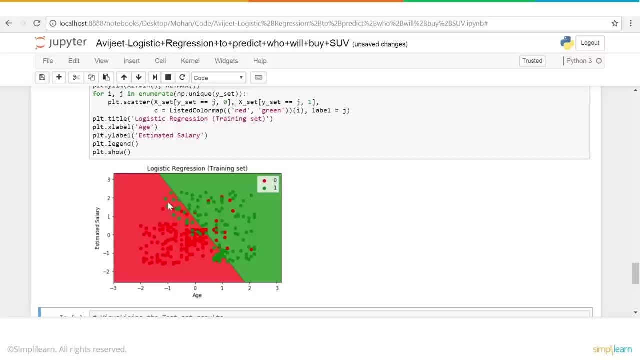 And these dots indicate it has been misclassified. So some of them have been misclassified. So that's what we are seeing: some red dots in the green area and some green dots in the red area right, Whereas if you probably it's not very clear, but you can see here that there are also red. 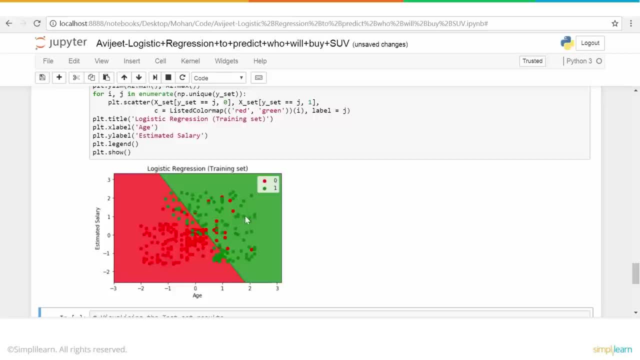 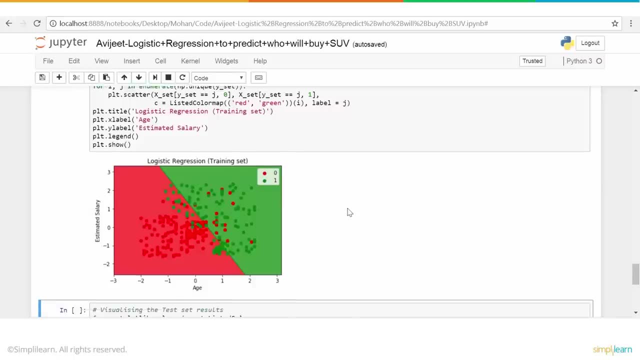 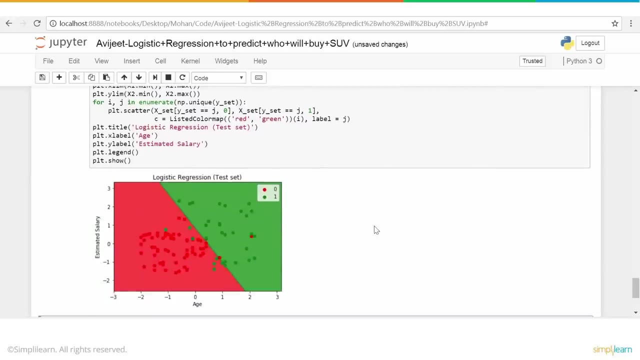 dots in the red area and the green dots in the green area. So those are the data points which are correctly predicted And these in the opposite locations are the ones that have been misclassified. rather Same for test as well. So test data set. also. if we visualize, we plot, we will see something similar. 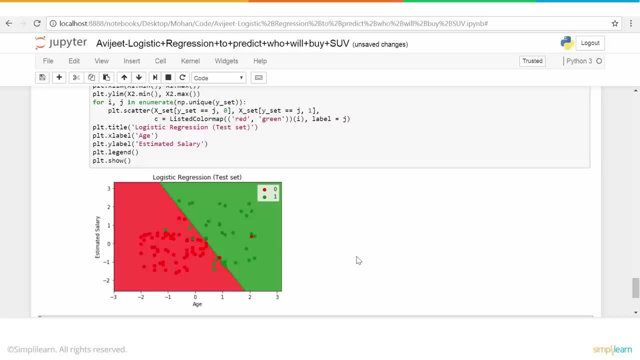 But this Also gives at a high level. whether is that a major in a major way. are there major misclassifications or there are only few? here and there, it gives a little bit of an idea about the accuracy as well, But then that is not sufficient for us, right. 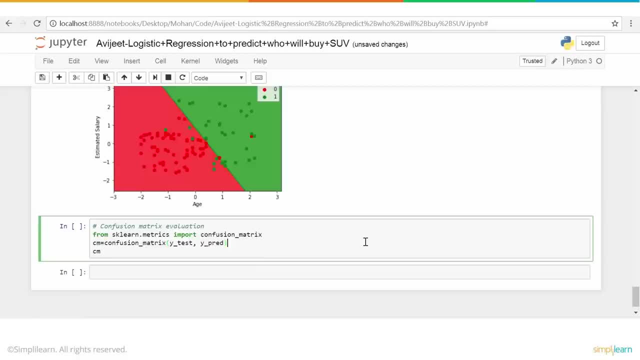 So we have to quantify this accuracy. So how do we do that? We do this using what is known as confusion matrix. So it's a readily available method or a class just there, And it takes two parameters, which is the you remember I told you we will be using. 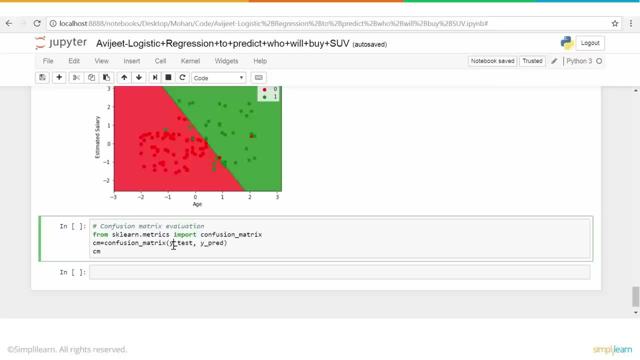 y test. So this is where we will be using y underscore test, which is our labeled value or labeled data set, And this is what is predicted by our model. Okay, y underscore pred is predicted are the predictions here. these are the values of: 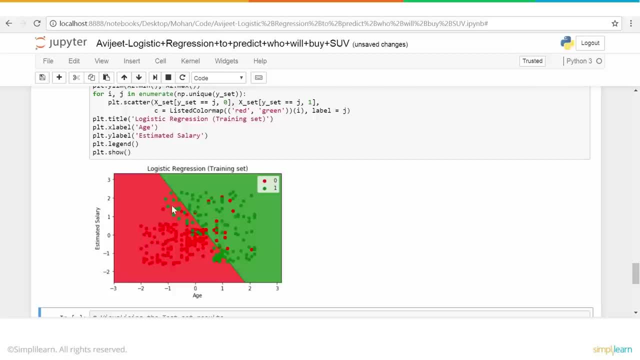 class one and the red color belongs to class zero And these dots indicate it has been done. So we can see that the class is done. So we can see that the class is done. So we can see that the class has been misclassified. So some of them have been misclassified, So that's. 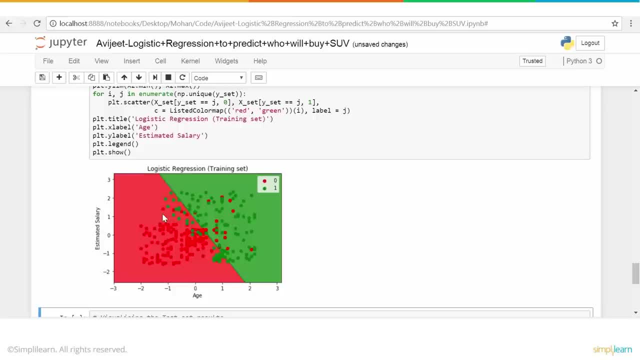 what we are seeing: some red dots in the green area and some green dots in the red area right, Whereas if you probably it's not very clear, but you can see here that there are also red dots in the red area and the green dots in the green area. So those are the data points which are correctly. 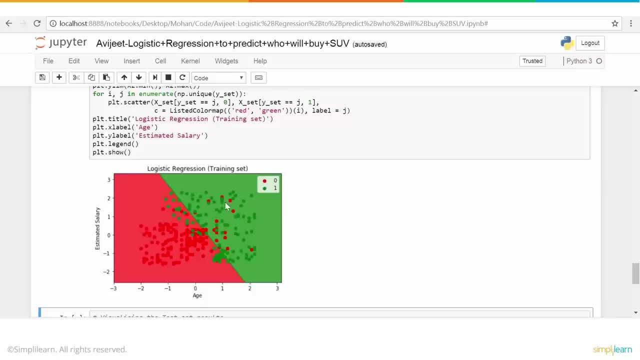 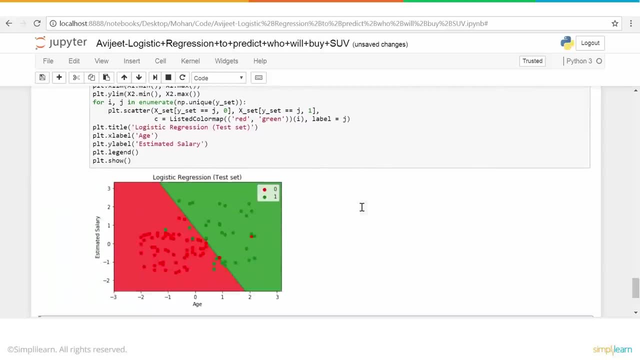 predicted And these in the opposite locations are the ones that have been misclassified. rather Same for test as well. So test data set also. if we visualize, we plot, we will see something similar, But this also gives at a high level. whether is that a major? 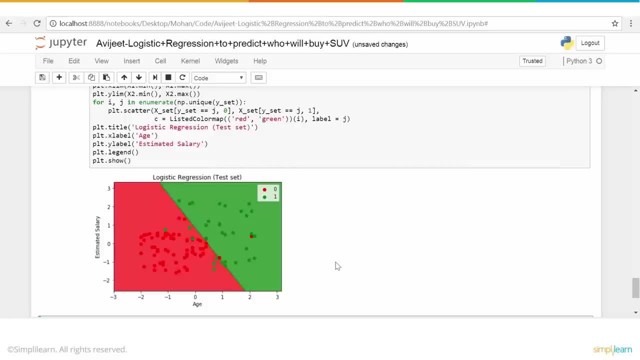 in a major way. are there major misclassifications, Or there are only few here and there? it gives a little bit of an idea about the accuracy as well, But then that is not sufficient for us, right? So we have to quantify this accuracy. So how do we do that? 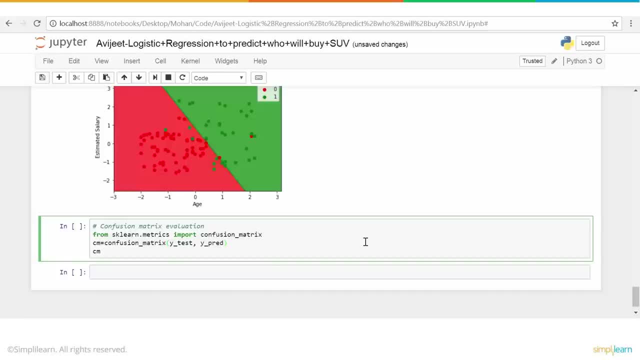 We do this using what is known as confusion matrix. it's a readily available method or a class which is there and it takes two parameters, which is the you remember i told you we will be using y test, so this is where we will be using y underscore test. 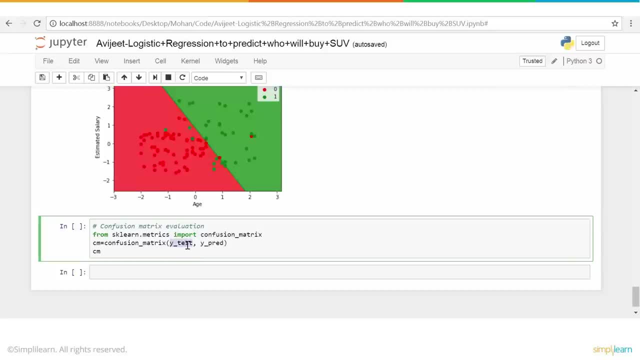 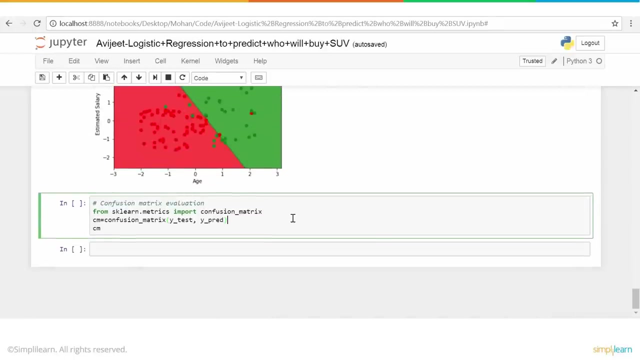 which is our labeled value or label data set, and this is what is predicted by our model. okay, y underscore pred is predicted. are the predictions. these are the values of here we saw this is y underscore pred. okay, so we we pass these two parameters and we create a matrix. and this matrix: 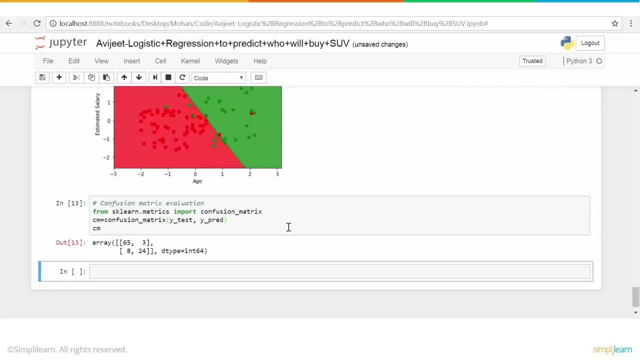 is known as confusion matrix. now, what is the significance of this? first thing is that the total number of values here is equal to the number of data sets in your test data. okay, so let's go ahead, and in the next cell, let me just add up these values: so 65 plus 3 plus 8 plus 24. 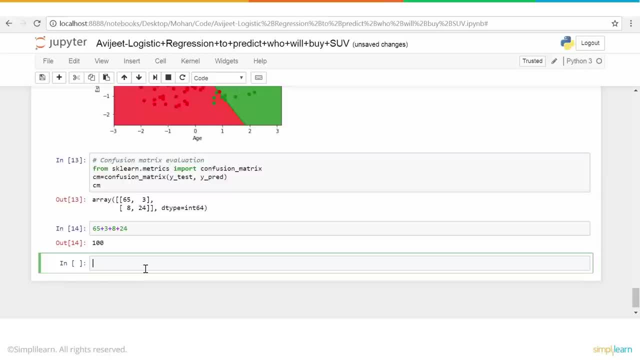 so how many are there? there are 100 in number, so there are totally 100 observations in your test data set. that is the first point. then the second point is the number in the diagonals, right, the total value in the diagonals. if that is a high, that indicates a higher accuracy, the higher that 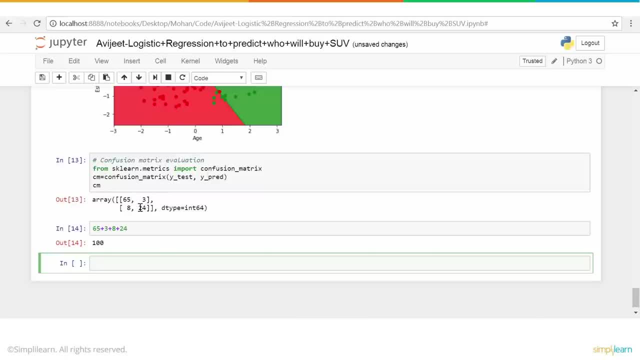 number is the total in the diagonal. the higher the accuracy. okay. and if we have quite a few numbers- non-diagonal locations, that means accuracy is not very high. so here looks like the accuracy is pretty good. now we can actually quantify the accuracy by using these numbers. so what we do is the sum along the diagonal. 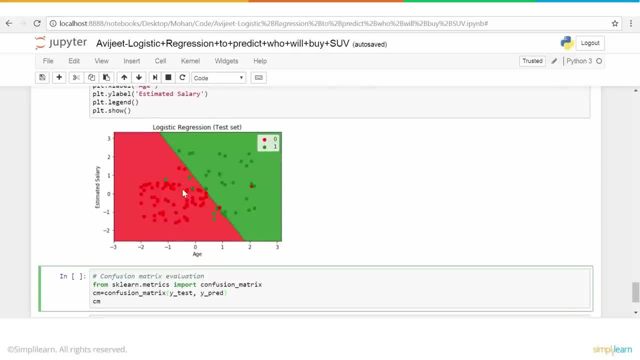 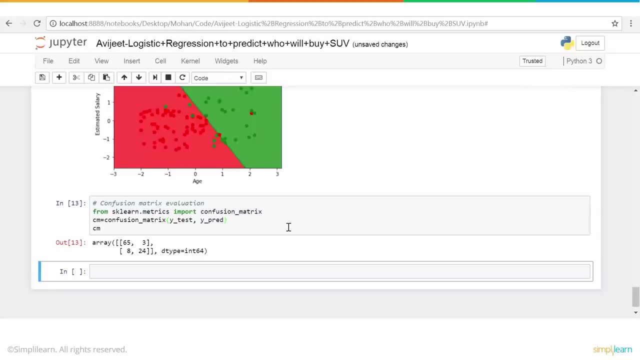 here we saw this is y underscore pred. okay, so we pass these two parameters and we create a matrix, And this matrix is known as confusion matrix. Now, what is the significance of this? first thing is that the total number of values here 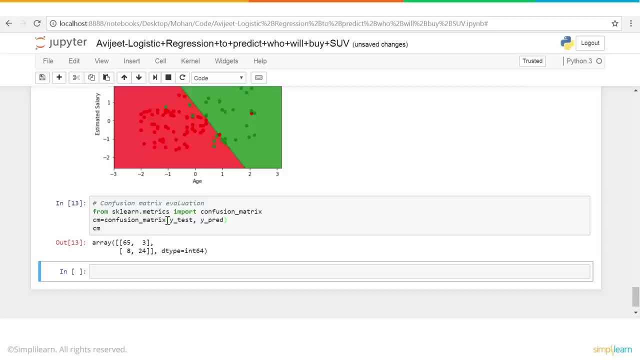 is equal to the number of data sets in your test data. Okay, so let's go ahead, and in the next cell, let me just add up these values: So 65 plus three plus eight plus 24.. So how many are there? 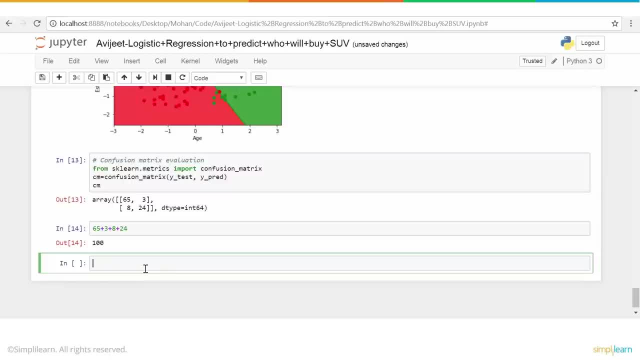 There are 100 in number. So there are totally 100 observations in your test data set. So let's go ahead. and in the next cell let me just add up these values: So 65 plus three plus eight plus 24.. So how many are there? 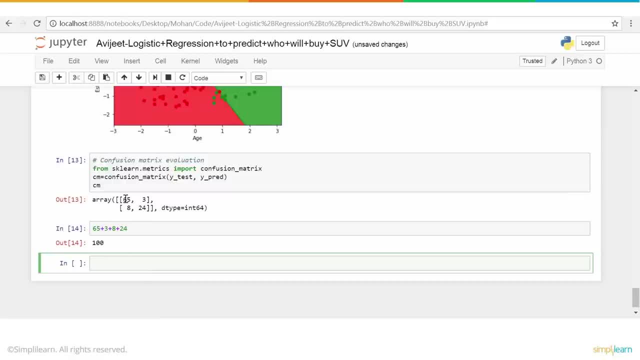 There are 100 observations in your test data set. That is the first point. Then the second point is the number in the diagonals right, the total value in the diagonals. if that is a high that indicates a higher accuracy, the higher that number is the total. 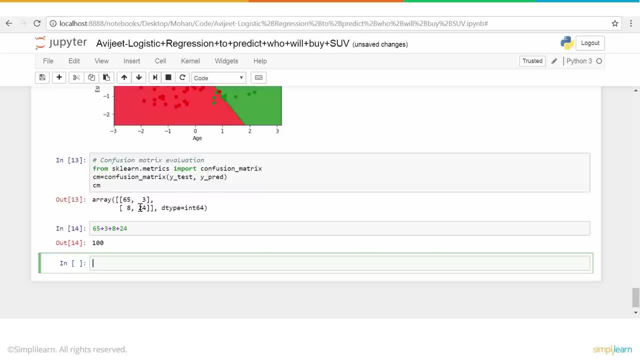 in the diagonal, the higher the accuracy. okay, And if we have quite a few numbers non diagonal locations, that means accuracy is not very high. So here looks like the accuracy is pretty good. Now we can actually quantify the accuracy by using these numbers. 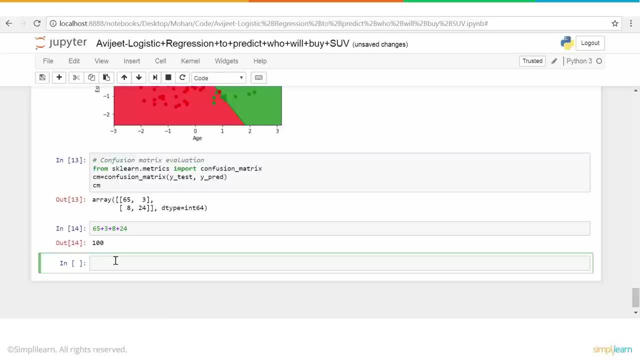 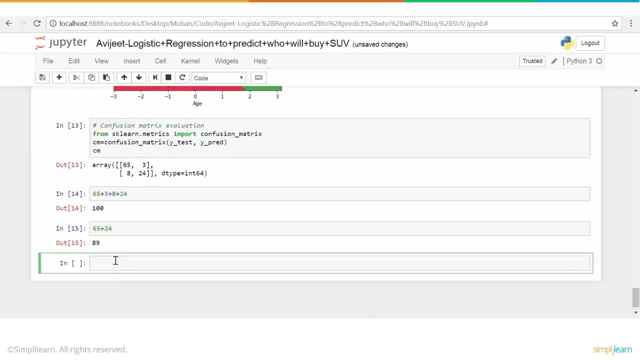 So what we do is the sum along the diagonal. we have to take and divide that by the total observation. So 65 plus 24 is what we have along the diagonal and we have 100 observations. So 89 by 100 is our percentage. 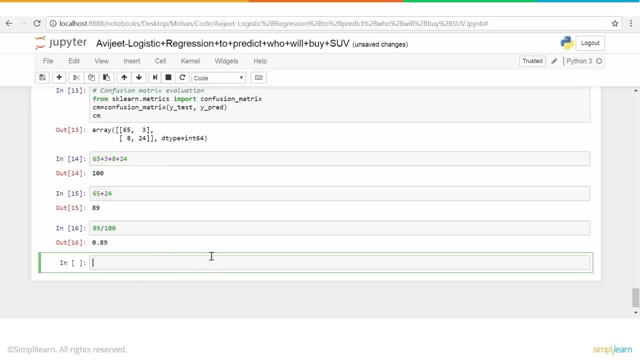 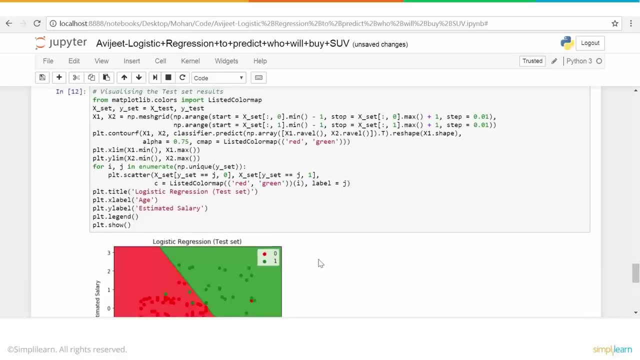 So we got about 90% accuracy for this particular model. Okay, so that brings us to the end of this demo. And we've come to the end of this demo. Thank you for watching. We will move on to the next demo. 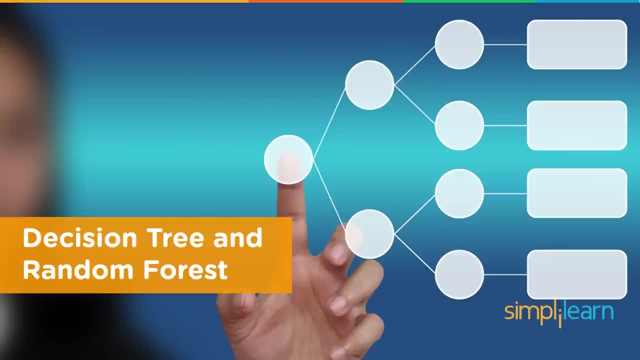 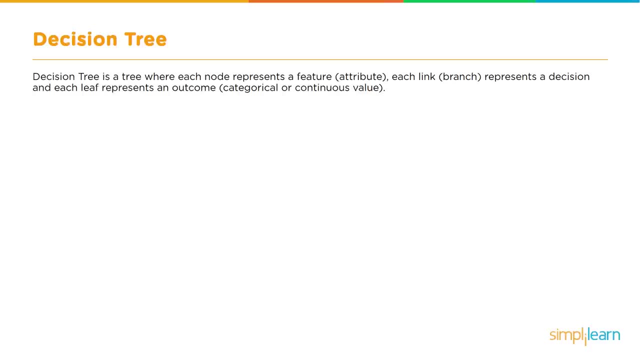 Alright, so the next algorithm is decision tree and random forest. they are being taken together because they are very closely related. So what is the decision tree? This is a tree, is another algorithm And, unlike logistic regression, which is only used for binary classification, decision tree 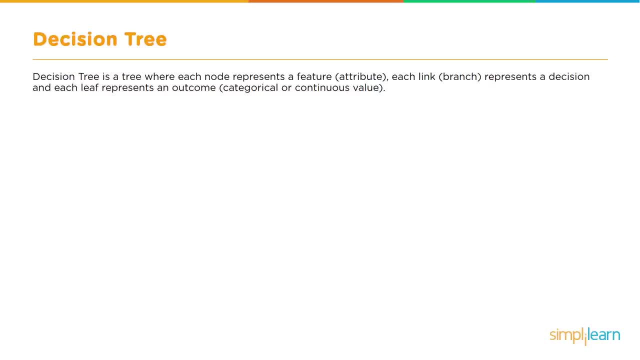 can be used for classification as well as regression- even though it is more popular for classification, And it can be used to classify multiple classes as well, not just binary classification. So how does decision tree work? One of the good things about decision trees is that it is easy to represent and show how. 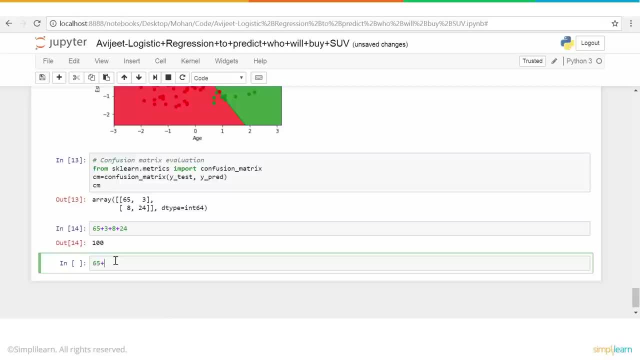 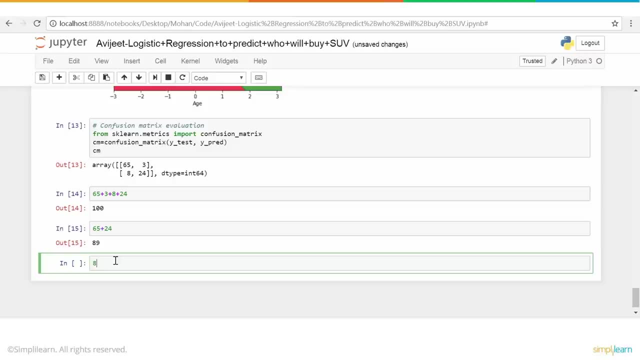 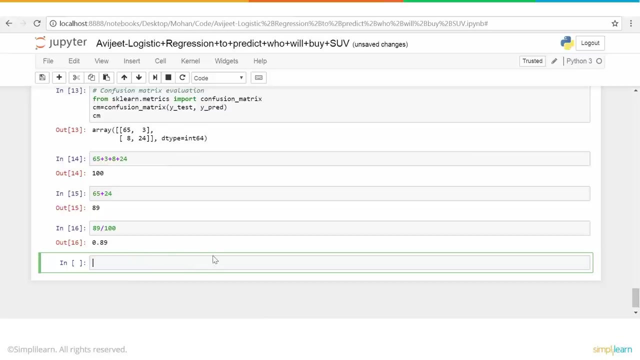 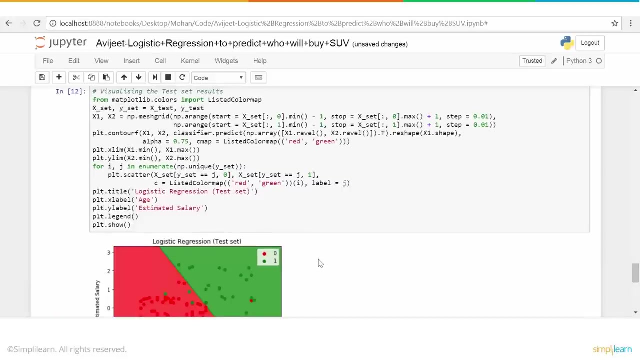 we have to take and divide that by the total observation. so 65 plus 24 is what we have along the diagonal and we have 100 observations, so 89 by 100 is our percentage. so we got about 90 accuracy for this particular model. okay, so that brings us to the end of this demo and, uh, we will move on to the next demo. 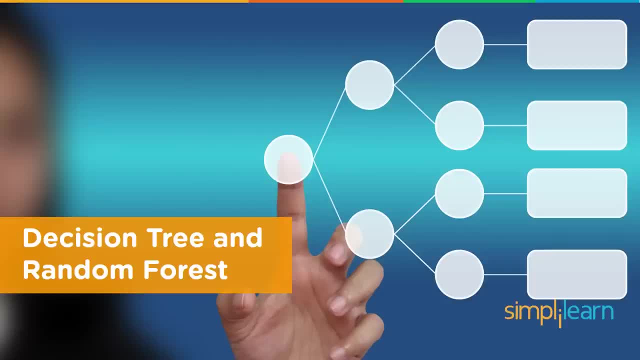 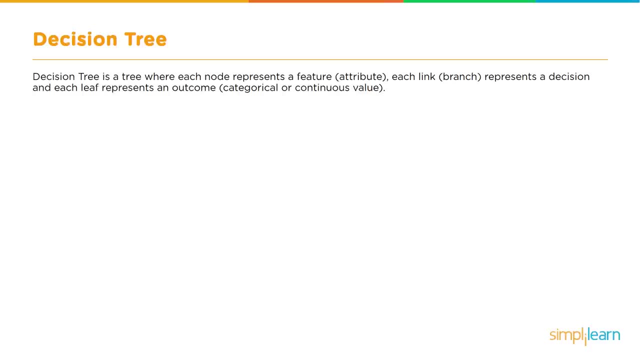 all right. so the next algorithm is decision tree and random forest. they are being taken together because they are very closely related. so what is a decision tree? decision tree is another algorithm and, unlike logistic regression, which is only used for binary classification, decision tree can be used for classification as well as regression, even though it is more popular for classification and 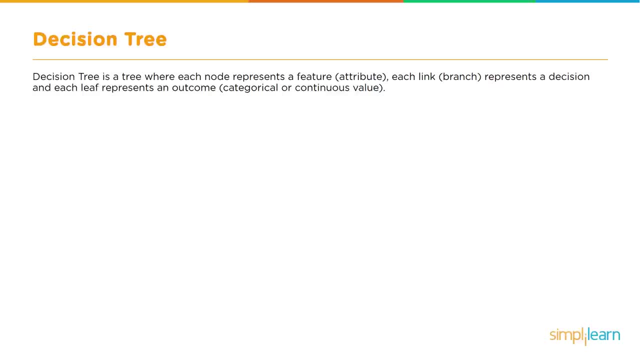 it can be used to classify multiple classes as well, not just binary classification. so how does decision tree work? one of the good things about decision trees is that it is easy to represent and show how exactly it works, and therefore it is very easy to understand as well. now let's 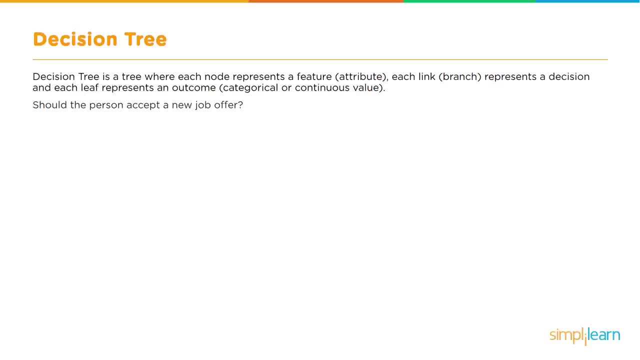 take an example. let's say a person receives a job offer and he needs to decide whether to accept the job offer or not. so we will use decision tree to come to the decision to accept or not to accept. so this is how, first of all, a decision tree looks. it is actually an inverted tree, so the root is at. 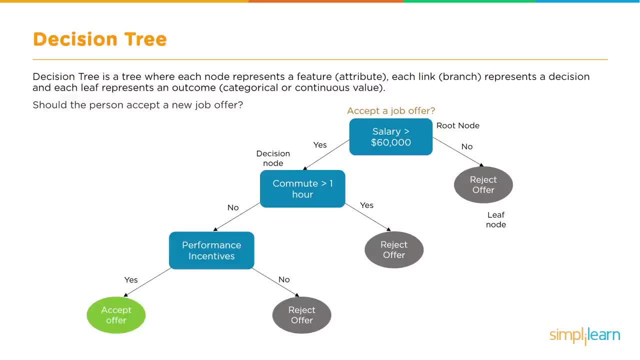 the top, okay so, and that is known as the root node. the node where the tree starts is known as the root node, and then we have the decision tree, where we start the decision tree, and then we have the some inner nodes or decision nodes, and we have the nodes where we have a decision, either positive or 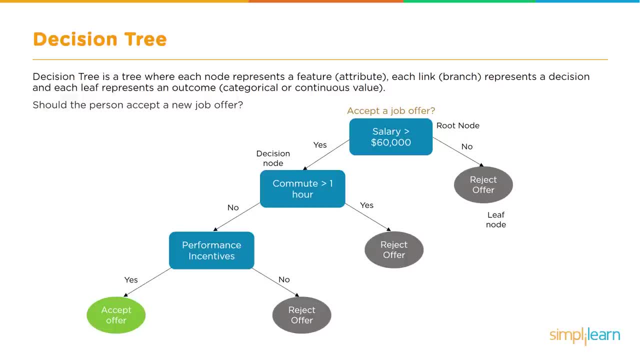 negative. these are known as leaf nodes or terminal nodes. okay, so we have the root node and we have leaf nodes or terminal nodes. there can be multiple of them and in between we have decision nodes or internal nodes. there are different terms used, so need not be hung up by the exact terminology now. 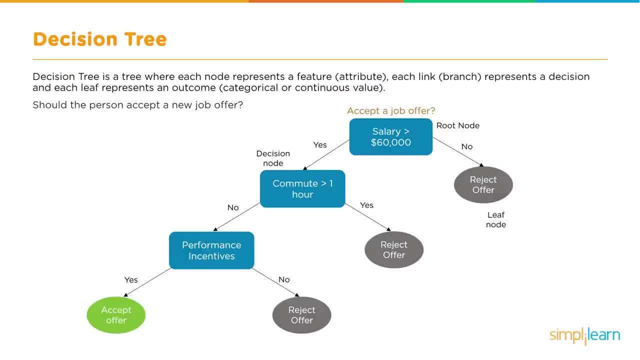 let's say, we have to use this decision tree to find out whether this person will accept the job offer or not. so first thing he considers is the salary. is the salary greater than sixty thousand? if no, it's a clear decision: the offer will be rejected. so we reach a decision. therefore, this: 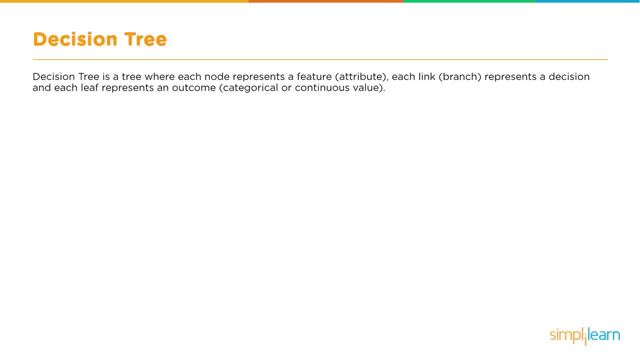 exactly it works And therefore it is very easy to understand as well. Now let's take an example. Let's say a person receives a job offer and he needs to decide whether to accept the job offer or not. So we will use decision tree to come to the decision. 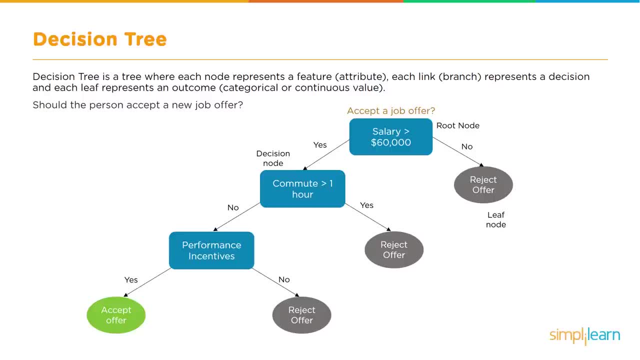 To accept or not. So this is how, first of all, a decision tree looks. it is actually an inverted tree, So the root is at the top, okay so, and that is known as the root node. the node where the tree starts is known as the root node. 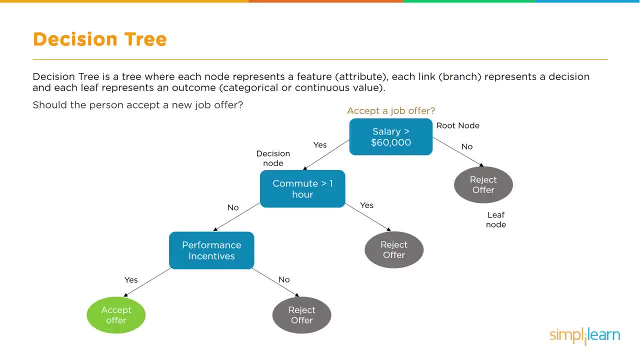 And then we have some inner nodes or decision nodes, And we have the nodes where we have a decision, either positive or negative. These are known as leaf nodes or terminal nodes. okay, So we have the root node and we have leaf nodes or terminal nodes. there can be multiple. 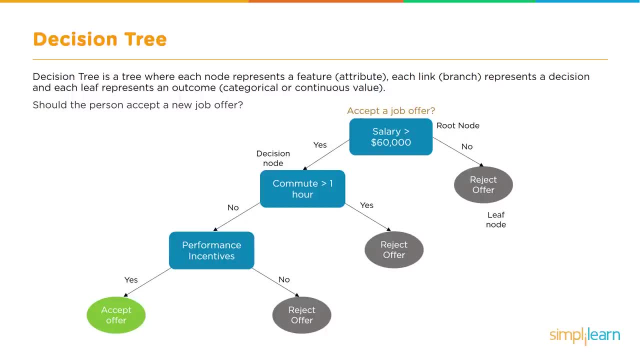 of them And in between we have decision nodes or internal nodes. there are different terms used, so need not be hung up by the exact terminology. Now let's say we have to use this decision tree to find out whether this person will accept the job offer or not. 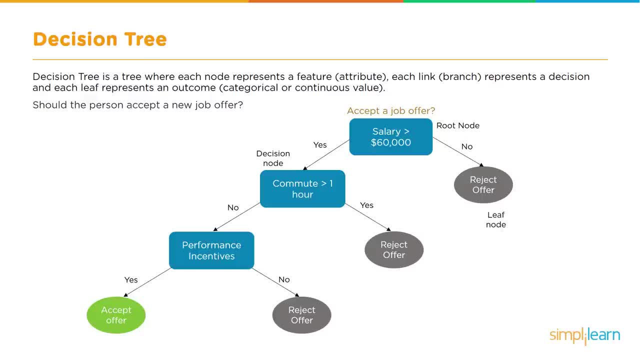 So first thing he considers is the salary. is the salary greater than 60,000?? If no, it's a clear decision: the offer will be rejected. So we reach a decision. This is a leaf node. Now, if the salary is greater than 60,000, it is not a clear cut decision because there 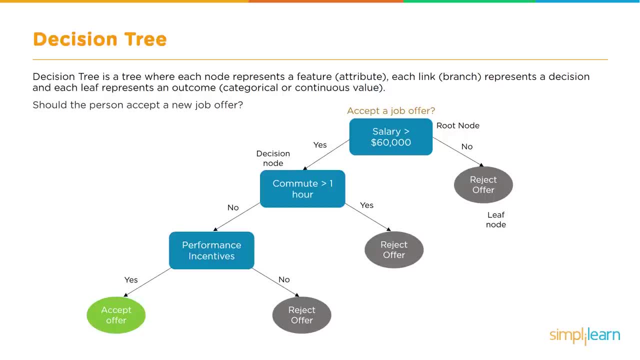 are probably other factors based on which the decision needs to be made. For example, what is the commute time? If the commute time is greater than one hour, then the offer is rejected. okay, So even though the salary is greater than 60,000.. 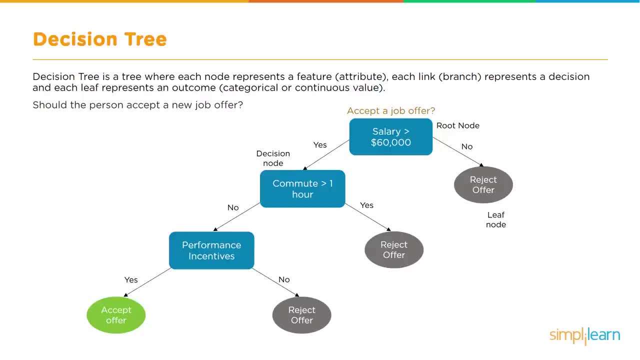 So this is again a leaf node. If the commute time is less than one hour, still it is not a confirmed decision because there are still a few other factors, For example performance incentives. Are there sufficient performance incentives as a part of this offer? 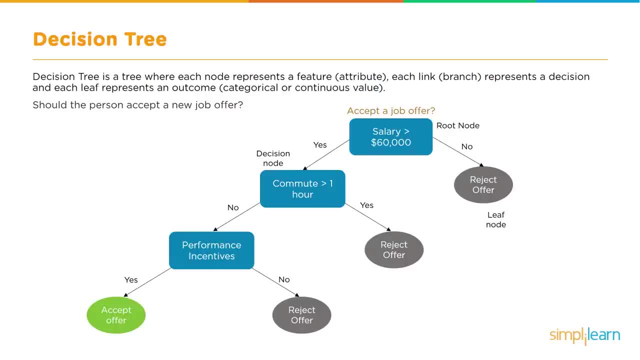 If no, then again the offer is rejected, and this is another leaf node. If yes, if there are sufficient performance incentives, then the offer is accepted. So this is another leaf node. By the way, keep in mind that these are all the leaf nodes. 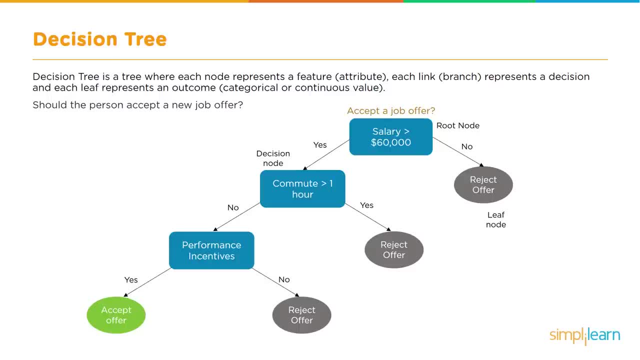 is a leaf node now. if the salary is greater than sixty thousand, it is not a clear-cut decision because there are probably other factors based on which the decision needs to be made. for example, what is the commute time if the commute time is Jersey? so we know that Gordon Waller is. 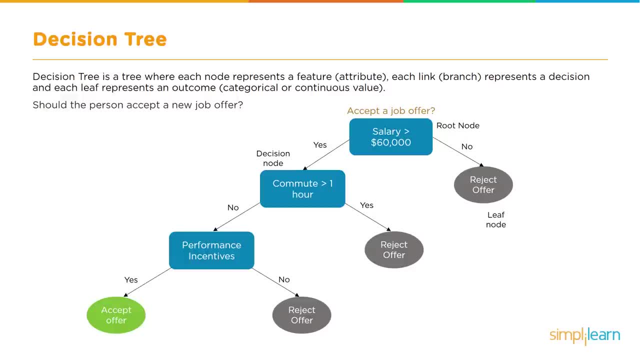 working day-to-day and so I would give him two fillers. an excuse: I pasted was the next supply model. other factors- we need to get more information accordingly- but also the number of options. they is greater than one hour, then the is rejected. okay, so even though the salary is greater than sixty, 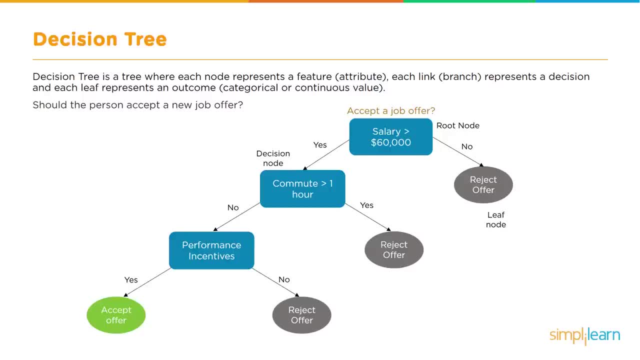 thousand. so this is again a leaf node. if the commute time is less than one hour, still it is not a confirmed decision because there are still a few other factors, for example performance incentives. are there sufficient performance incentives as a part of this offer? if no, then again the offer is rejected. and this is another leaf node. if yes, if there are sufficient performance. 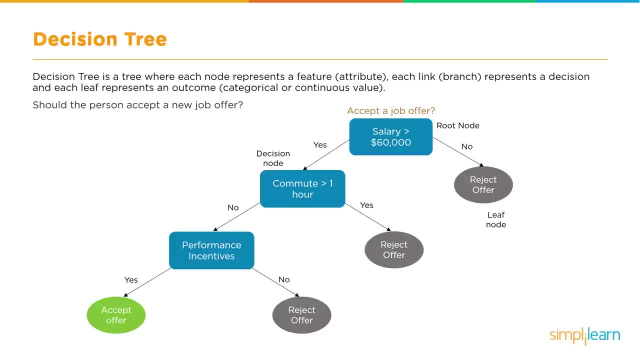 incentives, then the offer is accepted. so this is another leaf node. by the way, keep in mind that these are all the leaf nodes. this is a leaf node. this is a leaf node. this is a leaf node. there's a leaf node, and they, of course, belong to different categories. in this case, it is still a binary. 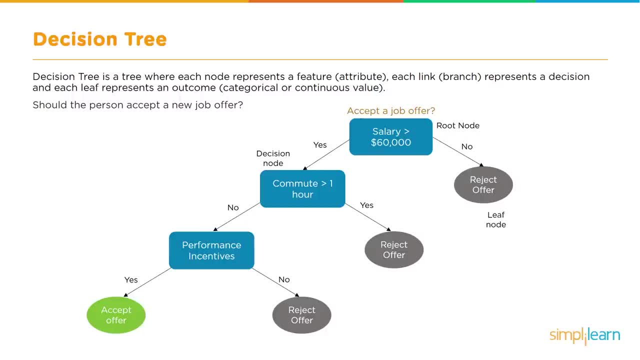 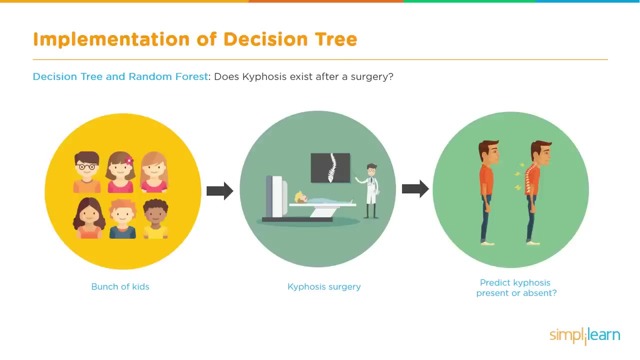 classification. so this belongs to one class, which is accept offer, and these leaf nodes belong to a different class, which is reject offer. so let's take an example and see how we can solve this problem using decision tree. let's say we have to implement a classification algorithm for kyphosis patient and the problem is a bunch of kids have been have undergone a. 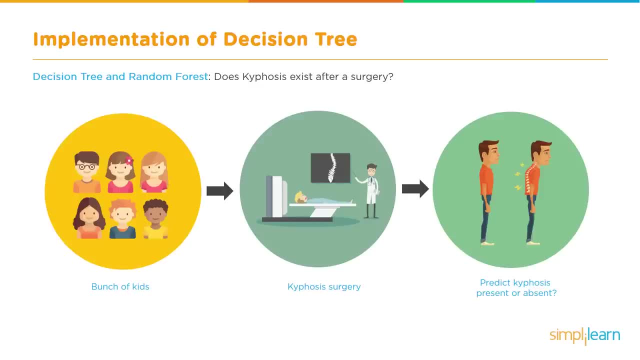 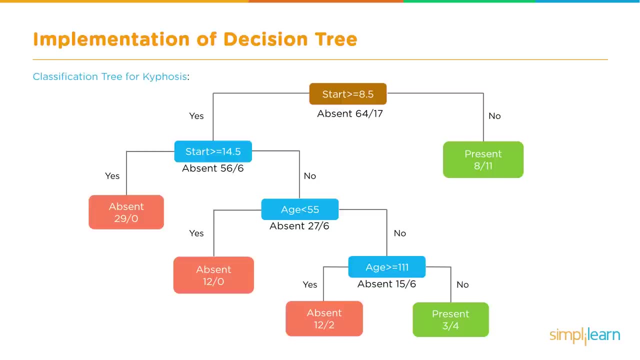 kyphosis surgery and we need to predict whether kyphosis is present in them or not. and how can we do this? using decision tree algorithm. so this is how the classification tree for kyphosis looks. so it starts with: if the age is greater than 8.5. so this is how the decision tree looks. so the 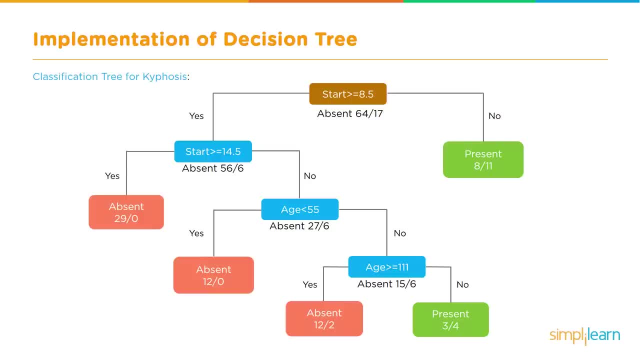 first criteria is the vertebra, the number of years of age number on which the surgery has been performed. if it is greater than 8.5, then we need to perform further analysis and look at other criteria. if it is less than 8.5, it is clear that kyphosis is. 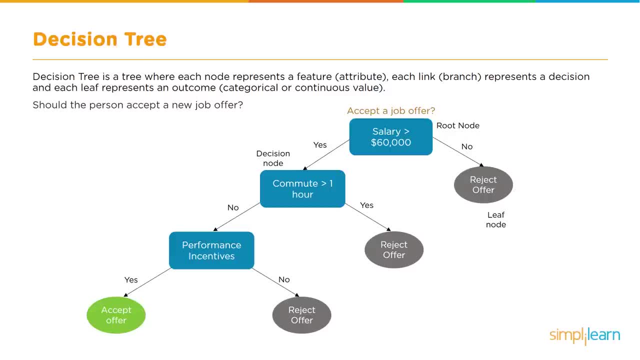 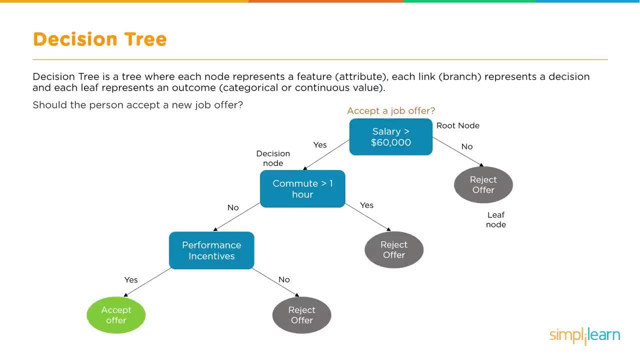 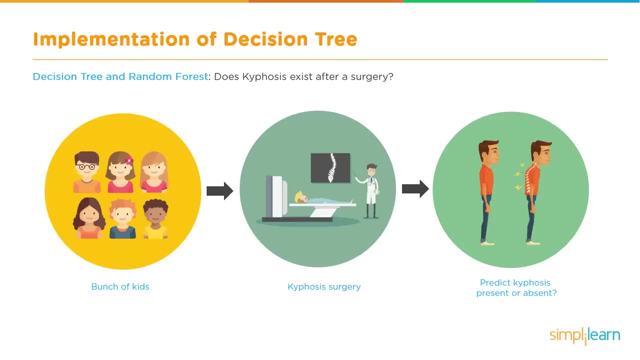 And these leaf nodes belong to a different class, which is reject offer. So let's take an example and see how we can solve this problem using decision tree. Let's say we have to implement a classification algorithm for kyphosis patient And the problem is a bunch of kids have undergone a kyphosis surgery and we need to predict. 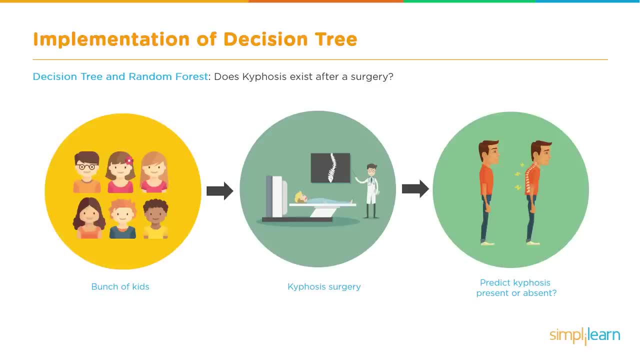 whether kyphosis is present in them or not. And how can we do this? using decision tree algorithm. So this is how the classification tree for kyphosis surgery works. So let's take an example and see how we can solve this problem using decision tree. 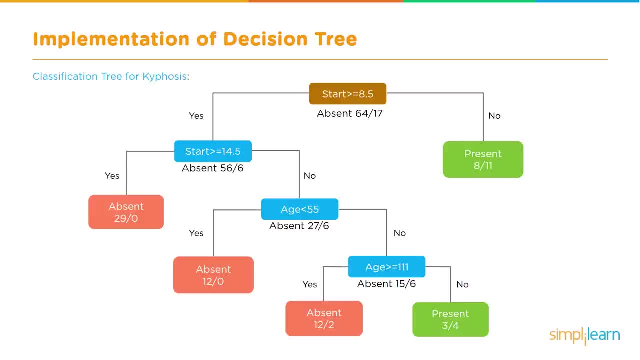 Let's take an example and see how we can solve this problem using decision tree. So let's take an example and see how the classification tree for kyphosis looks. So it starts with if the age is greater than 8.5.. So this is how the decision tree looks. 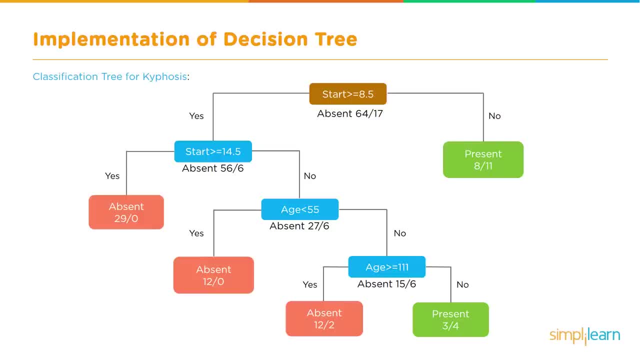 So the first criteria is the vertebrae, the number on which the surgery has been performed. If it is greater than 8.5, then we need to perform further analysis and look at other criteria. If it is less than 8.5, it is clear that kyphosis is present. 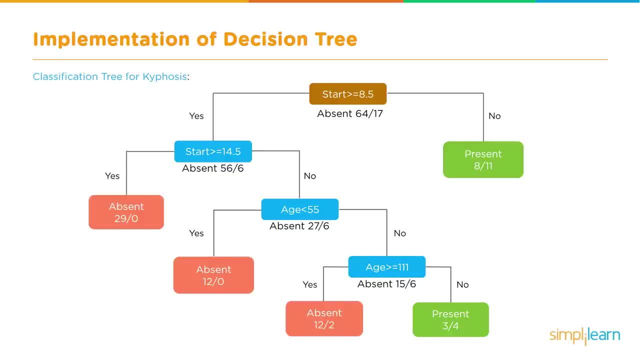 And if it is greater than 8.5.. then we check whether the vertebra operated upon is greater than 14.5 or not. if it is greater than 14.5, then kyphosis is absent. if not, then the next criteria is the age. if the person's age is less, 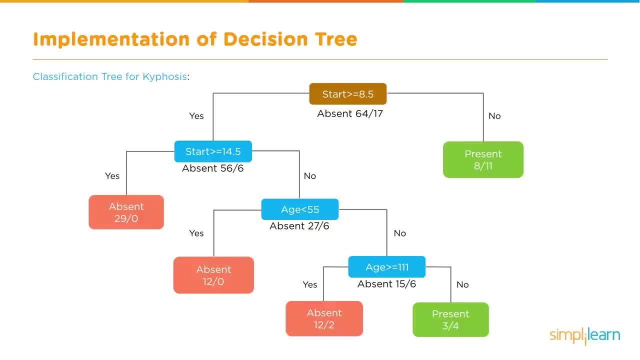 than 55 years, then kyphosis is absent. but if it is greater than 55 years, then a further analysis is required to see if the person's age is greater than 111 years, which is of course almost impossible, but yes. so if if no, then there is no kyphosis. then we check if the age is greater than 111 years. 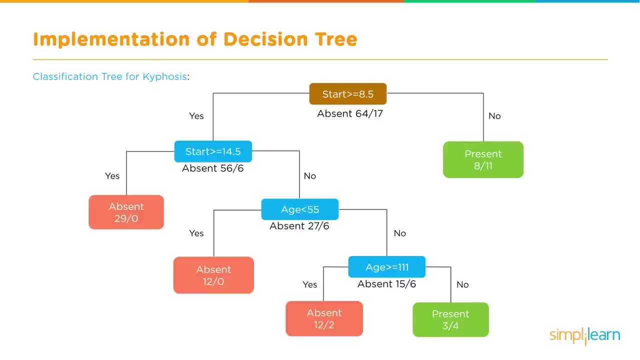 which means the person is between 55 and 111 years. if the person is between 55 and 111 years, that is this path. that means kyphosis is present, otherwise it is absent. so this is very easy to understand, but it is very easy to understand, and so if you are interested in this, then you can see that. 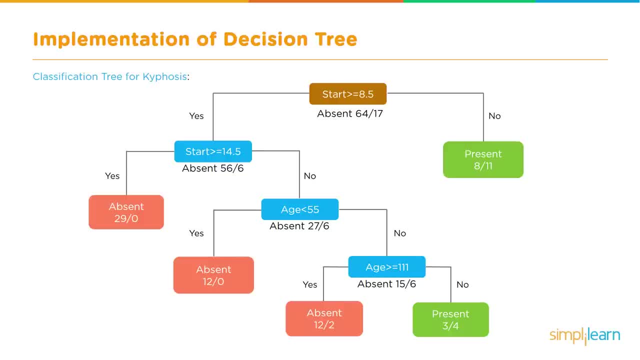 present, and if it is greater than 8.5, then we check whether the vertebra operated upon is greater than 14.5 or not. if it is greater than 14.5, then kyphosis is absent. if not, then the next is the age. if the person's age is less than 55 years, then kyphosis is absent, but if it is greater. 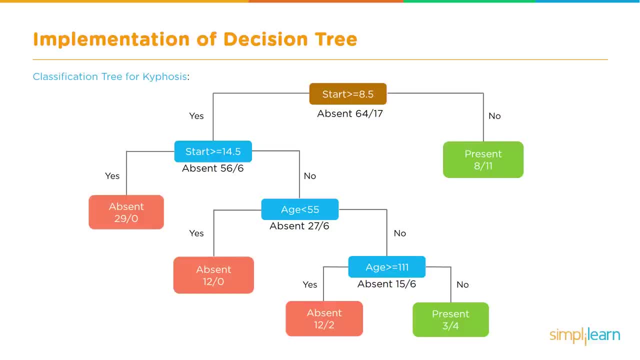 than 55 years, then a further analysis is required to see if the person's age is greater than 111 years, which is, of course, almost impossible, but yes. so if if no, then there is no kyphosis. then we check if the age is greater than 111 years, which means the person is between 55 and 111 years. if 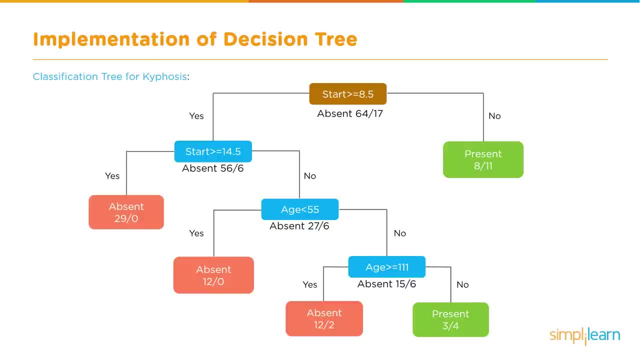 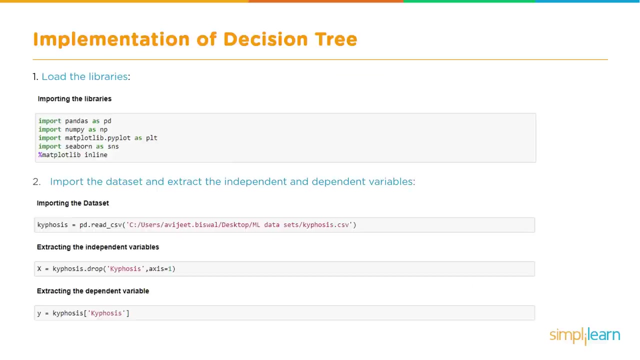 the person is between 55 and 111 years. that is this path. that means kyphosis is present, otherwise it is absent. so this is very easy to understand decision tree. and now what we are going to do is we are going to implement this in python in our jupyter notebook, and we have a data set that is: 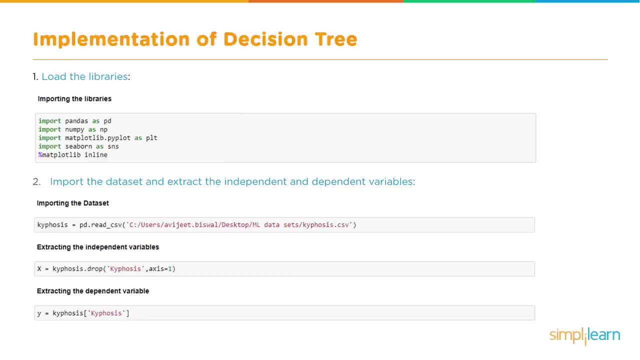 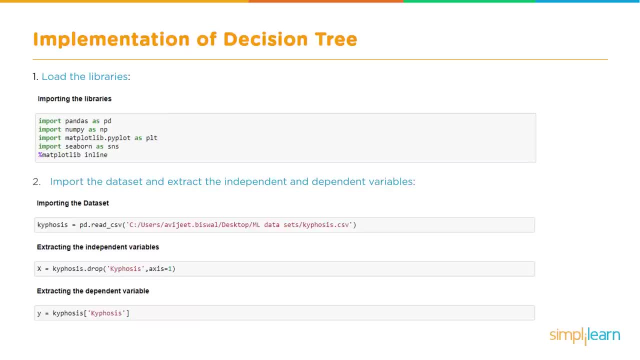 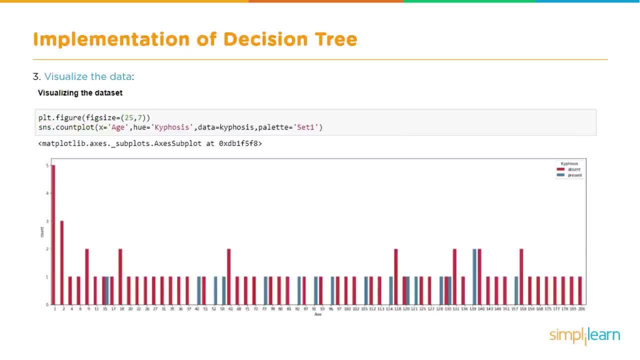 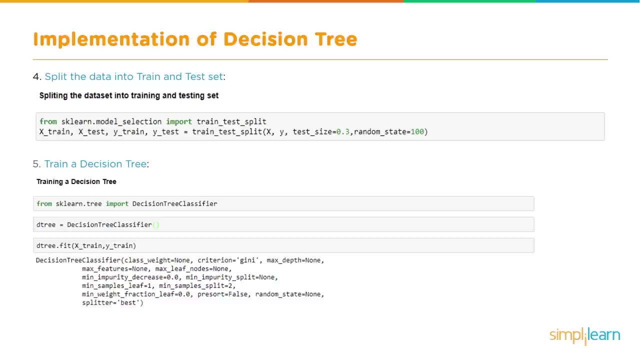 labels, which is the dependent variable, and then we visualize the data- this is how it looks- and then we, as usual, split the data into training and test data sets and then perform the training of the decision tree, and then we test that model with our test data and then, since this is a 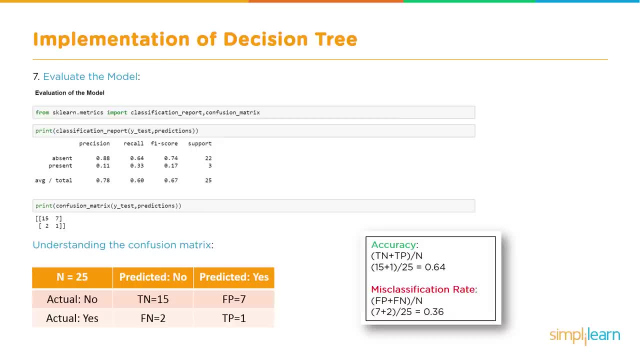 classification problem. we evaluate this model using the confusion matrix. remember we talked about this in the previous example as well. so this is the confusion matrix for this particular problem, and here you can see that 16 plus 3, 19 of them have been correctly predicted out of 25. 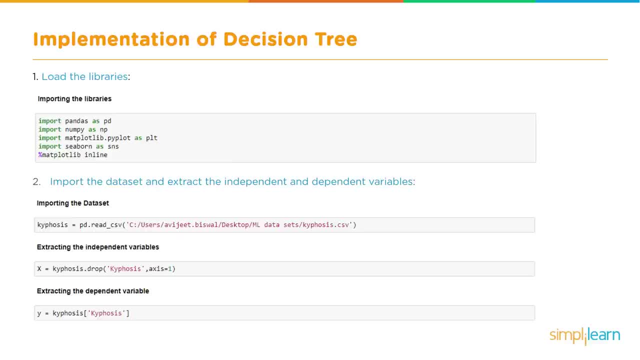 kyphosis is present in the data set and decision tree, and now what we are going to do is we are going to implement this in python in our jupiter notebook, and we have a data set that is available for this. and, once again, if anyone wants this data set, please put a comment under this video and we 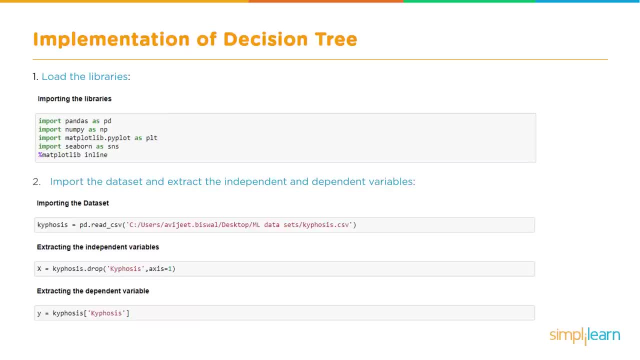 will be more than happy to share the data set with you. before we go into the jupiter notebook, let's take a look at what the code is doing. what are the various sections of the code? so first one of course we are going to do is we are going to extract the independent variables and then separate the 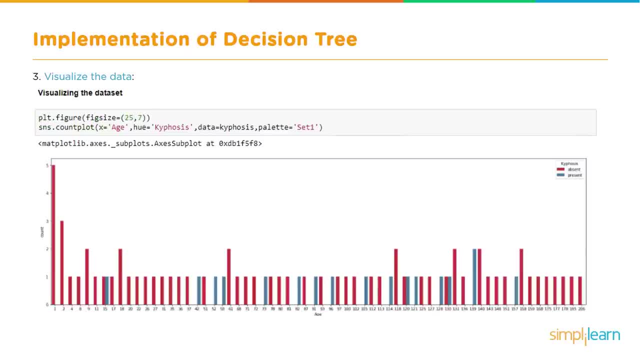 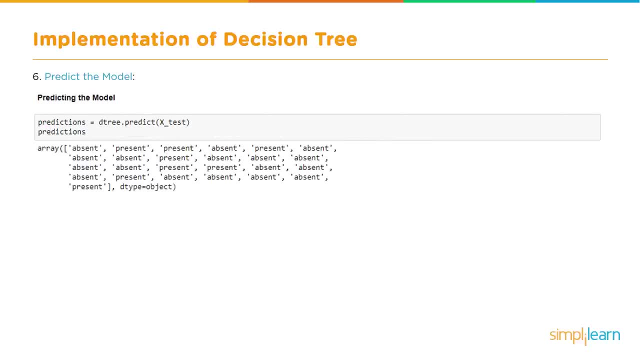 labels, which is the dependent variable, and then we visualize the data- this is how it looks- and then we, as usual, split the data into training and test data sets and then perform the training of the decision tree, and then we test that model with our test data and then, since this is a classification, 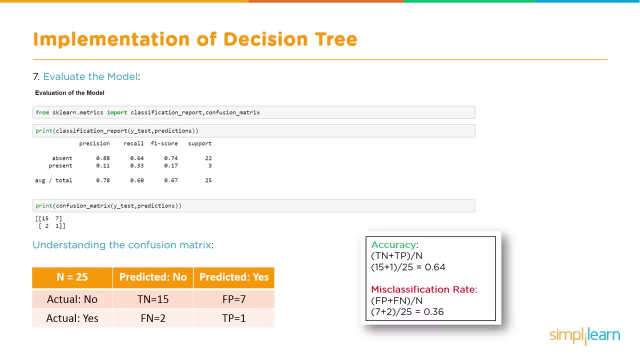 problem. we evaluate this model using the confusion matrix. remember we talked about this in the previous example as well. so this is the confusion matrix for this particular problem, and here you can see that 16 plus 3, 19 of them have been correctly predicted out of 25, which gives us a 64 percent accuracy, and this 4 plus 2, 6 of them have been misclassified. 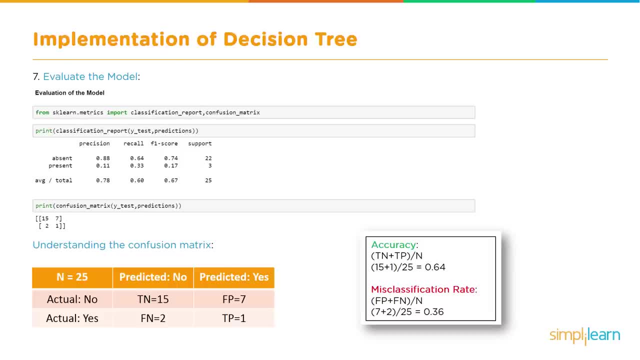 just to recap once again: how do we determine from the confusion matrix whether this is accurate or not? the numbers in this diagonal should be maximum. so here we see that out of 25, n is equal to 25, which is the total number of observations out of 25. in this case, in this diagonal, we have 16 plus 3. 19 of the values are here, so that's the. 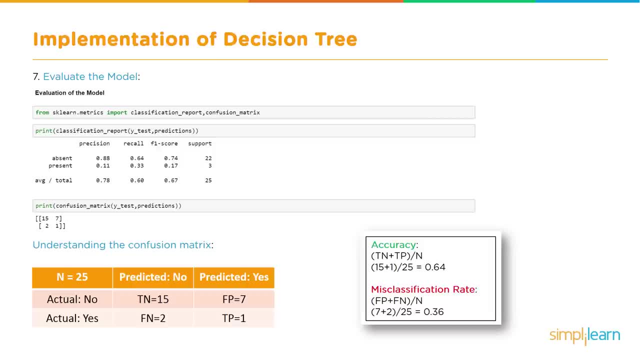 reason we feel there is good accuracy, which is 64 percent. they have been correctly classified. 64 percent of the observations have been correctly classified by this model, whereas 24 percent have been misclassified, which consists of this 4 plus this 2.. so that's how we use the confusion matrix. 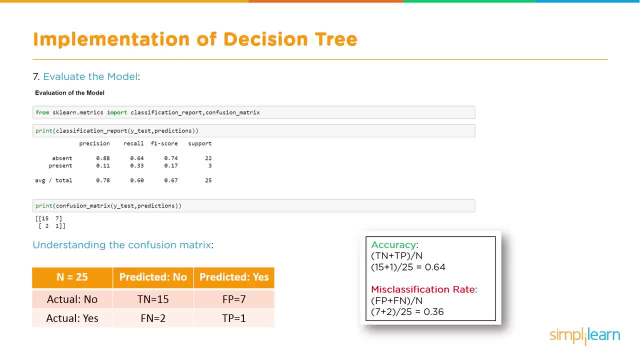 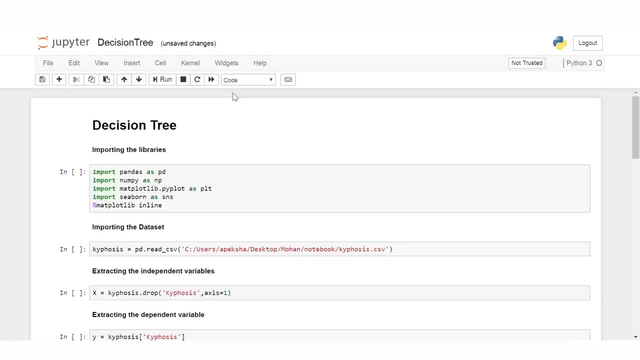 to determine the accuracy of our decision tree model. so let's go into the jupiter notebook and take a look and run the code and see how it looks. so this is our python notebook for decision tree and i will take you through the code, not line by line, of course, but we will see the blocks as: 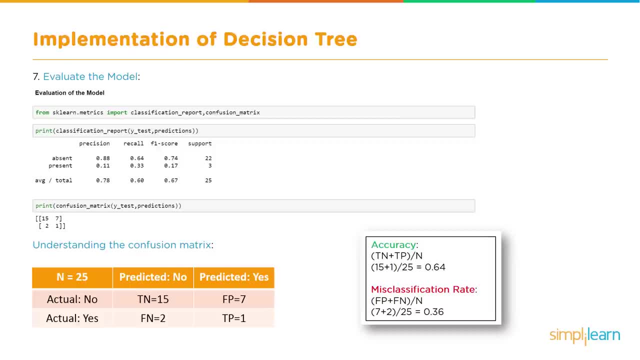 which gives us a 64 percent accuracy. and this four plus two. six of them have been misclassified. just to recap once again, how do we determine from the confusion matrix this is accurate or not? the numbers in this diagonal should be maximum. so here we see that. 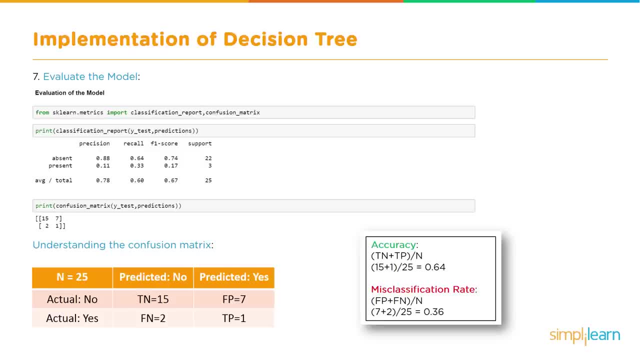 out of 25. n is equal to 25, which is the total number of observations out of 25. in this case, in this diagonal, we have 16 plus 3. 19 of the values are here, so that's the reason we feel there is good accuracy, which is 64. they have been correctly classified. 64 of the observations have. 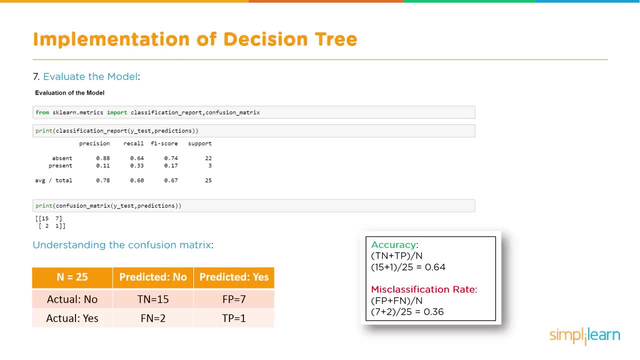 been correctly classified by this model, whereas 24 percent have been misclassified, consists of this four plus this two. so that's how we use the confusion matrix to determine the accuracy of our decision tree model. so let's go into the jupiter notebook and take a look and run. 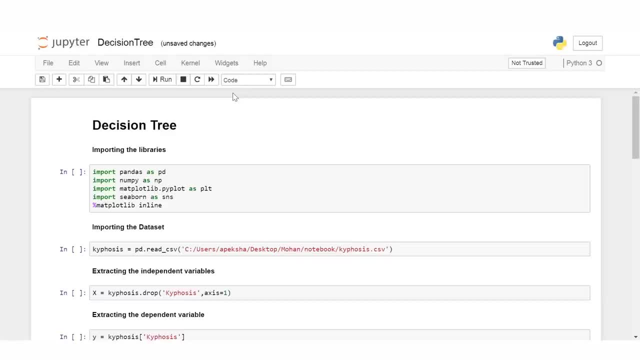 the code and see how it looks. so this is our python notebook for decision tree and i will take you through the code, not line by line, of course, but we will see the blocks, as always. the first block is to import the required libraries, like pandas and numpy and so on, and then we import the data. for this we are using kyphosis dot csv file, and then 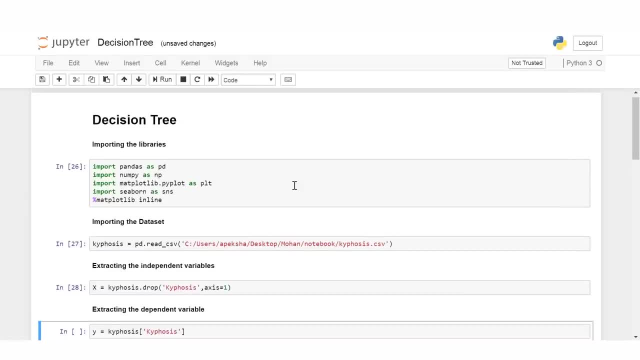 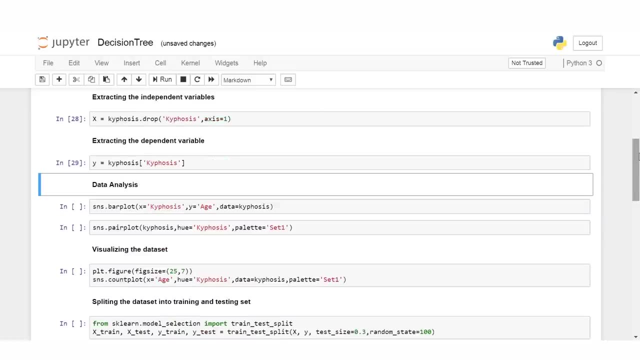 we extract the independent variables and then the dependent variable. dependent variable is the target, which is our classification, and also we call it as the label data, whether it is whether this person, individual, has kyphosis or not, and then we will run a little bit of initial exploratory analysis. 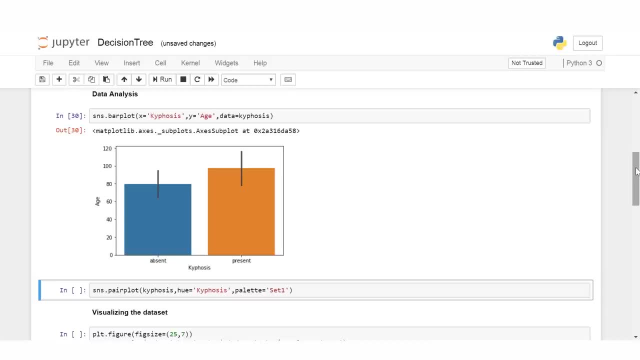 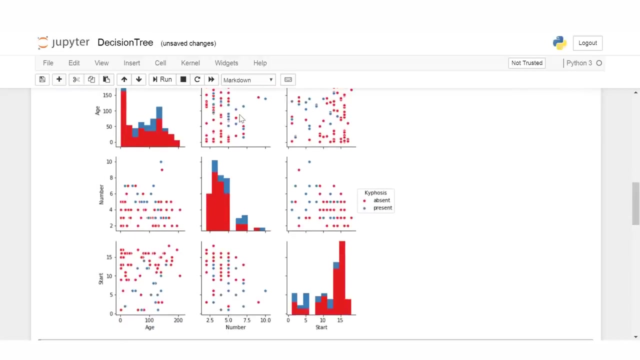 so, as a data scientist, whenever you get new data, you do that. so we plot age against whether the person has kyphosis or not, and then we plot the various parameters against each other. so, for example, this is like age versus the number and, by the way, the data. how does the data look? let's 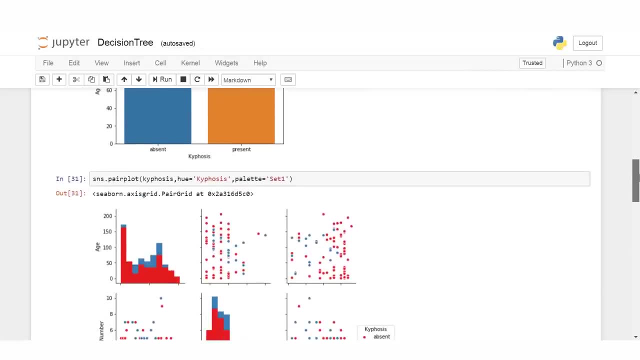 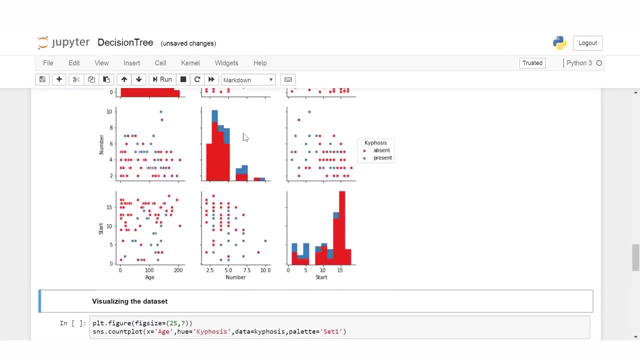 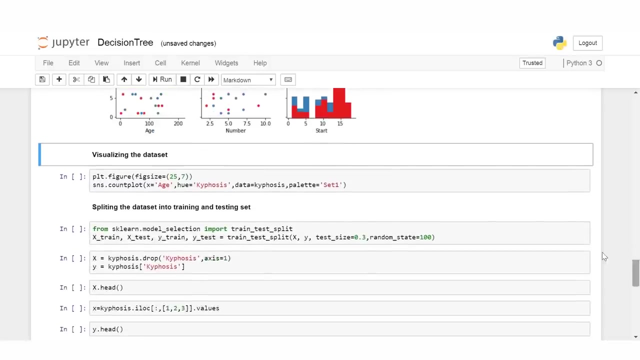 take a look at the data. this has primarily three columns, one attribute against the other. so, for example, this is age versus the number, the number versus the start, and so on and so forth. so this is just to give get a quick idea about the overall, how the overall data looks. so we can do. 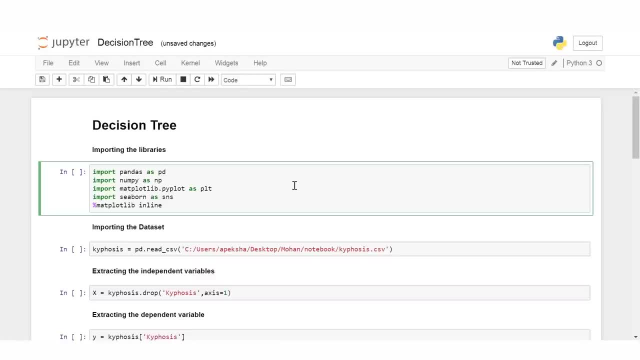 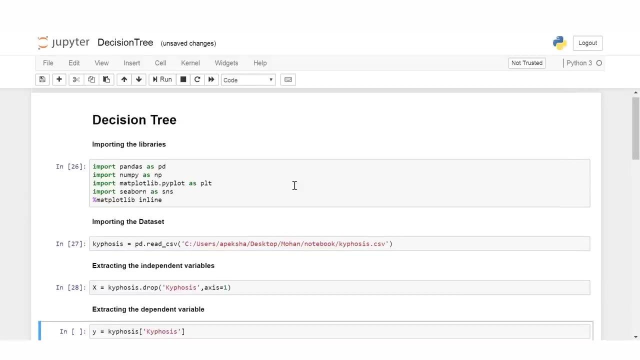 always the first block is to import the required libraries like pandas and numpy and so on, and then we import the data- for this we are using kyphosis dot csv file- and then we extract the independent variables and then the dependent variable. dependent variable is the target, which is 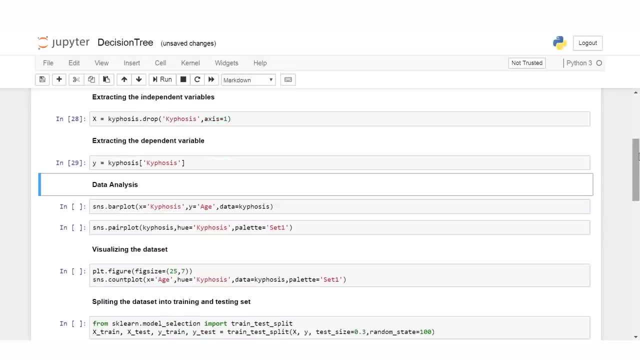 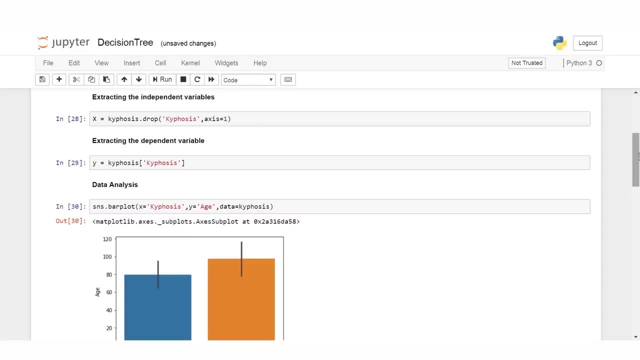 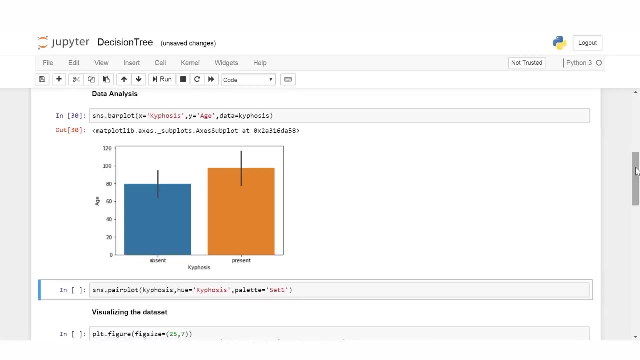 our classification and also we call it as the label data, whether it is whether this person individual has kyphosis or not, and then we will run a little bit of initial exploratory analysis on the data. so, as a data scientist, whenever you get new data, you do that. so we plot age against. 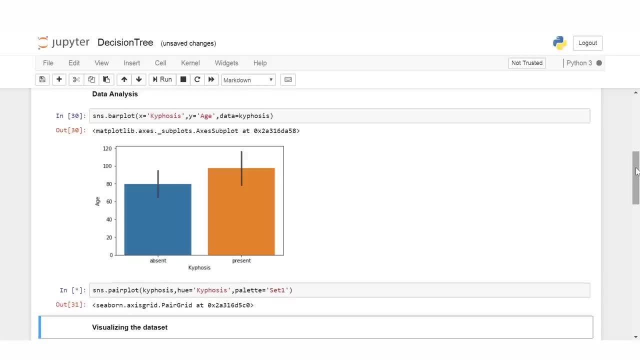 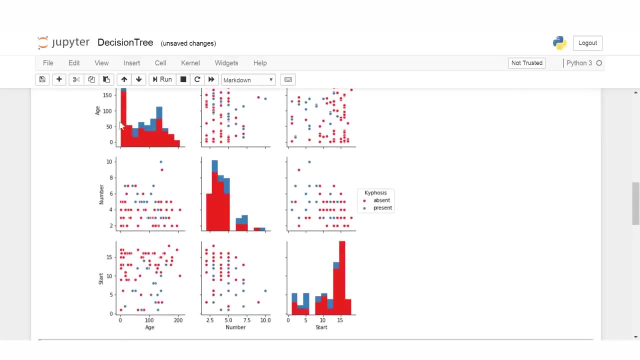 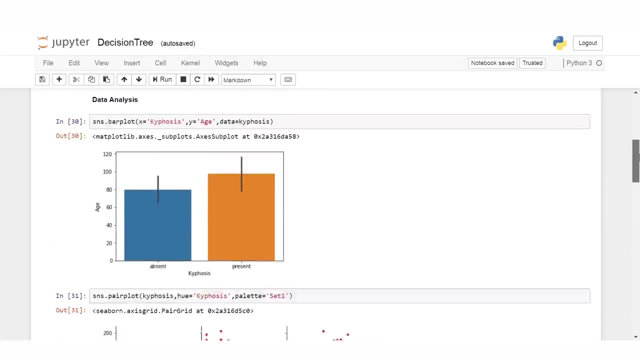 whether the person has kyphosis or not, and then we plot the various parameters against each other. so, for example, this is like age versus the number and, by the way, the data. how does the data look? let's take a look at the data. this has primarily. 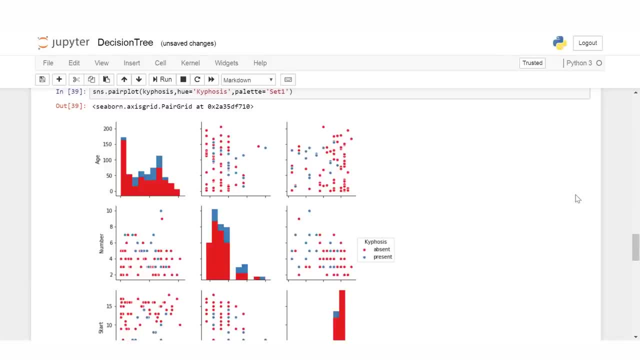 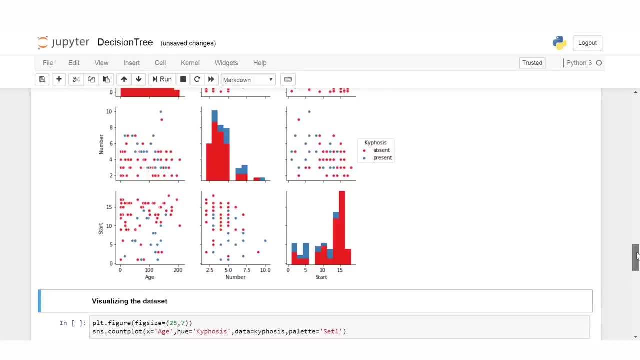 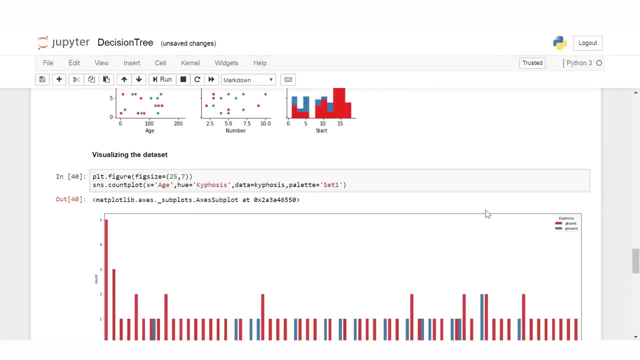 three columns, one attribute against the other. so for example, this is age versus the number, the number versus the start, and so on and so forth. so this is just to give get a quick idea about the overall, how the overall data looks. so we can do a few more visualizations like: 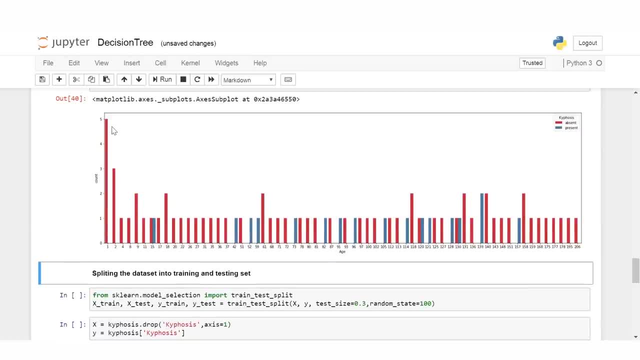 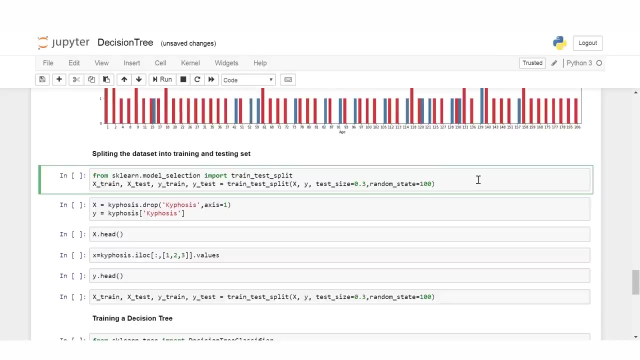 with respect to the age and the count, the number of vertebrae that have been operated upon, and the red color indicates kyphosis is absent and the blue color indicates kyphosis is present. so this is another view, and so on. so we can basically do as much of exploratory analysis we want. we can, and 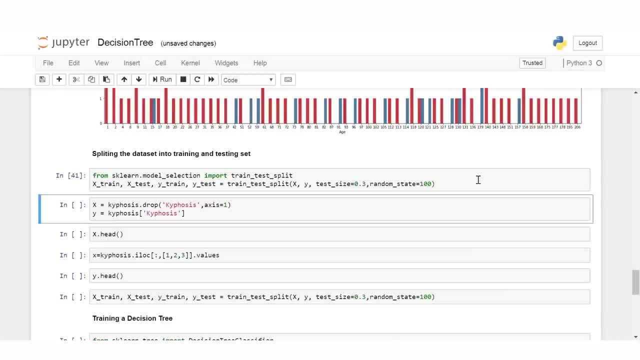 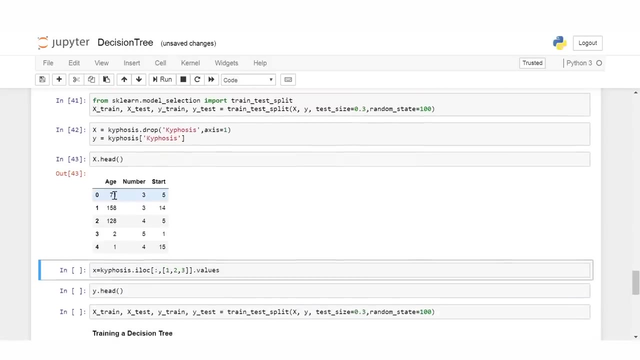 then we start training our model. so this is where we split the data into training and test data set, like in all of the machine learning examples earlier also, and we can visualize the data or just quick take a quick look at how the data looks, just the first four or five entries here. if we do, 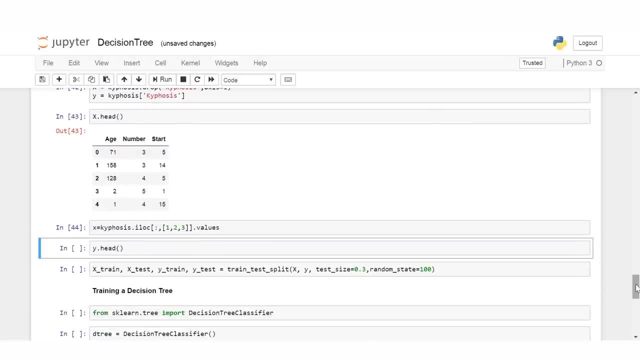 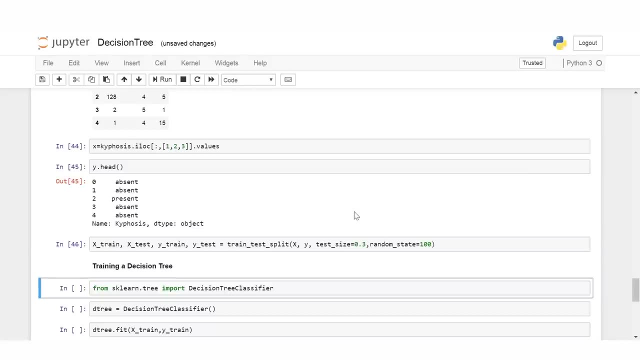 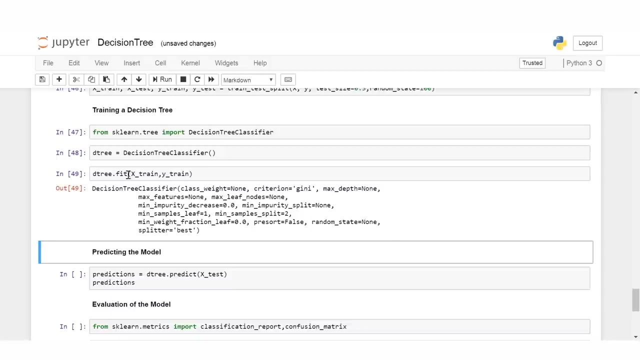 the head. that's what the head function does- and similarly y as well. we can take a look at how the target is looking and then we can get into the training of the decision tree. so we train our model with the training data set using this fit method and then we test whether the model is. 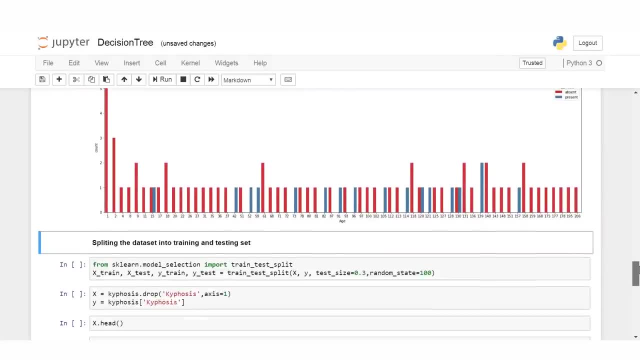 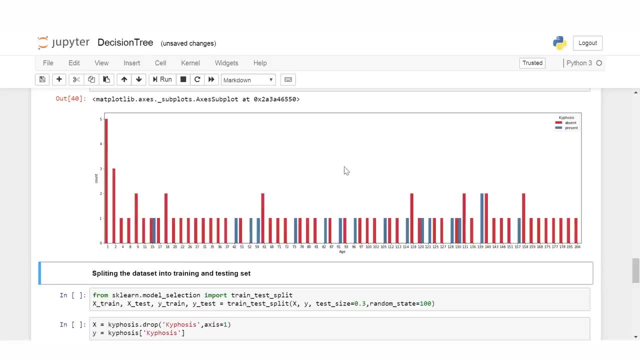 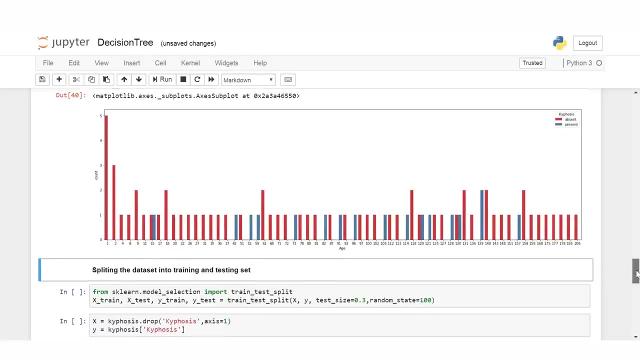 a few more visualizations, like with respect to the age and the count, the number of vertebrae that have been operated upon, and the red color indicates kyphosis is absent and the blue color indicates so this is another view, and so on. so we can basically do as much of exploratory analysis. 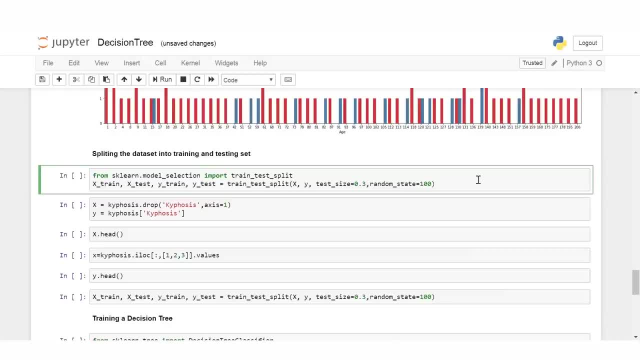 we can, and then we start training our model. so this is where we split the data into training and test data set, like in all of the machine learning examples earlier also, and we can visualize the data or just quick. take a quick look at how the data looks. 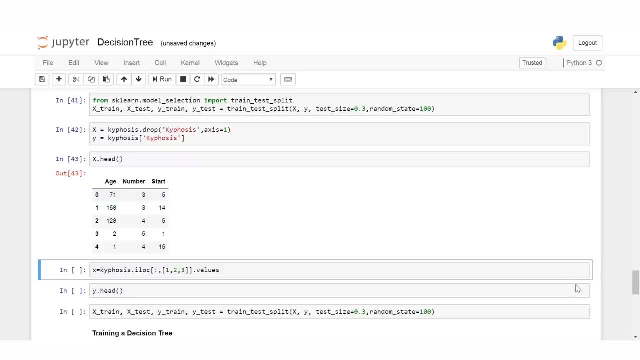 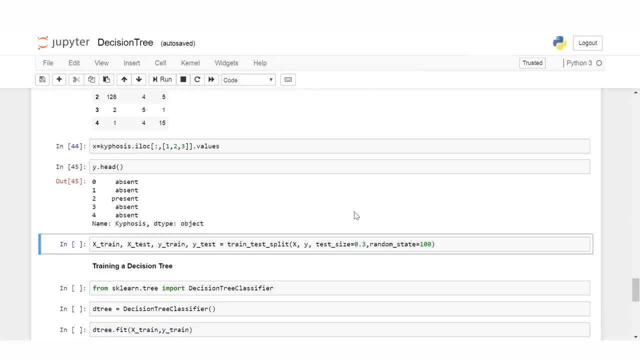 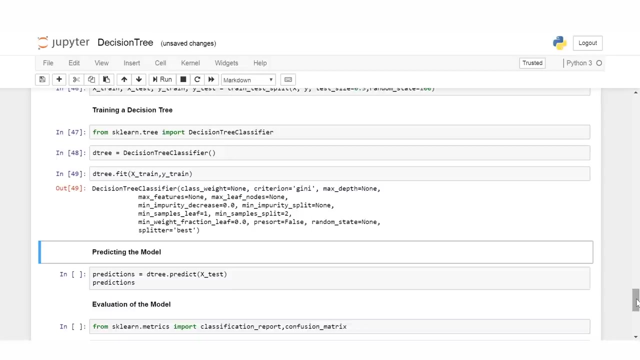 just the first four or five entries here. if we do the head, that's what the head function does, and similarly y as well, we can take a look at how the target is looking and then we can get into the training of the decision tree. so we train our model with the training data set. 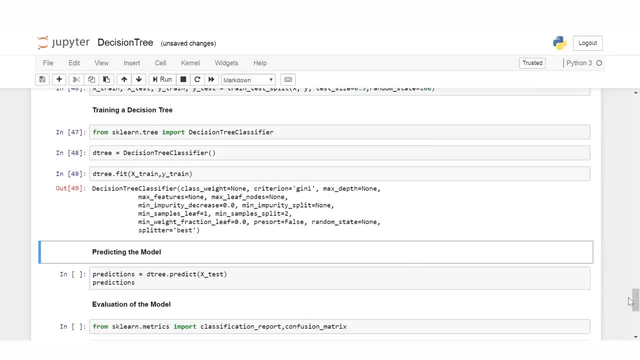 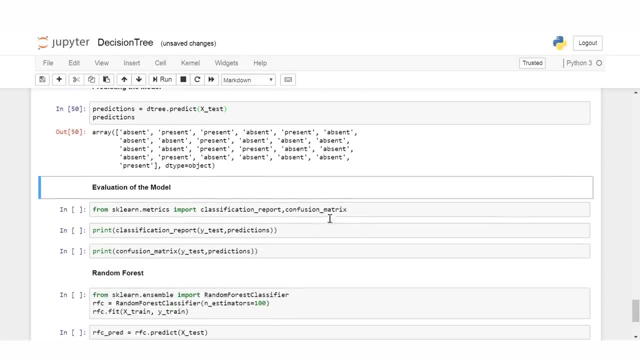 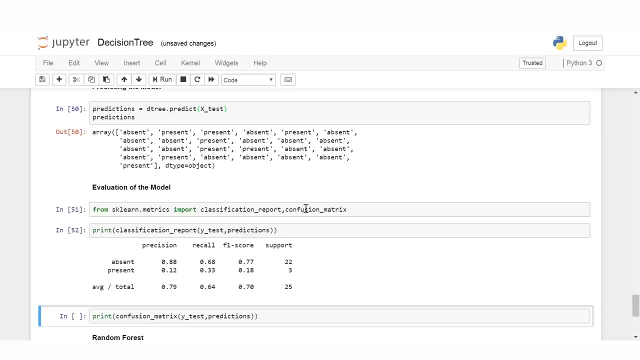 using this fit method and then we test whether the model is working fine or not using the test data set, and this is the result of our test data. and then we evaluate the model, and for evaluating we use the confusion matrix. so just let's take a quick look at the confusion matrix and see. 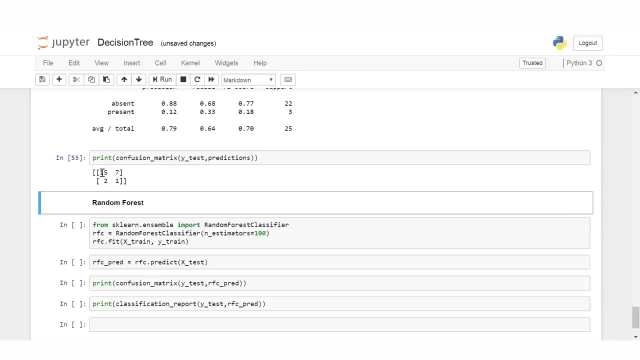 what is the accuracy? so we get about 16 right. as i mentioned, the diagonal values is what matters, so we have 16 of them correctly identified out of 25. so that gives us about 62- i think 70- accuracy. so that is using decision tree now instead of decision tree. 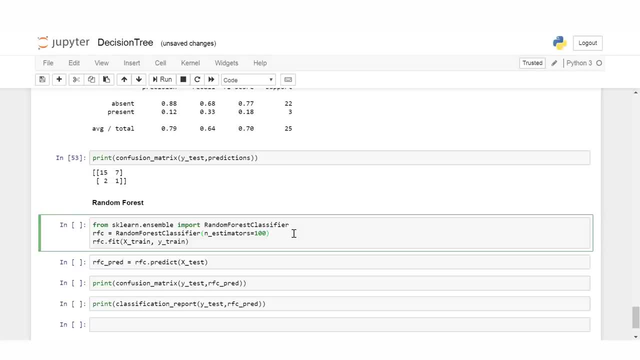 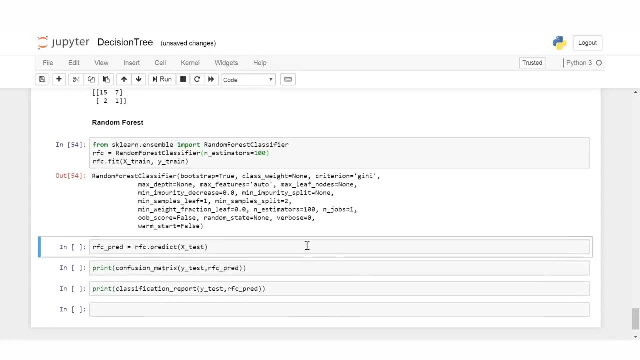 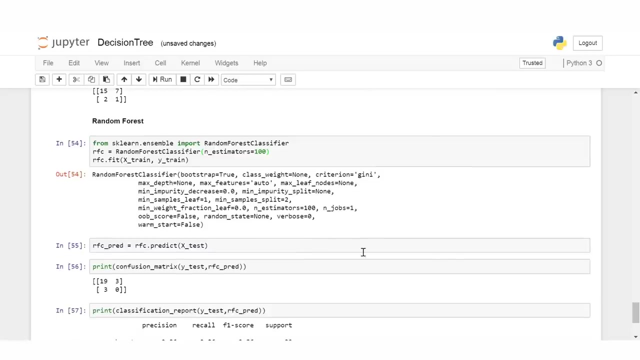 what happens if we use random forest. so we use, let's say, the- our forest consists of hundred trees- and we do the same. we train our model and then, with the test data set, we try to test the model, and here we see that we get 19 of them out. 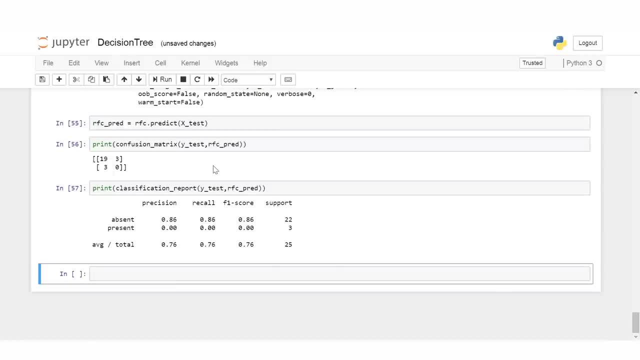 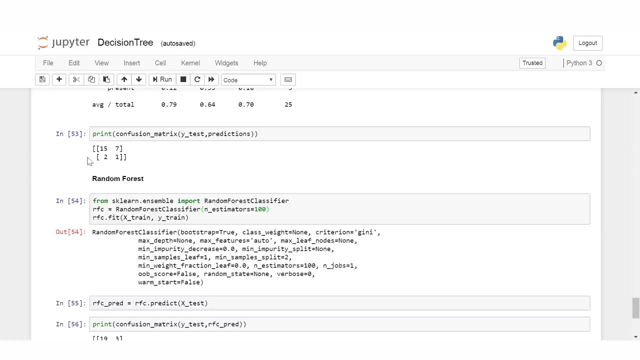 of 25 correct, so that is a much better accuracy. so this is about 76%. so 19 out of 25 is 76% accuracy and we saw in by using the decision tree. we got only 64 percent. that is, 16 by 25 was only 64 percent. so this is a quick demo of 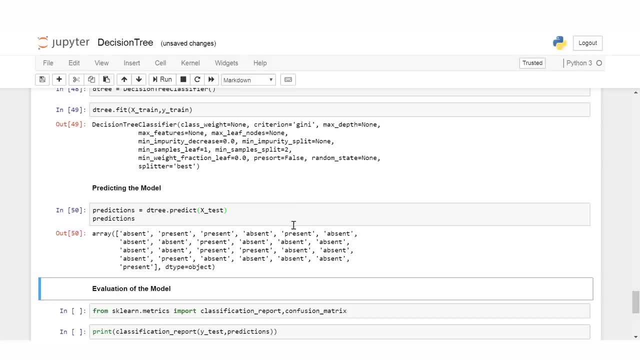 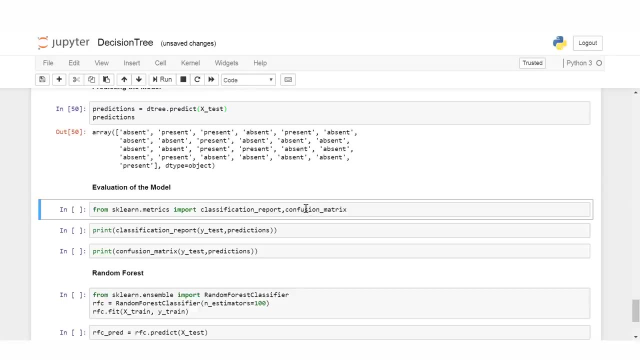 working fine or not, using the test data set, and this is the result of our test data. and then we evaluate the model, and for evaluating we use the confusion matrix. so just let's take a quick look at the confusion matrix and then we苦 through that and then check if the model is correct. if it is not, we go to fin. Finally, we cançket. 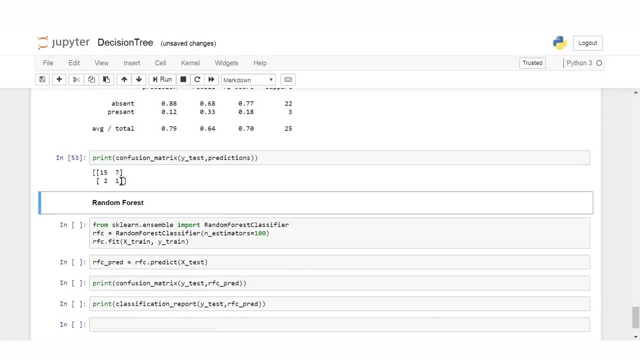 matrix and see what is the accuracy. So we get about 16, right, as I mentioned, the diagonal values is what matters. So we have 16 of them correctly identified out of 25.. So that gives us about 62,, I think, 70% accuracy. So that is using decision tree Now instead of decision tree. 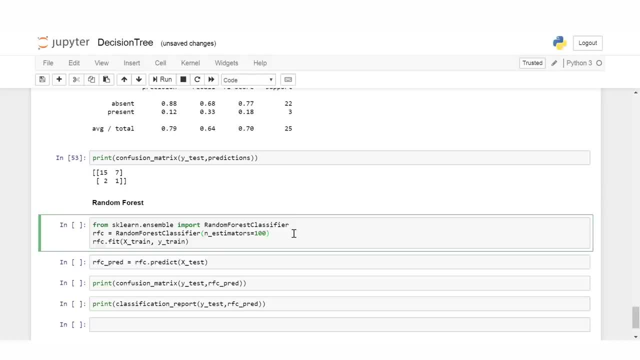 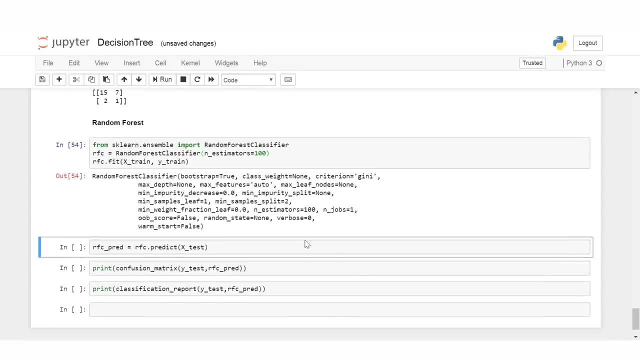 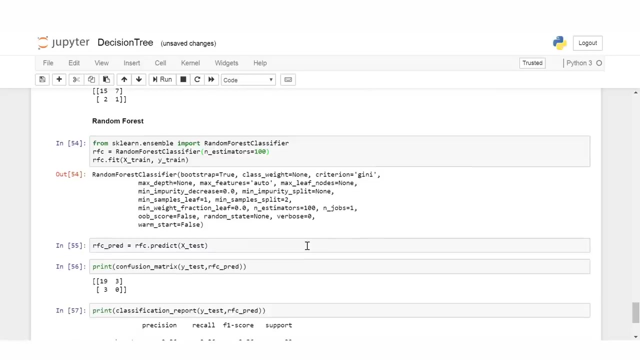 let's check what happens if we use random forest. So we use, let's say, the. our forest consists of 100 trees- And we do the same. we train our model And then, with the test data set, we try to test the model, And here we see that we get 19 of them out of 25.. Correct, So that is a much better. 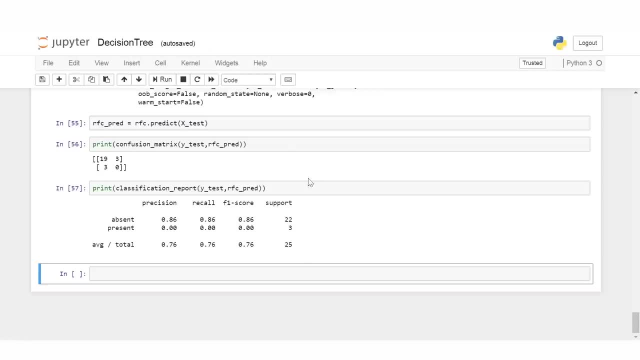 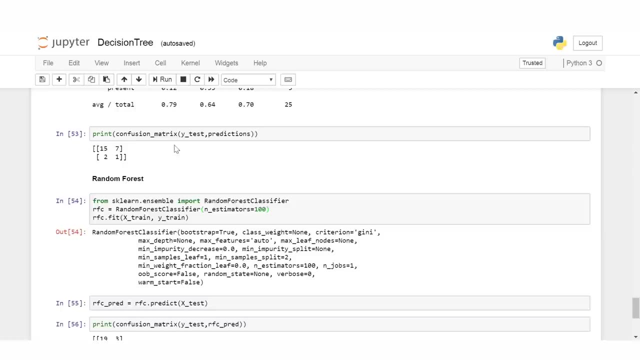 accuracy. So this is about 76%. So 19 out of 25 is 76% accuracy And we saw in by using the decision tree. we got only 64%. That is, 16 by 25 was only 64%. So this: 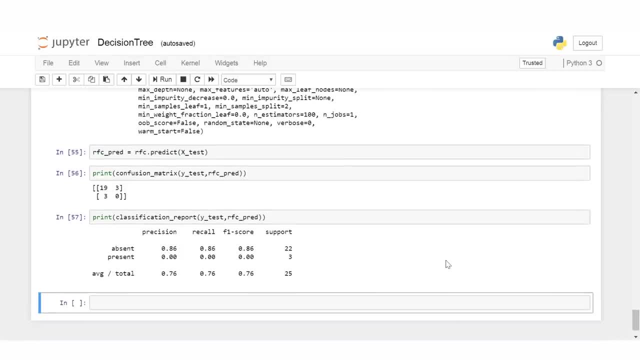 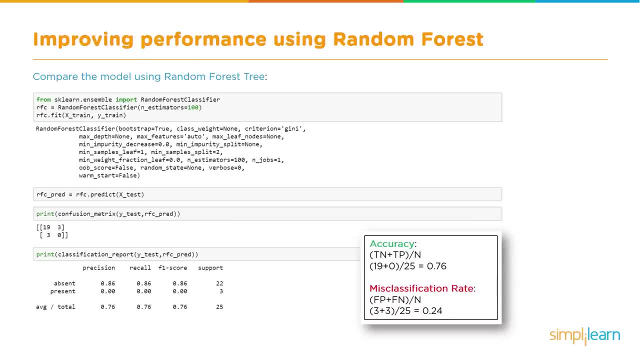 is a quick demo of implementation of decision tree. So once we evaluate the model, the next thing we can do is what happens if we want to improve the performance. So that's where random forest comes into play. So, in instead of using a decision tree, what happens if we use a decision? 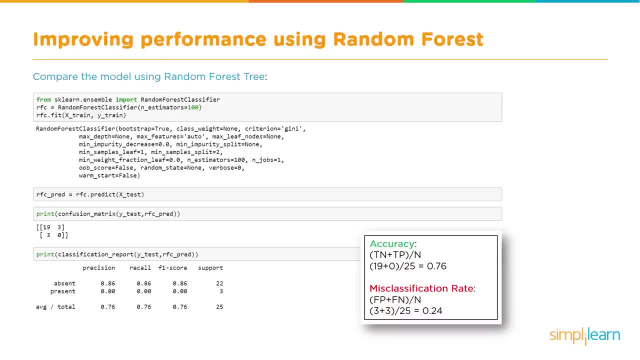 tree, we use a random forest. And what is a random forest? it's very similar to decision tree. only thing is that instead of using one tree, we use a number of trees. that's why it's called a forest. So we use multiple trees and we take like a average or a voting of all the trees for each. 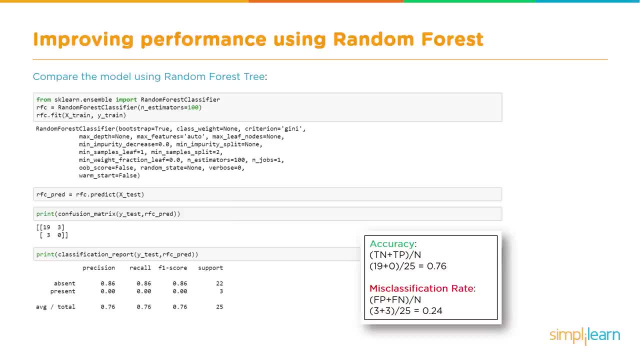 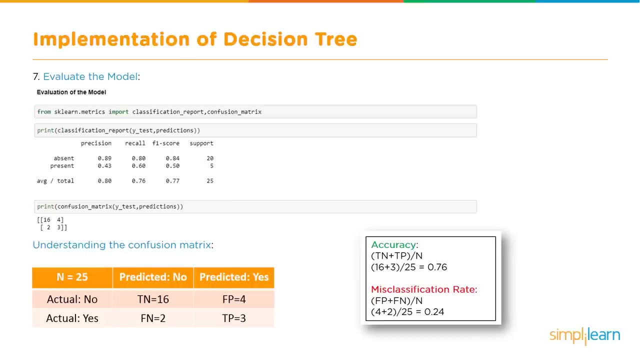 observation And we finally calculate or we finally classify each observation based on that. So in this case it helps in improving the accuracy. So, as we have seen here, if we take a decision tree, the accuracy now comes to 76%- Right, In the previous case it was only 64% using 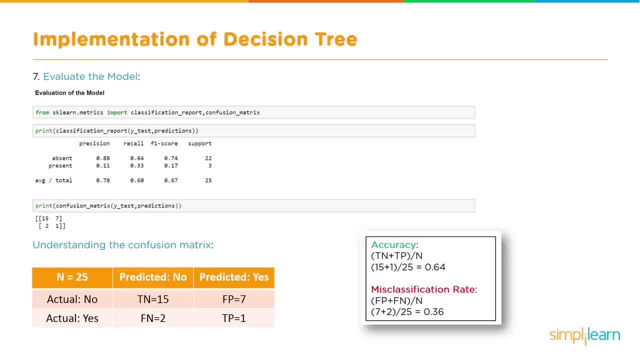 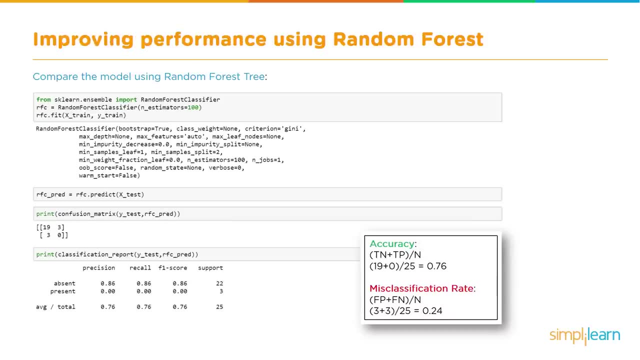 implementation of decision tree. so, once we evaluate the model, the next thing we can do is what happens if we want to improve the performance? so that's where random forest comes into play. so, in instead of using a decision tree, what happens if we use a random forest? and what is a random? 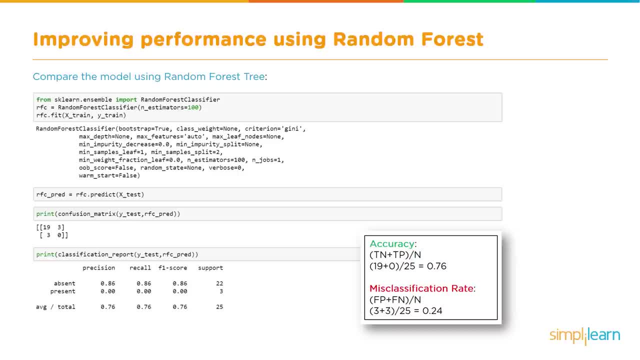 forest. it's very similar to decision tree, only thing is that instead of using one tree, we use a number of trees. that's why it's called a forest. so we use multiple trees and we take like a average or a voting of all the trees for each observation and we finally calculate, or we finally classify each. 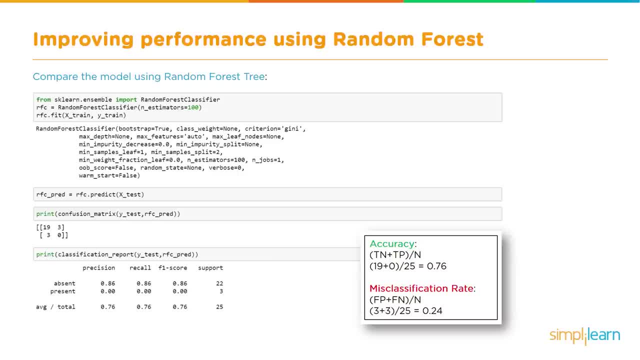 observation based on that. so in this case it helps in improving the accuracy. so, as we have seen here, if we take it decision tree, the accuracy now comes to 76 percent. right, in the previous case it was only 64 person using just the decision tree. now, when we use random forests, the performance has improved to. 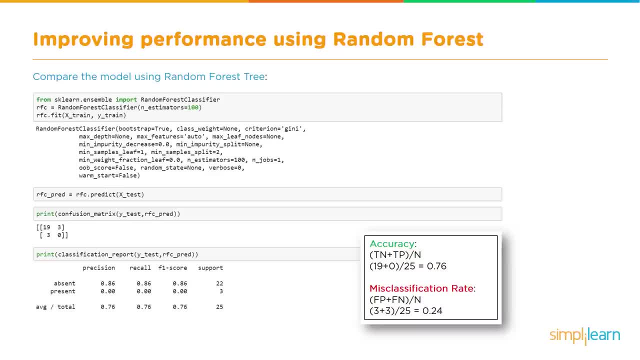 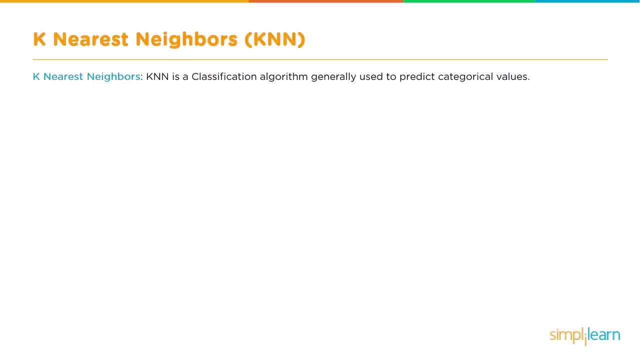 a good extent and it has become 76 percent. so random forests usually helps in increasing the accuracy when we are using decision trees as our algorithm. okay, the last algorithm is the K nearest neighbors algorithm. This is again a classification algorithm and it is actually very simple and 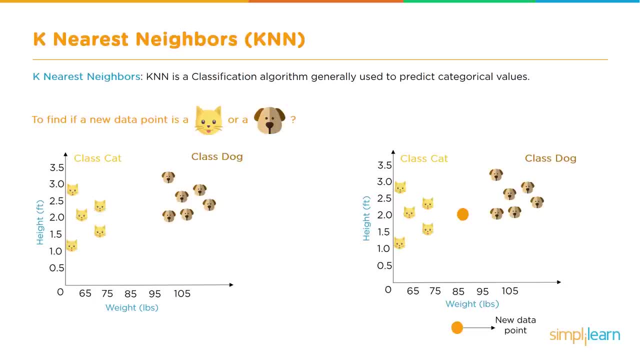 straightforward, very easy to understand as well. In this case, let's say, we have historical data of heights and weights and we also have the labels. So if the height and weight is in this range, these are cats, and if the heights and weights are in this range, these are dogs. So 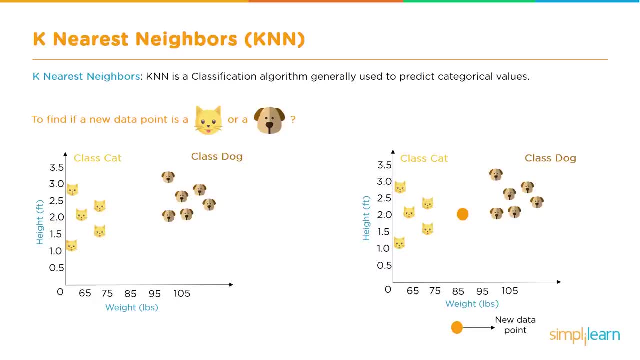 this is one class and this is another class. And now if we get a new point or new data set and we find that for this particular animal the height and weight if we plot it is here. So how do we determine whether it belongs to the cat class or the dog class? That is where the K here comes into. 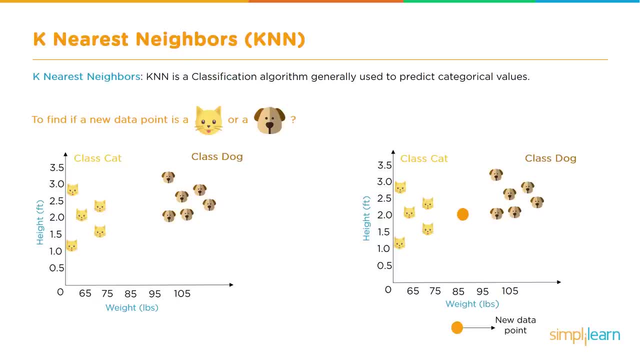 play. So when we are using this algorithm, we need to specify what should be the value of K. So let's say we say we determine that the value of K is 3.. So what we will do is we will find out the nearest value of K. So let's say we say we determine that the value of K is 3.. So what we 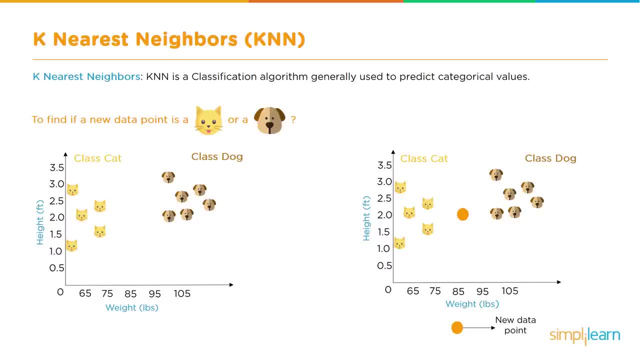 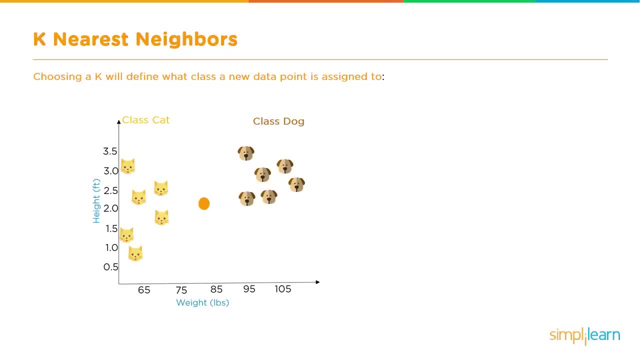 will do is we will find out the nearest 3 objects to this data point that we have. So let's go to the next slide here. Okay, And we define K as 3.. So what happens? We find the nearest 3 objects to. 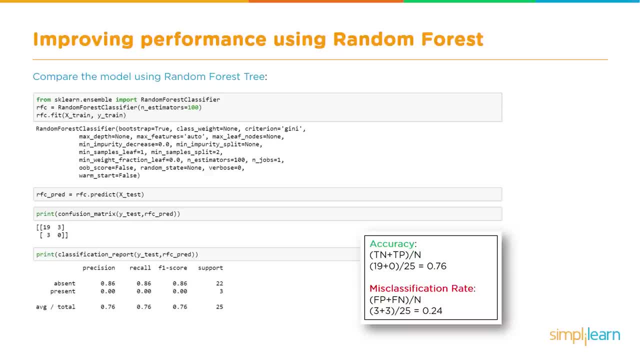 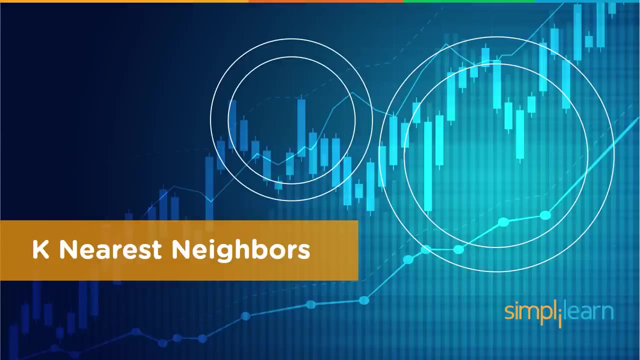 just the decision tree. Now, when we use random forest, the performance has improved to a good extent and it has become 76%. So random forest usually helps in increasing the accuracy when we are using decision trees as our algorithm. Okay, the last algorithm is the k: nearest neighbors. 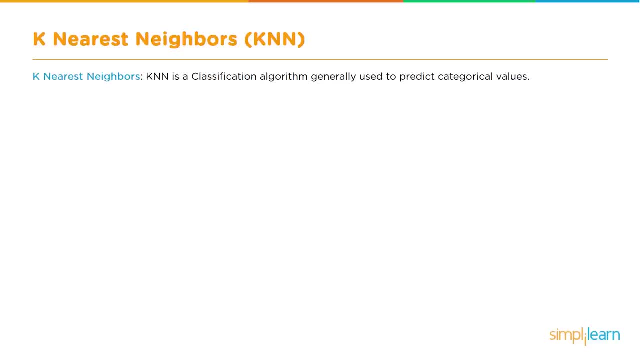 association algorithm, And it is actually very simple and straightforward, very easy to understand as well. In this case. let's say, we have historical data of heights and weights And we also have the labels. So if the height and weight is in this range, these are cats, and if 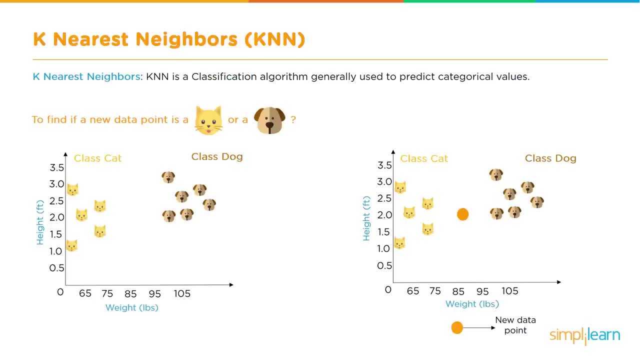 the heights and weights are in this range. these are dogs, So this is one class and this is another class. And now if we get a new point or new data set and we find that for this particular animal, the height and weight, if we plot, it is here. So how do we determine whether it belongs to the cat? 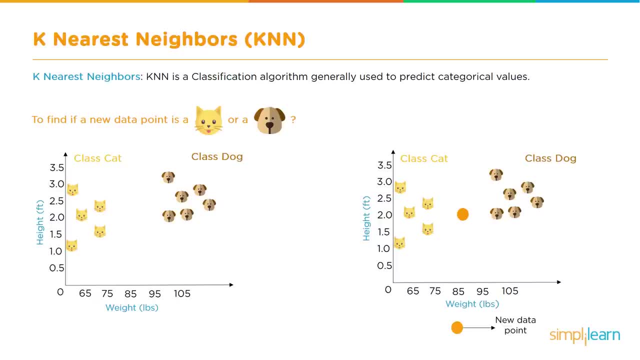 class or the dog class. that is where the k here comes into play. So when we are using this algorithm we need to specify what should be the value of k. So let's say we say we determine that the value of k is three. So what we will do is we will find out the nearest objects, nearest three. 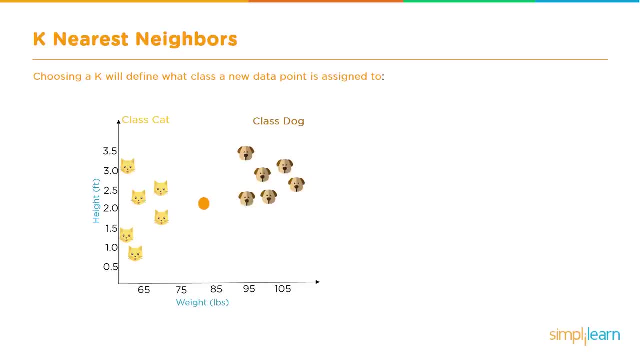 objects to this data point that we have. So let's go to the next slide here. Okay, and we define k as a value of k And we define k as a value of k. And we define k as a value of k And we define k as. 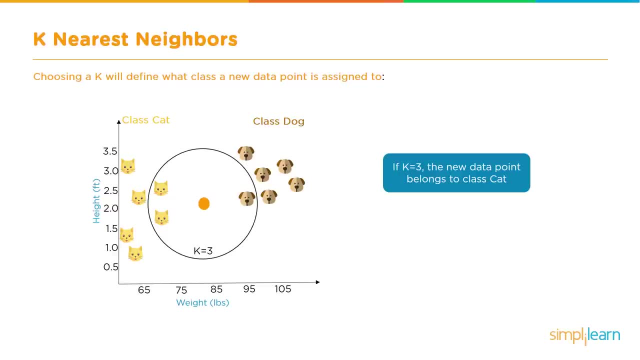 three. So what happens? we find the nearest three objects to this data point And then we find out what is the maximum number of items, which class the maximum number of items belong to? So in this case, there are two cats and there is one dog. Therefore, we determine that this new data point 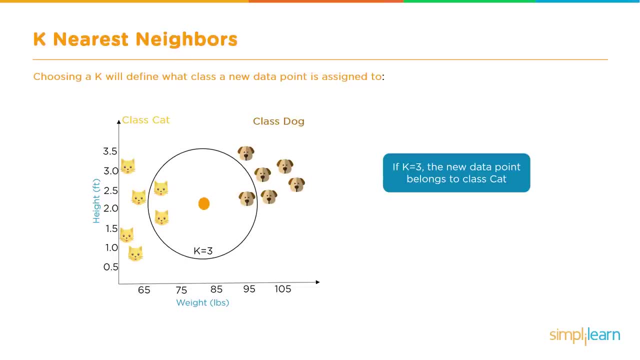 belongs to the cat class. Now what happens? if we say k is equal to seven? in that case these are the seven data points which are nearest to this new data point, And now you see that, instead of cats, dogs are more So, which means that now the point or this data or this new creature belongs to. 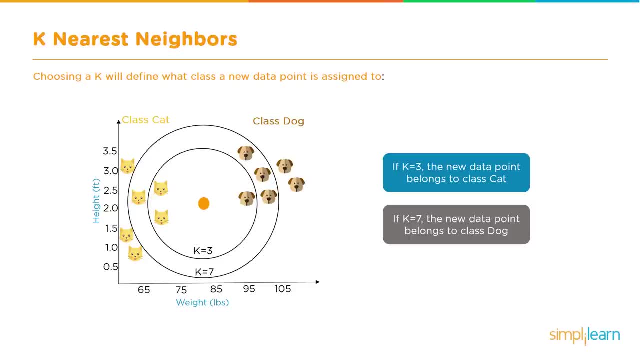 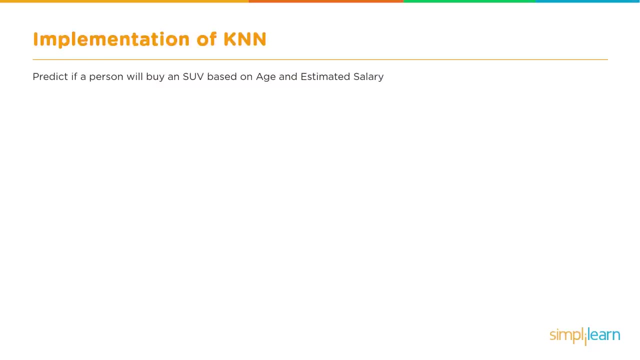 the class dog. So this is, while this is a slight drawback, but by trial and error we should be able to find out the right value of k And once we use that, that's how we train the model. Now let's use k nearest neighbors and take an example to solve one of our previous problems that we did. 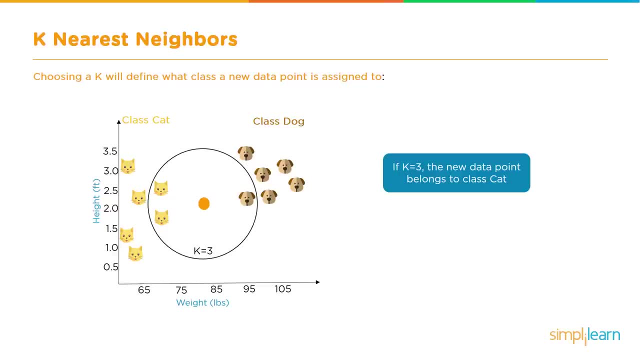 this data point And then we find out what is the maximum number of items, which class the maximum number of items belong to. So in this case there are two cats and there is one dog. Therefore, we determine that this new data point belongs to the cat class. Now what happens if we say K is 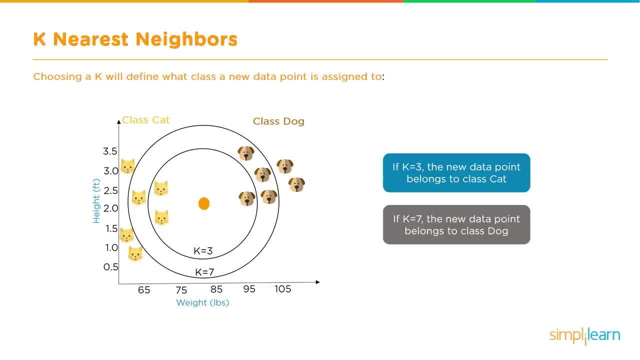 equal to 7?? In that case, these are the seven data points which are nearest to this new data point. And now you see that, instead of cats, dogs are more So, which means that now the point, or this data, or this new creature belongs to the class dog. So this is. while this is a slight 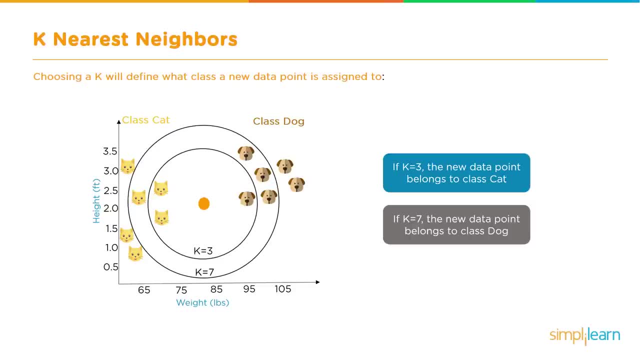 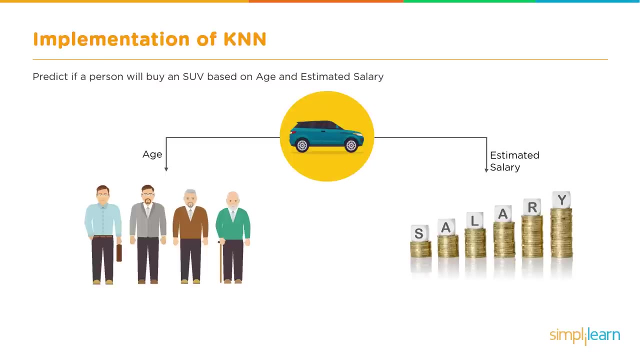 drawback. but by trial and error we should be able to find out the right value of K, And once we use that, that's how we train the model. Now let's use K nearest neighbors and take an example. So to solve one of our previous problems, that we did using logistic regression. whether a person 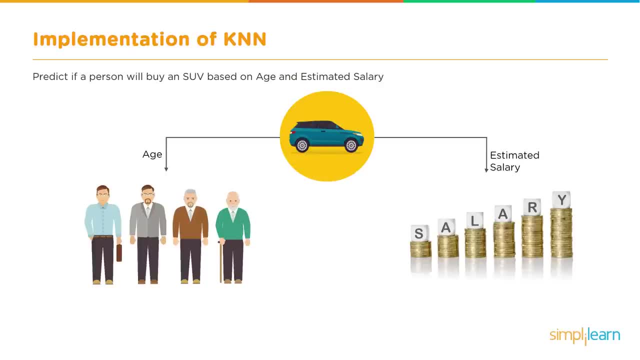 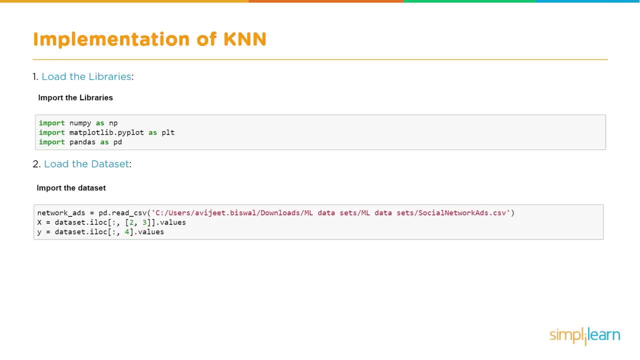 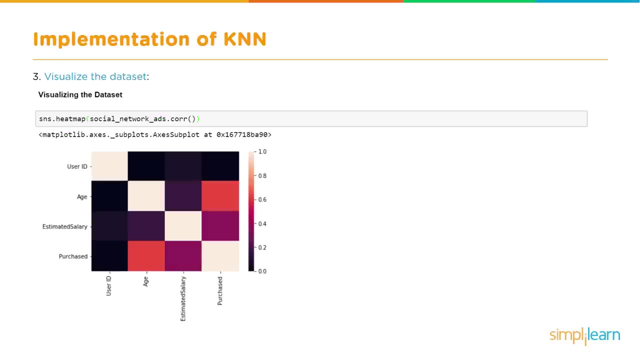 is going to buy an SUV or not, based on the age and estimated salary. So before we go into Jupyter Notebook, let's again take a quick look at the core. So what are the various sections in the core? As always, we import the libraries, we load the data set, we visualize the data, we split the. 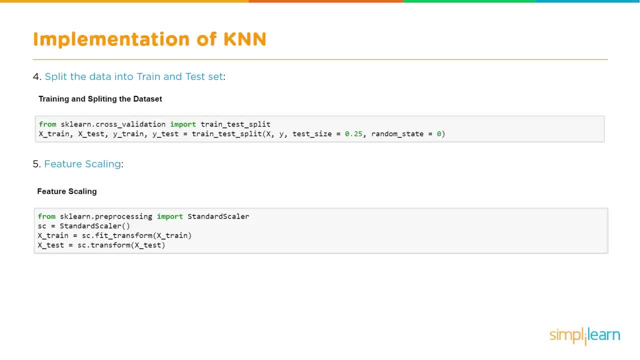 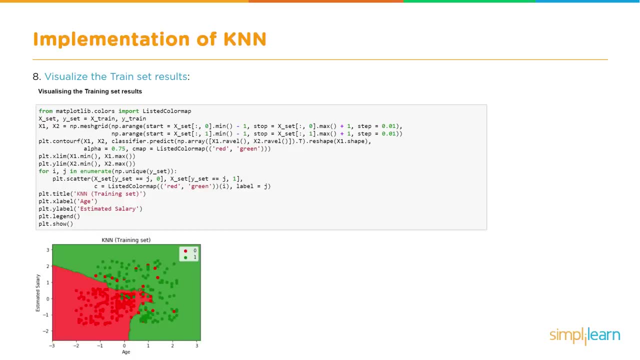 data into training and test data set. We do some feature scaling and then we train our model and then we test our model. We visualize the training set results and then we visualize our test results, And both of these seem to be looking pretty good. And then 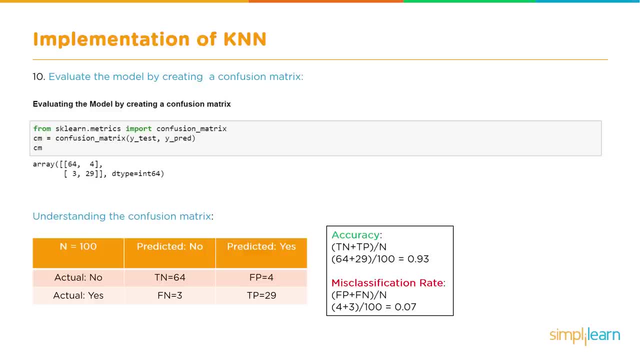 we evaluate our model using the confusion matrix. So remember, whenever we use a classification algorithm, the way to evaluate our model, to find out the accuracy of our model, is the confusion matrix. We have seen in logistic regression, we have seen in decision tree and now in KNN as well. 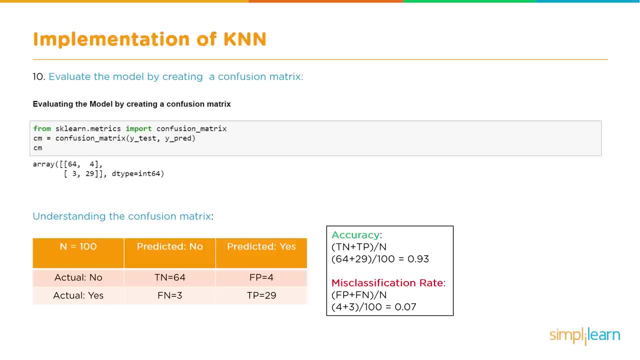 So in this case, once again, the total number of observations is 100. And we see that along the diagonal, which is the number we need to consider, there are 93 values, which means we achieve 93% accuracy and a few of them. 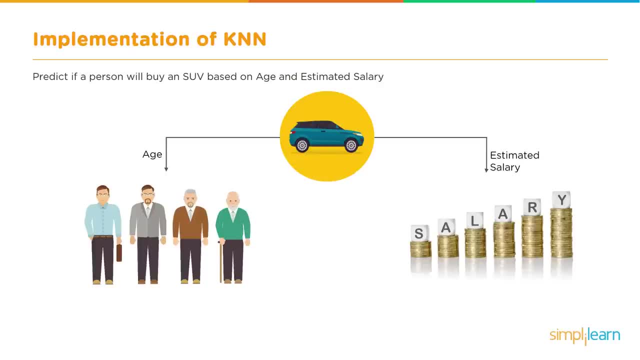 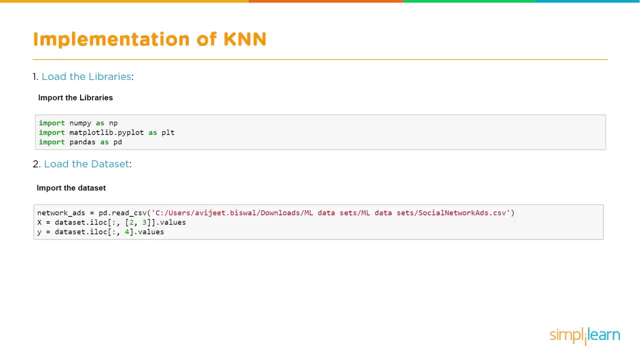 using logistic regression whether a person is going to buy an SUV or not, based on the age and estimated salary. So before we go into Jupyter Note, let's again take a quick look at the core. So what are the various sections in the core? As always, we import the 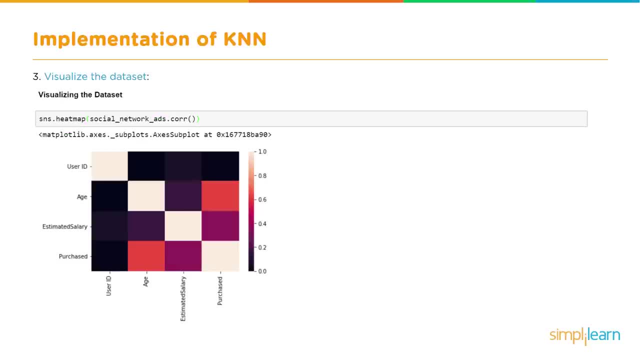 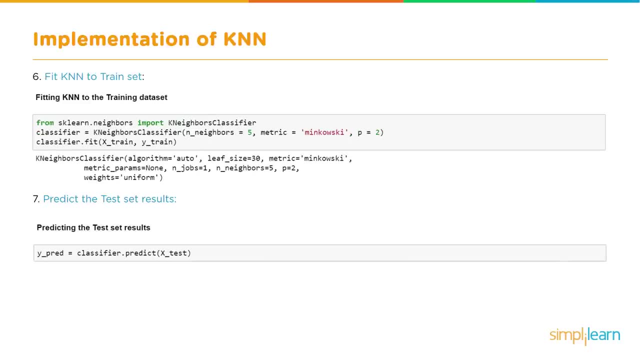 libraries. we load the data set, we visualize the data, we split the data into training and test data set. we do some feature scaling and then we train our model and then we test our model. we visualize the training set results and then we visualize our test results, And both of these. 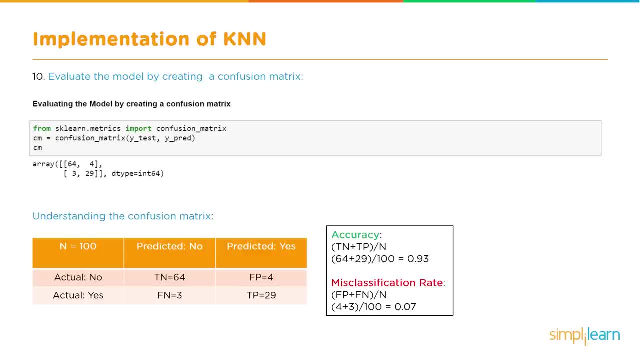 seem to be looking pretty good. And then we evaluate our model using the confusion matrix. So remember, whenever we use a classification algorithm, the way to evaluate our model, to find out the accuracy of our model, is the confusion matrix we have seen in logistic regression. 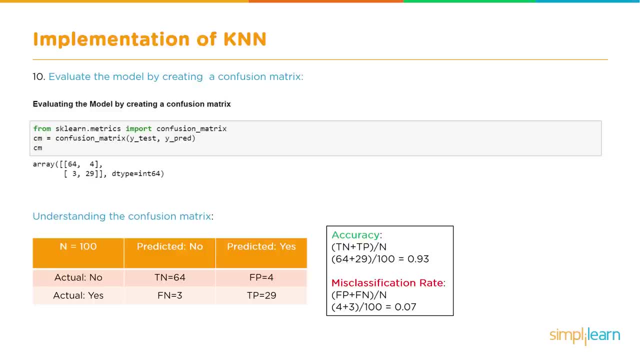 we have seen in decision tree and now in KNN as well. So in this case, once again, the total number of observations is 100. And we see that along the diagonal, which is the number, we need three values, which means we achieve 93% accuracy, and a few of them, that is, only seven of them, are. 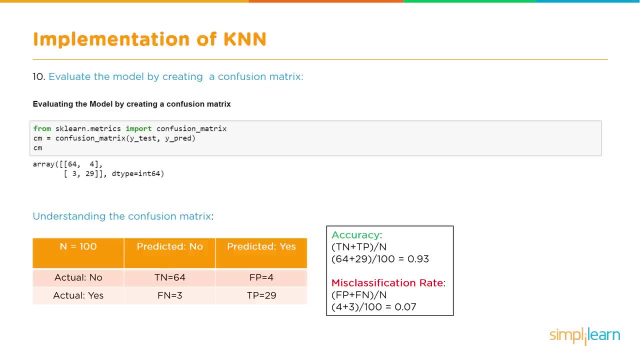 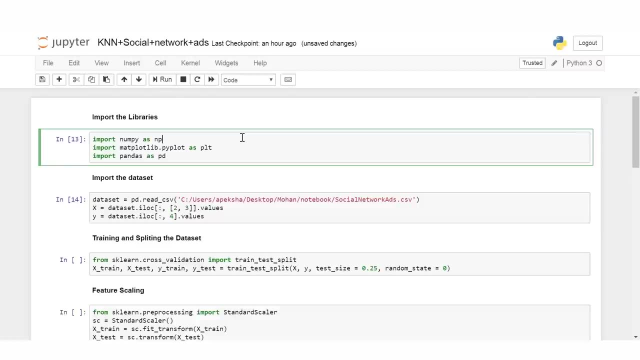 misclassified. So this is a pretty good accuracy compared to our previous example. So let's go and check how this looks in Jupyter Notebook. So this is my Python notebook for k nearest neighbor implementation And I will quickly walk you through this code. The first block is as usual. 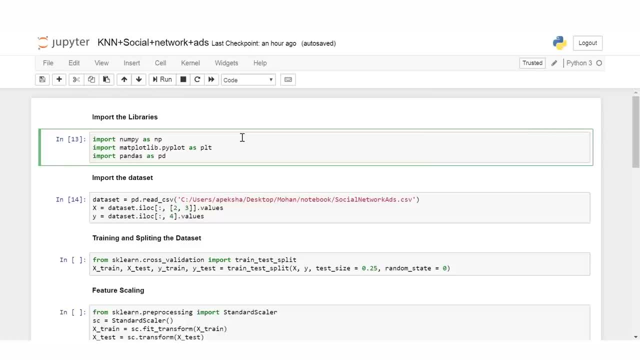 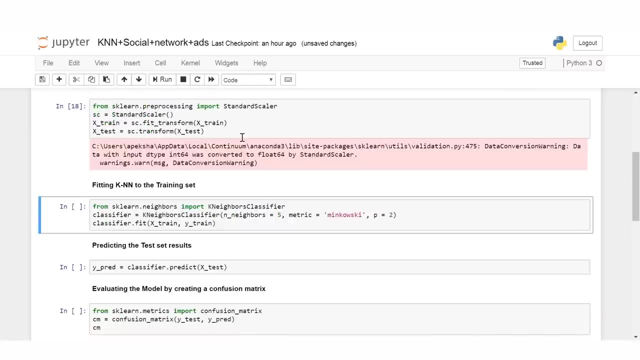 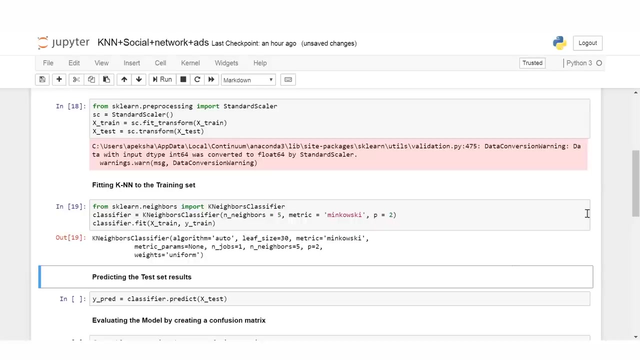 we are loading the various libraries like NumPy, pandas and matplotlib, And then we load the data set And we split the data into training and test data sets, And then we do feature scaling And then we start training our model, And here we are specifying k as five. Okay, And now the data set. 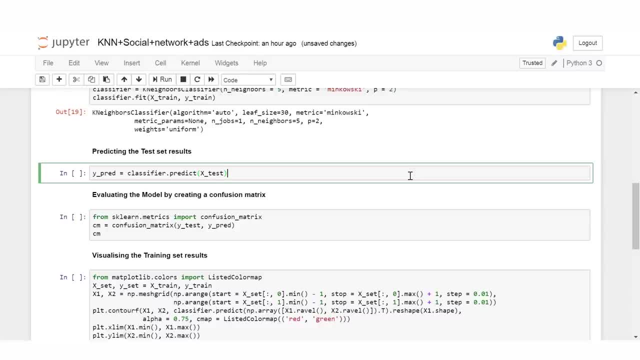 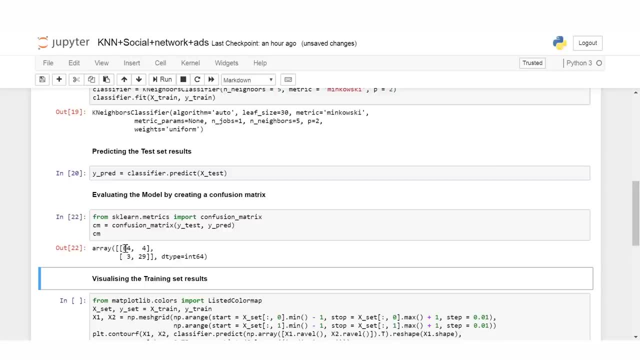 is trained. Now we go and test it with our test data set And here we are specifying k as five. And then we evaluate the model And here we get that, as you can see in the diagonal there are 73 entries, So total is 73, which means out of a total of 80,. 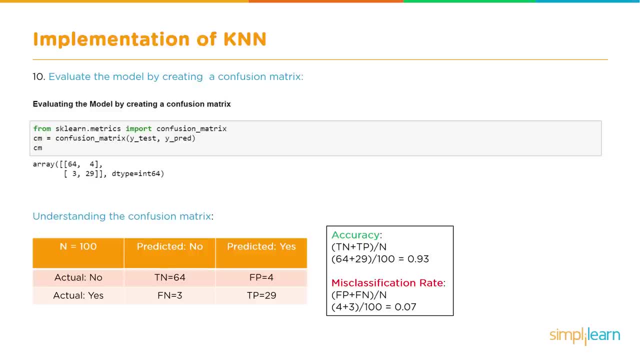 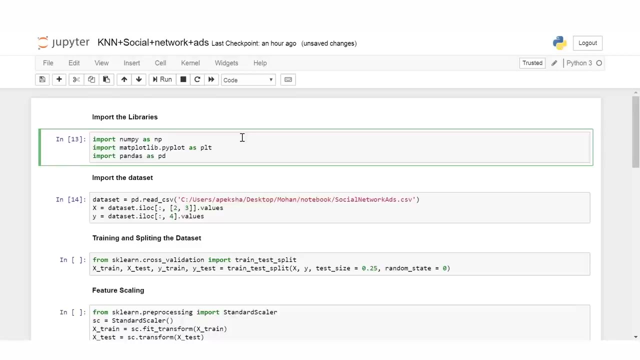 that is, only seven of them are misclassified, So this is a pretty good accuracy compared to our previous example. So let's go and check how this looks in Jupyter Notebook. So this is my Python neighbor implementation And I will quickly walk you through this code. The first block is: 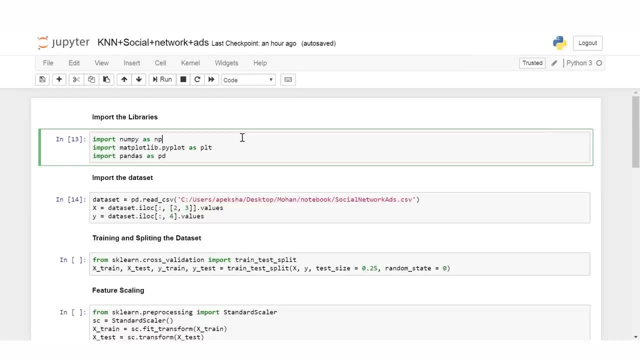 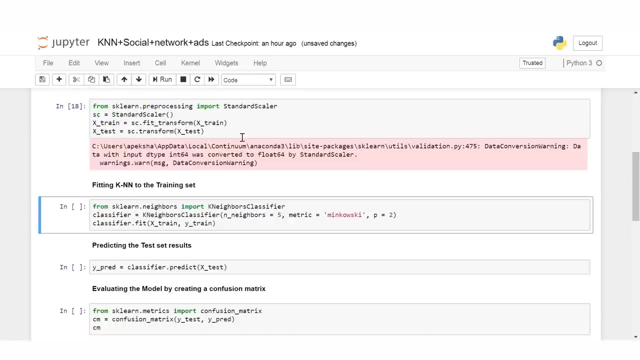 as usual, we are importing the various libraries like NumPy, pandas and matplotlib, And then we load the data set And we split the data into training and test data sets, And then we do feature scaling And then we start training our model, And here we are specifying K as 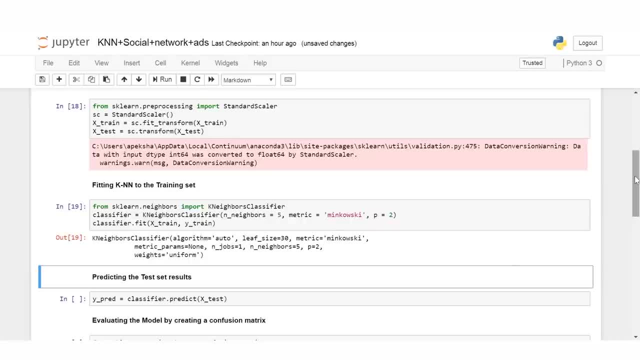 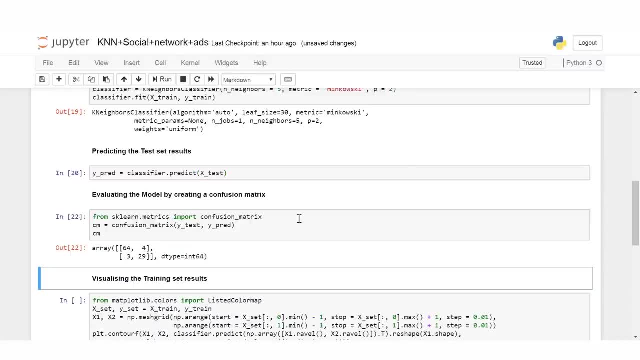 five. Okay, And now the data set is trained. Now we go and test it with our test data set, Then we evaluate the model And here we get that. as you can see in the diagonal, there are 73 entries. So 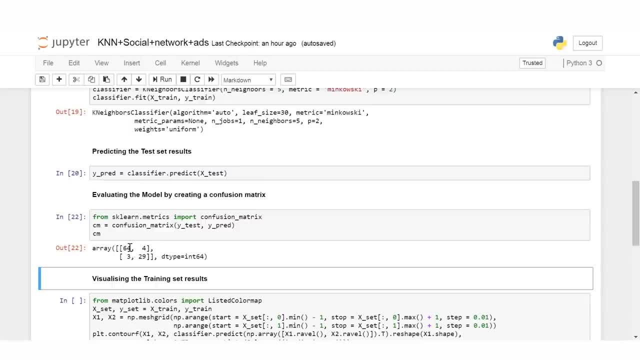 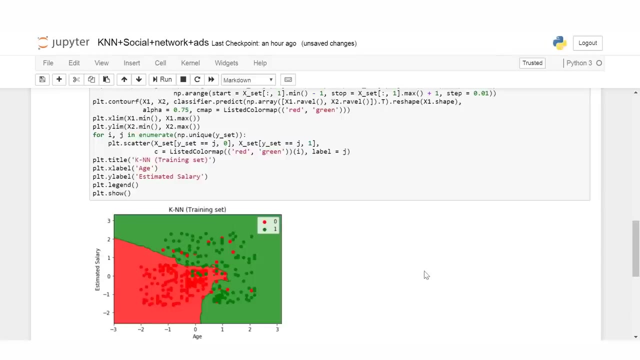 total is 73, which means out of total of 80,, 73 have been classified correctly, which is about 90% accuracy we are getting, And seven of them have been misclassified. We can now visualize the training results. So these are: 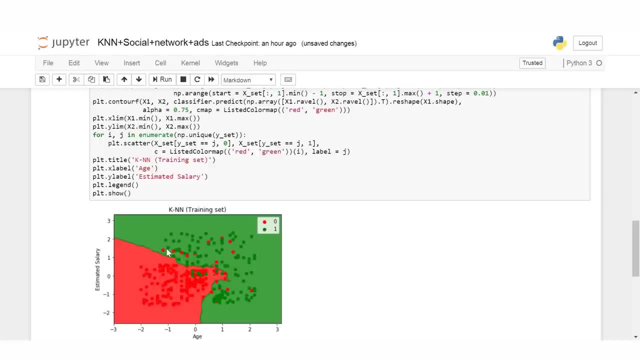 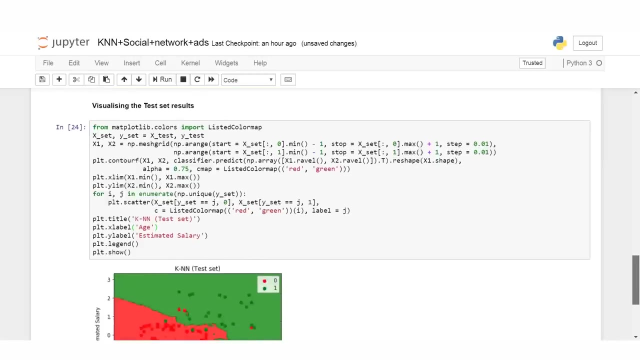 the zeros and these are the ones. This is the training set. So there are a few, as you can see, misclassifications. The green ones in the red area and the red ones in the green area are the misclassified values. And same way, we can check the visualize the results of the test data set. 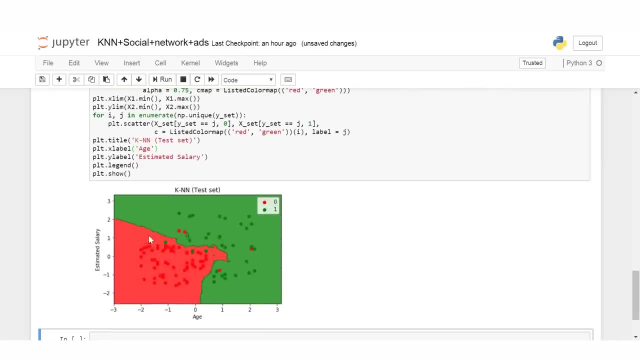 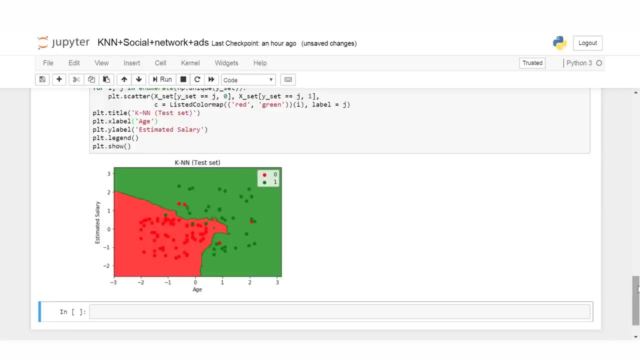 as well. And here again we see there are a few little bit of misclassification. And that brings us to the end of this Python notebook demo for KNN classification. So let's summarize what we have learned in this video. First of all, 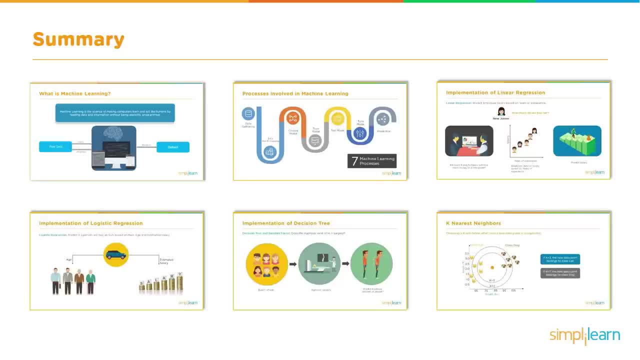 we started with an example of applications of machine learning, Then we learned about the definition of machine learning and then what are the various steps or processes involved in machine learning, And we then looked at some of the examples of machine learning rhythms. We took a look at linear regression, we then saw logistic regression, then decision trees.